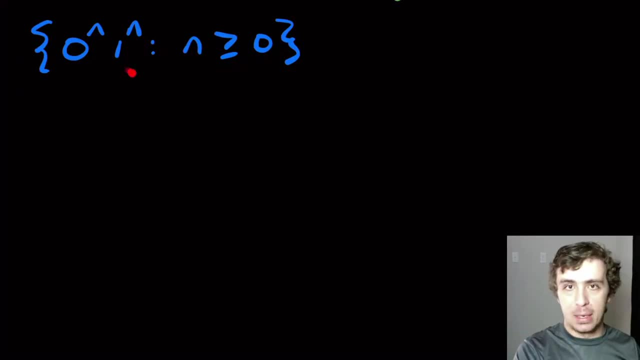 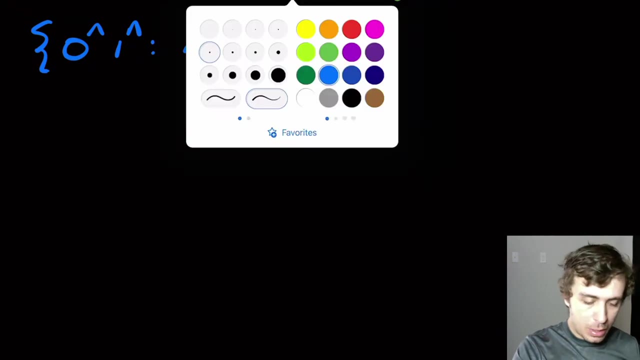 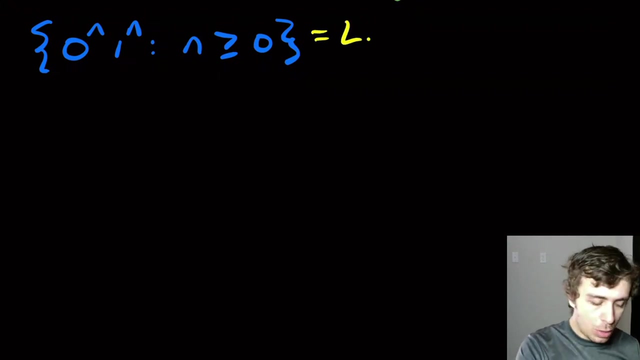 Okay, let's prove that this language is not regular. So how would you prove that this language is not regular? You always start every single proof of showing non-regularity by supposing that this thing is regular. So let's call this language L. So we're going to first suppose: 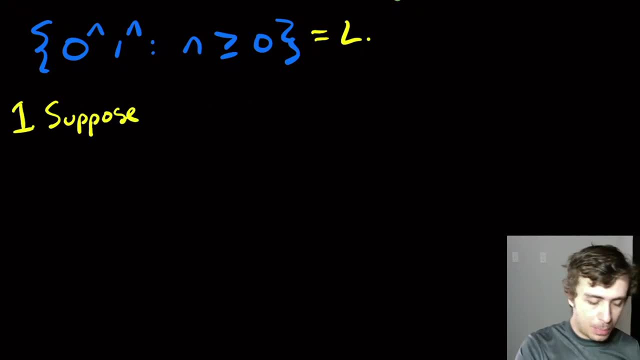 so this is the first step. suppose L is regular, Then what we need to do is: we know, we're assuming that L is regular, so that means that there is this pumping constant. we're going to call it p for this language, L, So there. 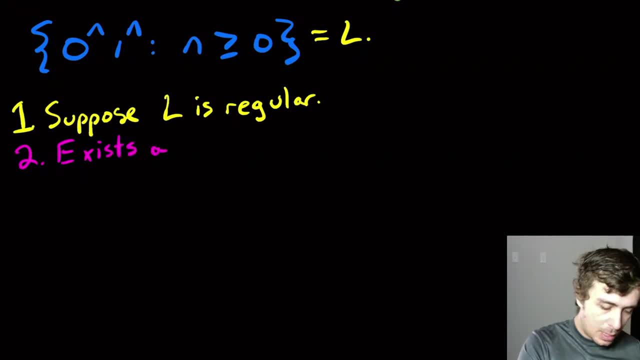 exists a pumping constant, constant p for this language, L, which corresponds to a DFA of that particular size, but we're not thinking of the actual DFA here. Okay, so there exists this constant, so now we got to pick a string that's in the language in length: total length at. 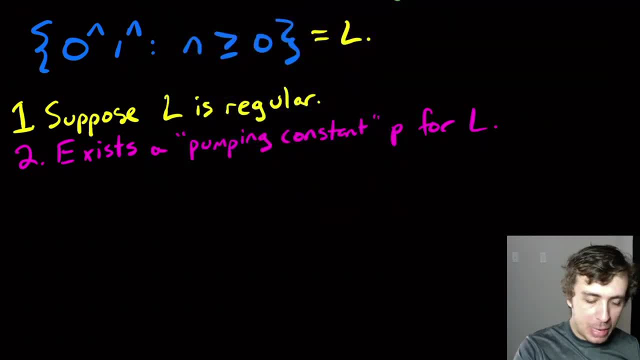 least p. So the typical strategy here is that there are a lot of strings that you can pick. The strategy is: whatever this number is, just substitute it in the exponent here. Well, there's only one type of exponent, it's just n. We're going to have more complicated. 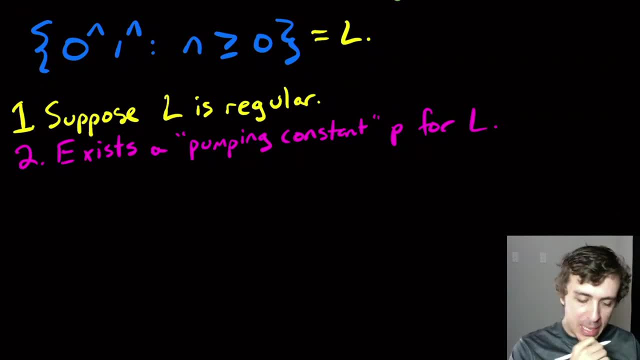 examples later. But here we just substitute this p in for n here. So what we're going to do is we're going to choose A string w to be zero to the p, one to the p. So I'm purely just substituting this p number in for. 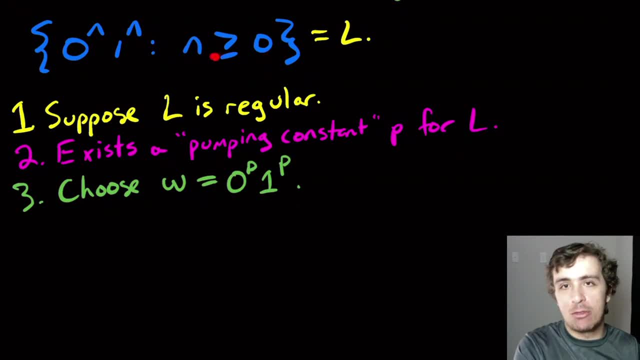 the n. Remember that n is a variable right here, because n ranges over all zero overall integers, at least zero. P is just some number. we do not know what it actually is. So I can't just pick the string zero one as an example, because I don't know that p is equal to one. P could be 10 trillion. 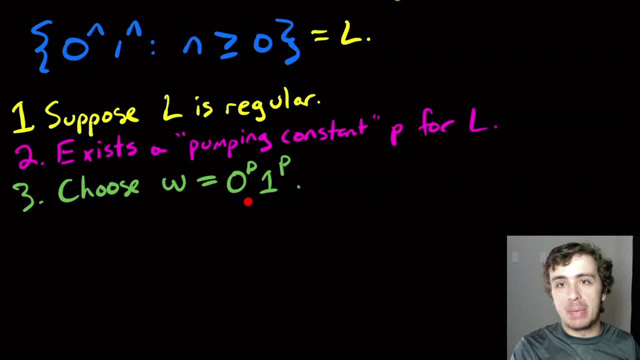 But this guarantees that the length of the string is at least p. In fact, it's at least 2p here, which is good, Okay. so what we need to do now is to look at every possible way of breaking this string up, because if we leave out any possible way of breaking it up, then it might be that that allows. 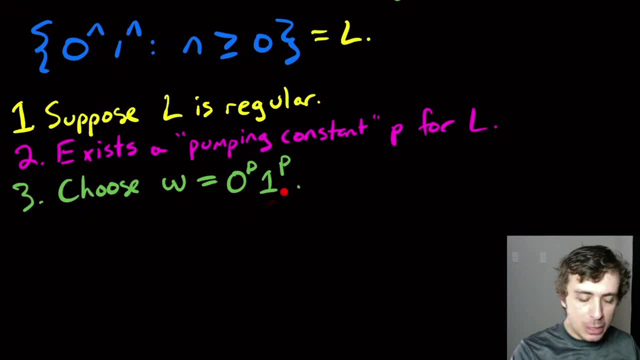 us to stay in the language forever. So if I show for every possible way of breaking the string up according to the rules And show that you can get out of the language at some point, then that means there's no possible way that this thing could have been a regular language, because it break the conditions of the. 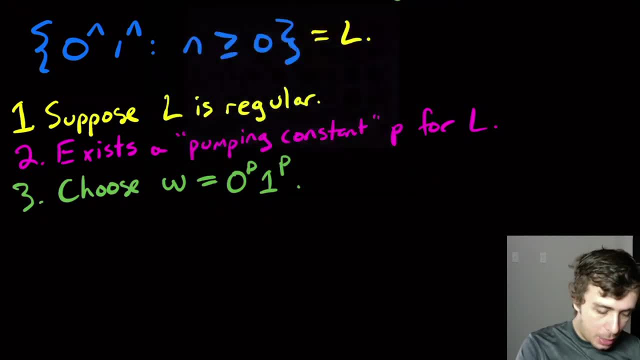 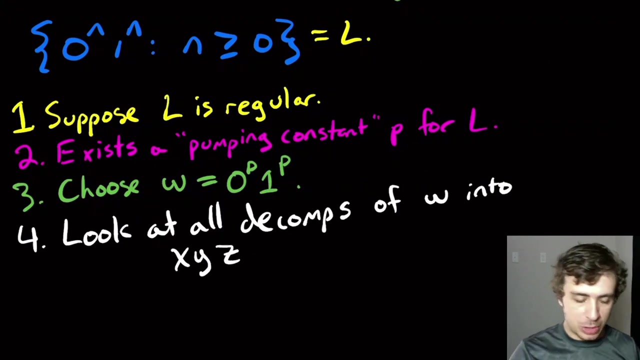 pumping lemma. So what we need to do here is to look at all decompositions. So look at all decompositions. I'm going to shorten it to decomps of spell, of correctly of w into x y z. I know other instructors use different variables. I'm just going to use x y z here. 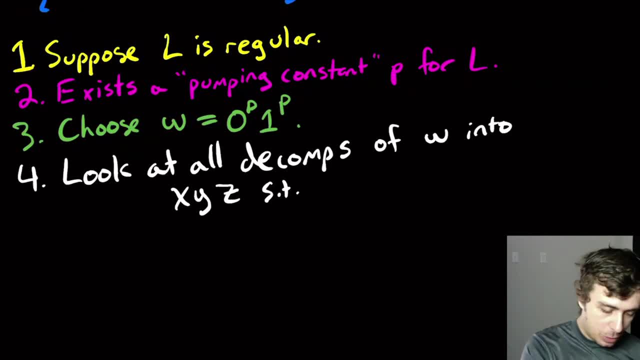 such that, well, remember the three conditions. I'm just going to call them a, b and c. Well, one of the conditions we're going to actually not do right now, the first two we're going to look at. So the first two pieces, x and y together, are, at most, p and the length of y. 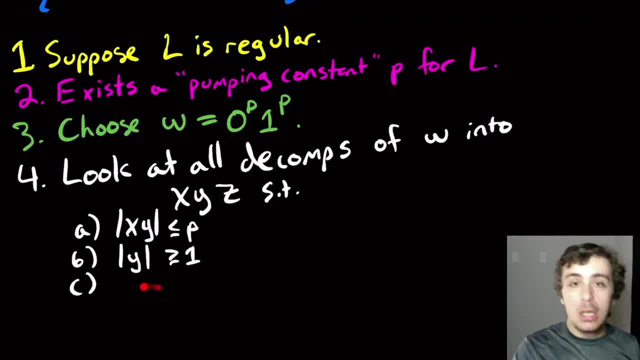 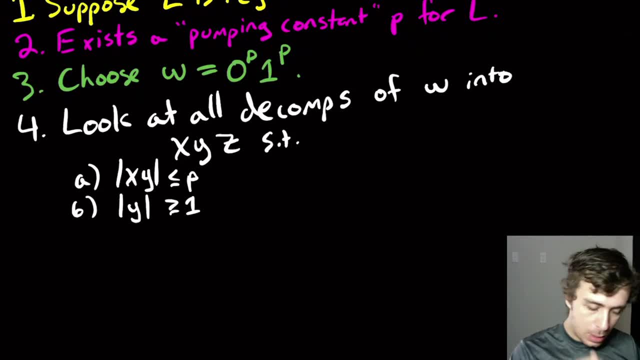 is at least one. The third condition that's going to allow us to get the contradiction that we care about. So, but we're going to leave that alone for now. So what are all the possible decompositions? Well, the x and y pieces are of length at most p. Well, the remember that x and y are the beginning. 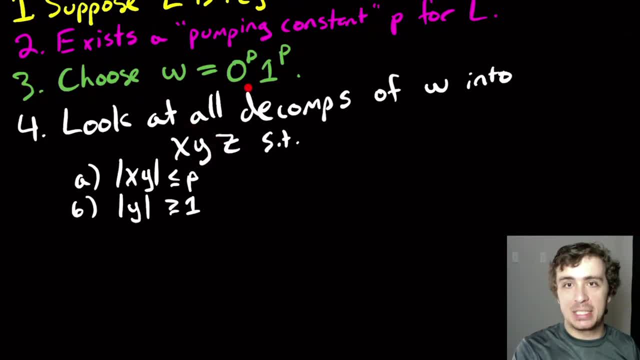 of the string. So look, x is at the beginning, y is next. So the beginning of the string, the first two pieces. So the first two pieces are at most p characters. So the x and y are entirely within the zeros here. So that means that, well, it could be that the x and y are a lot shorter than p characters, or it could 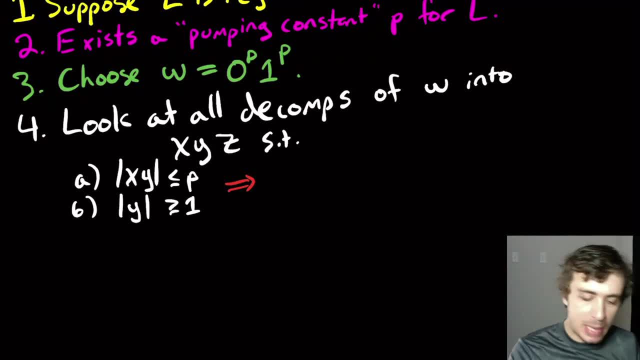 be all p characters. We don't know for sure, because we got to look at every possible decomposition. So all that we know is that x and y contain only zeros and no ones whatsoever. So x is going to be some number of zeros- I don't know how many, but let's just say alpha zeros. So alpha is the number. 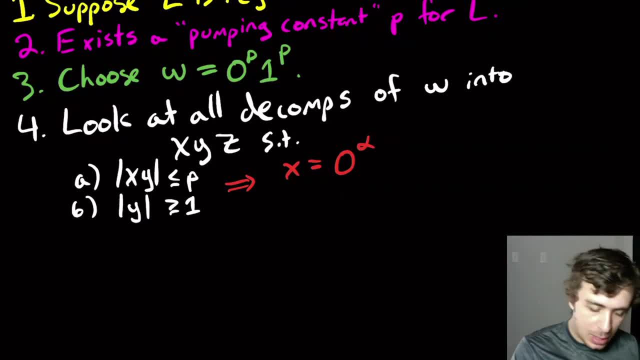 of zeros that x has is the length of x, and y could be a totally different number of zeros. I don't know for sure. Let's just call it beta for now. So what we know is that alpha is at least zero because x itself could be the empty string. Well, we know that y can't be the empty string because of the. 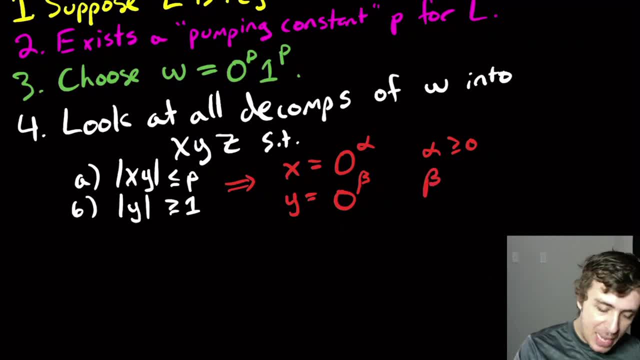 pumping lemma. So we know that the, that beta here is at least one. That's, that's all we know. And technically we do know that, although we're not going to use it, that alpha plus beta is at most p, because that's effectively saying this again: The length of x, y together is alpha plus beta. 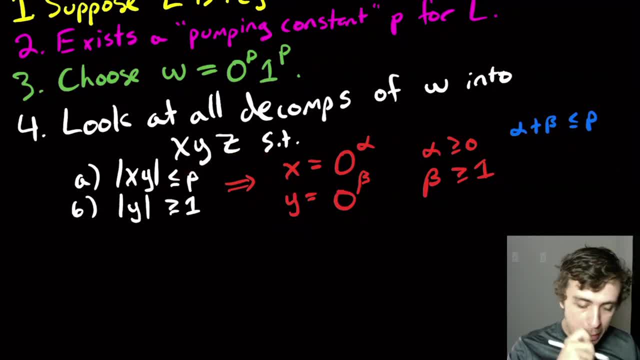 which is, at most, p according to this. Okay, so what we need to do is we need to choose an i, and we got to look at the string x, y to the i, z. So y to the i is y repeated i times. So what we? 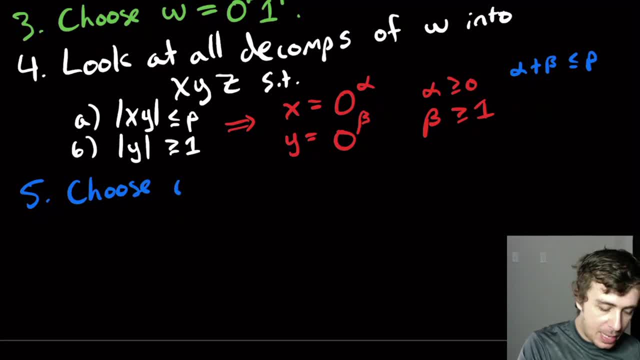 need to do is choose an i such that x y to the i z is not an l. Why do we want to do that? Well, the condition of the throat pumping lemma that I left out here says that no matter what value of i that you pick, you always stay in the language. But if I find one example where we actually leave the, 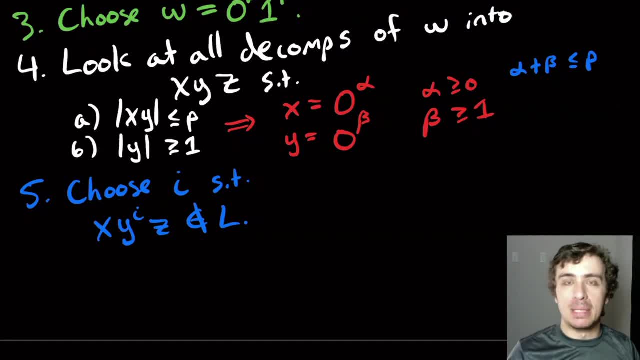 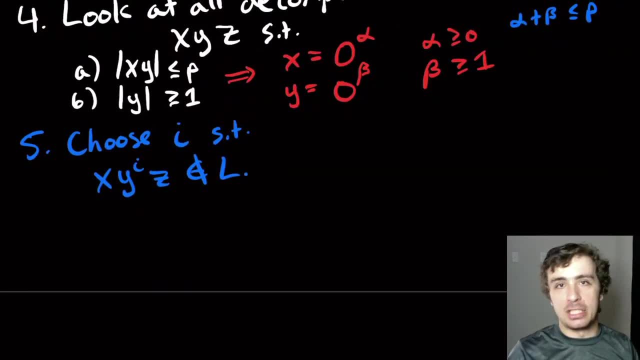 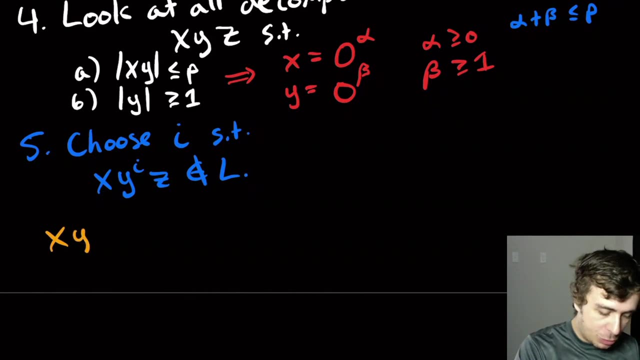 language, then that contradicts what the pumping lemma says, assuming that the language was regular. So that means that if we find an i that such that this happens, then the language is not regular. So let's, let's try to investigate what this is. So x, y to the i, z. Well, what I'm going to do is I'm 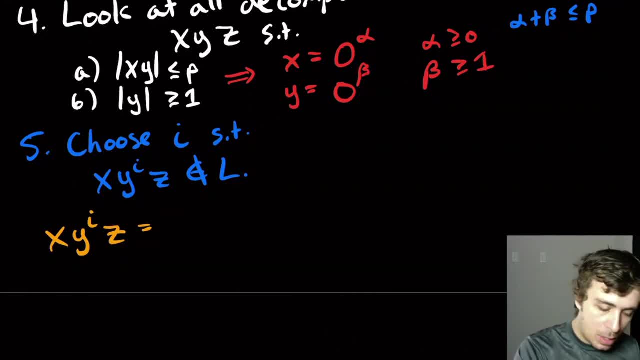 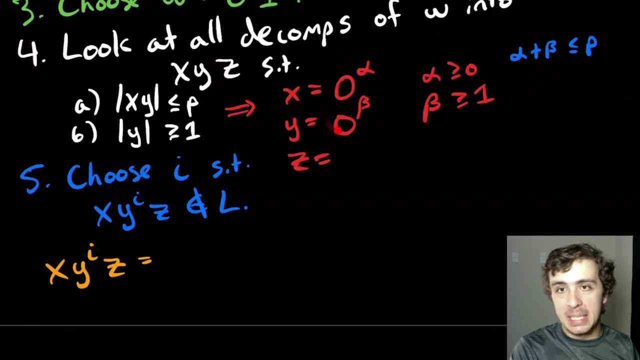 just going to copy and paste. I'm just going to copy and paste. I'm just going to copy and paste the pieces down. I actually need to say what z is. Well, we know that. z is the rest of the string. It's: we're breaking up w into three parts. Well, the first two parts were these two pieces here. 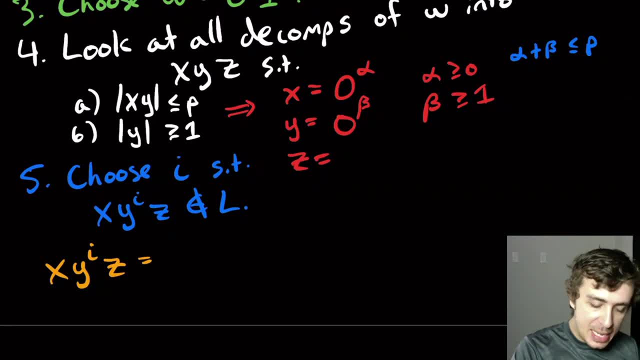 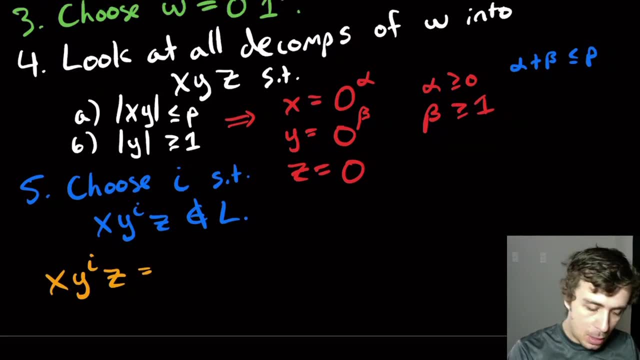 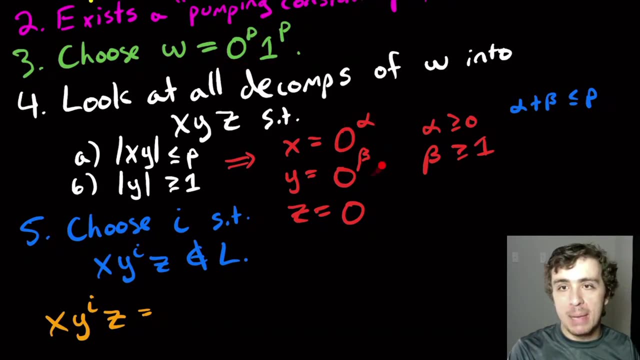 So z is the rest of the thing. So z is well, it's got to have some number of zeros. It might have none, but it has some number of zeros. We started off with p zeros right here. We took away alpha in this piece, We took away beta in this piece, So we're going to have p, which 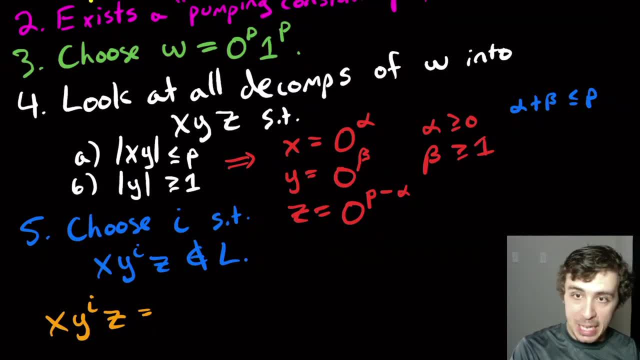 is what we started with: minus alpha, because that's what the x part has, minus beta, because that's what the y part has, And neither of the two pieces touched any of the ones. So the z part has all of the ones. So it's gotten greedy, It has all of the ones, All right. so then, what we need to do then down here, 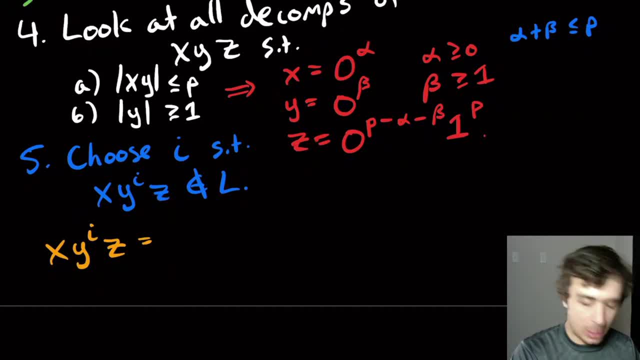 is just copy and paste these down here. So that's what I'm going to do. So I'm going to copy and paste the x part, which is zero, to the alpha We're going to have. i copies of y. So the number of zeros: 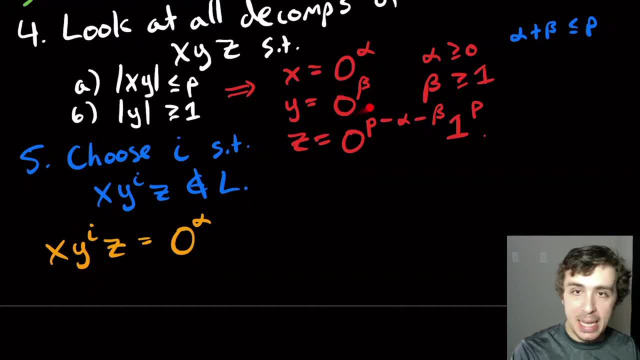 for this piece is going to be i times beta, because I have beta for each one of them and I have i of them. So I'm going to have i beta up here And then just copy one of the z's. So I'm going to have zero to the p minus alpha minus beta. 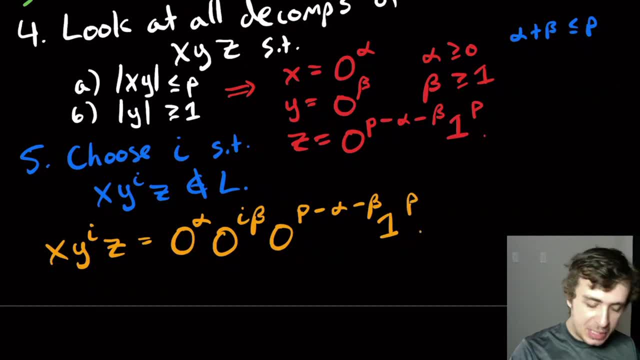 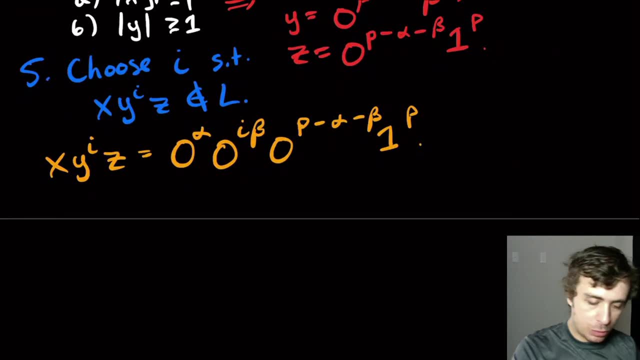 one to the p, And what we notice is that we have a whole run of zeros right here, So we can collect all of the exponents together, which is what I'm going to do. So if we just add them all up, well, we see that we have a plus alpha here and a minus here, So I'm going to 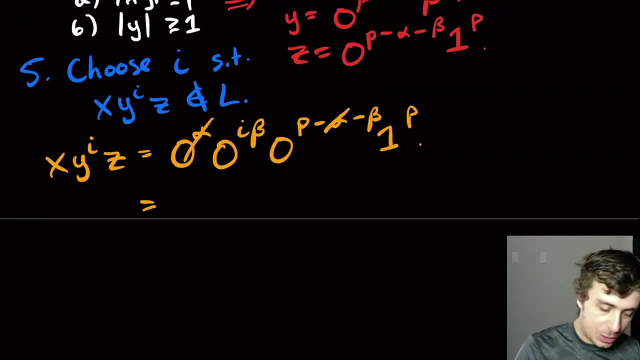 have the two z's. So that's what I'm going to do. So I'm going to cancel. I'm going to cancel those. So what we see here is that we have a plus- i beta and a minus- beta. minus i beta. 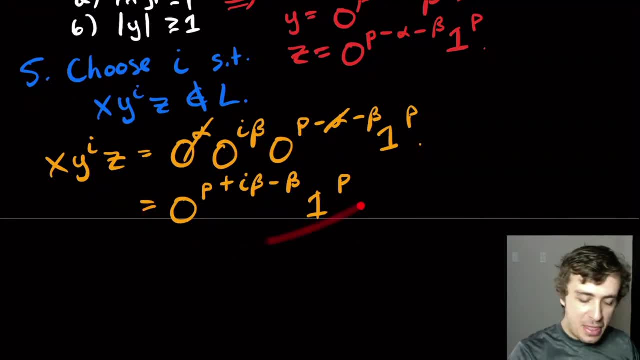 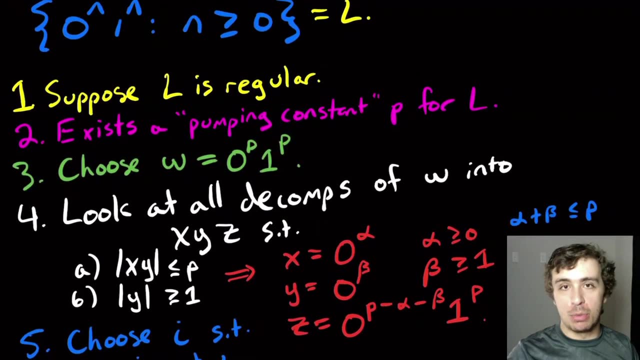 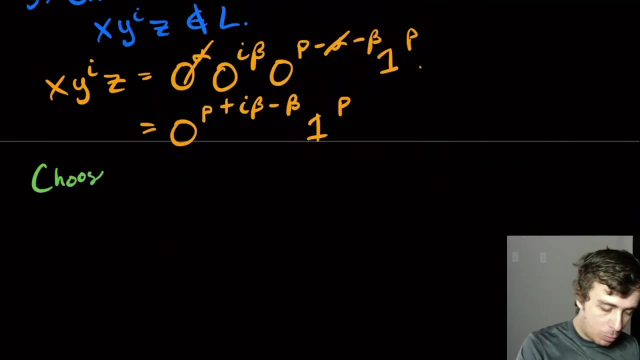 Those are going to cancel. So those two are going to cancel. So what I'm going to left with is zero to the p, plus i beta, minus beta, Because I have a plus i beta here and a minus beta here, And I still the language is. so what we need to figure out is choose an i, which is what we're trying to do. 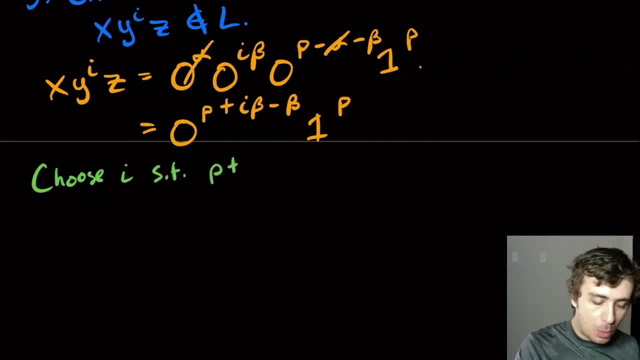 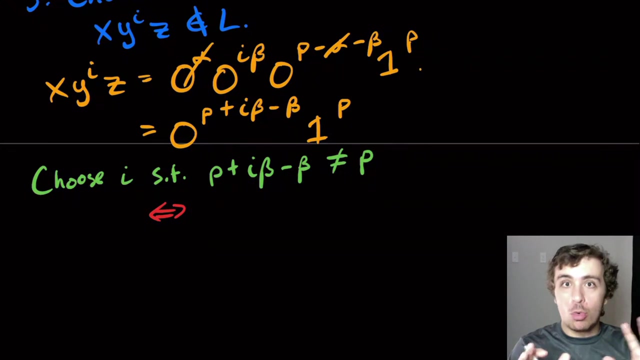 anyway, such that the two exponents are different. so beta plus i, beta minus beta is not equal to p. so then we see: okay, well, we got a p and a p here, so it's equivalent to saying: oops, so this is equivalent, it's. i'm not trying to work both sides of the equation here, i'm showing 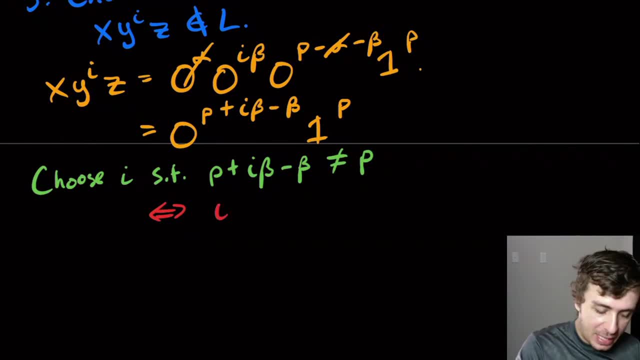 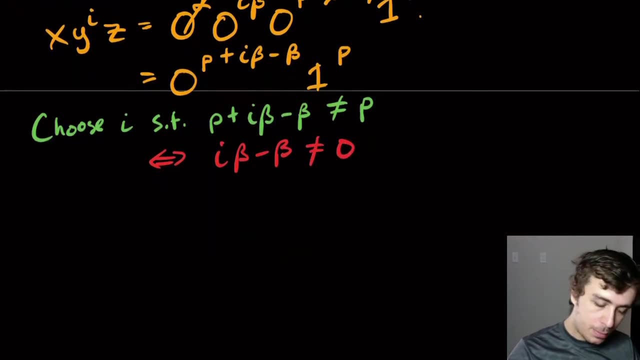 an equivalent statement. it's the same thing as finding an uh, an i, such that i beta minus beta is not zero, which is again equivalent to saying, if i move the beta over, i beta is not equal to beta and i'm going to divide by beta on both sides, and I'm allowed to do that because beta is not is at least. 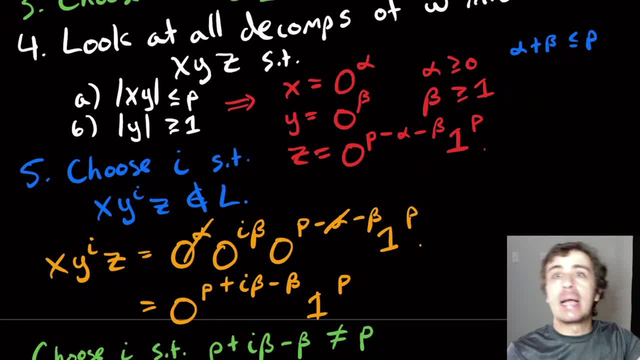 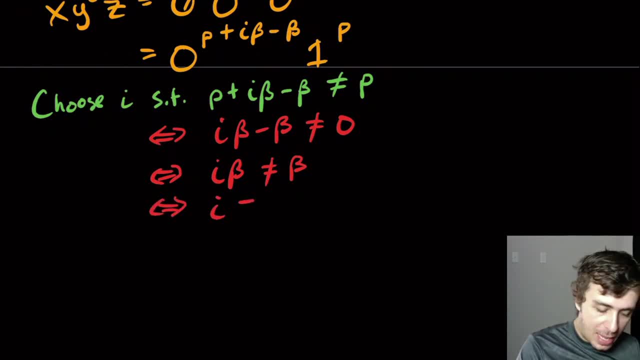 one, it's not zero. if it's something that's not zero, I can divide on both sides of the equation if I wanted to. so again, if and only if I is not equal to one. so I just got to pick a value of I. that's not one that will. it has to be at. 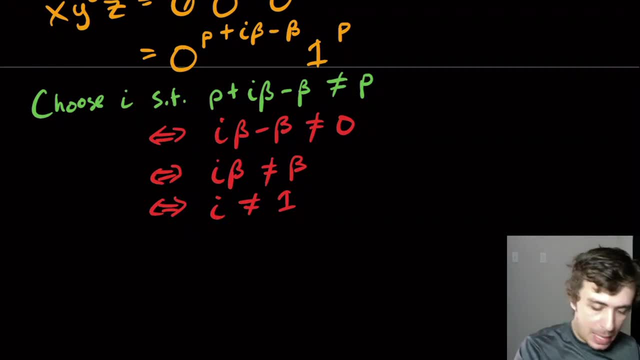 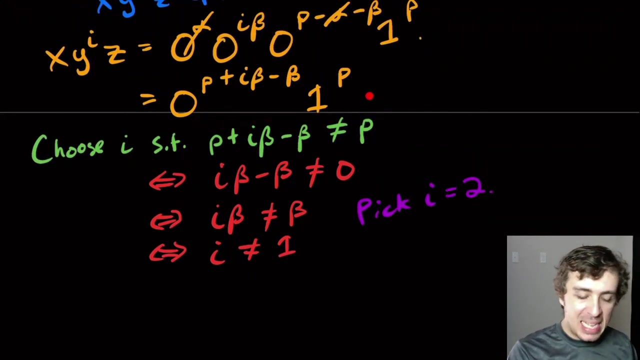 least zero, but it's not one, so let's just pick: I equal two. so let's pick: I equal to two. that's clearly not one. so therefore we have found an I, such that the resulting string is not in the language, and so therefore that contradicts the for all statement in the pumping lemma statement, and so therefore, 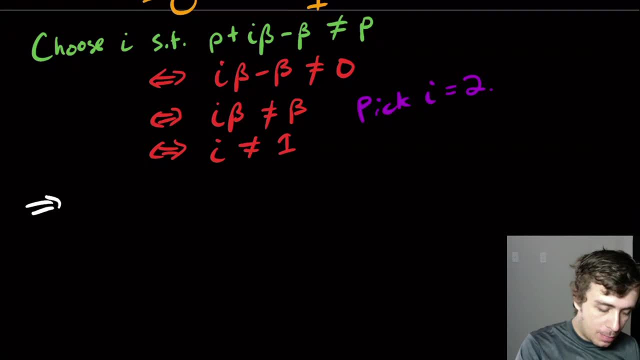 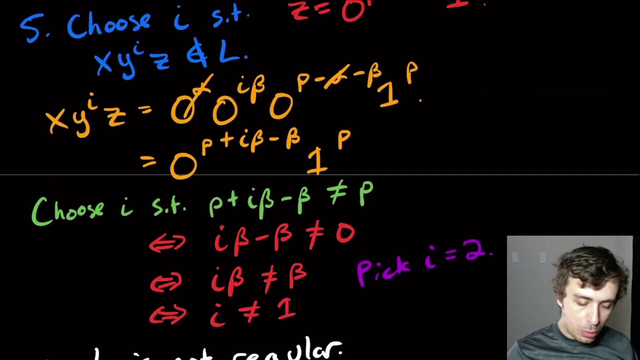 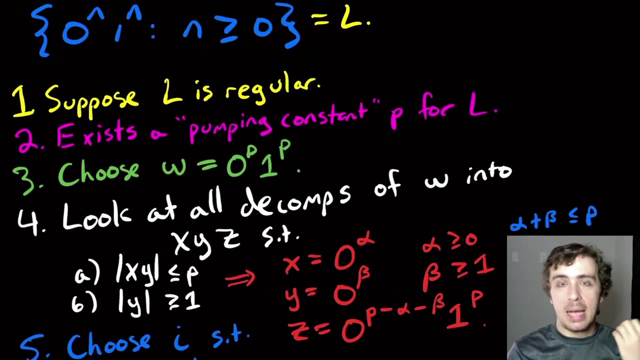 we're able to leave the language uh, and we looked at every possible decomposition of the string and so therefore, L is not regular. cool, so that effectively proves that this language is not regular. I've done it many times on the channel, but it's worth having a. 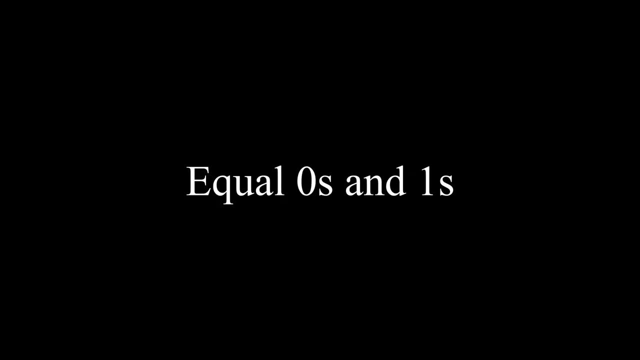 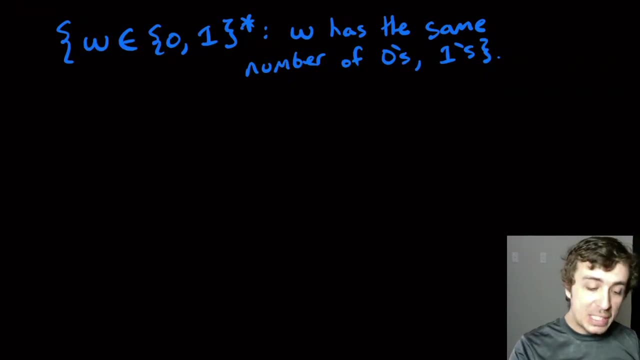 singular video about the topic. okay, so let's prove that this language is not regular. so it's the set of all strings over zero one star, such that the string has the same number of zeros and ones. so, as an example, if I look at the string zero one, zero, one that clearly has the 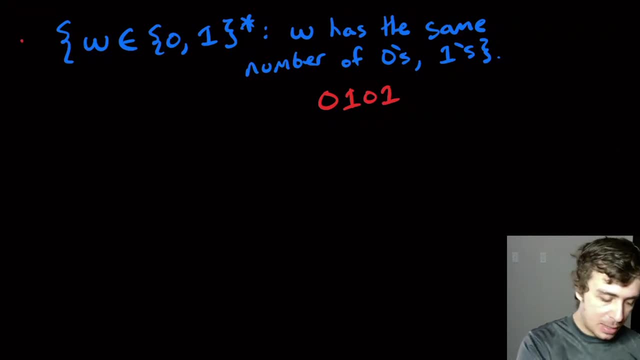 same number of zeros and ones in it. so that would be- let's call this language- L, so this would be in l. but if i look at the string, zero, zero, zero, one that has a different number of zeros and ones, and so that thing is not in l. okay, so i want to show that this thing is not regular. 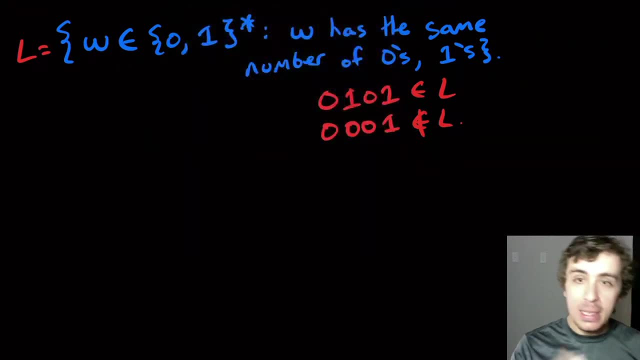 so there are actually several ways of doing that and one that's actually very straightforward. so i could go through the whole pumping lemma argument again and i will do that, but there's one way that you can do it which is really quick was let's actually i'm going to call this language- 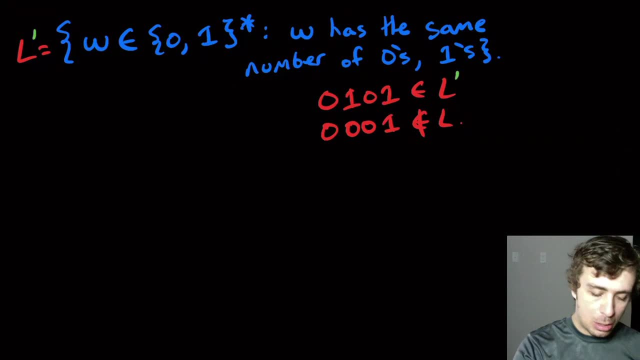 l prime. for now i may switch back to l, but i'm just going to leave it as prime. so let's look at l? l prime. well, it's kind of like the- the zero to the n, one to the n? example. it's just slightly different in that we have any ordering of the zeros and ones, but in the zero to the n, one to 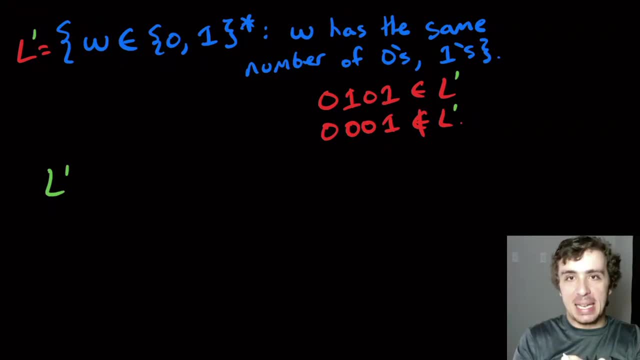 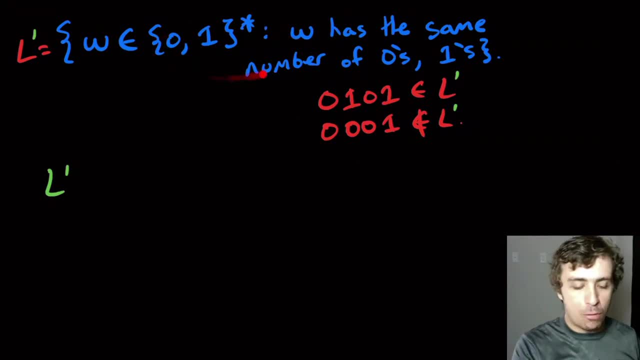 this without changing the regularity of whether this thing is regular or not, and it turns out we can. so what i'm going to do is i'm going to intersect this language, this, uh, same number one right here, with the set: zero star, one star. so we know that. 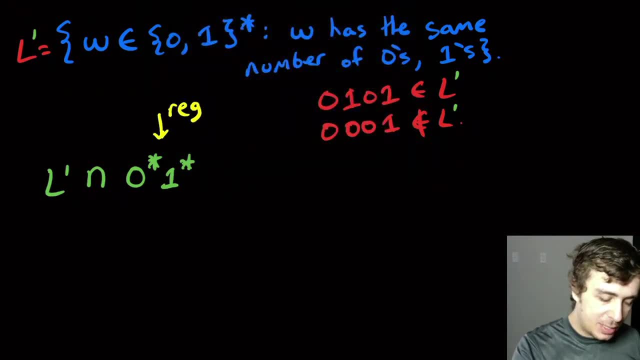 this thing right here is a regex. because it is a regex, so if this thing is regular, so if l prime is regular, then regular languages are closed under intersection and so, therefore, this thing is regular. but what is this thing? well, what is this set? well, it's the set of all strings that have a same number of zeros and ones, and the zeros come first. 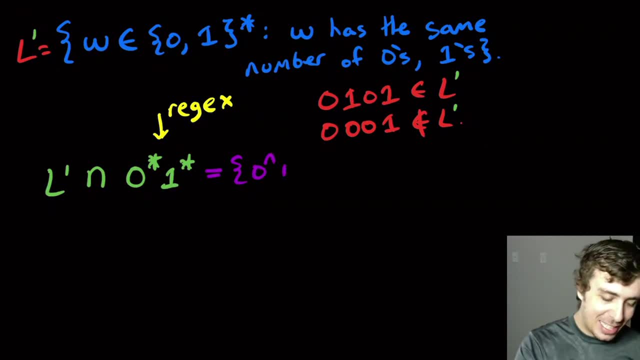 and then the one second. well, that's just, that's just zero to the n one, to the end. and we know already, because we've proven it before, that this purple thing is not regular. and so if l prime is regular, then the right hand side is regular, because we know this thing. 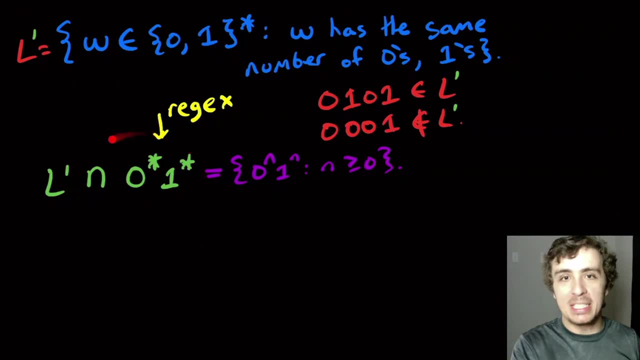 is regular. so the only possible thing, way that this thing could not be regular, is if the left thing is not regular. and so if the left is not regular, then the right hand side is not regular. that proves that it is not regular. so from that we can we have effectively. 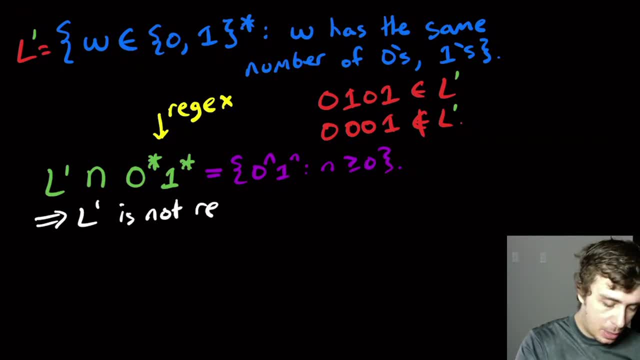 shown that L prime is not regular. but suppose that we wanted to prove this straightforward without any closure properties whatsoever. well, the thing that we can do is use the proof of zeros, the end ones again not being regular, verbatim, except changing L for L prime. because why, in fact, I have the proof. 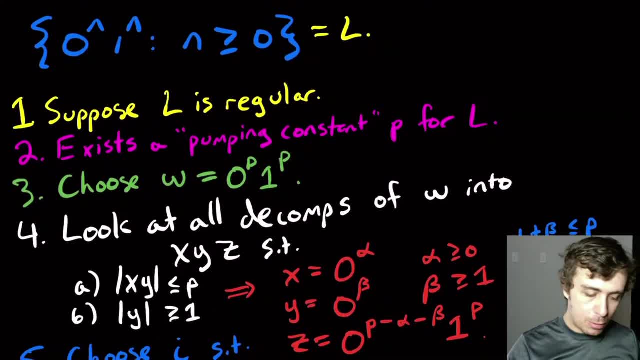 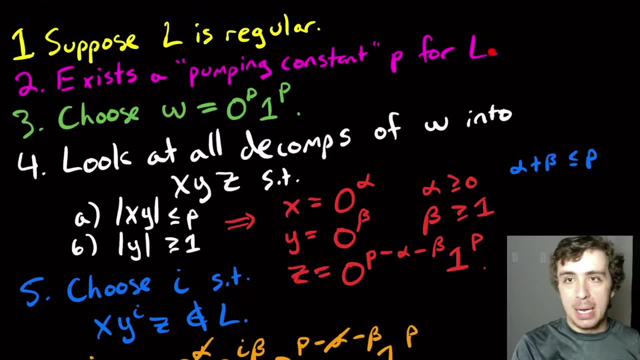 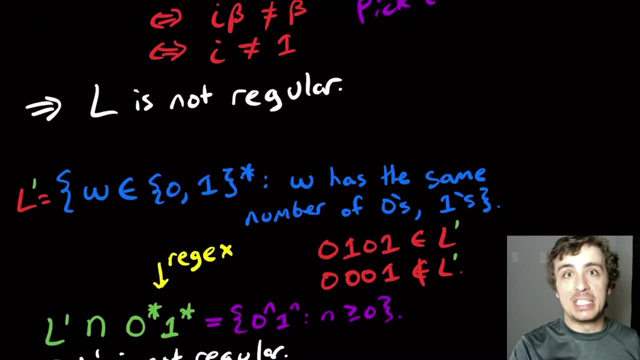 right here. so we have. we've shown before that zero to the n, one to the n is not regular. well, let's see. so suppose I just change this to L prime, L, prime. well, here this string is in the bottom language because it has the same number of zeros. 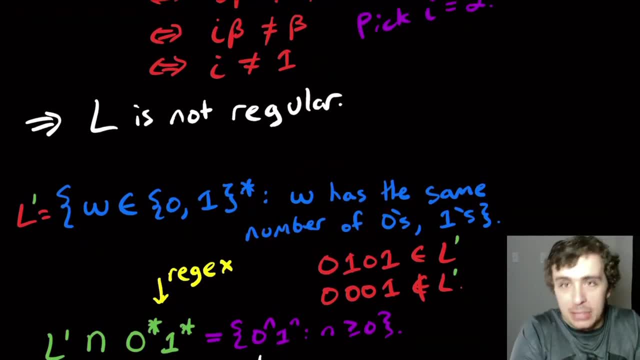 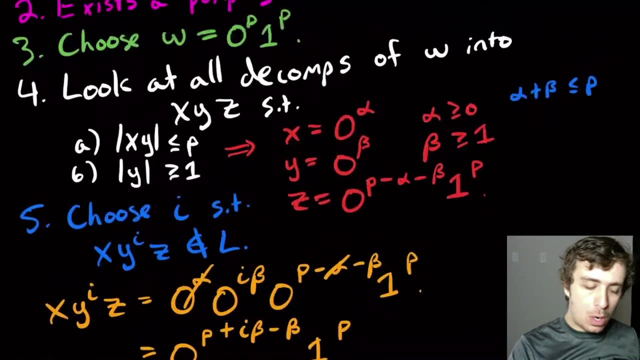 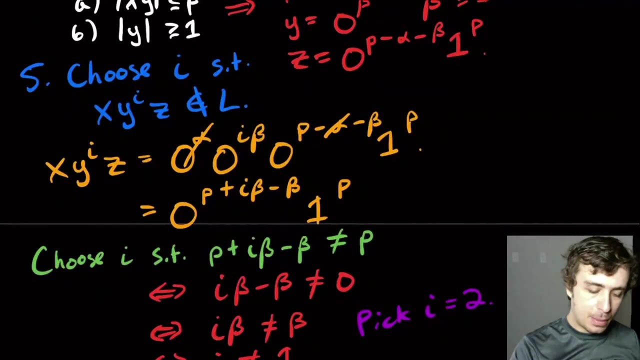 and ones. we don't enforce any ordering here. so as long as it has the same number, that's all right. so we can just change it to L prime, L prime, L prime, all we care about. so here it's the same string. therefore, all of the decompositions are exactly the same. so so this is exactly the same. well then, if 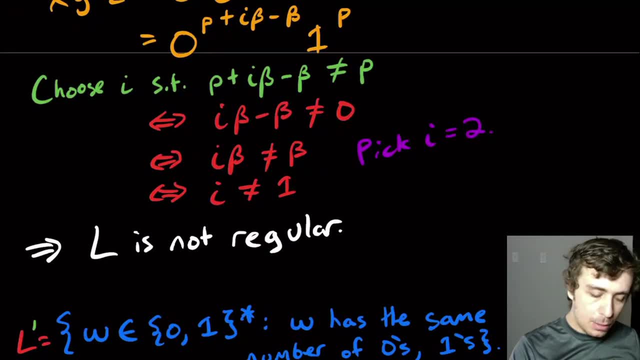 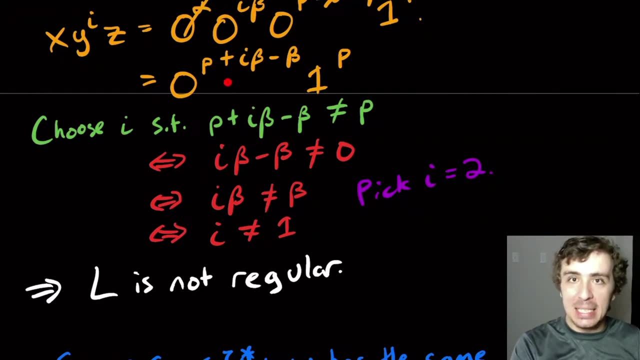 we look at the resulting string, which is: which is this one right? here the condition of being in the language is exactly the same, because we're not changing where the zeros are over here. so we didn't have a structural problem with zero to the n, one to the n, where you. 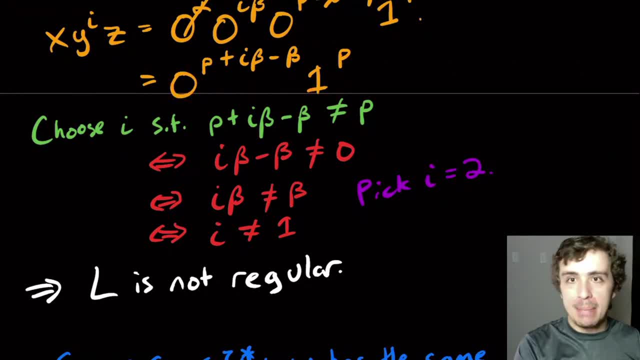 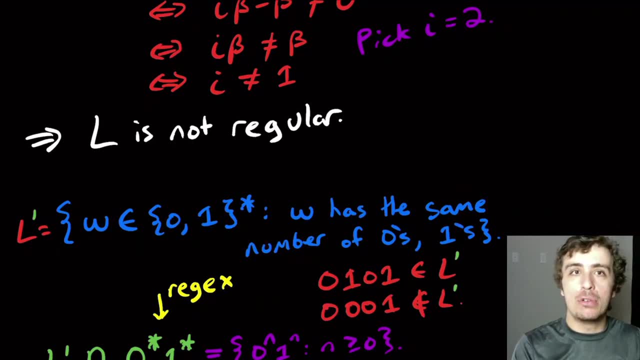 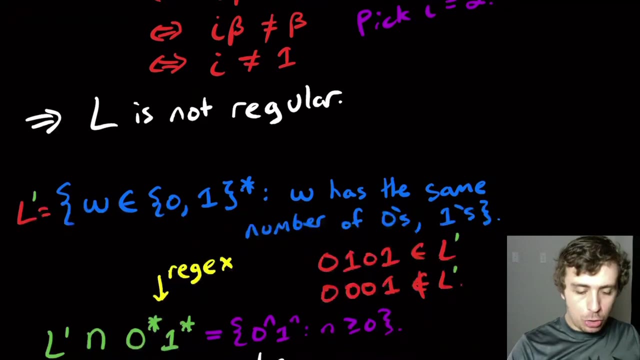 have. we're just checking the set whether they're the same number or not, which is exactly what this condition is, so, effectively, we can use the exact same proof as the zero to the n, one to the n example, which is pretty dang cool. so what? my advice is trying to use either closure properties or use the proof, or 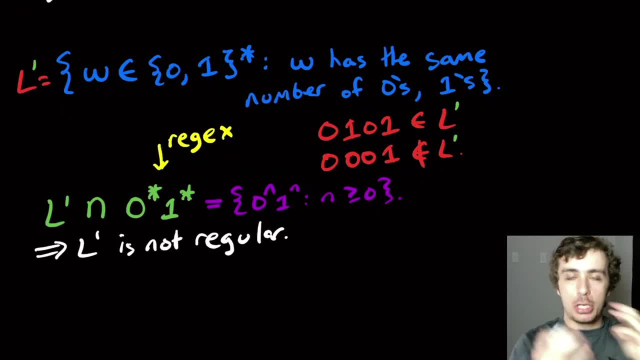 adapt the proof of some other language to use for this language and it turns out to be very, very powerful. another closure property technique which isn't very effective here, but we may see it later- is to use say like complement. if the language that we started out with is regular, then the complement language is. 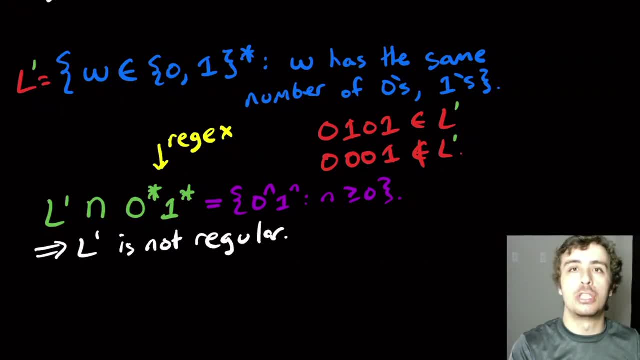 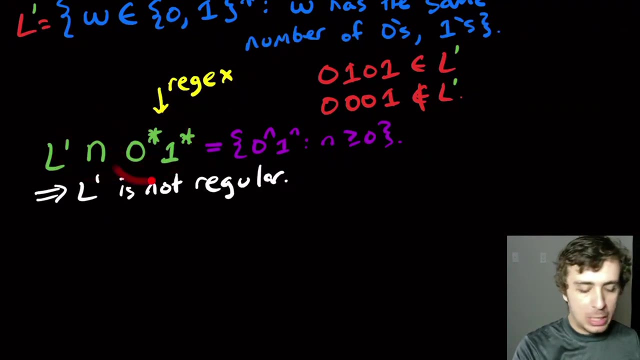 also regular, because regular languages are closed under complement. so if we can show that the complement is not regular, then that shows that the original thing is not regular, and sometimes that's a lot easier. so often we intersect things with regexes like this. it preserves the regularity of whatever this is actually. 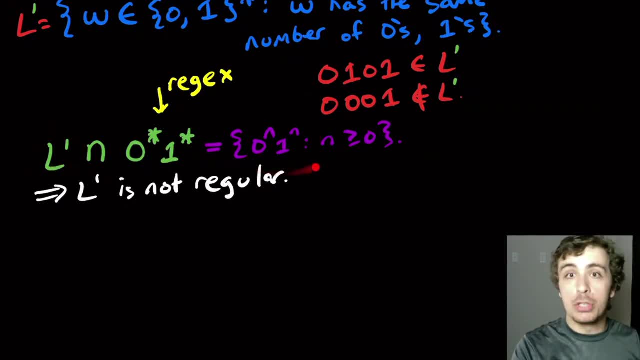 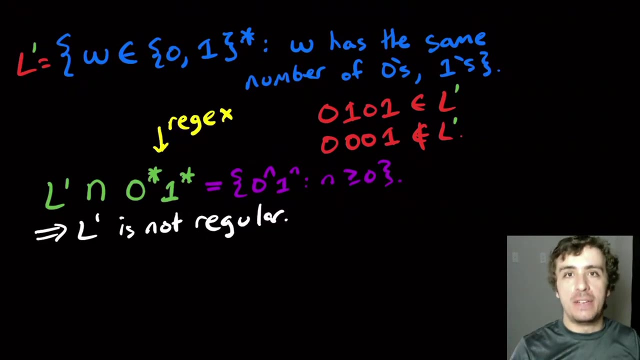 it doesn't. but if this thing is regular, then the resulting thing is regular. so then the contrapositive is: if the resulting thing is not regular, than the original thing couldn't have been regular, so it preserves the regularity in that sense. so use these techniques, it's very, very useful. 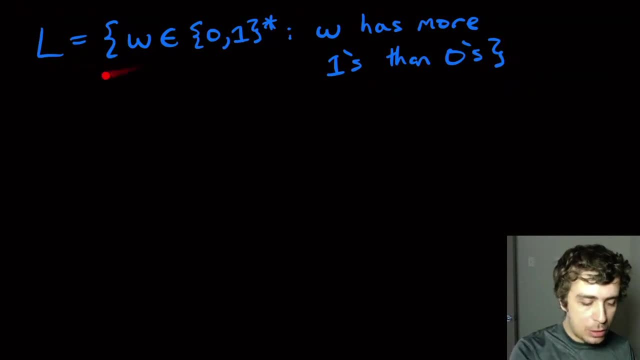 all right. so let's prove that this language, which I'm going to call L, is not regular, where W is a any string and zero one star, and W has more ones than zeros. so let's start the proof, as we normally would. so we would suppose that 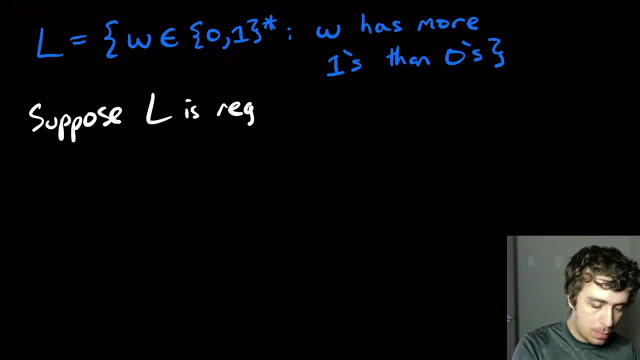 L is regular, then of course there exists a pumping constant P for L. so there exists a. I'm just going to shorthand it to call it the variable P for L, just for simplicity. so now what we need to do is we need to pick a string that's in the language and at least P characters long. so I've got a. 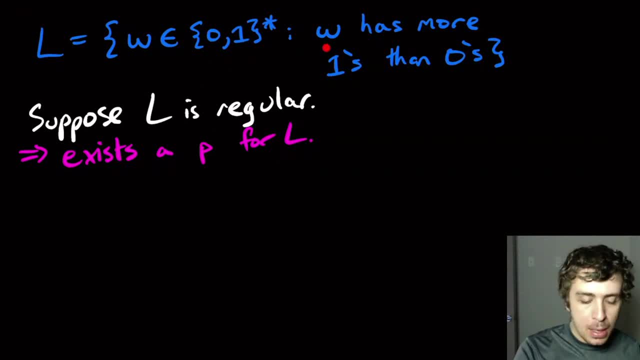 pick a string and a string and a string of two Shu, and my entering is principal g because the ден's champion of L to go, that's a .103. there are many that I could pick where W has more ones than zeros and has P. 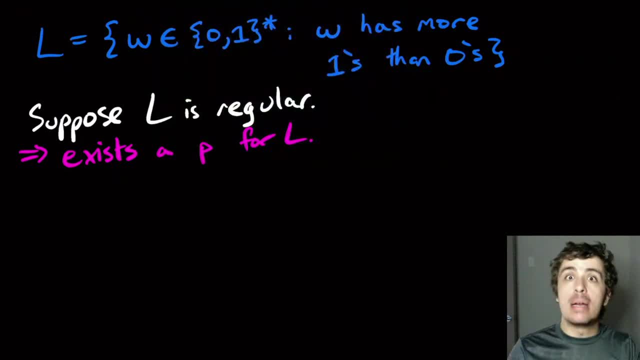 characters in it. so we could just try to model a proof like 0 to the n, 1 to the n and let's choose the following string: so let's pick. 0 to the P. well, I gotta have more ones than zeros, so let's pick. let's say P plus 1, okay, so I could pick. 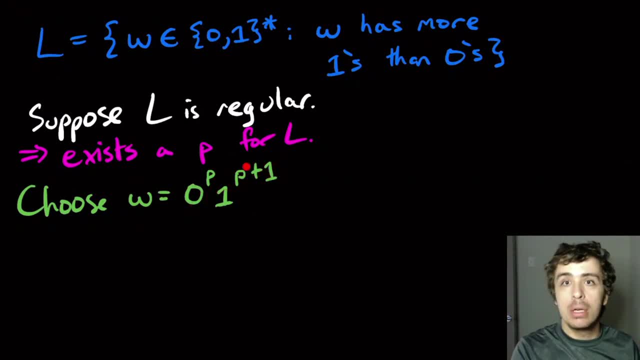 P plus 2, because that's more ones than zeros. also, I can't pick 0 to the P, 1 to the P no plus 1, because then it would not be in this language. it's got to start in the language and then we pump out of the language. okay, so then what do? 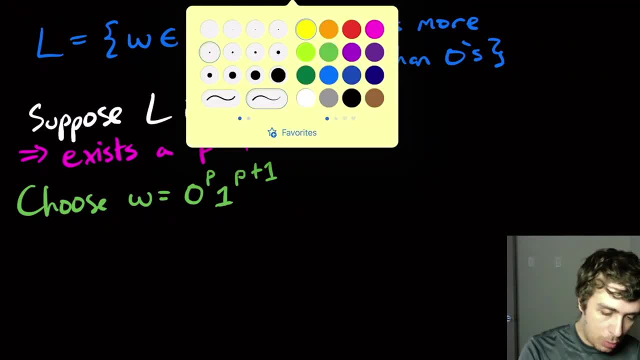 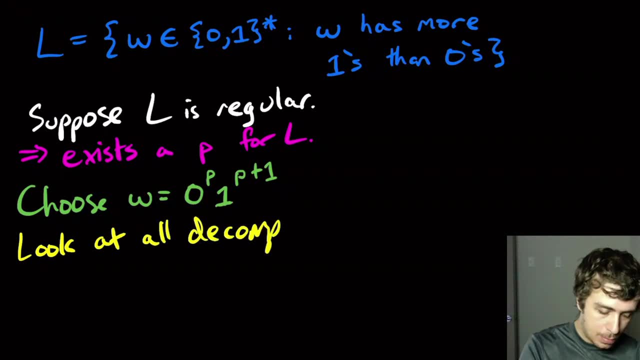 we do here. well, we got to look at all decompositions, as we always do. okay, so then, what do we do here? well, we got to look at all decompositions, as we always do. so we got a look at all decompositions of W into those three pieces X, Y and Z. 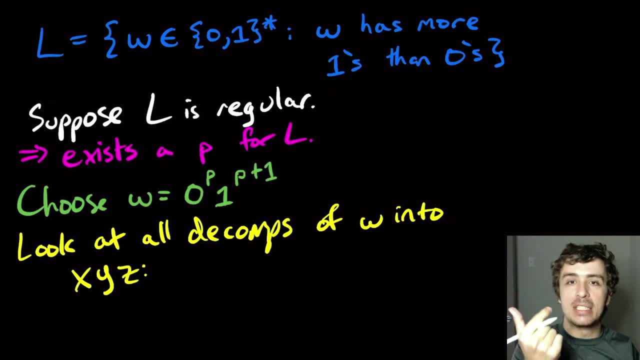 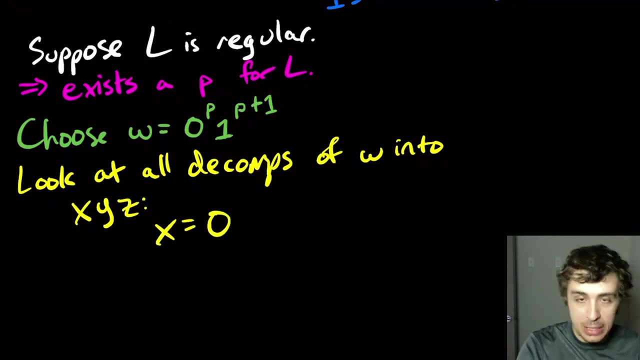 according to the rules that X, Y has length at most, P and Y is not empty, so Y has at least one character. well, since X and Y have at most P characters and the first P of them are zeros, that means that X and Y only have zeros in them. so we know that X is going to be some number of zeros. let's 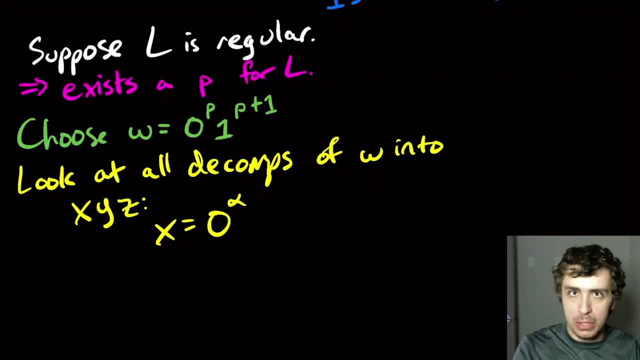 just call it 0 to the alpha. so alpha is the number of zeros that X has, or just the length of X. that's the same thing, and why it could be a totally different number of zeros. I have no idea what it is. I know that beta must be at least one, because y has to be non-empty and C is. 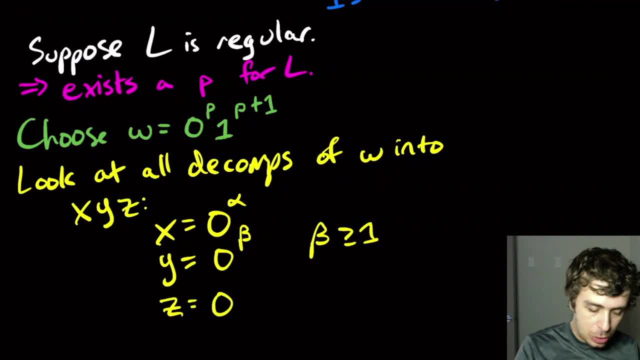 the rest of the string because we're only three parts and just like the zeroes will come and go, will follow numbers, so you can find that there are a zero and Z is the number of zeros that X has, or just the length of X of the string, because we're only three parts and just like the zero to the n one to the n proof. 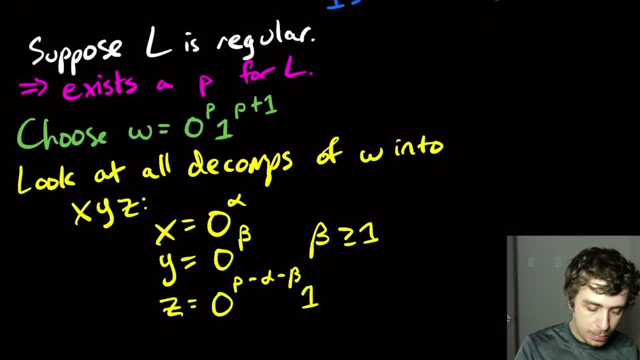 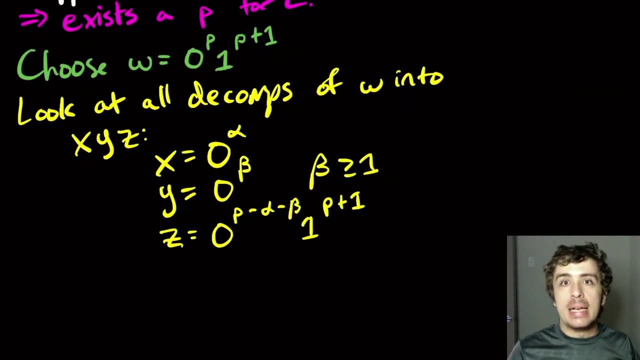 we're going to get something very, very similar. so note that z has all of the ones still, but this is the remaining set of zeros. okay, so now what we need to do is we need to choose an i or find a value of i such that the such that we leave the language. so let's pick a i. so let's look at x, y. 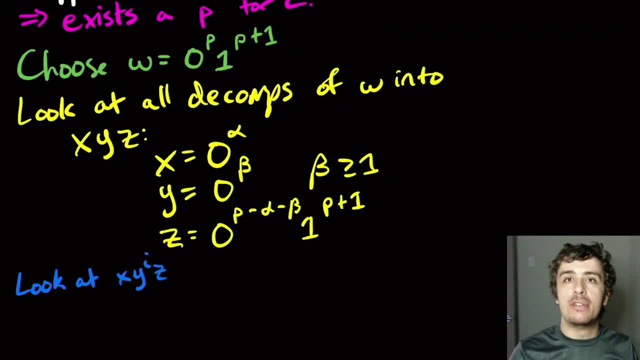 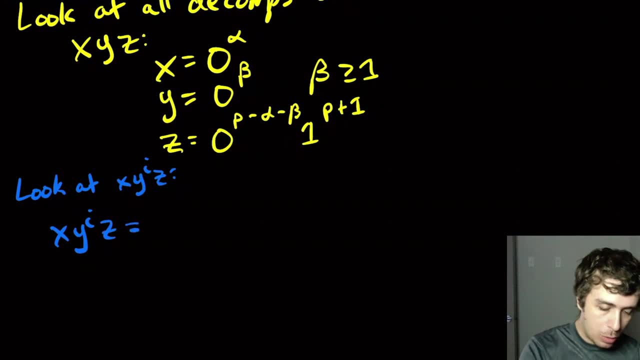 to the i z and see what values of i allow us to leave the language. so what is this thing? so x, y to the i z. well, we're just going to copy and paste the x bit so that zero to the alpha we're going to have i copies. 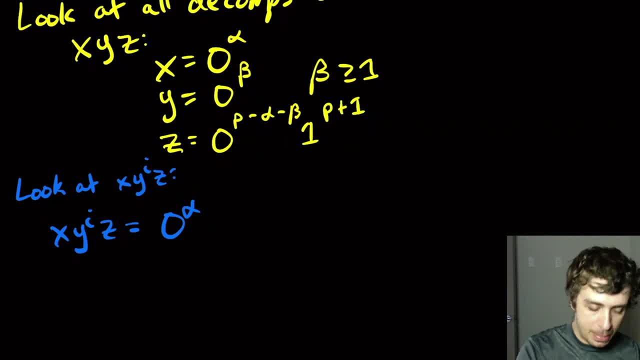 of the y bit. so that's going to be i times beta upstairs, so i beta upstairs and we have one instance of z, so i'm just going to straight copy this down: one to the p plus one, and, like the other proofs, we have a section of zeros that we can just 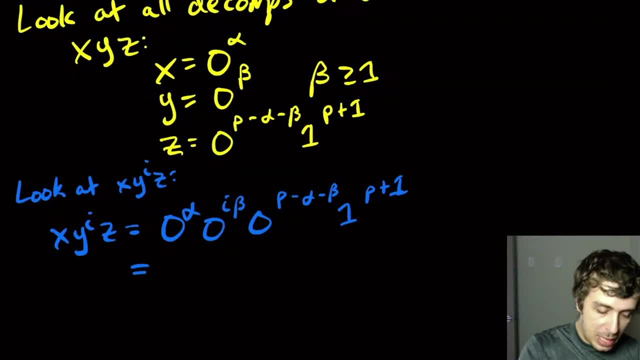 collapse all the exponents in. so the alphas are going to get killed off and, just like any other proof, we're going to have a section of zeros that we can just collapse all the exponents in, and then i'm going to do the same thing. so let's should look then at zx2. do i have a plus or i? 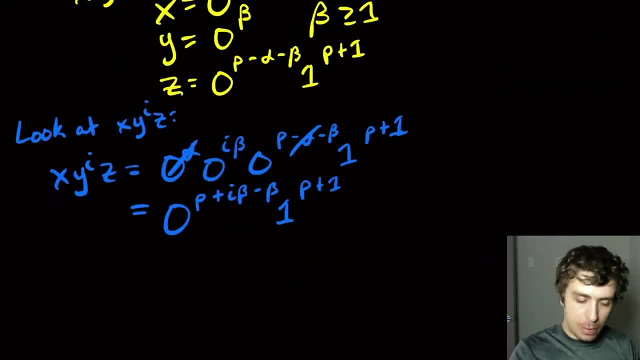 get a k. just do i get k controlled? so i will take an integral of zx2 Cup that i'm going to have p i plus i, beta minus, beta 1 to the p plus 1.. and of course this is only going to be in the language if the number of ones is bigger than the number of zeros. 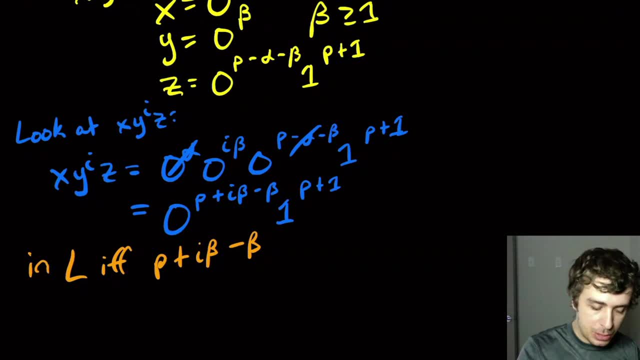 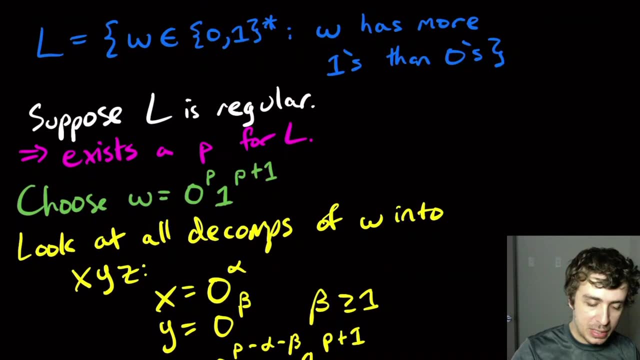 so this is in that language: l if, and only if, p plus i, beta minus beta, which is the number of zeros, is less than z7 times the x is doing the sl accomplishments here strictly less than p plus 1. and let's make sure that it's the ones, not the. 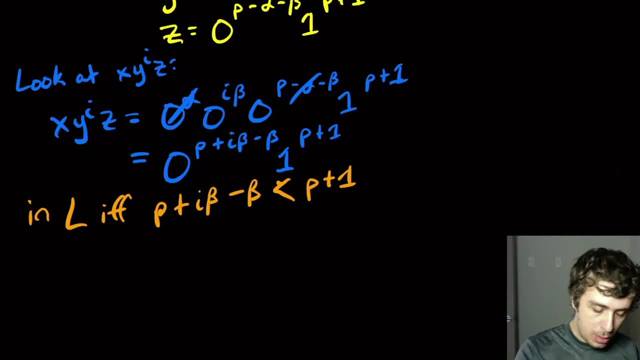 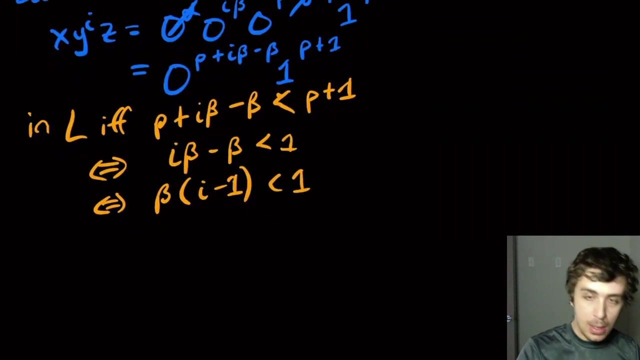 zeros- yep, more ones than zeros. so this is true if, and only if, I beta minus beta is less than 1, so that means, so let's just factor beta out. so that's gonna be beta times. I minus 1 is less than 1, and so what do we know? so we know that beta. 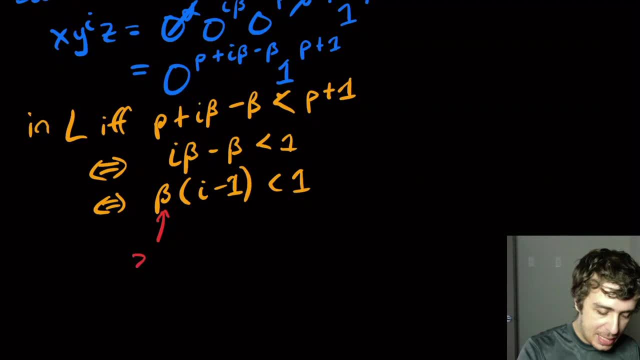 is at least 1, so that guy is at least 1. so the only way that this could be strictly less than one is if we choose I to be 1, because if we pick I to be 1, or, or I guess, if we pick I to be 1, or I guess, if we pick I to be 1, because if we pick I to be 1, because if we pick I to be 1, or I guess, if 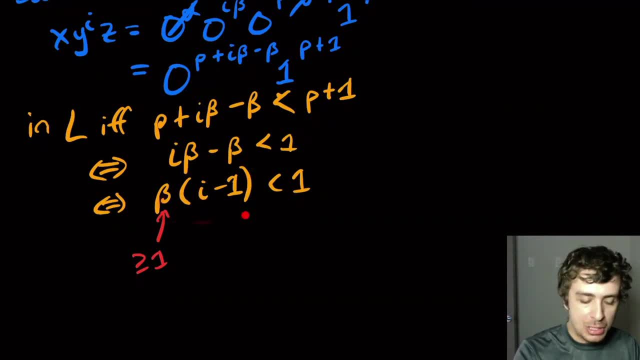 we pick i to be zero, so one or zero allows this inequality to be true, but we want the inequality to be wrong. so because we want to be out of the language, so let's pick i equal two. so but if we pick i equal to two, then let's see, so that's one here times one. so then let's try to investigate. 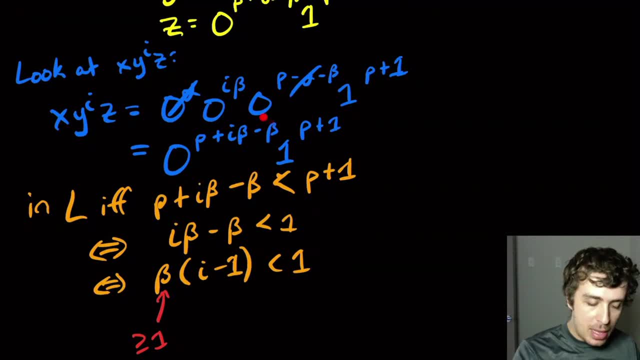 what the string actually is. so if we look at what the string actually is, so the inequality falls and we're done. but let's just actually see why. well, if we pick i equal to two, we have one beta right here, and so we would have p plus beta one. there's one beta here and then p plus one. 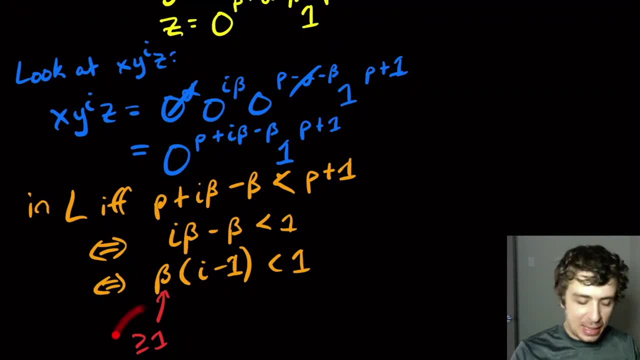 so we don't know what beta actually is, but we know that it's at least one. so that means that the number of zeros is at least as many as the number of ones. it might be more than the number of ones, but it cannot be strictly less so. 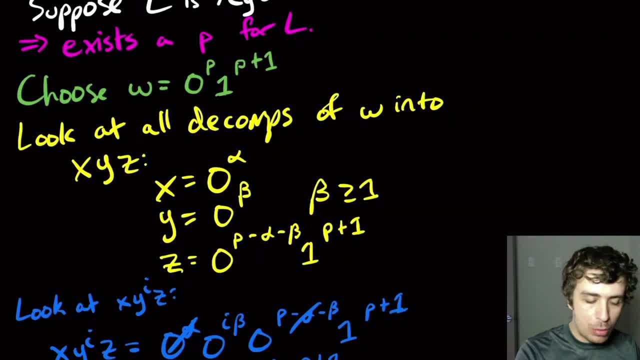 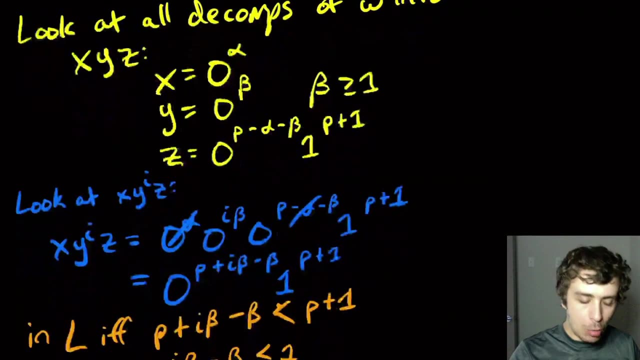 you actually can, for this very similar reason, pick any reasonable number plus whatever, and you will still find eventually an i that works, because if we pick, let's say, a thousand right here, p plus a thousand, well it could be that beta itself is equal to one. but if i pick, 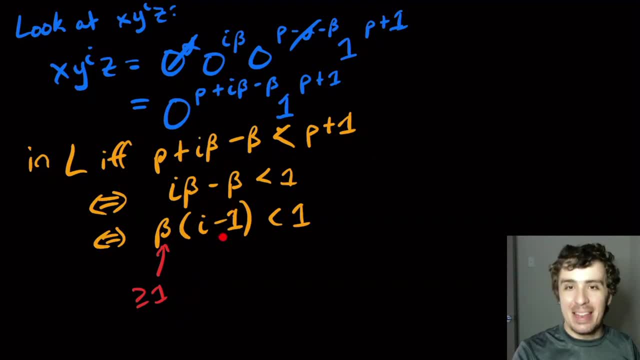 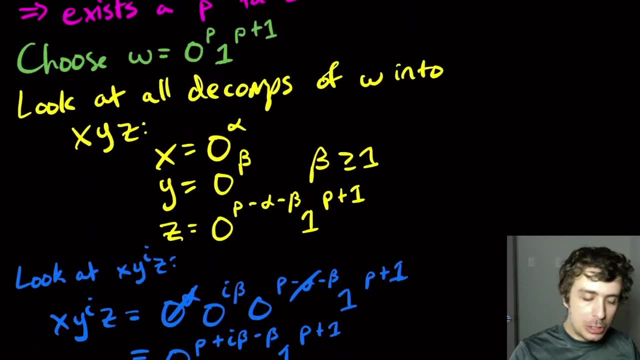 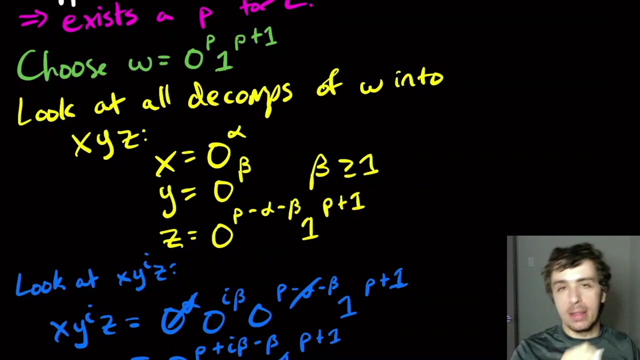 i to be a thousand and one, then that will mean that, uh, this inequality will still be false in that particular scenario, so as, because we're pumping in the zeros, then that allows us to pump out of language, just by putting more zeros in and not changing the number of ones. 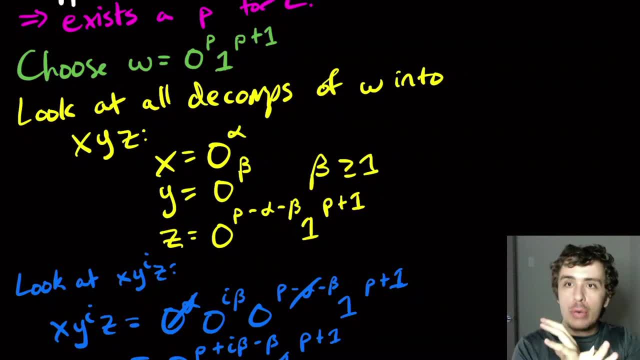 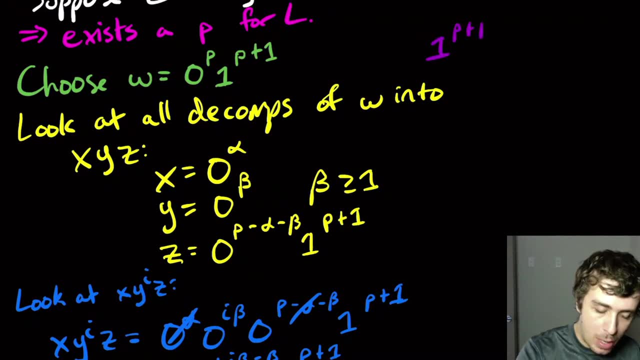 by the way, you can actually um, if you screwed up, you actually in choose this other string. let's say, uh one to the p plus one zero to the p. so now you're pumping in the zeros, uh sorry, in the ones. then if you put more ones in, then the number of ones is still gonna be more than the number of. 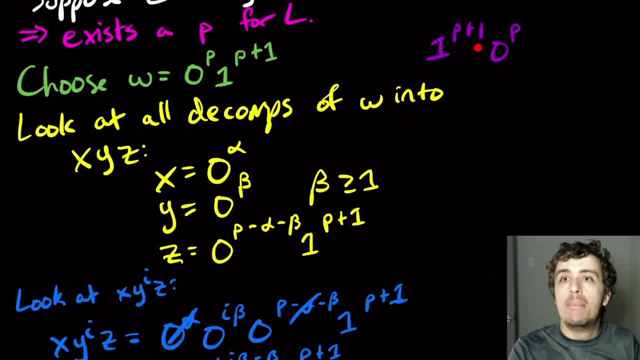 zeros, so you'll never leave the language there. but since we have exactly one more one than zero at the start, if we pump down, then we must take away at least one of the characters over here, and so we won't have strictly more ones than the zeros. this is what i call a straddling the borderline of. 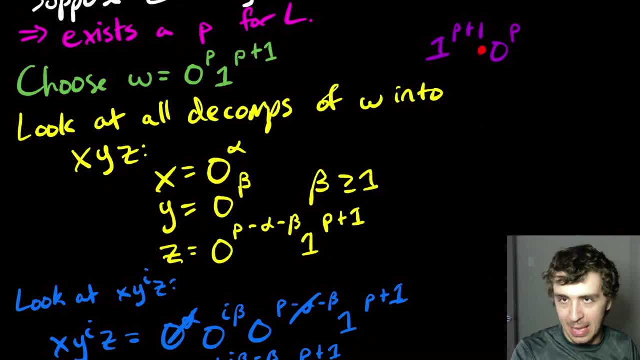 being not in the language. conversation 갈 is barely in the language, one character away from not being in the language. so that's just something that i would recommend doing here. if we have ourselves putting more characters in, we want to put the part that we want to put more of in at the start, because we can only take one away. 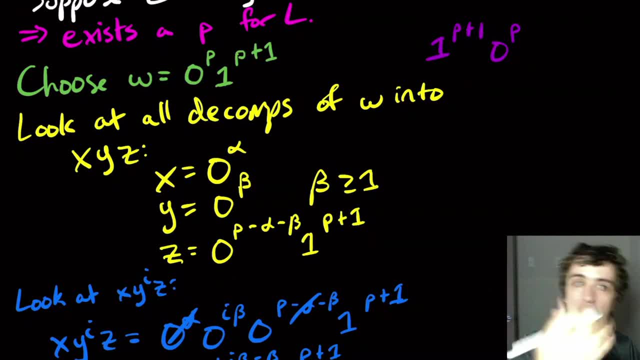 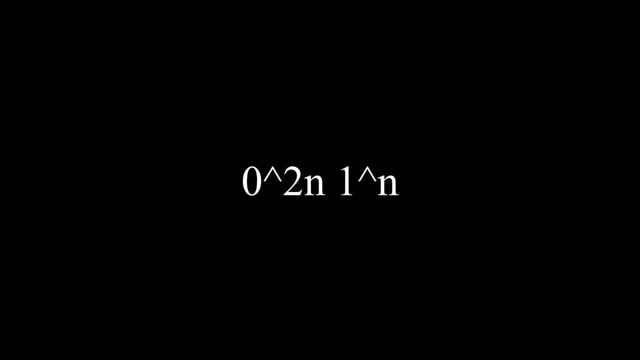 in the worst case scenario, versus adding as many into the string as we wanted to. so this was a lot easier than this one, but we get the same conclusion, just done a different way. cool, okay. so i want to prove that this language, which is the set of all strings, 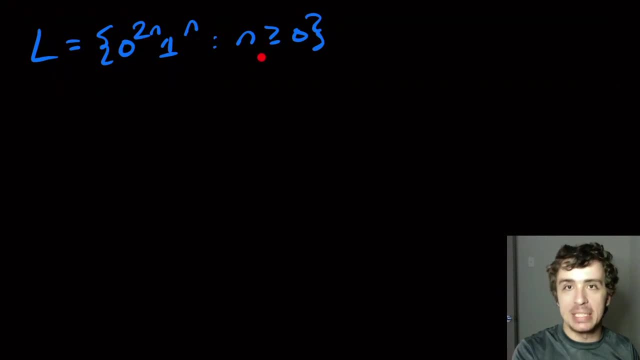 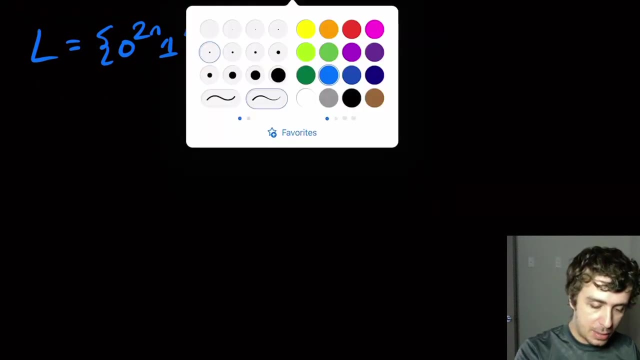 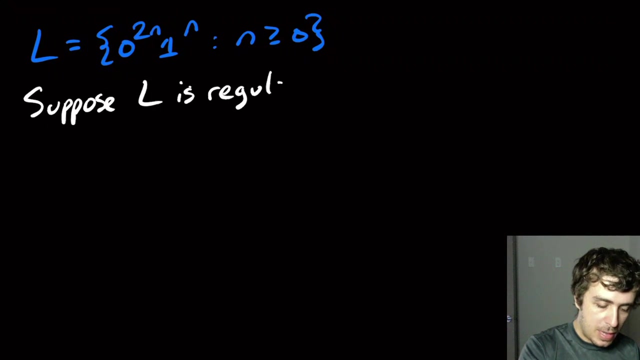 of the form zero to the two n, one to the n, where n is at least zero, is not regular. so here we'll use a standard pumping lemma proof technique. so let's suppose that l is regular. then, as always, we need to pick a pumping constant p. 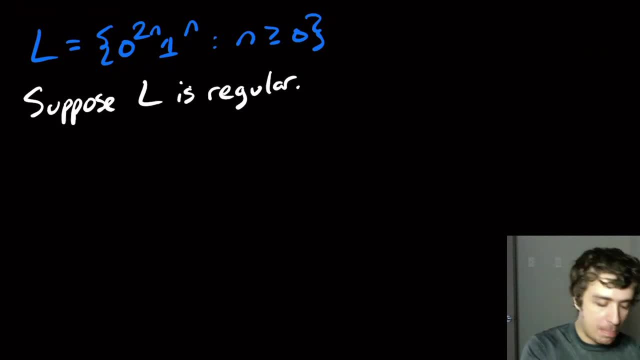 for not pick. we know that there is a pumping constant, p, for this language, so there exists a p for this language. i'm just shorthanding same pumping constant here, okay, well, now we need to pick a string that's in the language and has length at least p. well, the 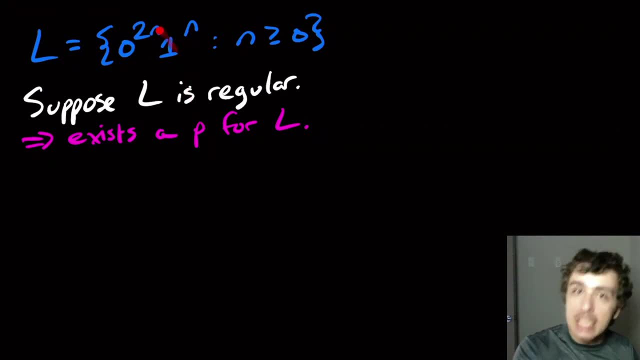 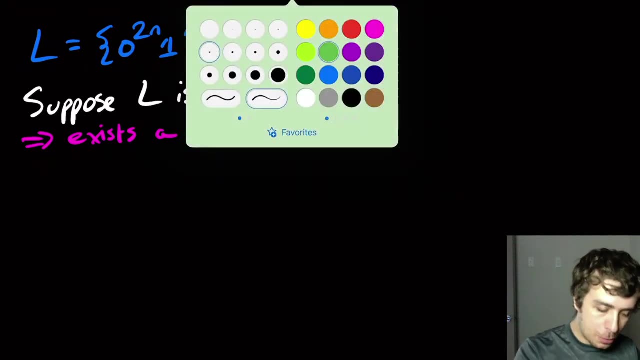 same thing. so if i were to put a string that was a number or for a short length, as long as it was not a number, so it's going to be less than the length of the string. and now we can put a number in this to get the length of the string, which is equal to zero. so now we just need to. 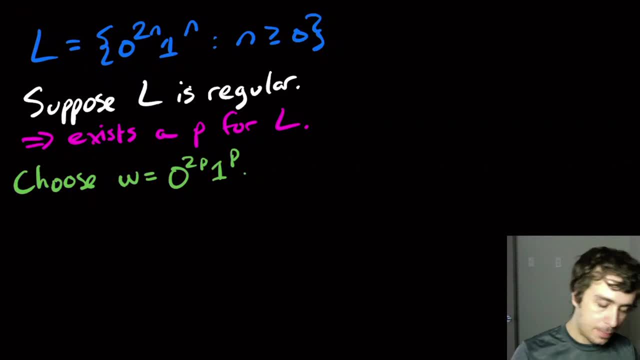 get that into our memory, which is also a common technique. whenever you have n's and exponents and stuff is put the p where the n is. it doesn't always work, but it is a generally a good idea, so fine. So now what we need to do is to look at all decompositions. I'm just going to shorthand the 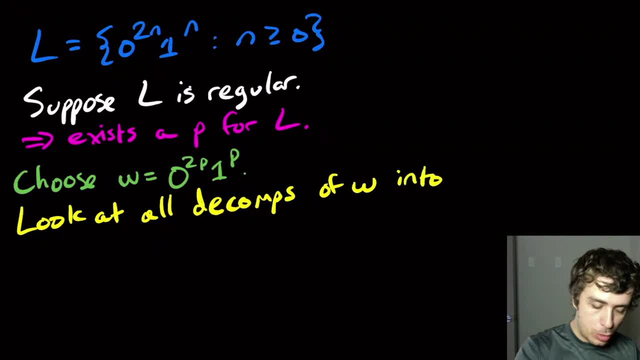 word of w into x, y and z, according to the three, the two rules, which are that x and y together have at most p characters. So the first two bits have at most p characters and the y bit is non-empty, so it has at least one character. Well, if x and y have at most p characters, and they're at the 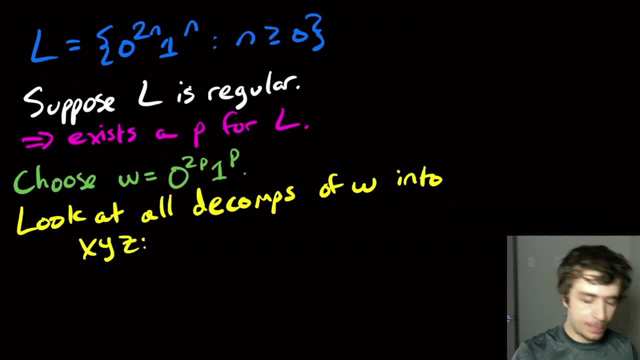 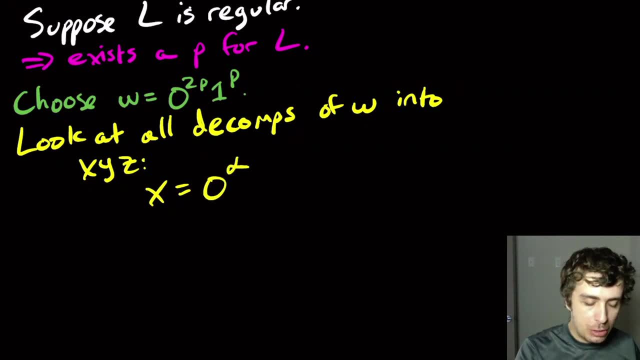 beginning of the string. they must entirely consist of zeros. So- and I don't know how many zeros they have, they have some number though. So let's just say x has alpha zeros in them in it, Y has. it could be a totally different number. let's call it beta, and we know beta is at least one, because we 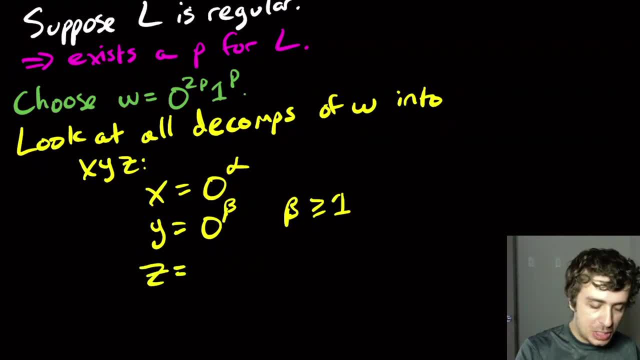 know y is non-empty and z is the rest of the string. So we're going to have zero to the two p, because that's what we started with, minus alpha, because that's what the x part had, minus beta, because that's what the y part had, and we have all of. 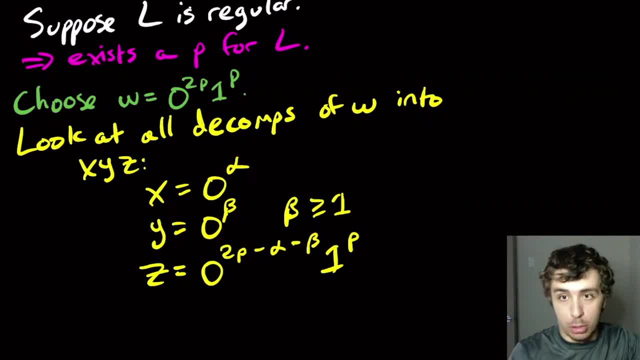 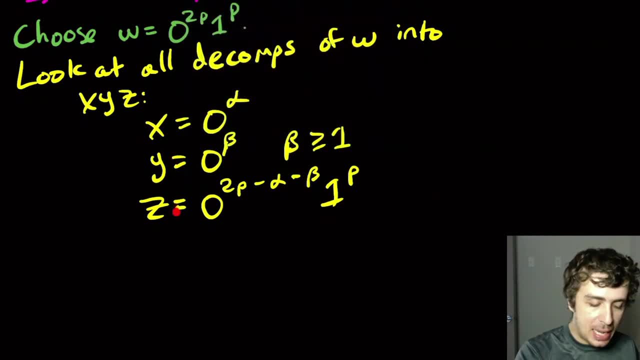 the ones here, because the first two pieces never touched the ones. So we need to now choose a value i such that x, y to the i. z is not in the language, because we want to escape the language, because we want to escape the language. So we're going to have zero to the two p, because that's. 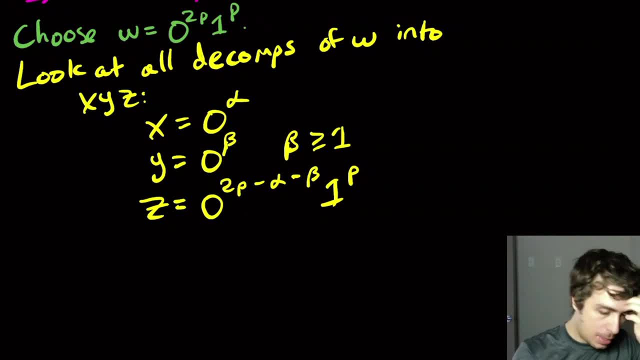 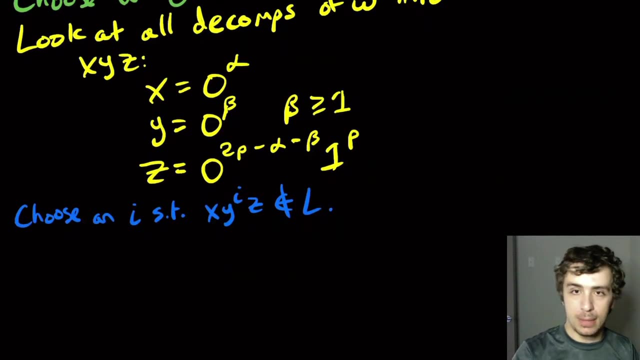 because that would contradict the statement in the pumping lemma that the fact that this was regular. So let's choose an i, such that x, y to the i z is not in the language. Well, what is x, y to the i z? Well, that is well, let's just copy and paste the pieces down, So we're going to have zero to. 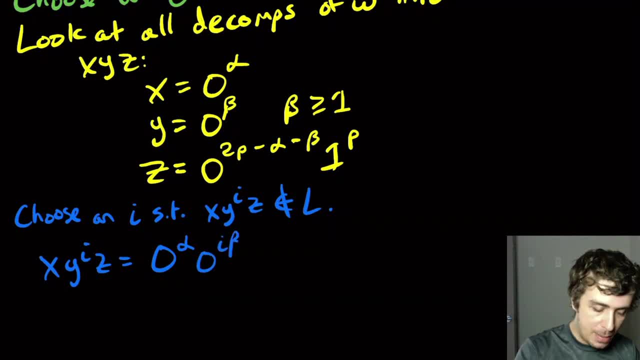 the alpha, zero to the i beta, because we had y is zero to the beta and we have i copies of it and then the z part I'm just going to paste down. So zero to the two p minus alpha, minus beta, one to the p and we have a consecutive run of zeros. 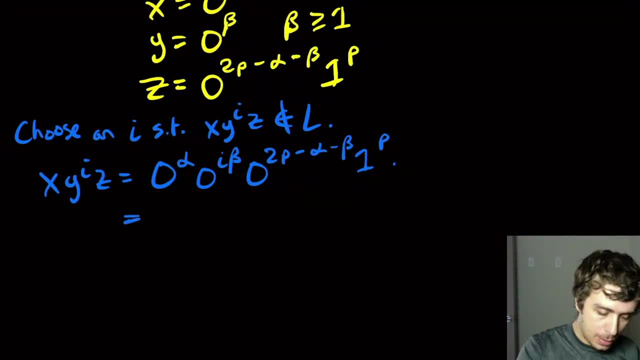 here. So let's just collapse all the exponents together. So that is the same thing as well. the alphas are going to get killed off here because we have a plus alpha, minus alpha. So we're going to have two p- because that was not killed by anyone- plus i beta, because that's from the y bit minus. 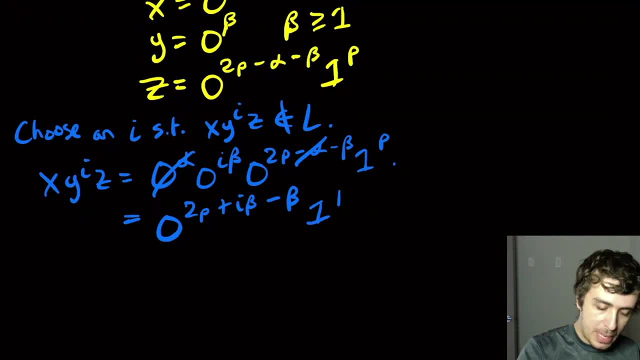 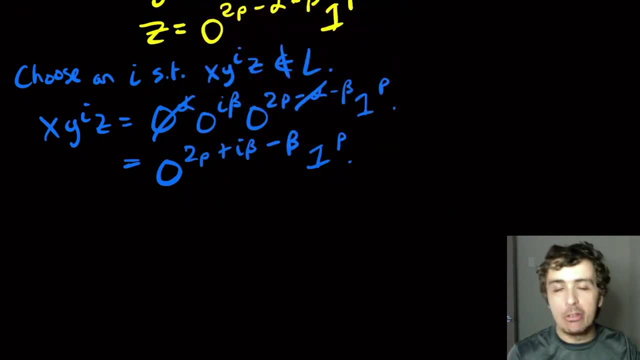 beta, because we have this minus beta here, and then one to the p here, because we never touched that. Okay, so we want to see when this thing is in the language so we can pick an i for which it isn't in the language. So this is in the language if, and only if. 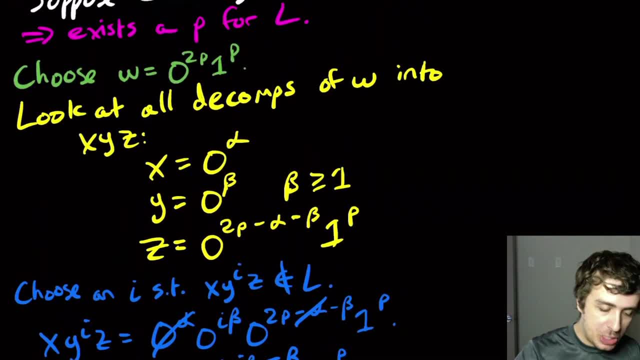 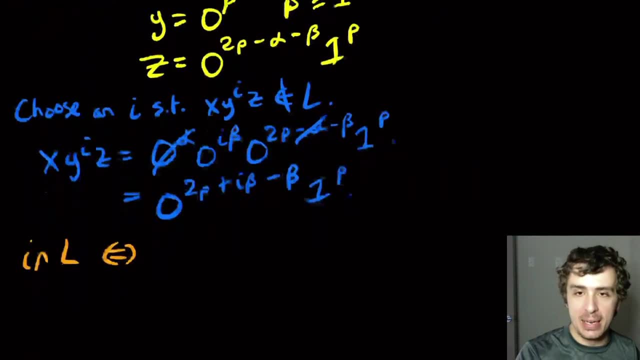 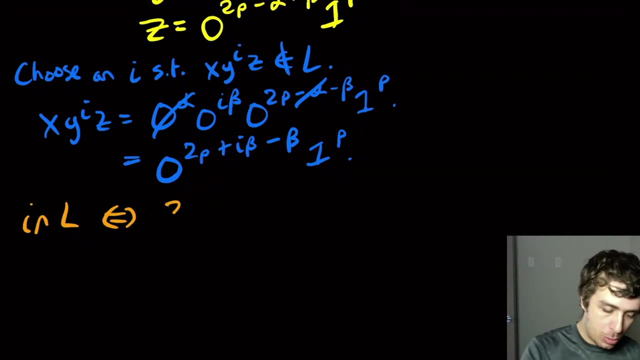 Um, let's see. Well, the language is your vi, which says that the number of zeros at the beginning is twice, exactly twice, the number of ones at the end. so that means that two times this number is equal to this number. so 2p plus i, beta minus beta equals 2p. that's the condition to be in the language. 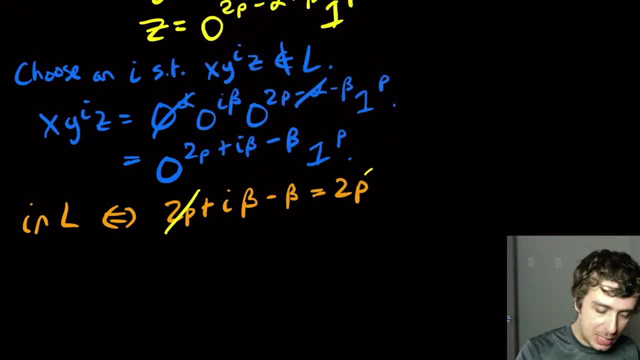 well, here we can just subtract from both sides and this is the same. this is nl, if and only if this is true. so we're going to have: i beta minus beta equals zero. i'm going to add beta on both sides and divide by beta, because i'm allowed to do that, because beta is not zero, it's at least one. 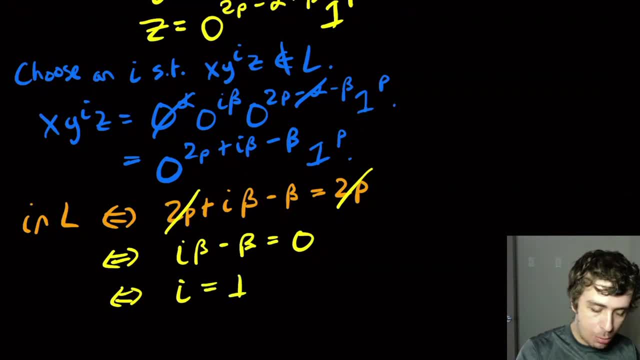 so that's if, and only if, i is equal to one. you can kind of see that here. well, let's just pick an i that's not one. so this is kind of like the zeros at the end, one to the end proof, but the the the condition to be in l is slightly different, so let's choose. 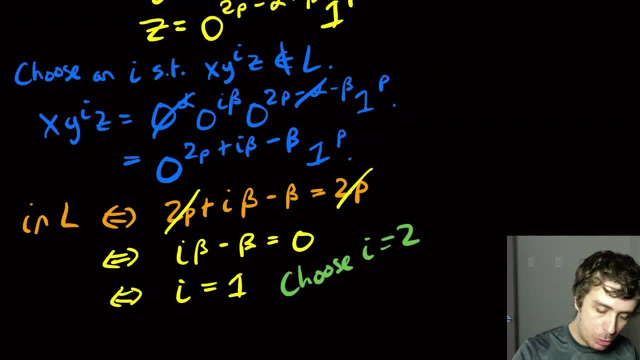 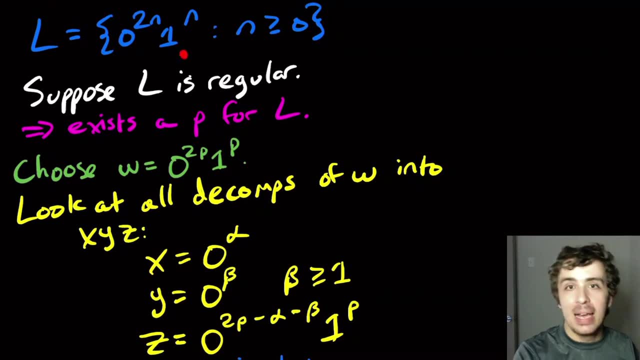 i equal to two, and that will be enough, because we're going to be adding some zeros in the beginning and not changing the number one, so the relationship of it being exactly twice as many is not going to be held anymore. cool. so zero to the two, n. one to the n is not a regular language. 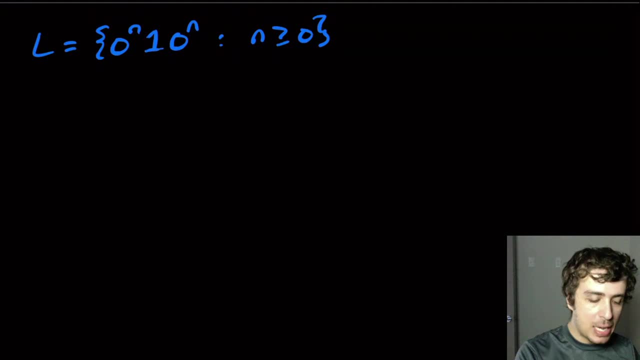 okay, so let's prove that this language, l, which is all the strings of the form zero to the n, one zero to the n, where n is any number, at least zero, is not regular. so here is kind of like the two halves of the string have to be exactly the same, with uh the one separator in between. 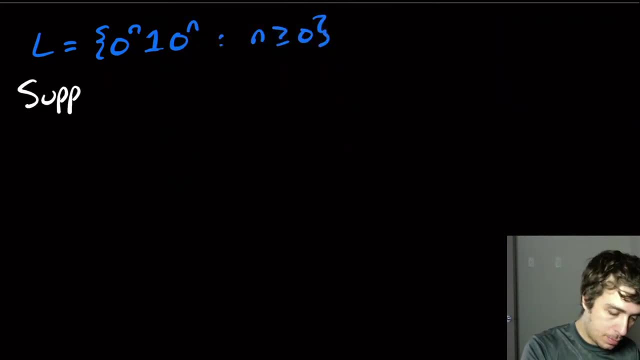 so let's suppose that l is regular. then by the pumping lemma there is a regular string. so there exists a pumping constant, uh p for l- let's use pink for this. so there exists. i'm just going to shorthand it to p for this language, so that now what we need to do is to 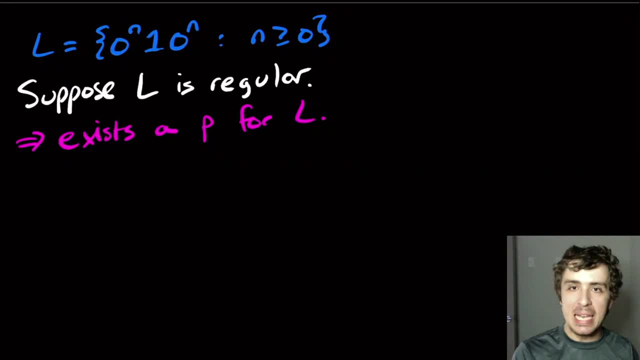 pick a string that is of length at least p, and in the language, and the trick usually is to substitute this p in for the exponent which is, and it's going to work in this case too. so, uh, this is. so let's choose w equal to zero to the p, one zero to the p. note that this is in l. 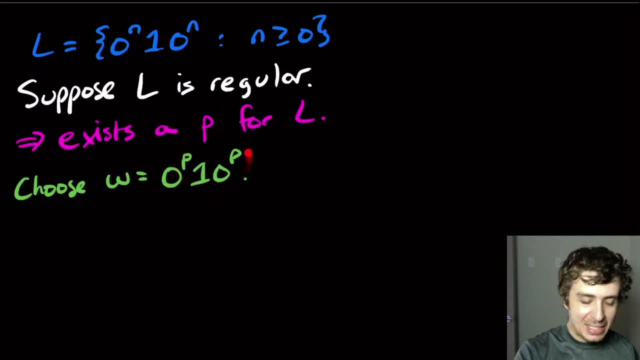 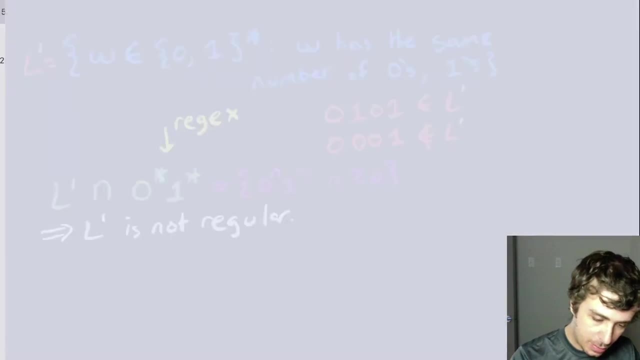 because i just substituted the p in and it's length two p plus one, which is definitely at least p, which is good, okay. so then now we need to look at all the compositions of this string into those three parts. all right, notability crashed, i'll probably have to add: 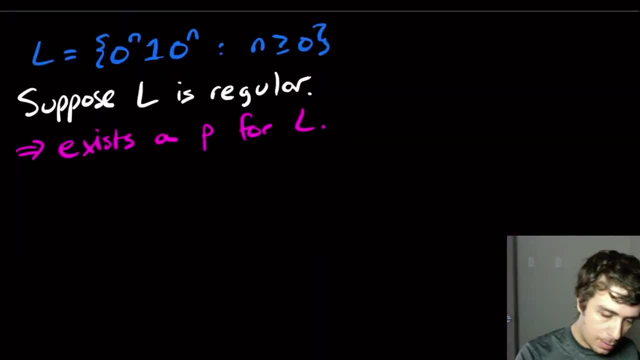 edit this out later. all right, my string went away, so let's. let's choose it again. w equal zero to the p. one zero to the p, let's uh. so now we need to look at all the compositions. i'm just going to shorthand the word of w into x, y, z. 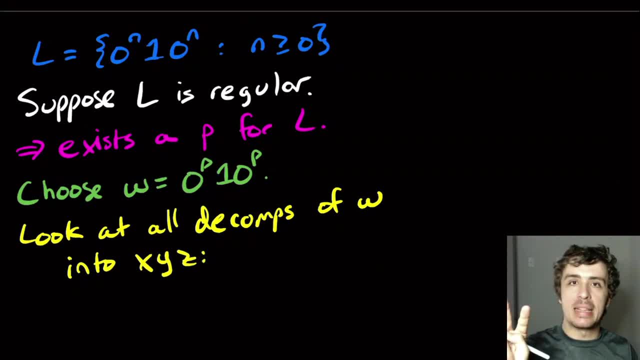 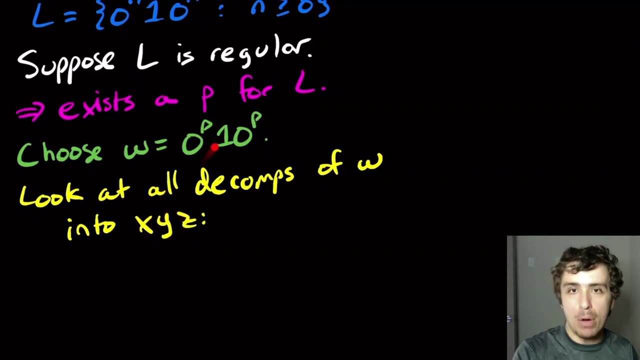 according to the two rules, which are that x, y has length at most p, so the beginning bit has at most p characters and y is non-empty, so it has at least one character. well, here, since the first p characters are zeros and the the first two pieces are of length at most p, so that means that x and y 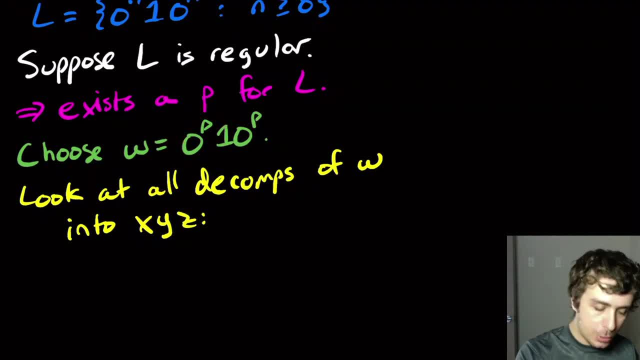 are entirely in this little region here. so we know that x is going to be some number of zeros- i have no idea how many, but it's some number of zeros- and it's going to be some number of zeros, some number. I'm going to call it alpha. whatever it is, Y is going to be some number of zeros. I 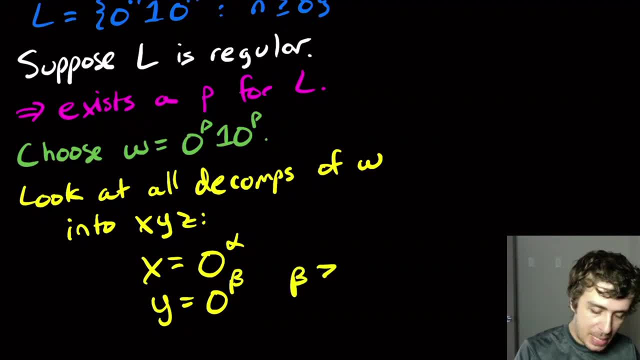 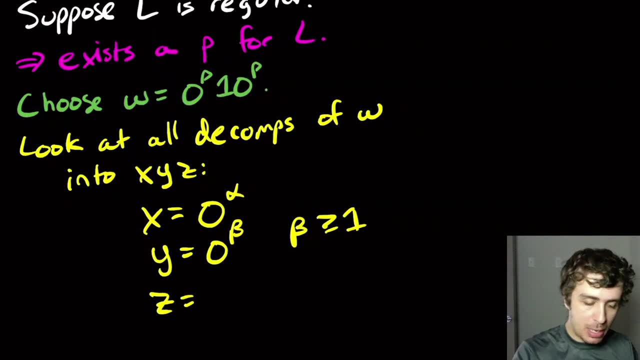 don't know what it is, but I'm just going to call it beta. And we know that beta is at least one, because y is not empty And z is the rest of the string. Well, we have p, because that's what we. 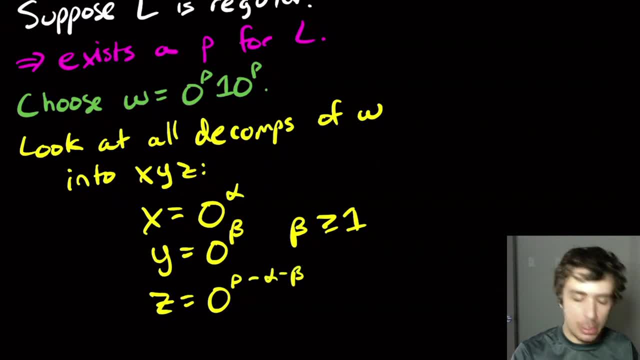 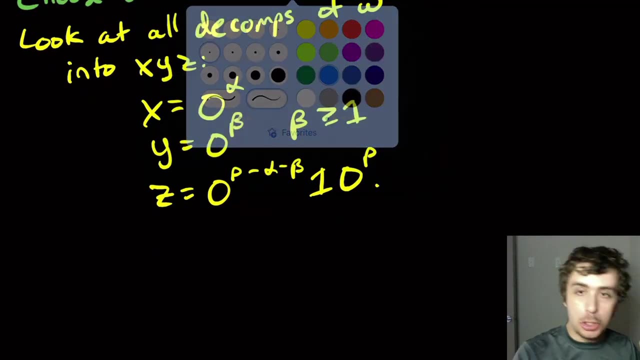 started with minus alpha, minus beta zeros. We started off with p zeros and we took away these, these two, And we have the one separator still there and all of the zeros at the very end still there. So then, now what we need to do is to choose an i such that x, y to the i, z is not in the 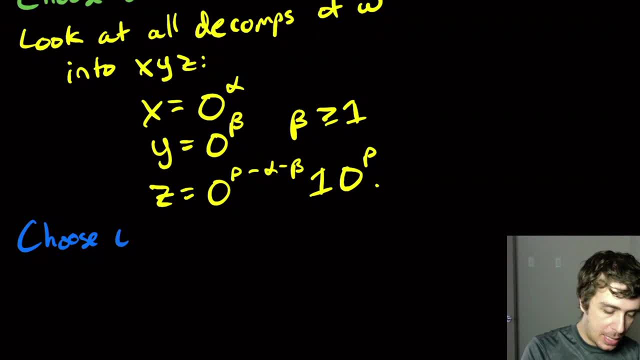 language. So let's choose an i such that x, y to the i, z is not in L, because the pumping lemma says that it's always in L For every i, But if we find one that is not in L, then that contradicts it and contradicts the. 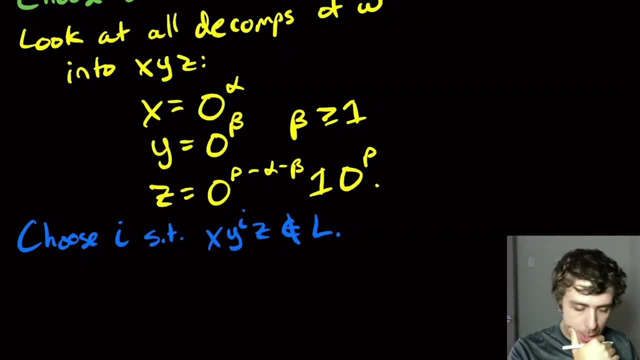 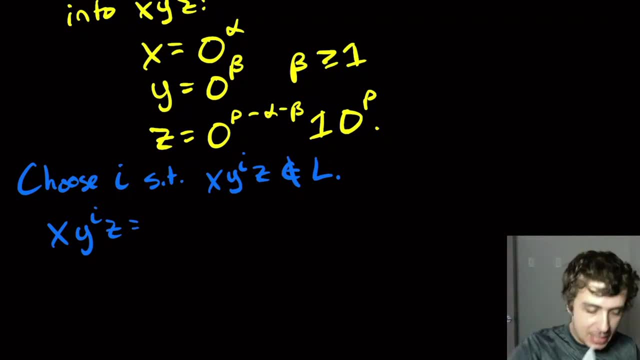 fact that this thing, we suppose that this thing is regular. Okay, so let's investigate what this string is: x, y to the i, z. Let's just copy and down. copy down the pieces. So we have zero, z alpha, That's the x bit. We have zero to the i, beta, That's the y bit, i times And then the z bit. 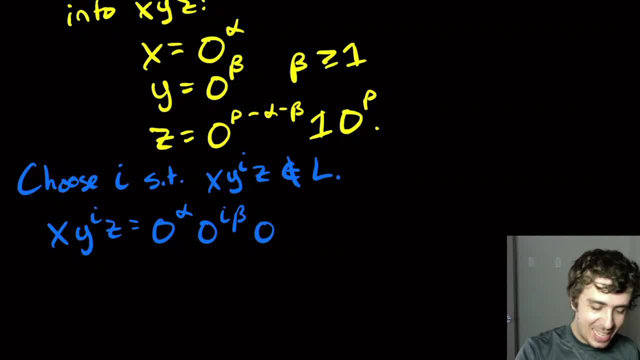 one time, Oops, not z- Zero to the p, minus alpha, minus beta, one zero to the p. So here I have a consecutive run of zeros. This one doesn't count because there's a one separator, but I can combine these ones because 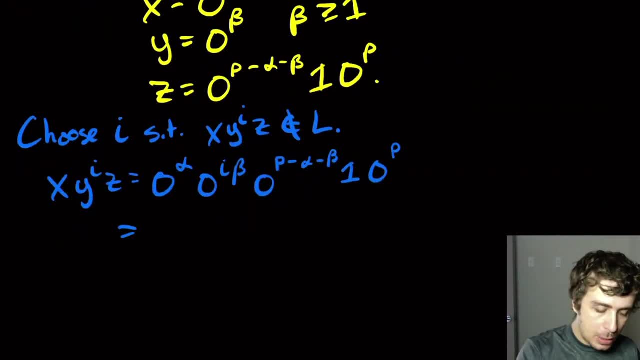 they're all zeros. I'll just put the exponents together. So the alphas are going to get killed off. So I'm going to have zero to the p, plus i beta, minus beta one, the separator, and then zero to the p. Well, the only way that this thing could be in the language at all is if the two exponents 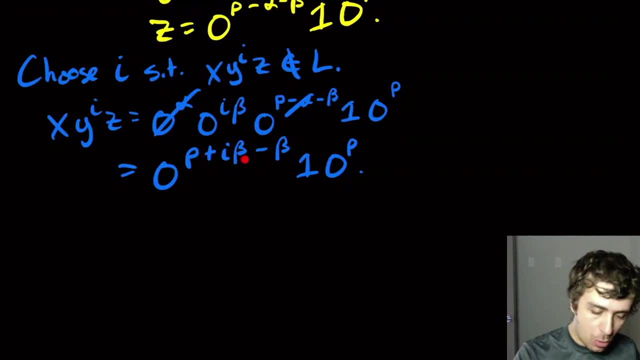 are identical. So this is in L if, and only if, these two numbers are the same. So let's write that down. So this is in L, if, and only if, p plus i, beta minus beta equals p, because those are the two exponents. 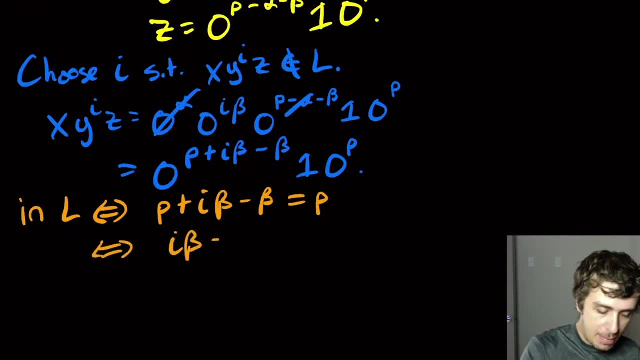 So this is if, and only if, i. beta minus beta equals zero, And this is if, and only if, i is equal to one. So if I choose any value other than one, then we can find that this thing is not in the language And I will just pick i. 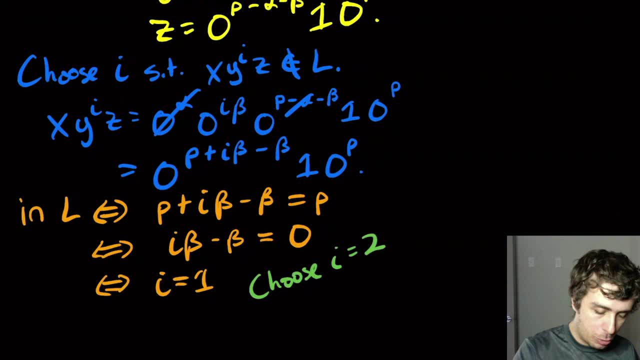 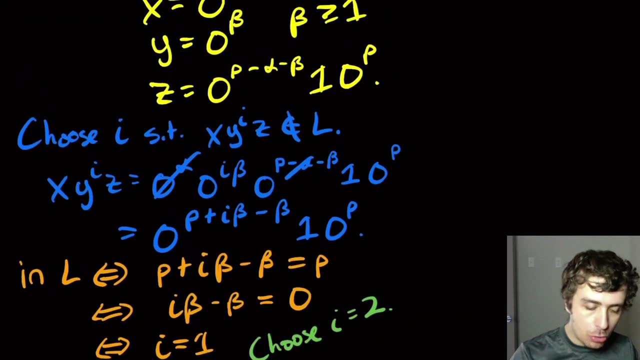 equal to two. So choose, i equal to two. And this is kind of like the zero to the n, one to the n- proof. It's structurally a little bit different because we've got the zero to the n, one to the n. 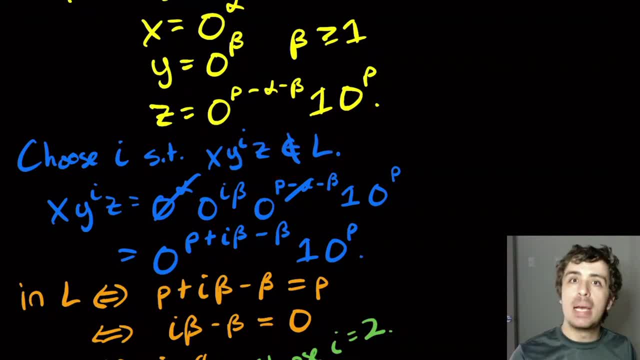 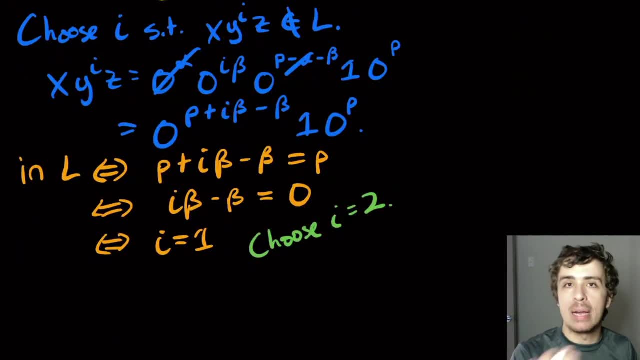 proof. It's structurally a little bit different because we've got the separator and that's the same set of characters, but it's identical in the conclusion and how essentially the same and how we were able to show that this thing is not regular by finding a string that is not in the 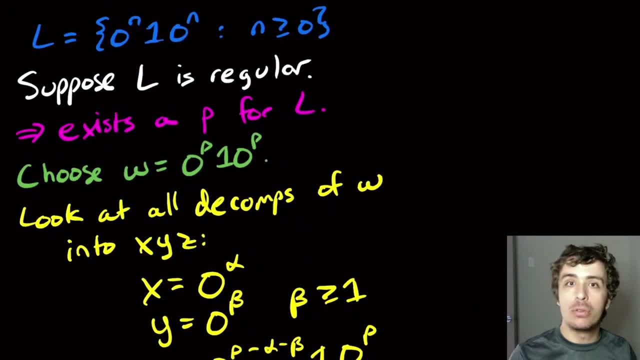 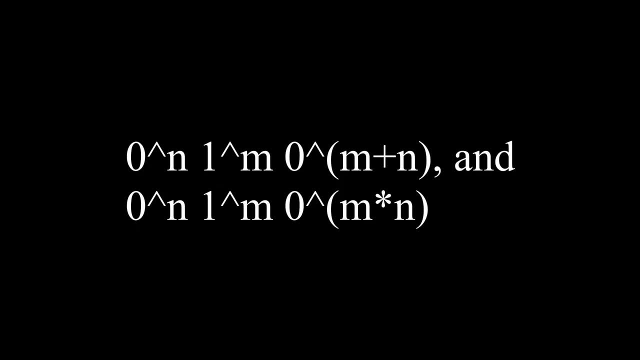 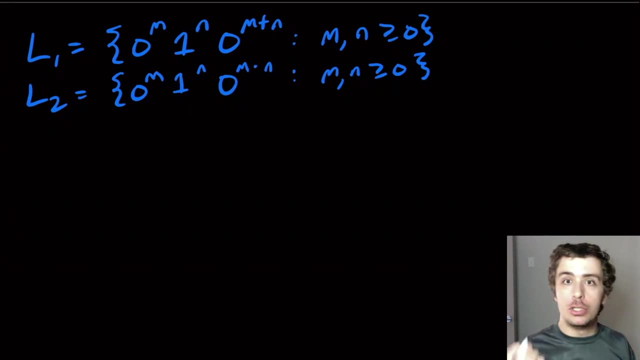 in the language. Cool, So we have shown that zero to the n, one zero to the n is not in. it's not a regular language. Okay, so the next two proofs I want to do all in one fell swoop And because they're very, very similar to each other. 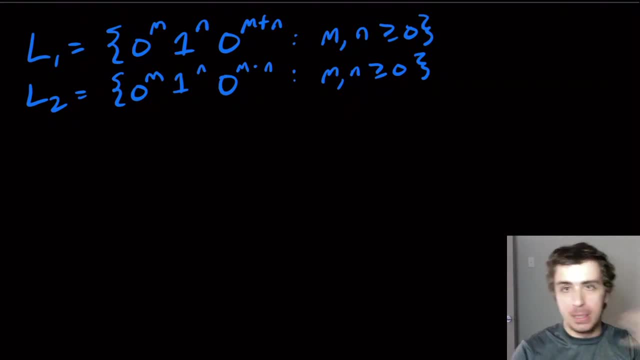 so that we can kind of do both of them in the same proof but just slightly change it at the very end. So we have two languages here which are zeros ones, then zeros of the form, some number of zeros, some number of ones, And in the first case the number of zeros at the end has to be: 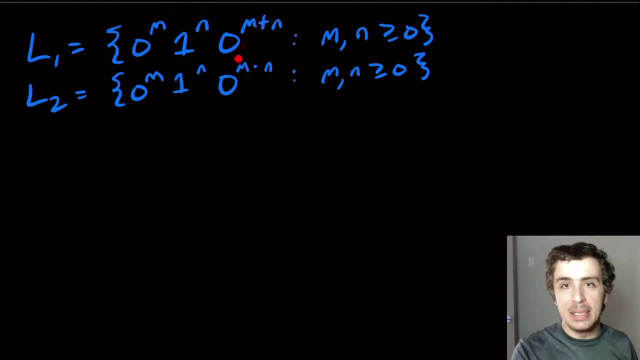 the number of zeros in the beginning plus the number of ones at the end, And the second one is the product of the number of zeros and ones in the beginning. Okay, and I want to show that both of these are not regular. So what I'm going to do is I'm going to have a language, L prime, or actually. 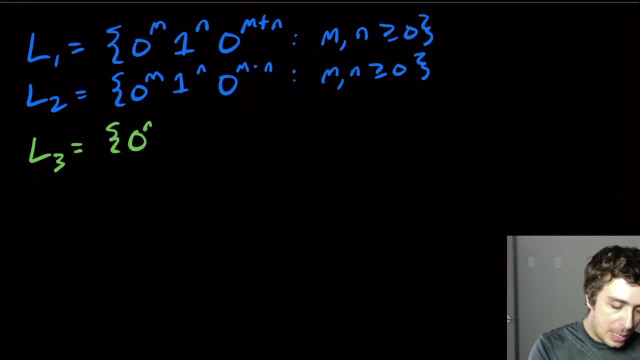 I'm going to change it to three, which is going to be generalizing both of these, and then we'll hoist it back to the original two and we'll see how. So I'm going to have zero to the n, one to the n. 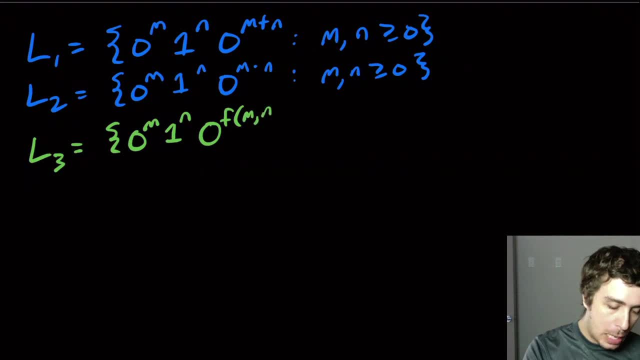 and then zero to the f, some function of m and n, And then the first example is: the function is just adding the two, and the second language is just multiplying the two, And then we'll see if- and only if- it's in L3, and then we'll see what the 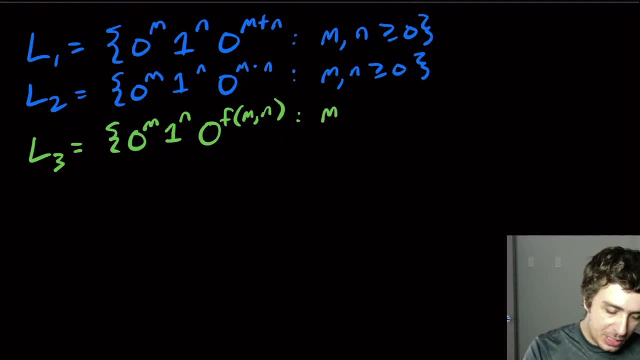 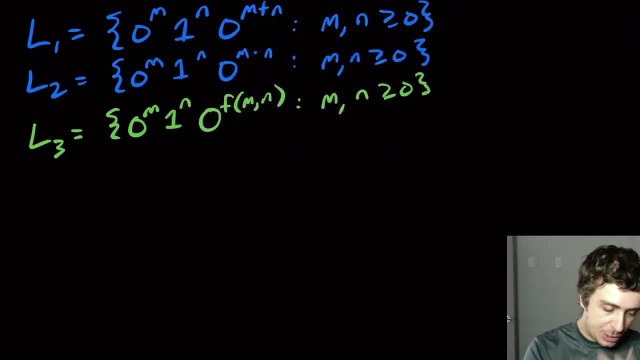 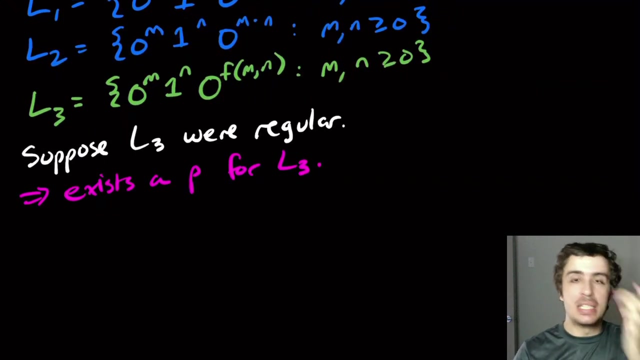 function is at the end. Okay, so this is m and n, at least zero. Okay, so then let's suppose L3 were regular. Then that means there exists a pumping constant p- I'm just going to shorthand it- for there's a pumping constant p for L3.. So now we've got to pick a string that is of length at. 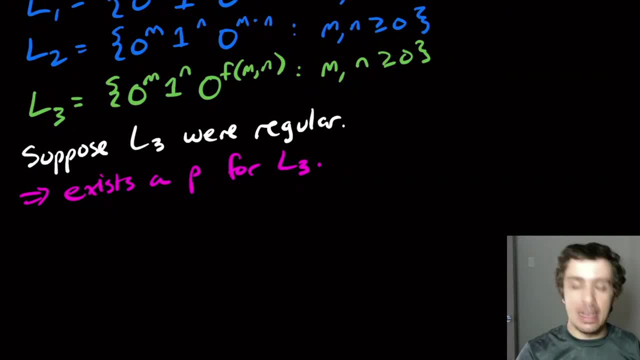 least p and is in that language. So what I'm going to do is I'm going to just borrow this by substituting p in for the exponents, And it turns out that there are other parameters that will work for the first two languages, but it turns out that if you just substitute p, it's really easy. 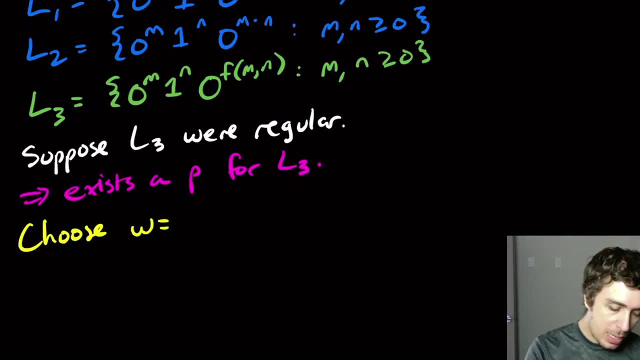 So let's choose w equal to zero to the p, one to the p and then zero to the f. some function, the function f on p and p, just substituting m and n for p or p for those two. So this is definitely of length, at least p. Well, this function can't be worse than zero. 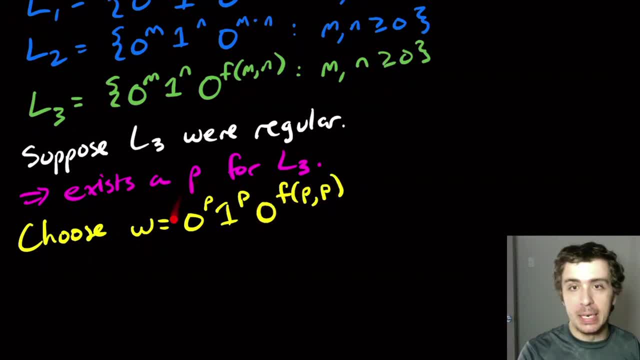 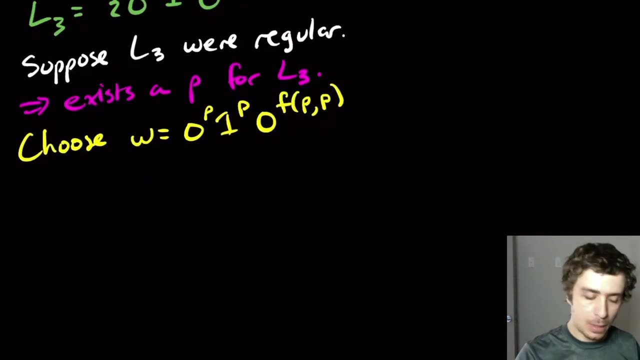 so even if there were no zeros over here, I'll still have more than p characters to start with, which is great. This is in L3 also, because I'm just substituting in the number p for m and n, and that's all we needed. Okay, so then now we need to look at all decompositions. 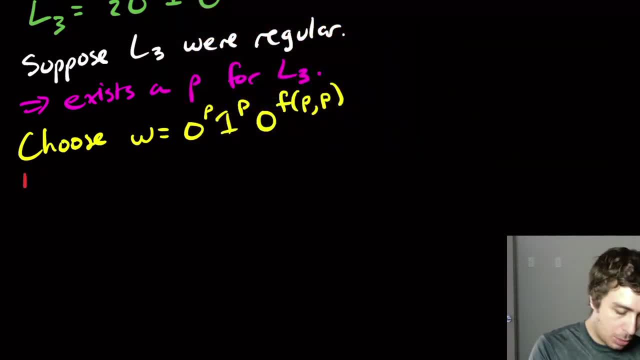 of this string w into those three pieces. So look at all decompositions of w into x, y and z. according to the two rules that x and y are of length at most p and y is non-empty, meaning it has at least one character. 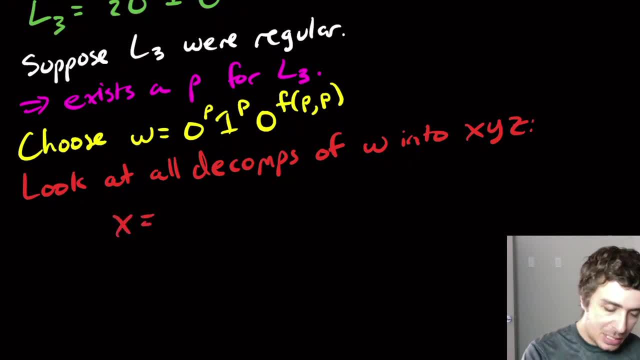 So we have the x, because this string starts off with p zeros. that means an x and y are both only zeros, but I don't know how many of them. So let's say x has alpha zeros, y has some zeros and y has some zeros and y has some zeros. So I can start with the number beta of zeros. 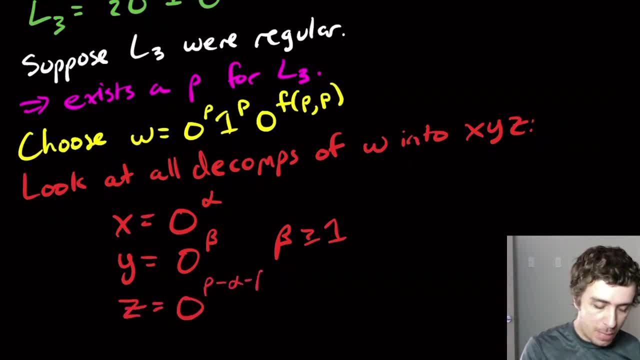 I have no idea what the number is, other than it's at least one, And z is the whole rest of the string. Well, I'm going to have p minus alpha minus beta, 1 to the p, and then all of the zeros at the end. 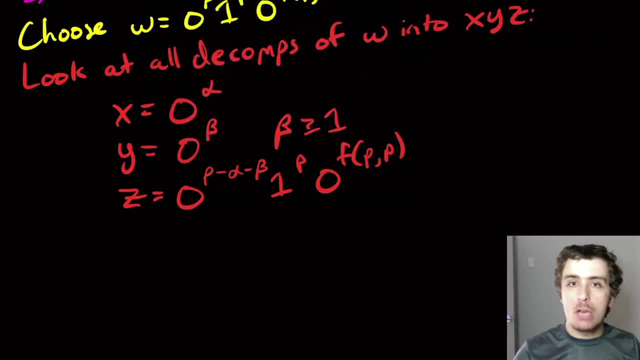 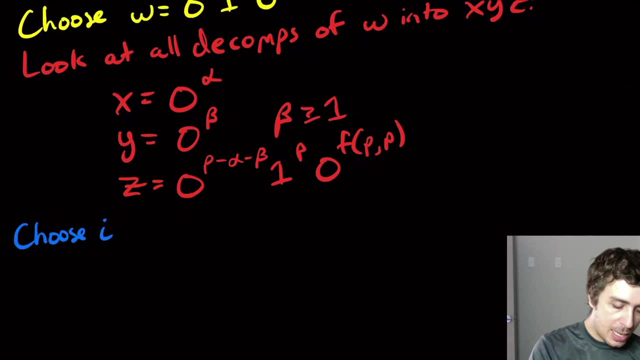 which is that f function p of p. Okay, so then now what we need to do is to choose a value. i such that this is not in the language anymore, And i such that, technically, we need to choose functions f1 and f2, also, such that 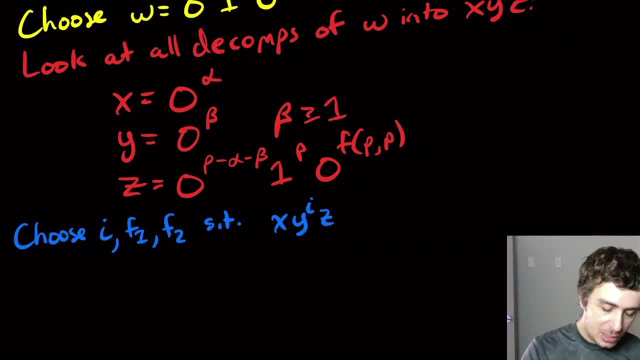 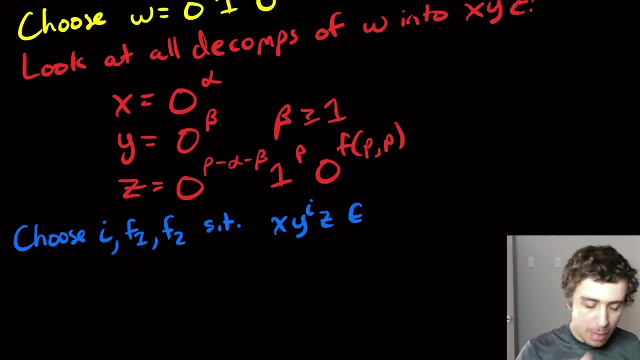 let's see. so it's a, x, y, i. z is not in, okay, so I'm abusing notation a little bit. So it's not in l1 or l2.. So the functions are going to be different. Note that f1 corresponds to checking whether or not it's in. 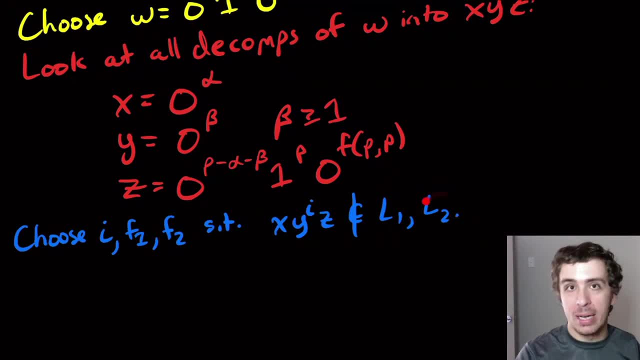 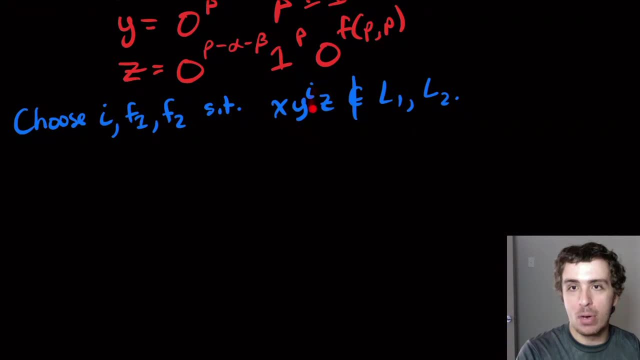 l1 or not and f2 is whether or not it's in l2.. Okay, I'm abusing notation a bit because there's no f1 and f2 written here, but note that the f1 and f2 are corresponding to the function. 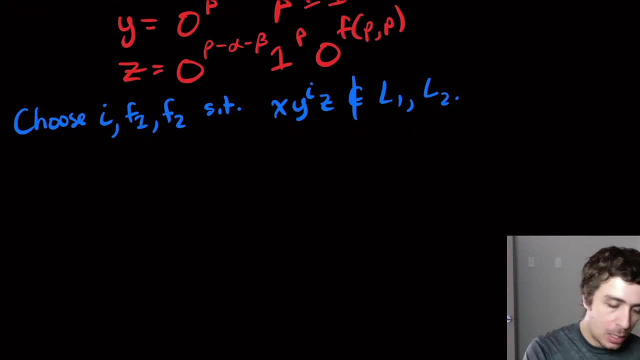 f, that's written for what z actually is. So let's actually compute what x, y to the i, z is. Well, that's going to be zero to the alpha, because that's what the x thing is, then zero to the i, beta. 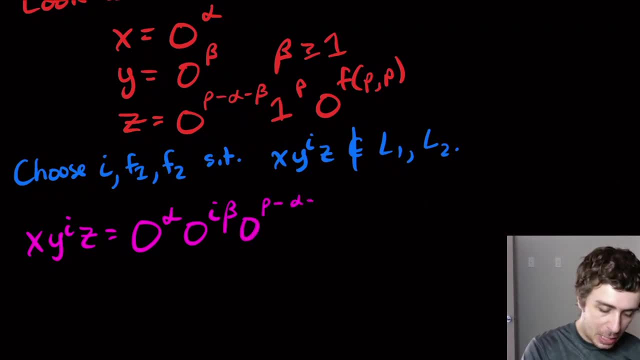 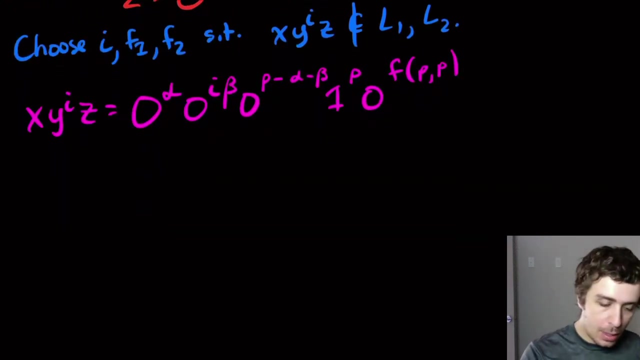 and then just the z bit, So zero to the p, minus alpha, minus beta, one to the p. and then I'm just gonna write f here for now, because this is just a general case. Now let's check whether or not it's in l1 by substituting f1 in. So the f1 thing, well, f1 is just adding the two. 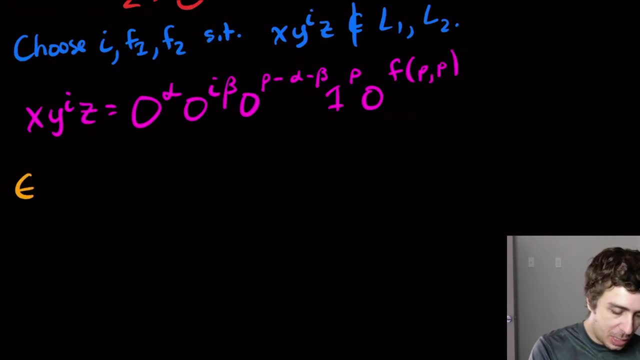 values. So here this is going to be in l1, if and only if, let's see. so here what we have is that the number of zeros at the beginning plus the number of ones here equals in this case 2p. So what is the number of zeros here? Well, the alphas are going. 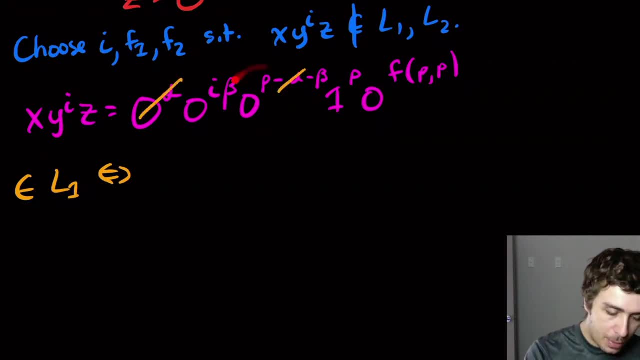 to get killed off. so we're going to have the number of zeros over here is going to be p plus i beta minus beta. so p plus i beta minus beta plus the number of ones here, which is just p, is equal to f1.. Well, f1, remember, it's just adding the two. 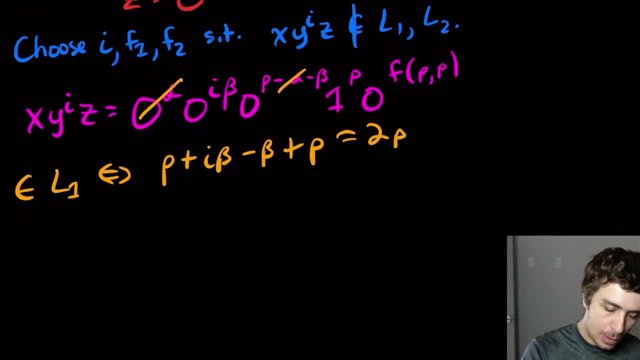 parameters. so that's going to be equal to 2p. So here, well, notice that we got 2p over here. so this is oops. so this is if, and only if, i, beta minus beta equals zero. and then you can check for yourself that this is if and only if i equal to one and like other. 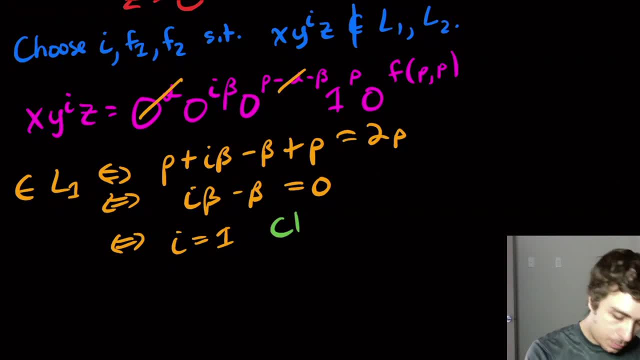 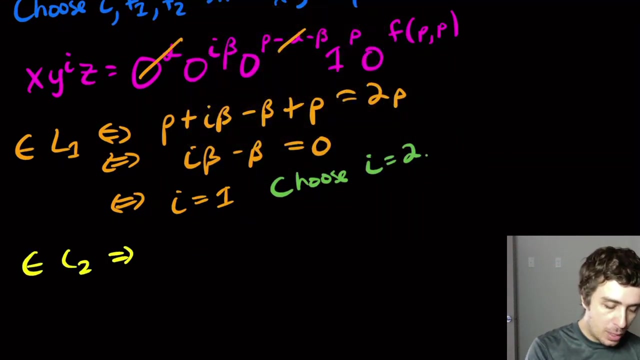 proofs we've done before on this channel. we can, we can choose a different value of: i, let's choose it, uh, two, we can pick zero or three or whatever. all those will work. so then now let's do the, the other one that this thing is in l2, if and only if, multiplying the number of zeros times. 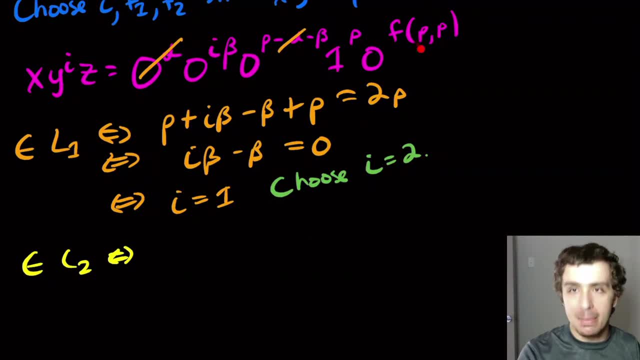 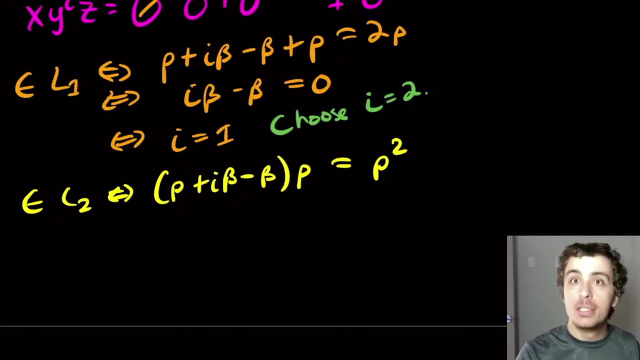 the number of ones equals p times p, because remember, the second language had the two parameters multiply each other. so here let's do uh, so we have p plus i beta minus beta times p is equal to p squared. so note that p is at least one, so we can divide by p on both sides. 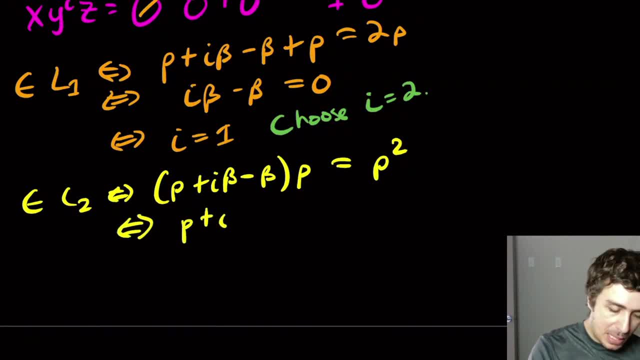 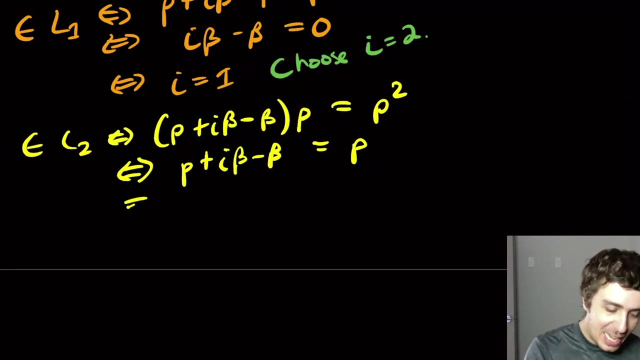 so we're going to get p plus i beta minus beta times. p is equal to p squared plus i beta minus beta, no p there at the end, and we divide it by one p on the right side, which we were allowed to do, and this is very, very similar to this. so this again is: 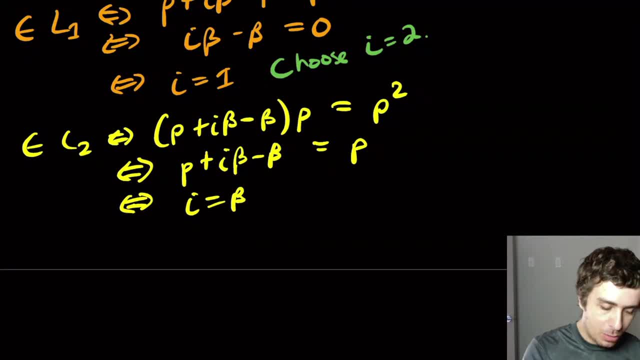 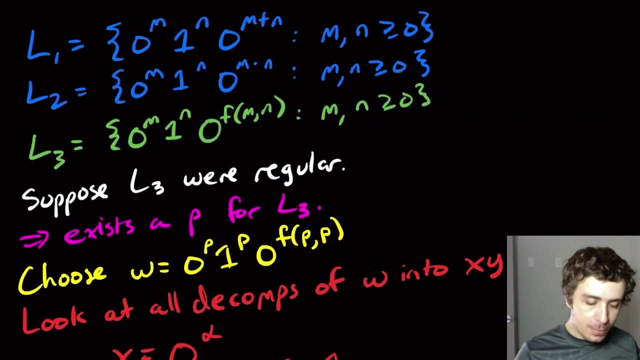 true if, and only if, i is equal to, oops is equal to one, and we can again choose the i parameter to be two, also cool. so what you should see from this is that you can actually show that, um, multiple languages that are very similar are all non-regular. 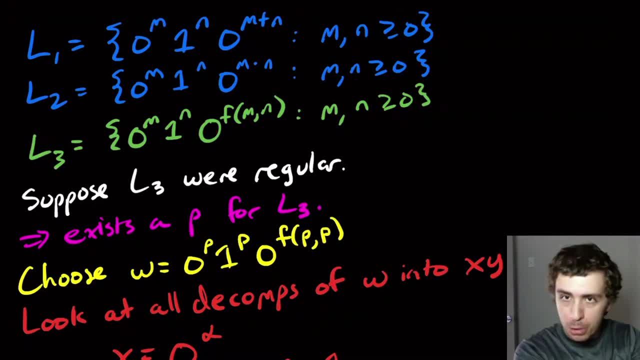 just by generalizing them. do the proof in the generalized case and then specialize it based on the languages at the very end, instead of having to do all the work over and over and over. so here, l1 and l2 are not regular. i'm not going to claim that l3 is not regular, because it very. 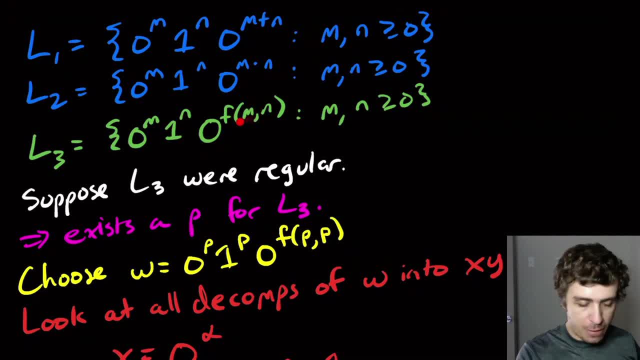 much depends on the general y i, for example. but if we do the check between the finalول, woah, that'll make that change either to 200 or it'll do anything at all. i'm not going to be letting you just say that she just started planning. hello, sorry, as simple as that. so 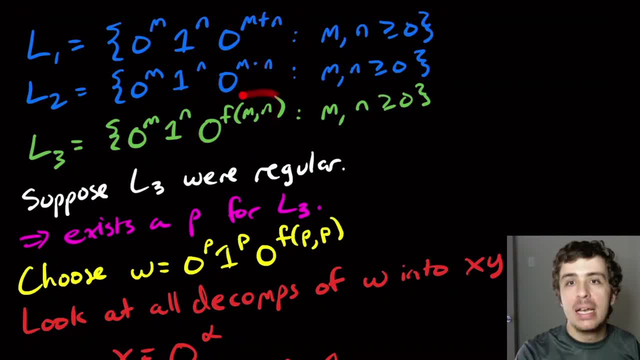 if you find some error in here. so, since every udah one gets one, well dan, and it'll do that same thing. but anyway, if you find server that only has executable quê leff o, China o l a 爱 just M, you can actually show that this is. I'd have to think about it, but you can't claim. 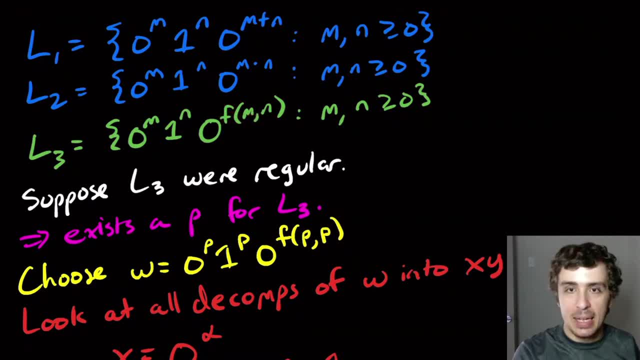 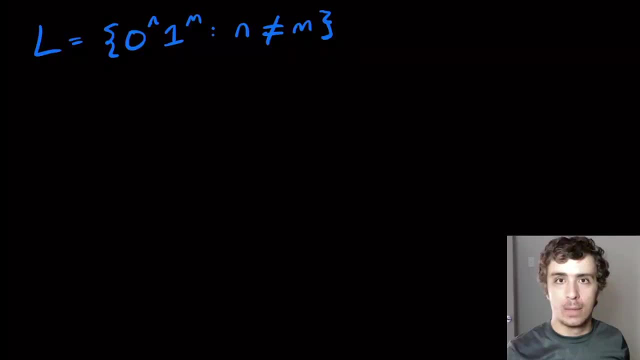 anything based off of this F could be technically anything here. So L3 we can't claim is regular or not regular, it depends on F. but L1 and L2 are definitely not regular. Okay, so let's prove that this language is not regular. So here it's all strings of the form. 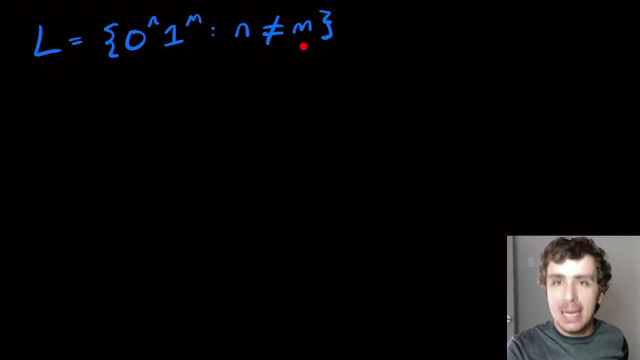 zero to the N, one to the M, where N is not equal to M. So this is a very challenging language, but I'm going to show you a really nice trick that I've done on the channel already, but I'm going to do it again here. So let's again suppose that this thing is, let's say that this is a 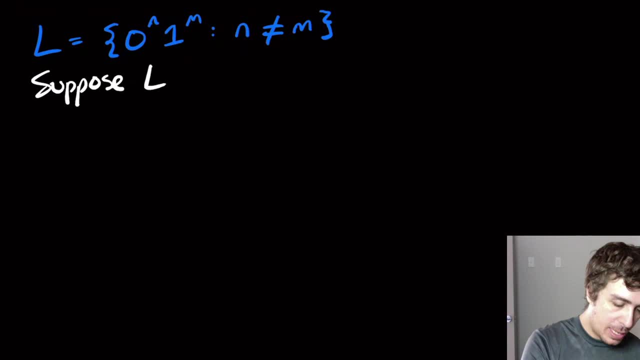 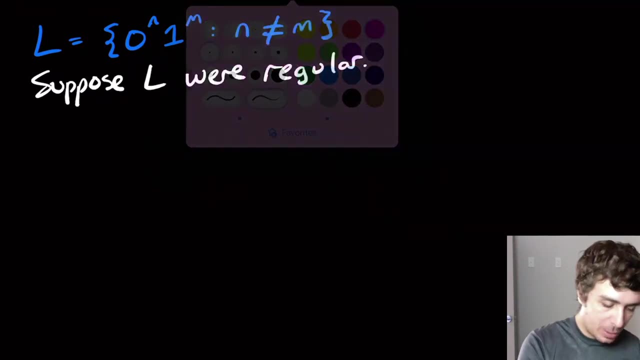 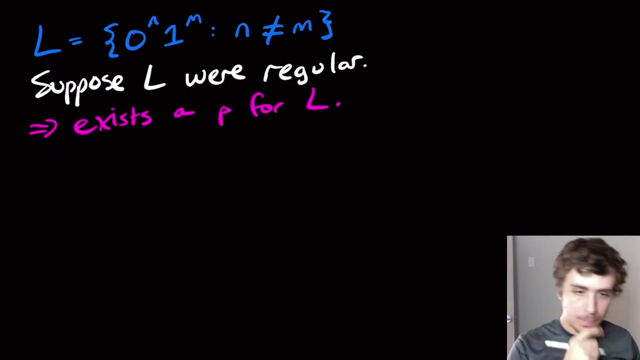 regular. So suppose L were regular, then what we know is that there exists a pumping constant, P, exists a P for L. Okay, so then now what we need to do is we need to pick a string that is in the language and length, at least P, So you may pick. okay, choose W equal to zero to the 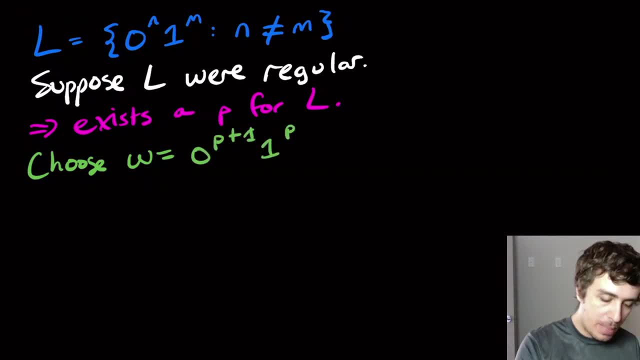 p plus 1, 1 to the p, And that's actually pretty reasonable. It's a reasonably good choice because it's length at least p. the two exponents are not the same, so we're good to go. then It turns out that this won't work, because if I put more zeros in to the left side, 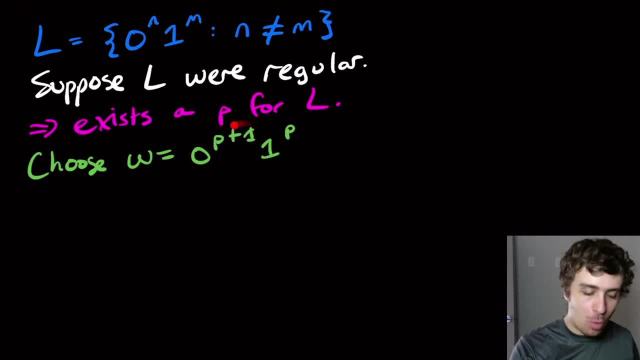 then I'm toast right Because I'm going to have more zeros, and I'm trying to get out of the language meaning that we have exactly the same number of zeros- sorry, the same number of zeros and ones. But if I put more in then I'm going to still have more zeros than ones, and that's not. 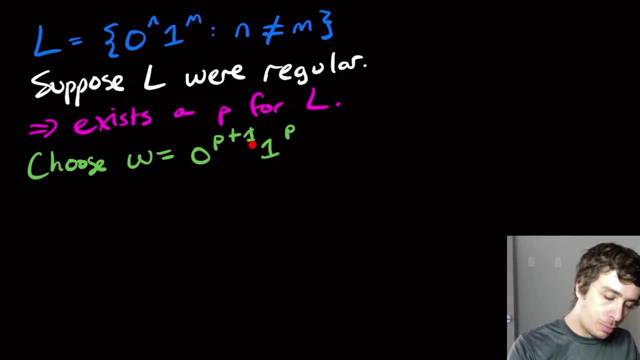 good, If I try to pump down because I want to have these two be the same, then I could subtract one from here. but I got to look at all decompositions and I might not be able to get exactly one. I might overshoot the mark and then now they're. 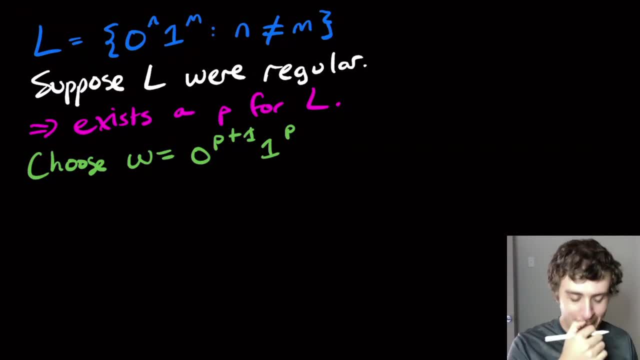 still the same. So I'm going to have to look at all the decompositions and I might not be able to get exactly one. I might overshoot the mark and then now they're still the same. So I'm going to not equal and I haven't left the language, So we're going to use something that I've done on. 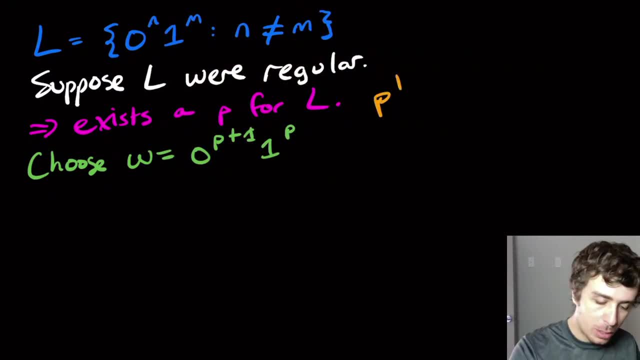 the channel and you can search for it, but I'm going to show you it again here, called the p factorial trick. It's very tricky And I did it in orange because of Halloween, obviously, But so this string will not help us. Instead, let's pick this string Zero to the p, one to the p. 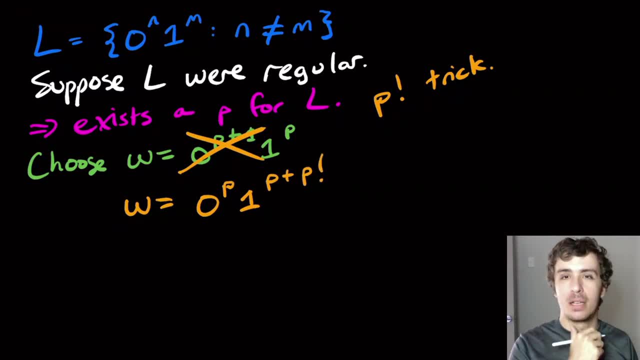 plus p factorial. Let me think How. How did you come up with that? So I'll give my reasons at the end, but the basic idea is: remember when we try to pump down here and we couldn't get nailed down exactly one Well here. 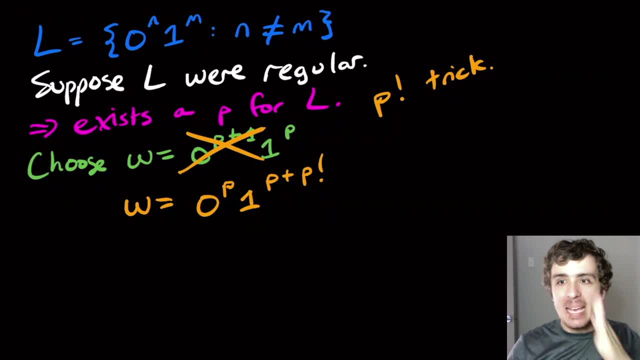 it could. the number of things we take away could be anything from one up to p. So I don't know what that is, what number it actually is. It's some number between one and p. So let's just do something that we can do. So let's just do something that we can do. So let's just do something that we can. 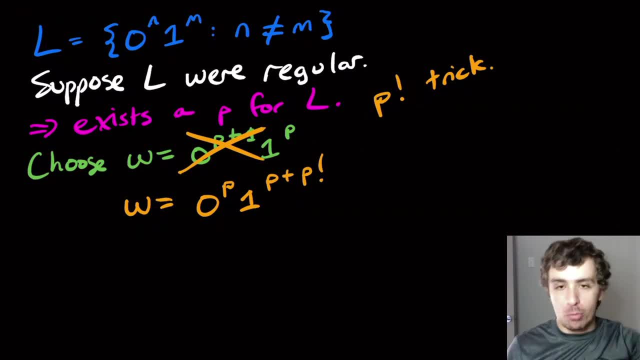 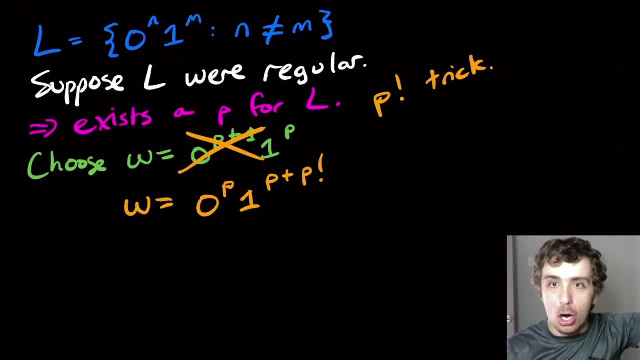 it is, we will eventually hit the same target, which is p factorial. And why p factorial is because it's equal to one times, two times, three times, blah, blah, blah, up to p. So if I pick, if it happened to be five, for example, then, and let's say p was ten- 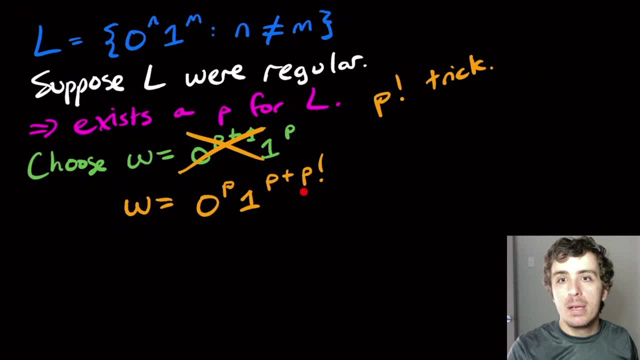 so the number of characters i'm adding or deleting is 5 and p is 10.. well, 10 factorial divides p over 5 divides 10 factorial, and so if i add 5 over and over and over, i'm eventually going to get there. an open question is whether or not you can do better than this, but this is um, this is totally. 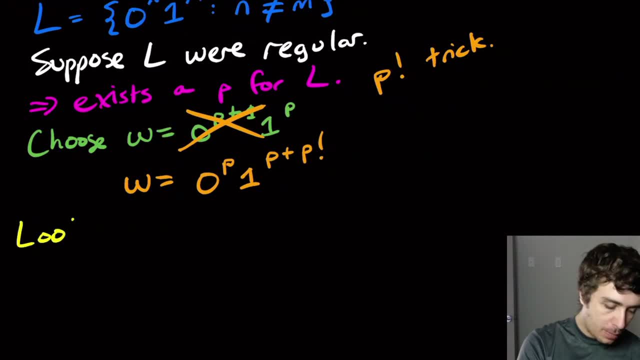 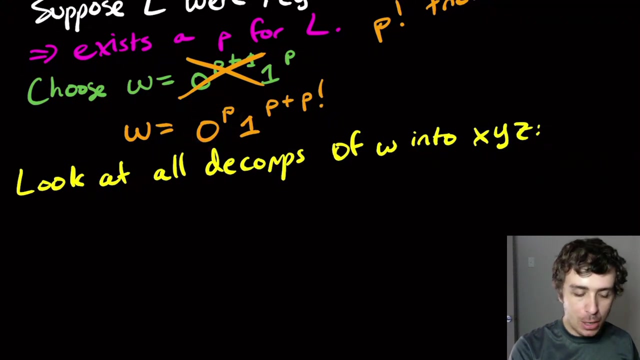 fine for our purposes. so we gotta look at all decompositions of w into x, y and z according to the rules, where x, y has length at most, p and y has at least one character. well, we know that the first uh, p characters are zeros. so we know that x and y are only zeros. 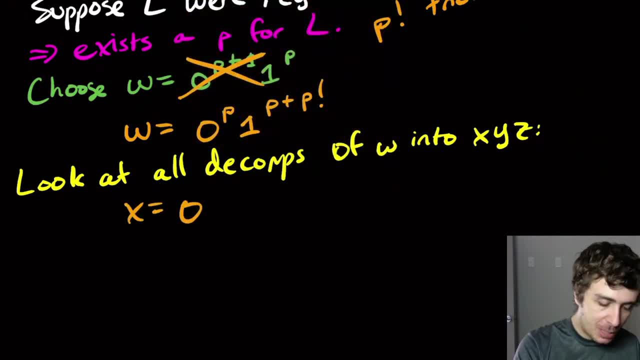 so here, we know that x and y are put before each other, and so we know that is going to be some number of zeros. let's call it alpha. y is going to be some number of zeros, call it beta, and we know that, since y is not empty, beta is. 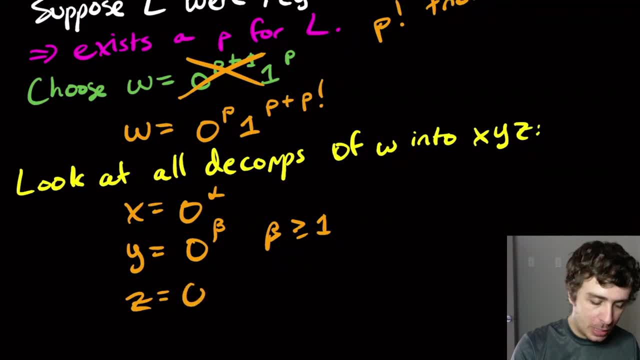 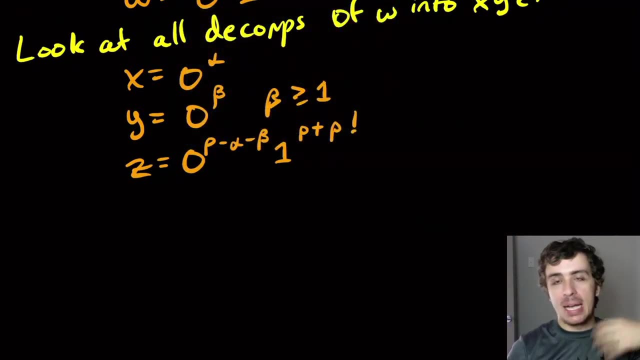 at least one, and Z is the whole rest of the string. so we got P minus alpha, minus beta 1 to the P plus P factorial- still there, okay, so then now we want to see when is this thing in the language and we want to pick an eye for which it's. 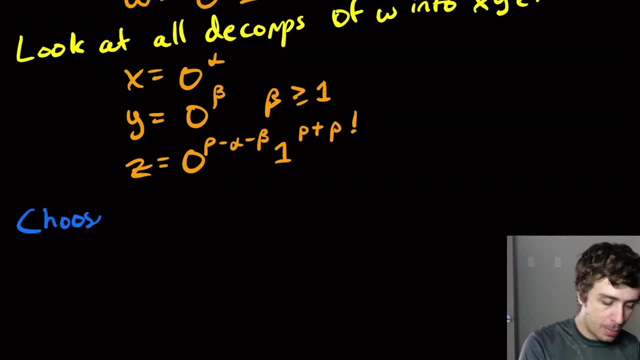 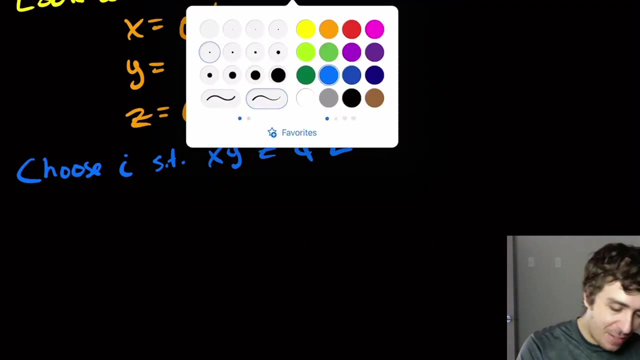 not in the language, because we want to contradict what the pumping lima says. so we want to choose an eye such that x, y to the iz is not in L. okay, but we better figure out when it is in the language so that we can figure it out later. 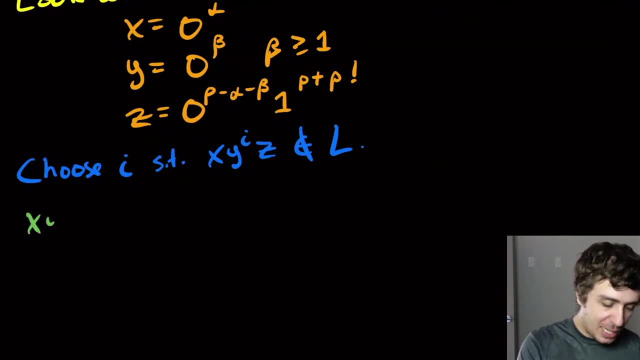 okay. so what is x, y to the I Z? well, let's just copy down the pieces. so we have 0 to the Alpha, 0 to the i beta, 0 to the T, so try and find two 2's, okay. and then find 0 to the x? y to the iZ. soク porکân. 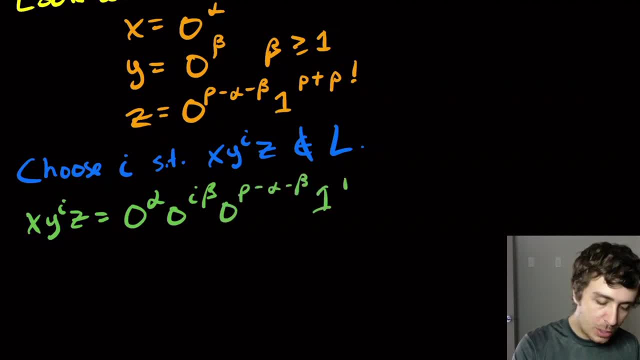 the p minus alpha, minus beta 1 to the p plus p factorial. and let's collapse the zeros again. so we have 0 to the p minus. so the alphas get killed off. I should say p plus i beta minus beta 1 to the p plus p factorial. so what we can show. 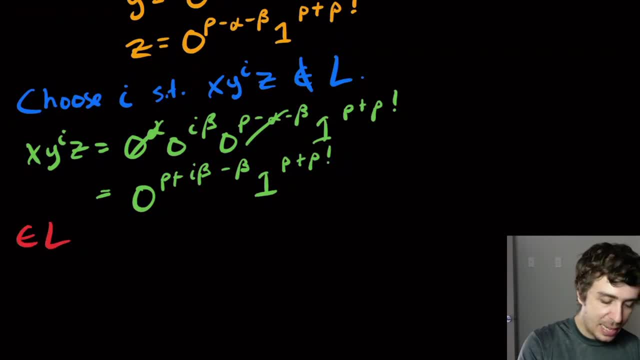 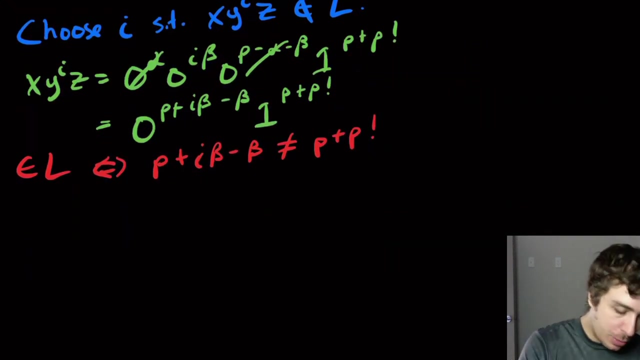 here that that this thing is in the language if, and only if, these, these two numbers are different. it's in language if and only if they are different, because that's what the language was defined to be. so p plus i, beta minus beta is not equal to p plus p factorial. so if, and only if, well, we can subtract. 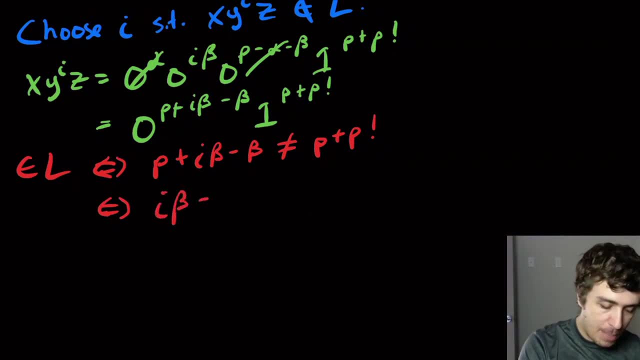 the p in both sides is equivalent, so i beta, beta minus beta is not equal to p factorial. So let's factor the left side, So beta i minus 1 is not equal to p factorial. Well, since we got to make an assumption, 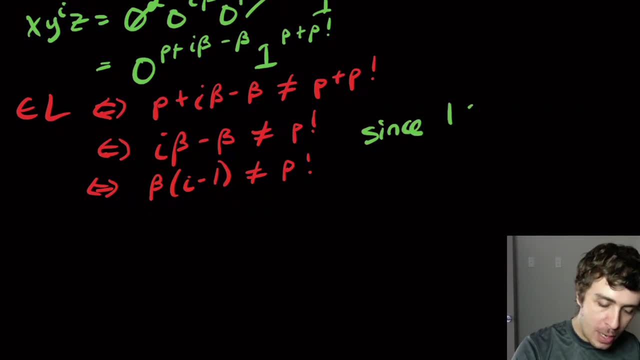 So, since 1 is less than beta, so beta is at least 1, that's the condition, But it's also at most p, Because the first two pieces are of length at most p. Well, the second piece, therefore, is at most length p. 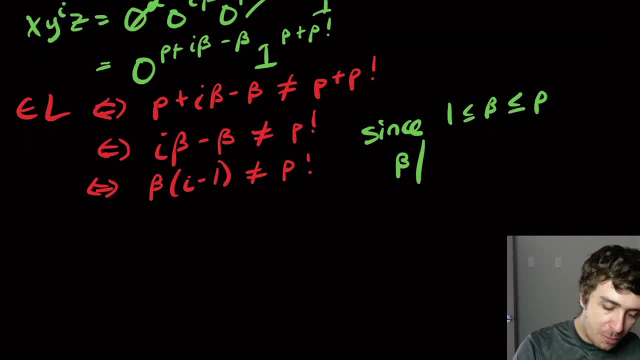 So that implies that beta divides p factorial. So if you haven't seen this notation before, this means that b is a divisor of this. So we can divide by beta on both sides and I have an integer on both sides. So if, and only if, i is not equal to p, 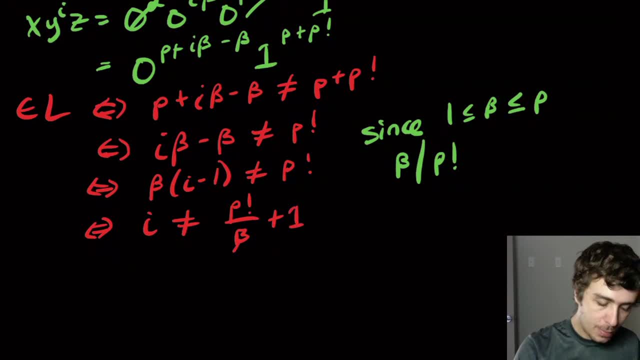 Factorial over beta plus 1.. So as long as i is not equal to this specific number, then we're in the language. So let's pick that number to get out of the language. So let's choose i to be p factorial over beta plus 1.. 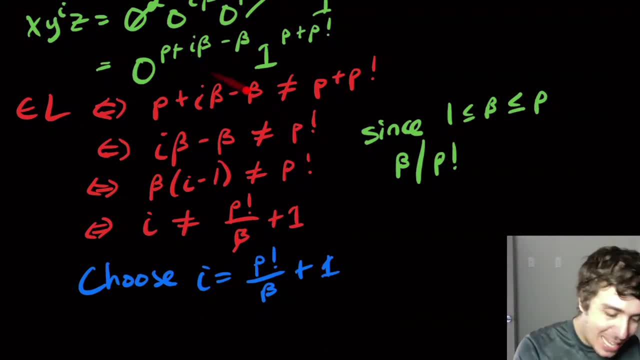 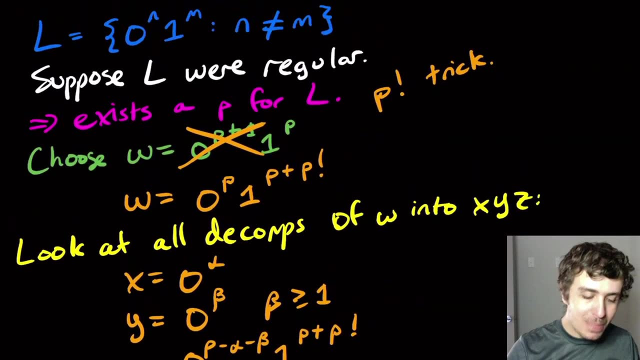 And that's it. And if you substitute it back in, then we're gonna have the same number of zeros and ones, So a very complicated To a problem that's very, very similar to a different one, which it's way easier. 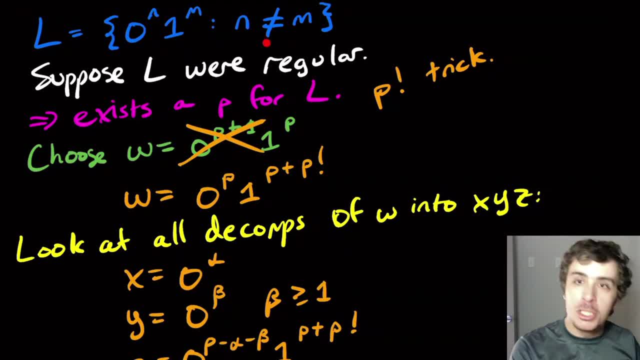 Which shows that getting two numbers to be equal is way harder than getting two numbers to not be equal, Because there are a lot more numbers that are not equal to something than there are equal. Cool, So we have shown that 0 to the n, 1 to the m, where the two exponents are different, is not regular. 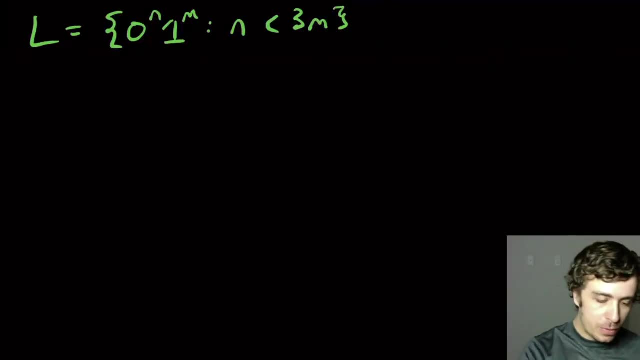 All right, so let's prove that this language, 0 to the n, 1 to the m, where n is less than strictly, less than 3m, is not regular. So this turns out to be a very standard proof. So let's suppose that l were regular. 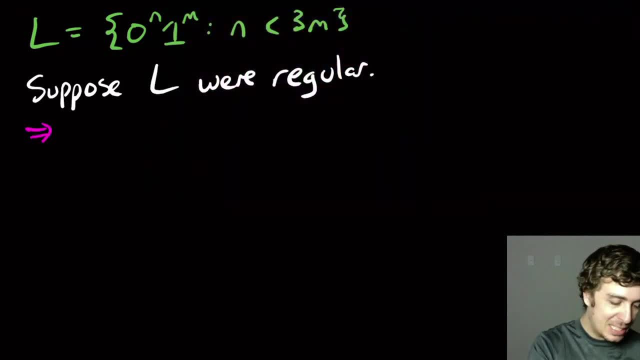 Then, by the pumping lemma, there exists a pumping constant p. I'm just going To abbreviate it to exist a p for this particular language, l. So now what we need to do is we need to pick a string that is in that language, l, and has length at least p. 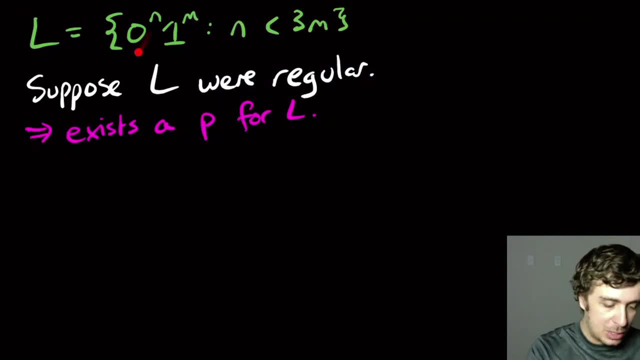 So let's think: Well, let's pick a string that has some number of zeros, some number of ones, and the number of zeros is strictly less than three times the number of ones. So what we want is a lot of zeros, because 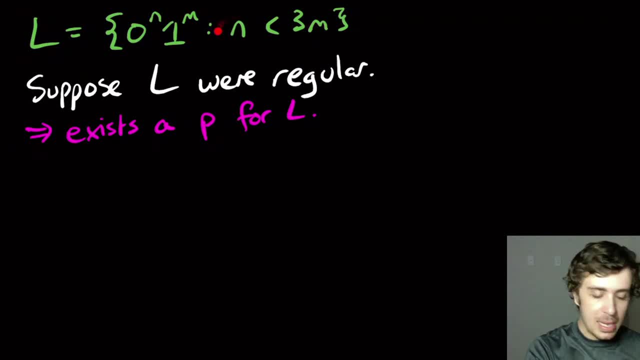 We're going to be multiplying the number of ones by three. that's in the range of where n needs to be, because we want to eventually contradict this. So let's choose, Let's see. So what can we pick? Well, what I'm going to do is I'm going to pick p ones, to start with. 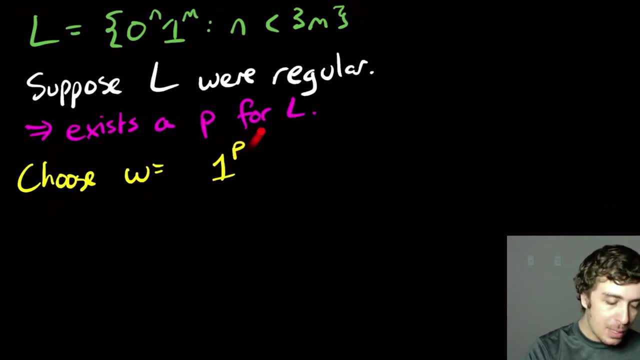 And what we need is that the number of zeros is less than three p, because that's what the condition up here is saying. So what I'm going to do Is I'm going to pick zero to the three p minus one. So this is just barely in the language. 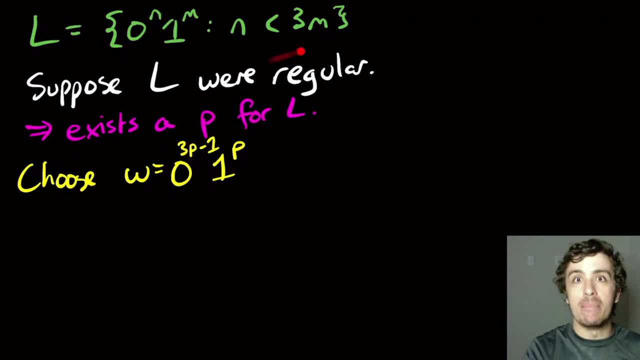 If I had one more zero, then it's going to immediately leave the language And in fact that's exactly what we're going to try to do. So this is the string that we're going to pick. It's in the language because it matches the condition and it has length at least p. 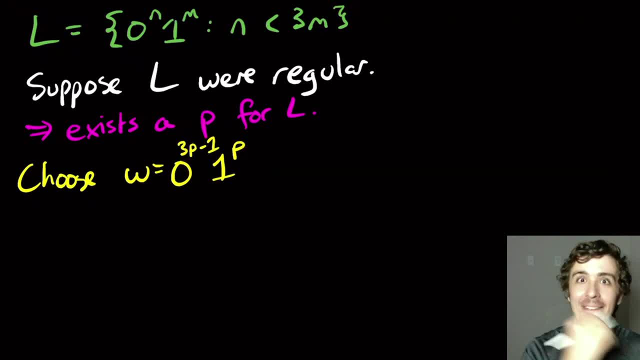 In fact, it has four p minus one, which is definitely at least p Cool. So what we need to do now is we need to look at all the compositions of this string into those three parts, according to the rules. So look at all the compositions. 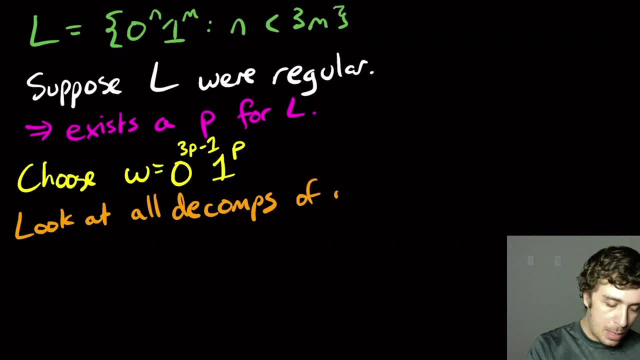 I'm going to abbreviate it to decomp again of w into x, y and z, And the rules are that x and y have length at most p and y is not empty, So y has length at least one. So what are these? 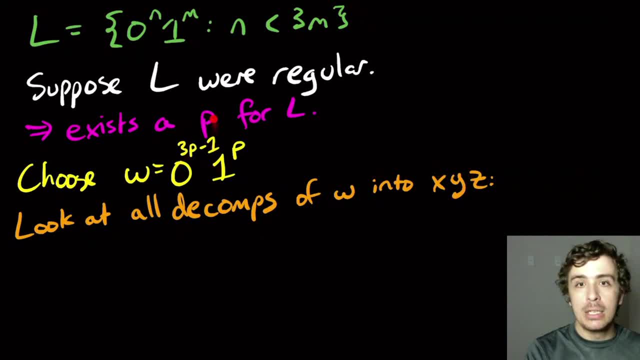 Well, Uh, x, y has length at most p, and the first p characters at least, are zeros. So we know that x and y parts are consisting of zeros. So x is some number of zeros. I'm just going to call the number of zeros alpha. 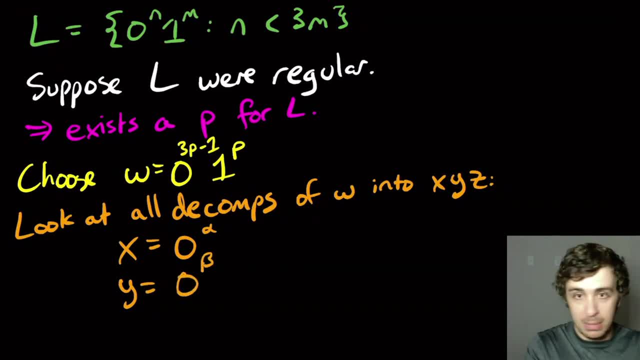 Y. I'm going to call the number of zeros beta, because they may be totally different from each other. Beta is at least one, because we know y is not empty and z is the whole rest of the string. Well, we have three p minus one. 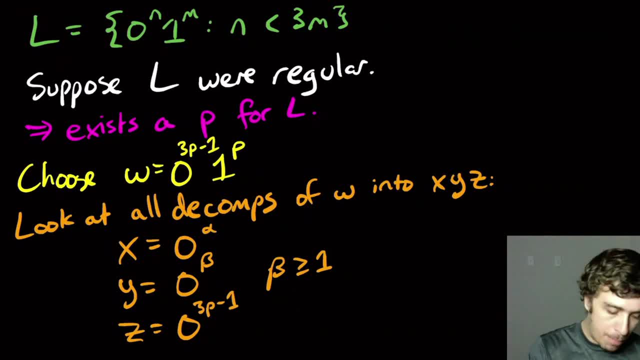 Zeros in total, minus alpha, minus beta, from the x and y, taking that many zeros, And then we have all of the ones still in there. Okay, So this is just one. All possible decompositions are of this form that we ever need to consider. 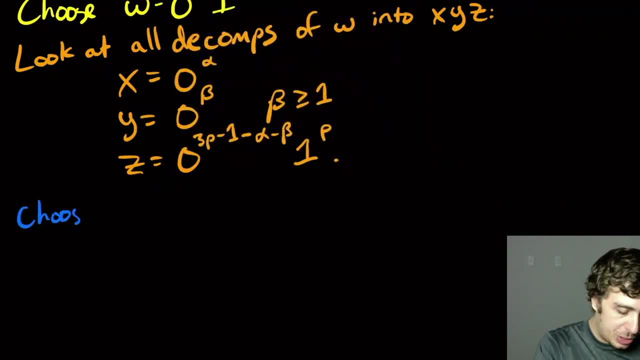 So what we need to do now is to choose some value i, some number i, such that x? y to the i is not in L, because we want to contradict the for all statement in the pumping lemma. So let's look at what x? y to the i is. So x? y to the i z is. let's just copy the pieces down So we have zero. 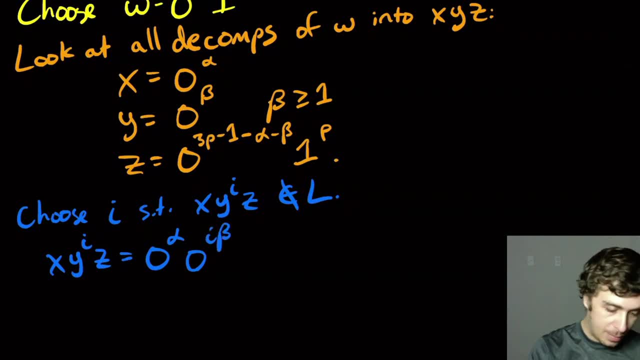 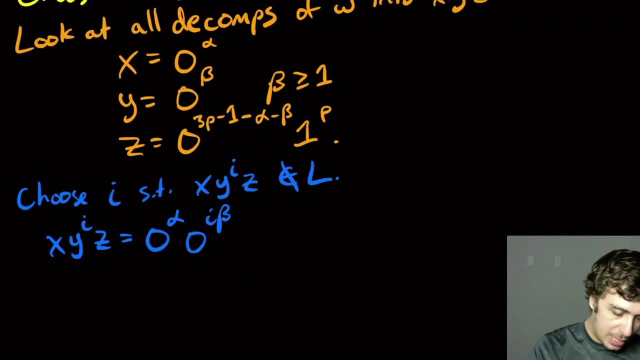 to the alpha, zero to the i beta, because we have i copies of y and then I'm just going to copy z down, So I'm going to do it again. So zero to the 3p, minus 1, minus alpha, minus beta, 1 to the p. 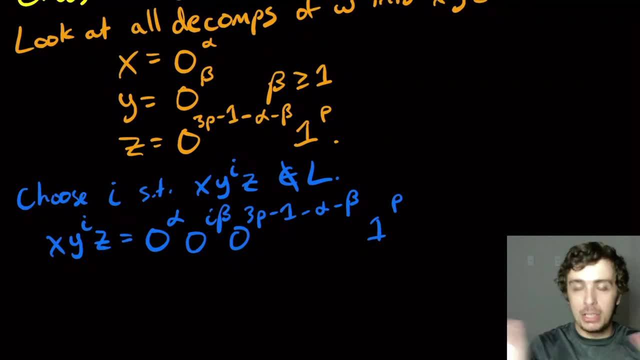 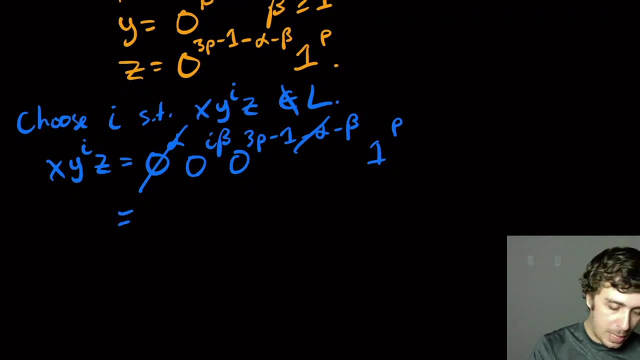 So this run of zeros, we have a run of zeros here, so I can just collapse the exponents down. So the alphas are going to get killed off, plus alpha, minus alpha. So here we're going to have zero to the 3p minus 1, plus i beta. 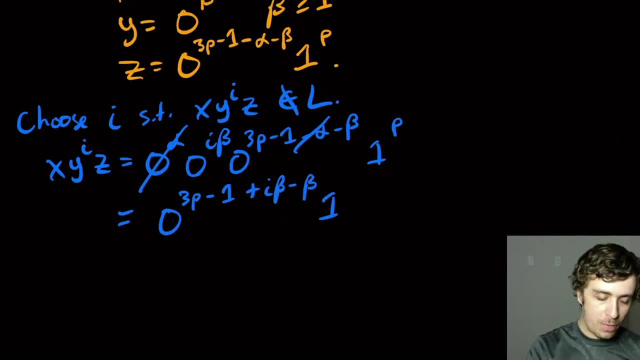 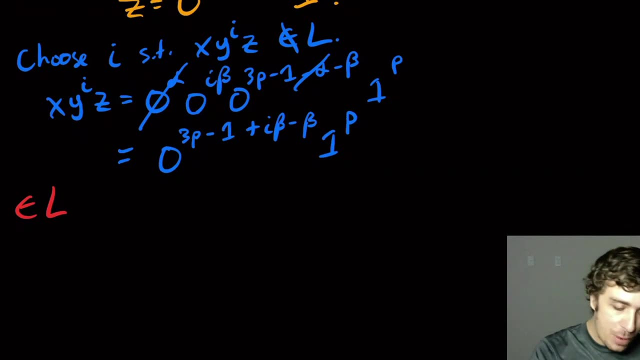 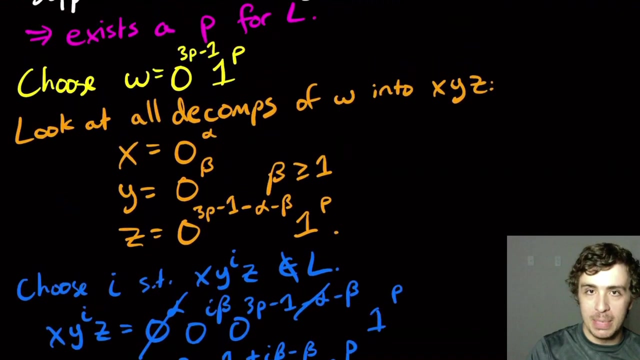 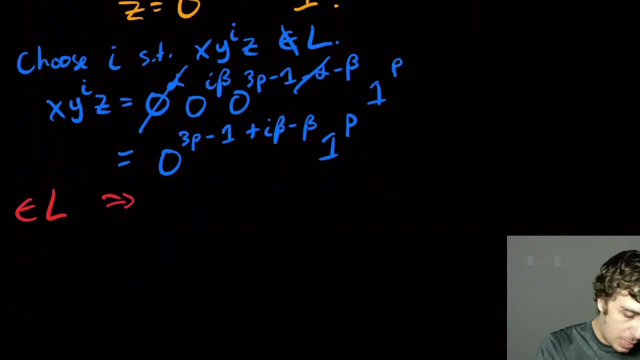 minus beta, and then all of the ones are still there. So what we can reasonably conclude now is that this thing is in L if, and only if, the number of zeros is strictly less than three times the number of ones, because that's exactly what the language is saying. So it's in L if, and only if. 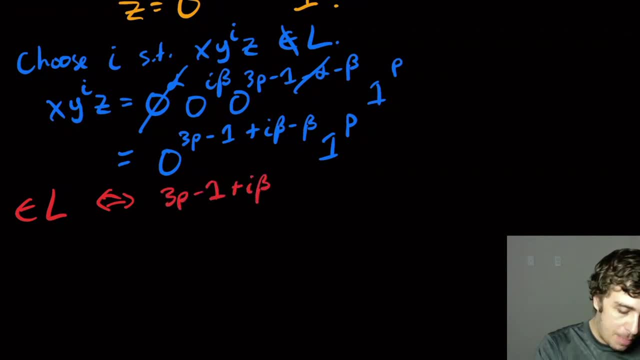 3p minus 1 plus i beta, minus beta is strictly less than 3p, three times the number of ones, which is what that is. So this is if, and only if, we can minus the 3p on both sides, it's exactly the same. 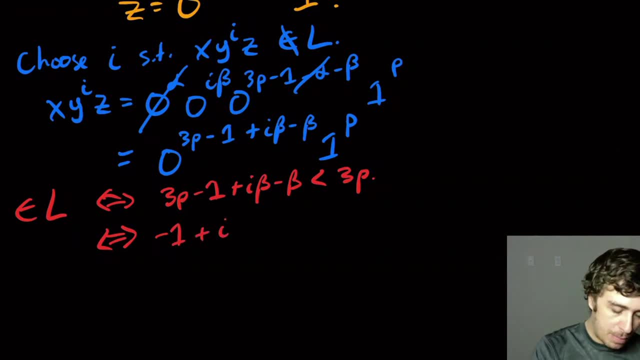 it's equivalent expression. So minus 1, plus i beta, minus beta is less than 1.. And then I'm just going to algebraically manipulate things. Oops, this needs to be zero, because I submitted it. So I'm going to do this. So I'm going to do this, So I'm going to do this. 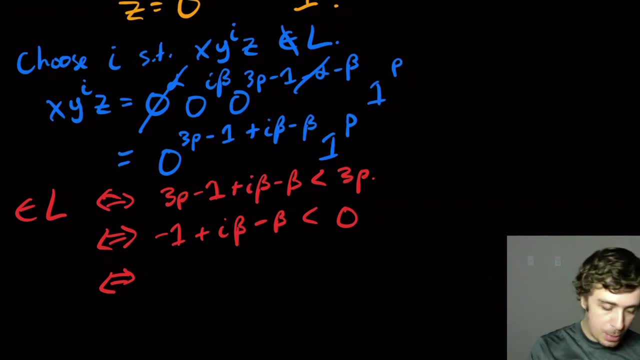 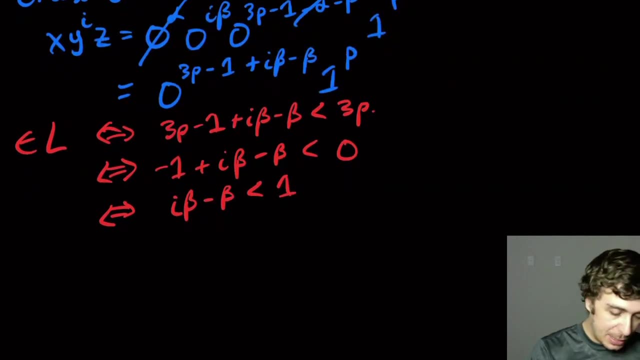 So I subtracted 3p on both sides, So then I add 1 to both sides, So i beta minus beta is less than 1.. And then let's see: So if we pick an i such that this right, this left-hand side, is strictly. 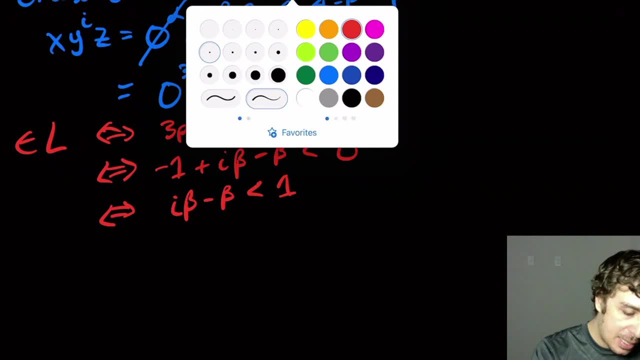 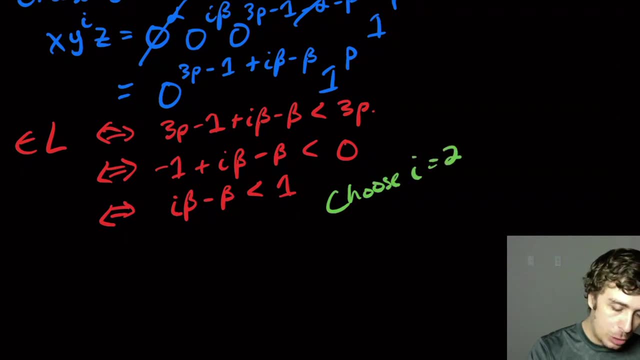 is either 1 or bigger, then we're done. I claim that we can pick 2 for this, So let's choose i equal to 2.. Well then, what happens is 2 beta minus beta is equal to beta, And we know that that is at least 1, because 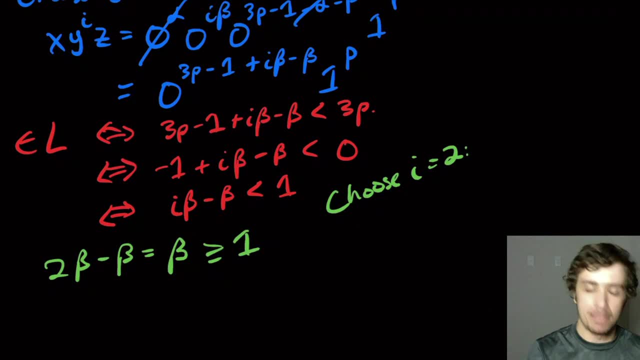 the part that we pump is not empty, So this thing is at least 1.. And so that contradicts the fact of this being less than 1.. And so it is not in the language for that reason. So, x, y to the power 2,. 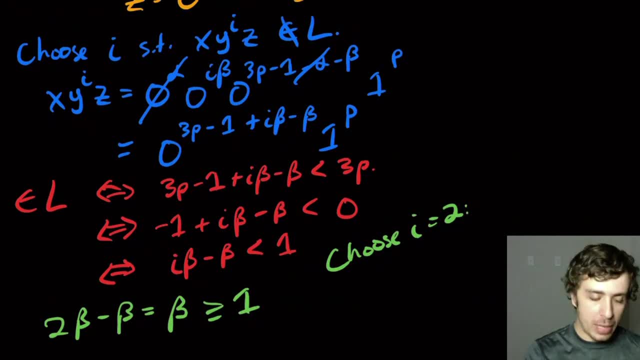 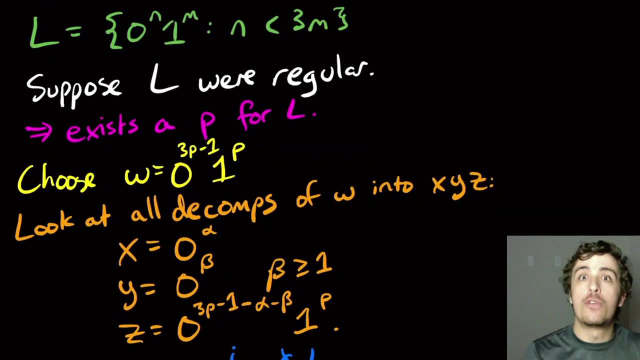 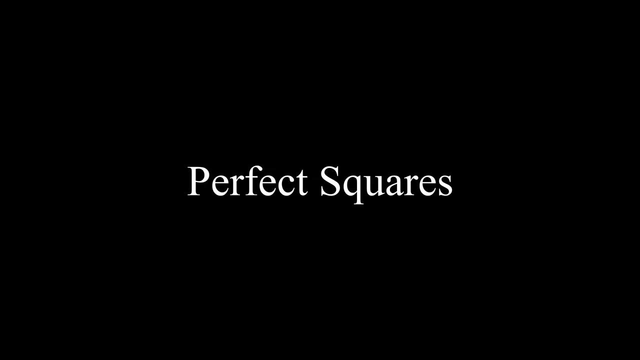 z is not in the language And then therefore, that contradicts the for all statement saying that based on the assumption that this were regular And so therefore it is not regular. Okay, So let's prove that this language is not regular. So n squared up here is for all. 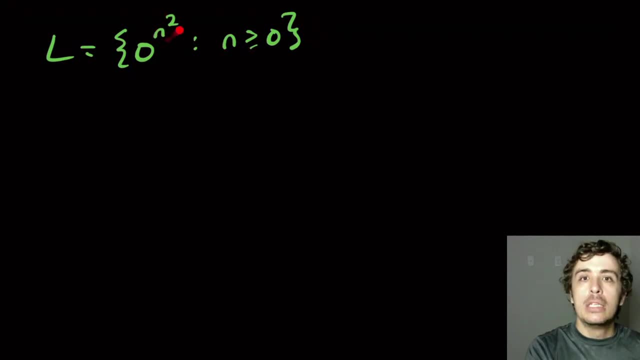 integers, at least n, sorry, at least 0.. So this represents a perfect square number of zeros. Okay, So, like oh, 0 zeros are in there. so the empty string, or 1 zero, or 4 zeros, or 9, 9 zeros, 16 zeros, etc. 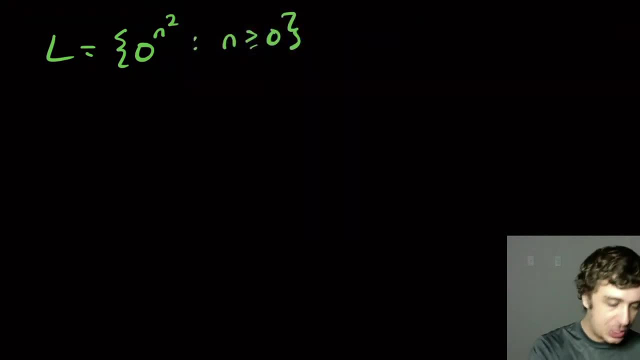 And we claim that this is not regular. So let's proceed as we would normally do. Suppose l were regular, Then what we know is that there exists a pumping constant p for this language l. then what can we do? well, we need to pick a string that's in the language. so the usual technique is: 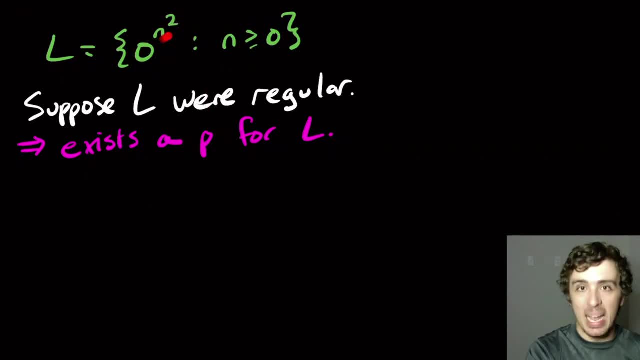 to substitute the p into the exponent right here. where n is not n squared, it'd be n. so the string that I'm going to pick here choose w equal zero to the p squared. well, that's clearly in the language, because I just substituted the number in, and p squared is always at least p when p is an integer. 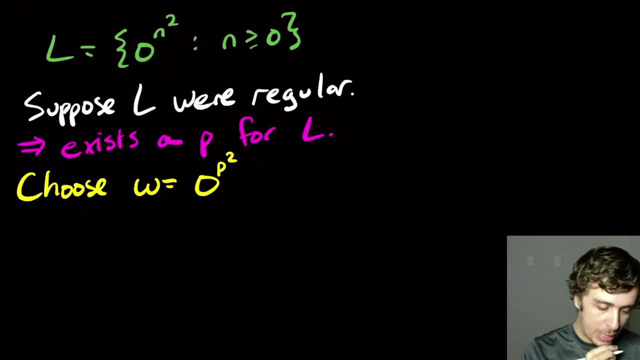 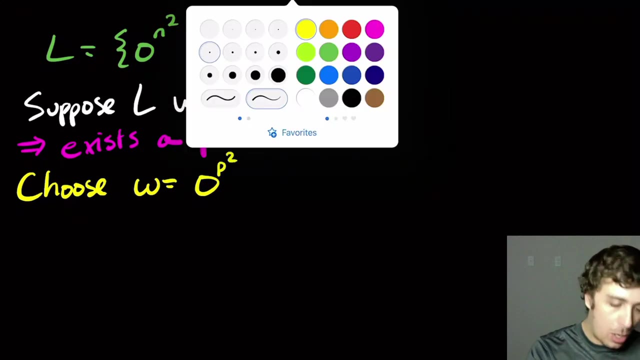 and so that's. that's all that we actually need. it turns out that this string does work. generally, if you have a string that's in the language and long enough, it's not necessarily going to work, but in this case it does. so what are we going to do? well, we got to look at all decompositions of 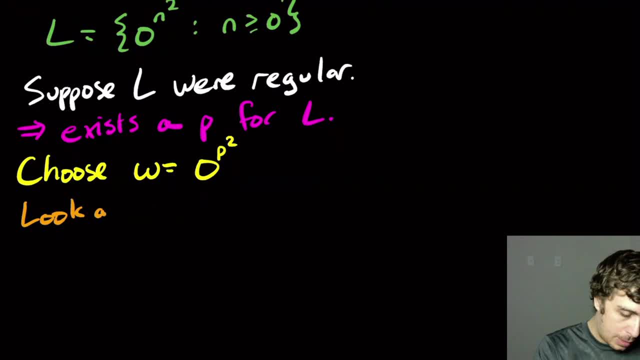 the string into those three parts. so look at you all decomps of w into x, y and z, according to the three parts. well, since the whole string is zeros, here we know that the x part is going to be some number of zeros, y is some number of zeros, and 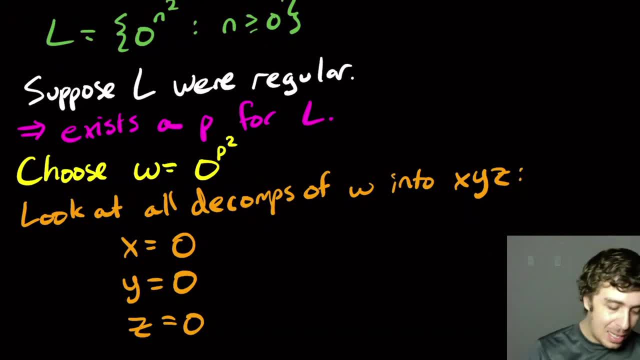 z is some number of zeros, because the whole string is zeros. um, let's call the x part alpha number of zeros. y is a beta number of zeros, where we know beta is at least one, because y has to be non-empty. and then the z part is p squared minus alpha, minus beta. okay, so let's, let's. 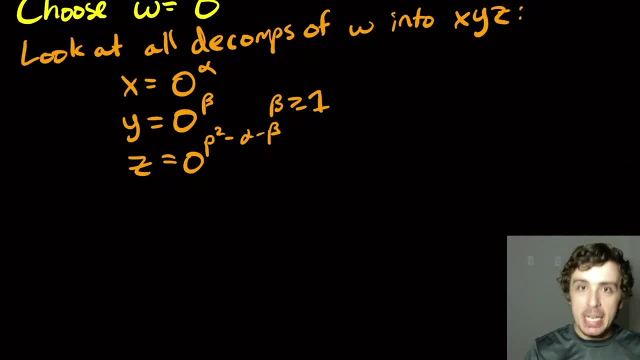 think: well, here, what I'm going to do is I'm going to pick a particular choice of i's. so actually, first off, what do we need to do? well, we need to choose some value i, such that x, y to the i z is not in the language, because that would contradict the for all statement of this. 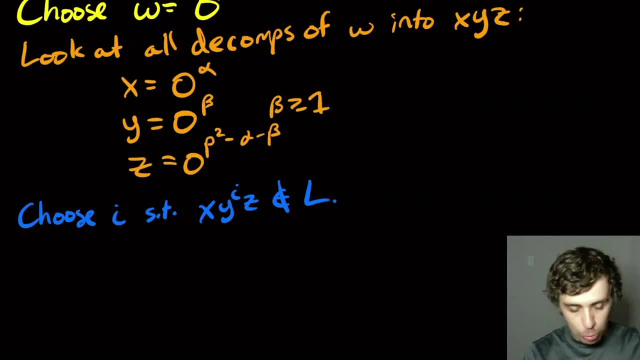 beta, so we're going to pick a particular choice of i's. so, actually, first off, what do we need to do? well, we need to being in the language um, and then we'll show us that it's not regular. well, here I'm going to pick a particular choice of i and we'll see why it works. the reason for that is it's hard to get. 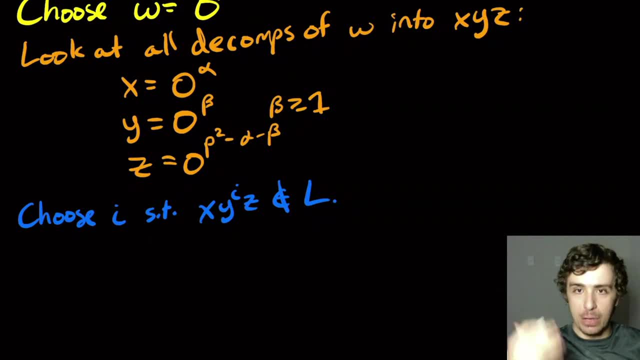 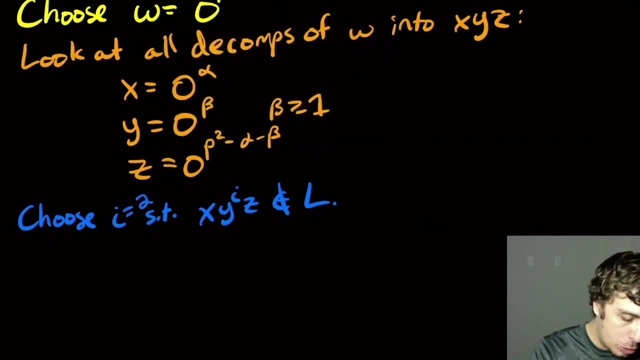 this to work in the general case, but if you look at a specific example, it's a lot easier. so what we're going to do here is: I'm going to pick: i equal to 2. okay, it turns out i equal 3 also works, but, um, i equals 2. 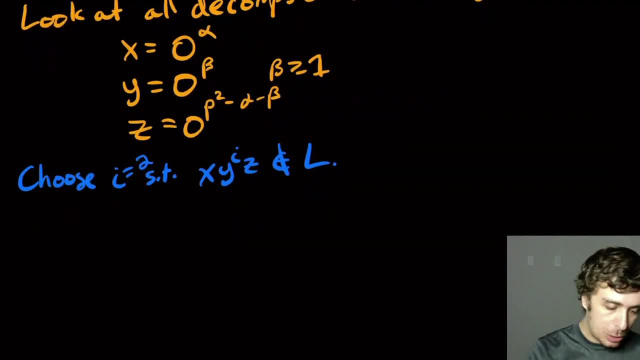 is the one that is usually done and the one I'm going to do here. so what is i's? what is this string x, y squared z? and we want to show that it's not in the language. we don't know that it actually is not in the language yet, but we need to show it, so let's just copy down the pieces. so zero to the. 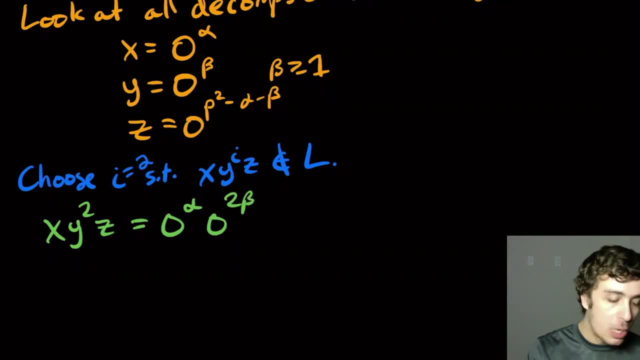 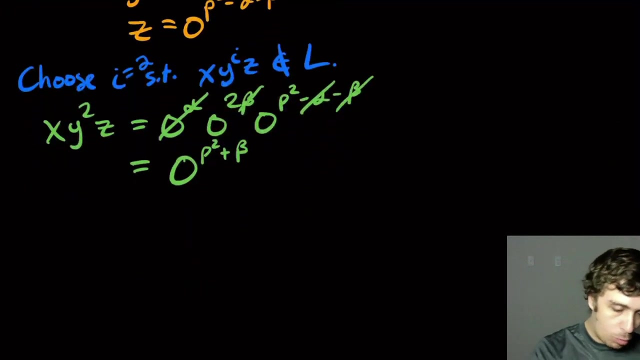 alpha zero to the two beta, because I have two copies of y here and then the z part, which is just copied straight down from the decomposition upstairs, and then, when the dust settles, the alphas get killed off and one of the betas gets killed off. so I'm going to have p squared, my plus beta here. okay, and what we need to show or prove is that 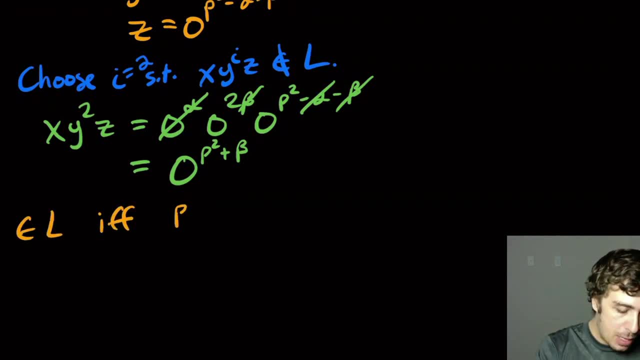 this is thing is an l if, and only if, p squared plus beta is a perfect square. well, let's see. so let's see if we can get this to work. so let's see if we can get this to work. so we know that p squared is strictly less than this number that we just derived, and how do I know? 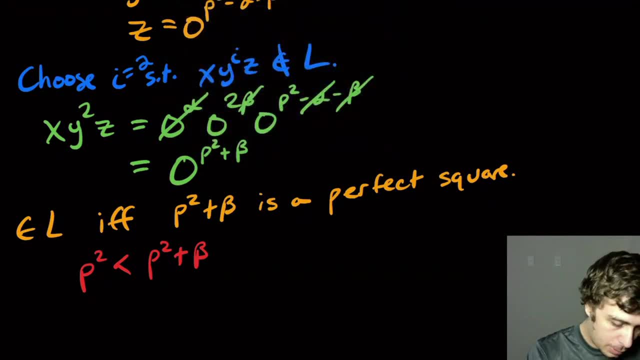 this and I'll actually put it below. so we know that because the beta itself is at least one. and we know that because the part that we pump, which is which length is beta, has to be the part that we pump is not empty. so the number of characters must be at least one. so we know that because the 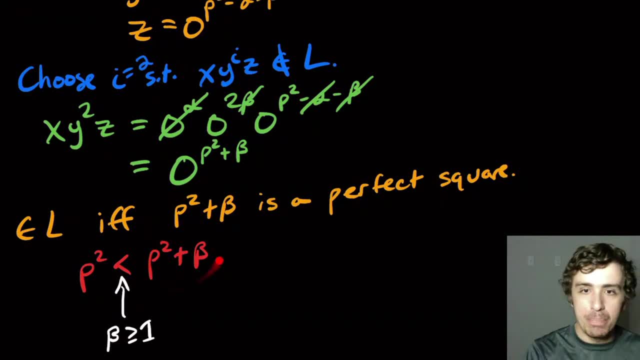 beta itself is at least one. so this thing is at least p squared plus one, but it could be a lot higher, but it is definitely at least one. so we know that it's not equal to this perfect square right here, because it's strictly larger than it, but it turns out that this thing is always at most. 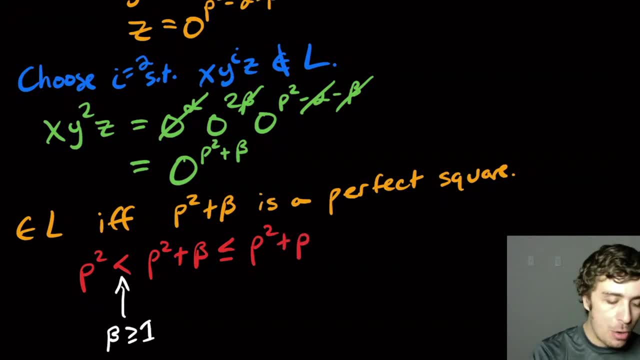 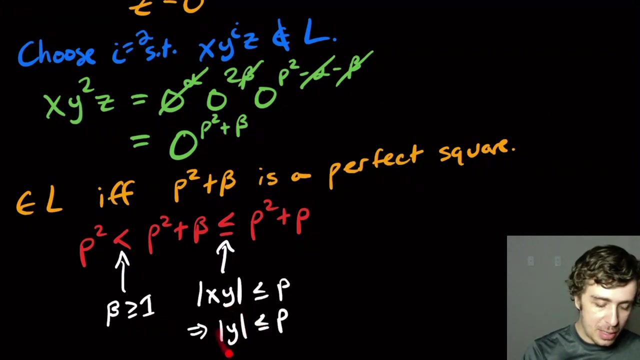 p squared plus p. and how do I know that? well, I know. let's put it below. I know that because the length of x, y whole thing is at most p, which implies that the length of y is at most p and the length of y is beta. so the largest that the length of y could ever be is p characters. 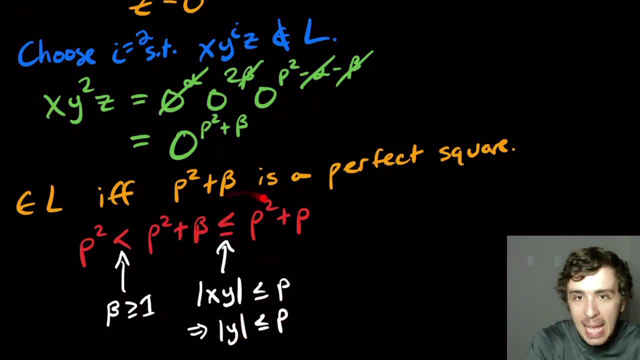 so this thing is at most this. it could be a lot less, but it's certainly at most this. but I actually claim that this is strictly less than the next p squared plus p squared plus p squared. so this is a perfect square upward after p squared. so this is a perfect square. this is. 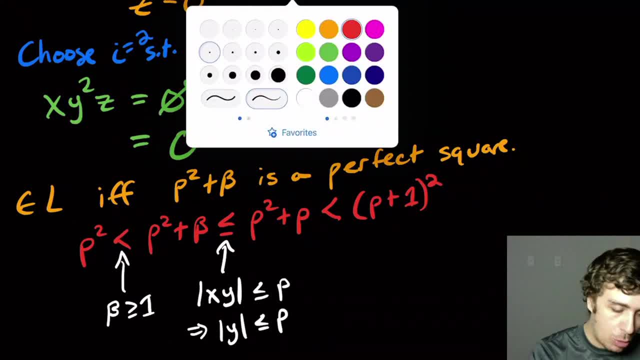 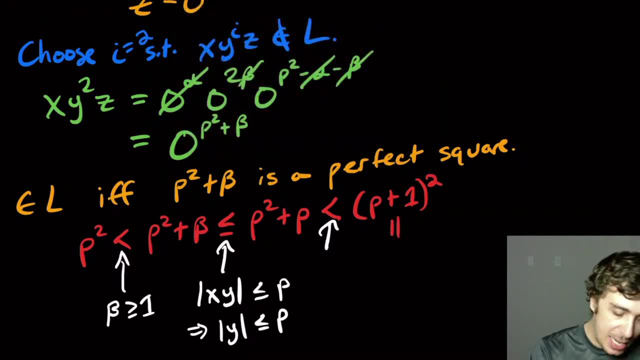 clearly a perfect square, and I claim that there's a strict inequality there. and how do I know that? well, let's see. so this, this right hand side, is equal to p squared plus 2p plus 1, and the reason it's a strict inequality is because of that, it's because of that little bit right there, so that plus. 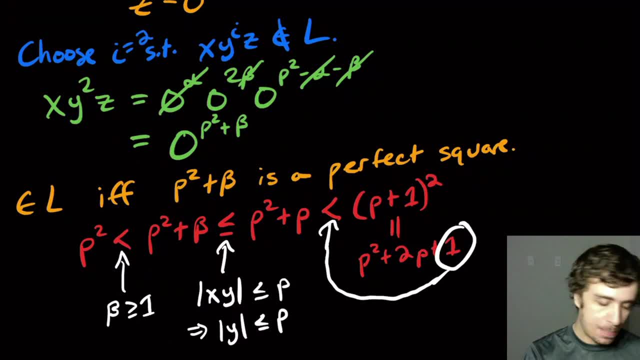 1 gets that this is a strict inequality. so what we have derived here is that the length of the, the of the string that we just made, is not equal to that perfect square because of the strict inequality and it's not equal to that perfect square because of that strict inequality. and 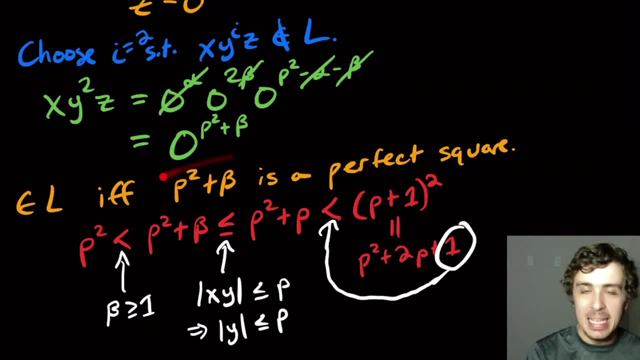 there's no perfect squares in between these, because they are consecutive perfect squares, and so therefore, this length, whatever it is, is not ever a perfect square, and so that that's how you show that this is not a regular language, because if it were, then we would always hit. 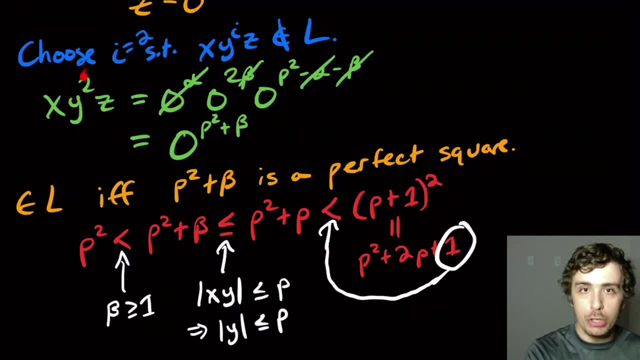 a perfect square, no matter what I value you choose, but we just chose one where we landed on a non perfect square- the this thing right here. so this actually gives you good reason to why the I equal 3. what I mentioned earlier also was not a perfect square, but it is rather from the previous point of Anna and to step aside from that, because now we have this f? squared. 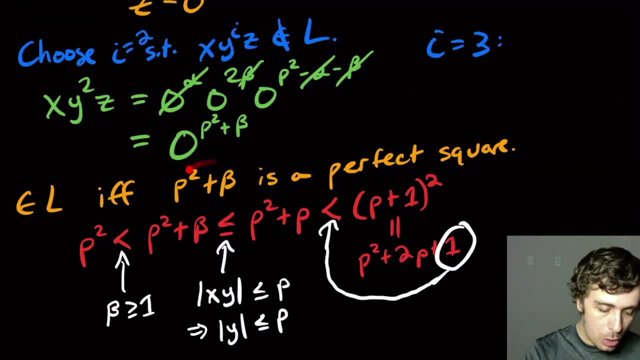 works because if you substitute i equal 3, you're going to get a p squared plus 2 beta here, and then here the upper bound will be p squared plus 2p, which is still going to be strictly less than p squared plus 2p plus 1. so the i equal 2 and the i equal 3 also work. i think maybe the i equal 0. 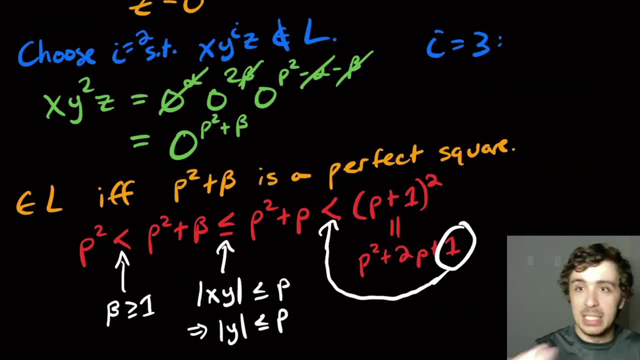 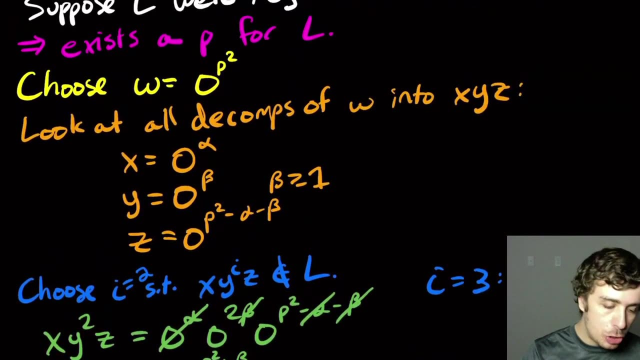 one also works, but i haven't checked- but higher ones. it's a lot harder to make sure that it's not actually a perfect square because it because it could potentially be equal to this one if it goes any higher than than p squared plus 2p. okay, cool, so that's how you show that the perfect. 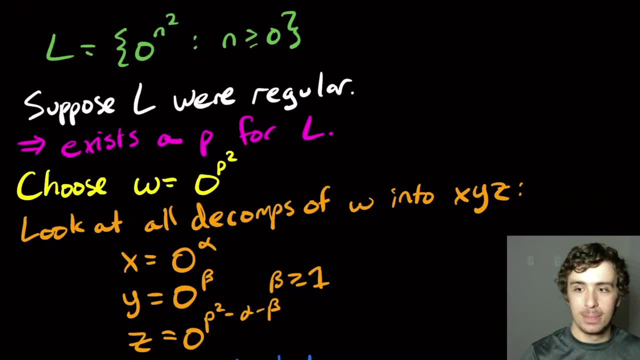 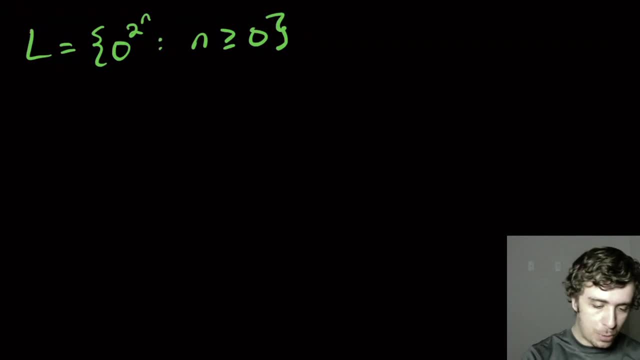 squares language is not regular. so i, i, i to prove that this language, which is the set of all strings of zeros that are a perfect power of two, for any power of two that you want- is not a regular language. so, for example, in here we have a single zero which corresponds to when: 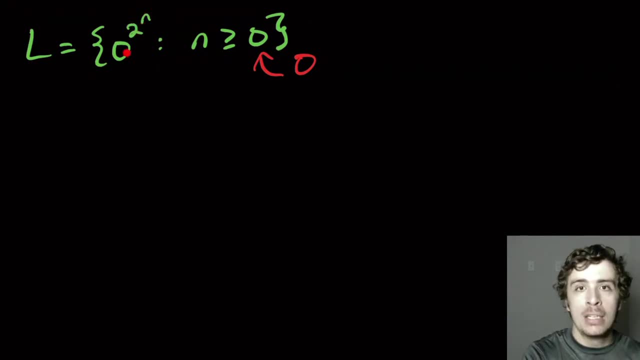 n is zero, two to the power: zero is one, so that's one zero. we also will have two zeros and then four zeros, and then then eight zeros, and etc. so I want to convince you that this is not a regular language, so let's suppose that it were. 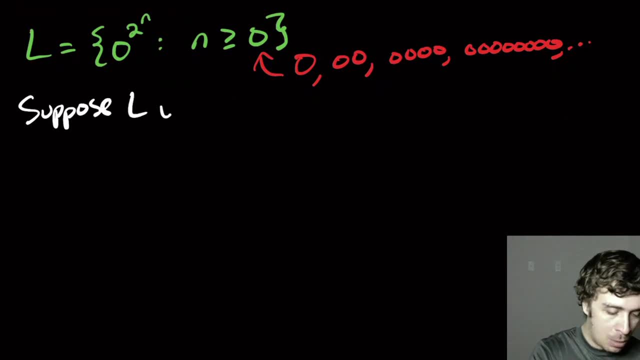 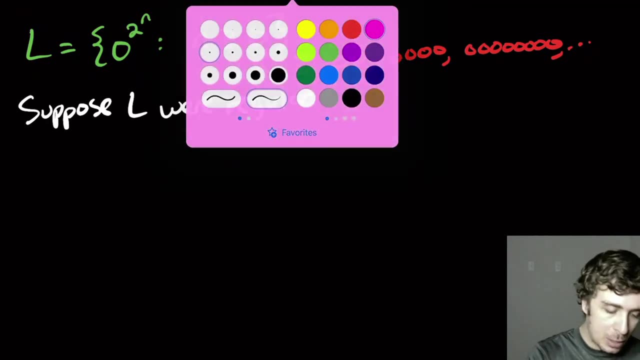 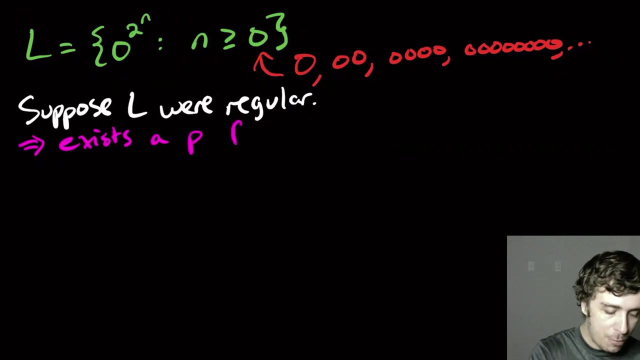 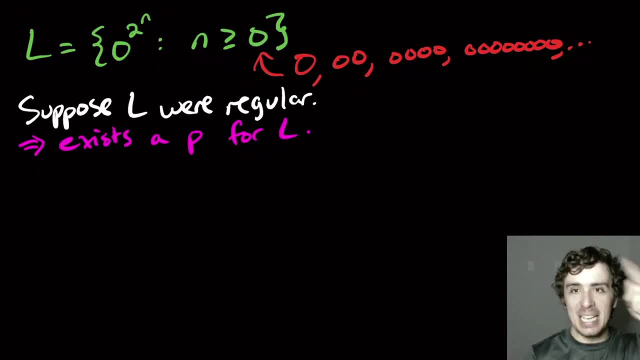 then now what we need to do is we need to pick a string that is in that language and of length at least P. so let's choose some string W, well. well, the usual convention is to place the P wherever there's the variable in the exponent. so here I'm gonna put 2 to the power P. well, 2 to the P is definitely at. 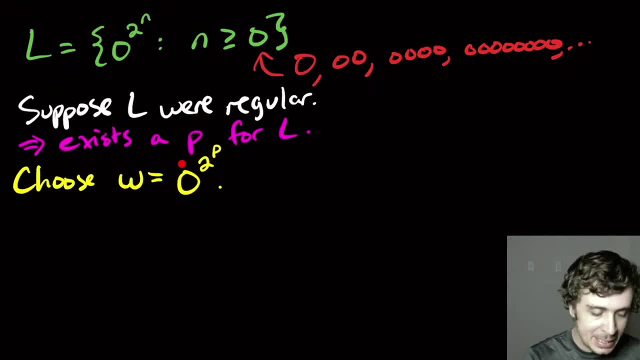 least P, so that's no problem. and this is in the language, because I just substituted the variable in, so that's no problem. so what we need to do then is to look at all decompositions. look at all decompositions of this string W into X, Y. 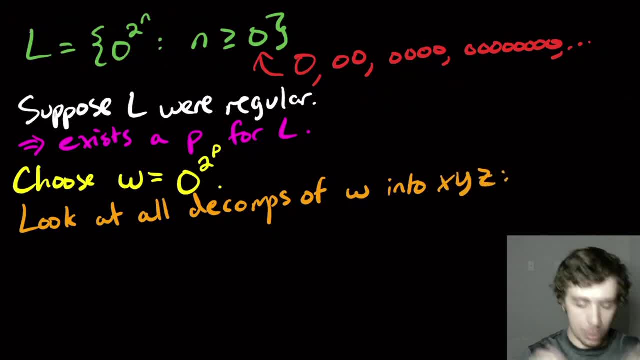 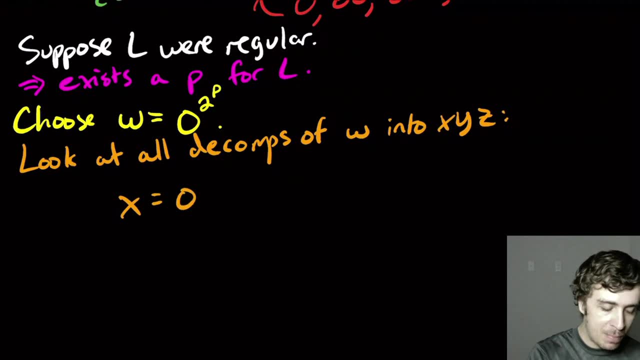 and Z, according to the three, into the coordinates of the rules. so here, since the string is all zeros, we know that X, Y and Z are equal to zero. so we know that X is some zeros- let's call it alpha- the number of them, Y, is some number of zeros. 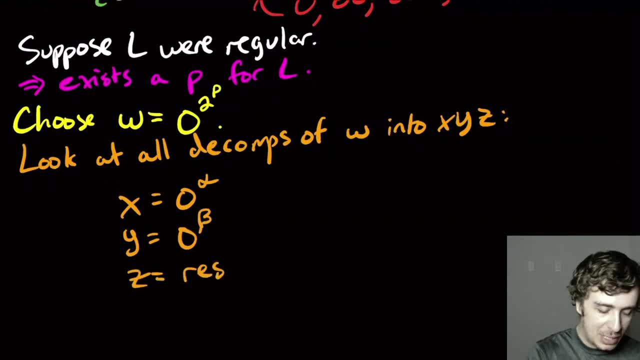 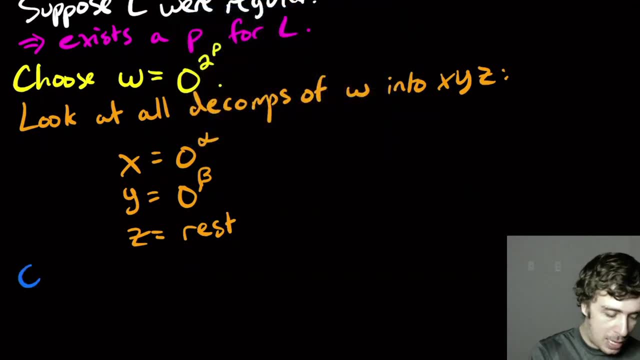 let's call it beta and Z is the rest. I'm just gonna be lazy and say: rest here. so then now what we need to do is we need to choose a value, I, so some number, I such that X, Y to the I. Z is not in L because it would contradict the for-all. 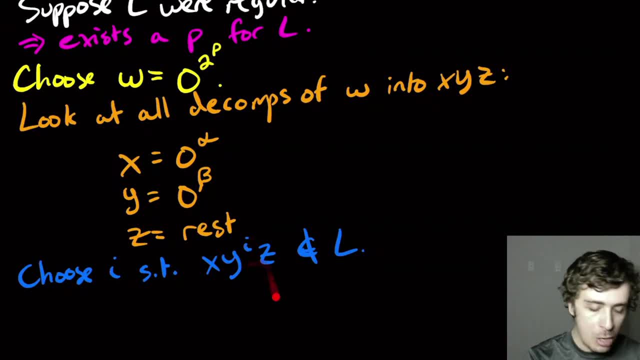 statement that that X, Y to the I, Z is not in L because it would contradict the for-all statement that that, no matter what I you pick, you always stay in the language. but here we want to find one where you get out. so let's think: well, if we so, here we're dealing. 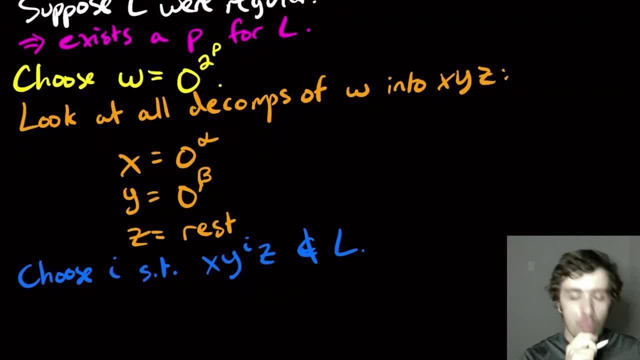 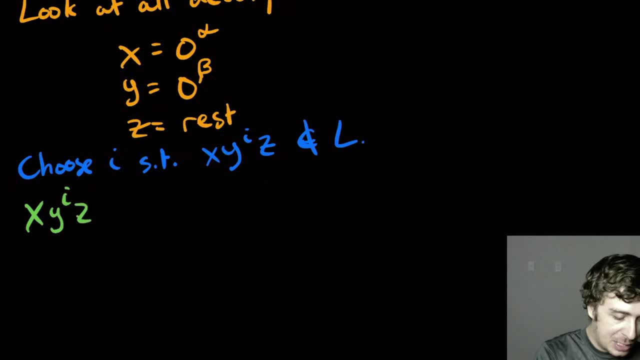 with perfect squares. so if we so, let's actually look at this. let's look at this in general. so what is X, Y to the I, Z? so that is equal to just copy down the X piece. then I have I copies of the Y piece. so I. 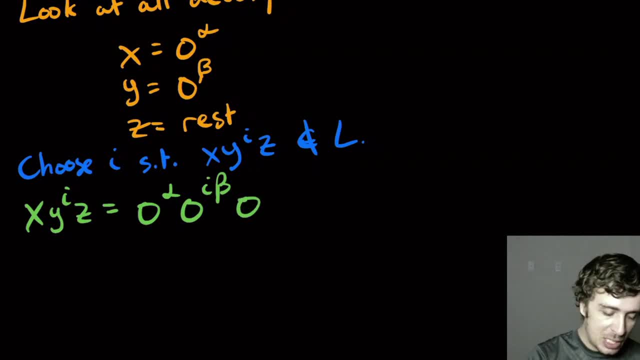 times beta, number of zeros. and then the Z part. well, that's gonna be P, 2 to the power, P minus alpha, minus beta, because we had 2 to the P to start with. the X piece took alpha away and the single Y took a single beta away, and and that's. 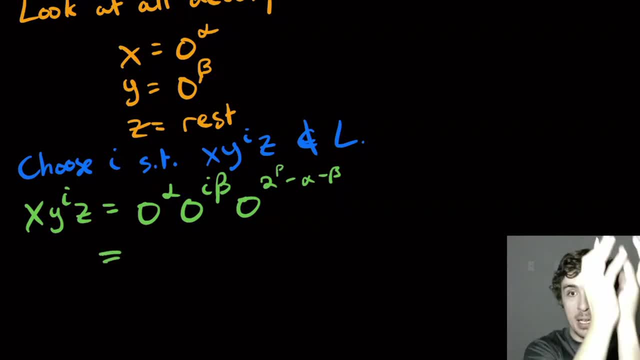 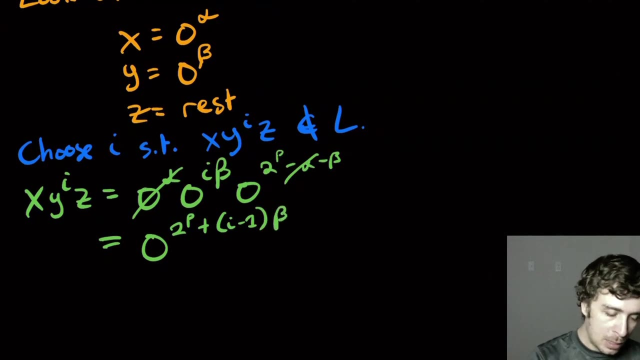 the whole string. so since we have all a whole bunch of zeros, we can collapse them together to get a single exponent. well, the alphas are gonna cancel. so I'm going to have 2 to the power, P plus I minus 1 times beta. so what we can. 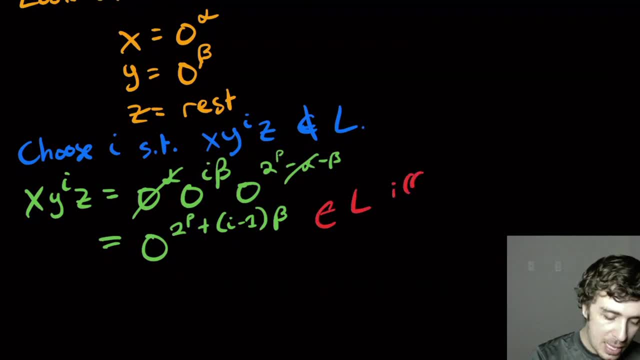 infer from this is that this thing is in L if, and only if, that exponent is a perfect square. so 2 P plus I minus 1 times beta. it not a perfect square is a power of 2. I should say power okay. so let's see. so what we can do is to think: well, if we, if we say I equal to 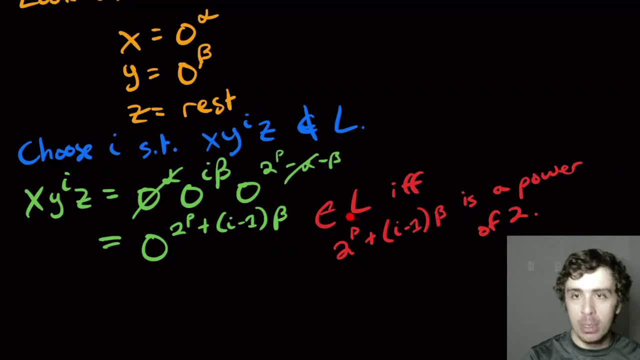 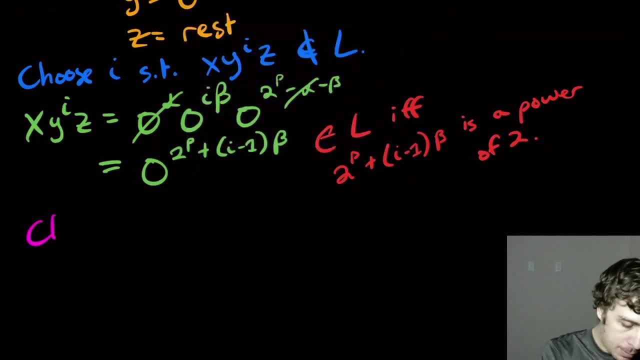 1, then this thing would be 0, and so 2 to the P plus 0 is to the P, which is a power of 2. so what if we said I equal to 2 as an example? so let's choose, let's choose: I equal to 2. 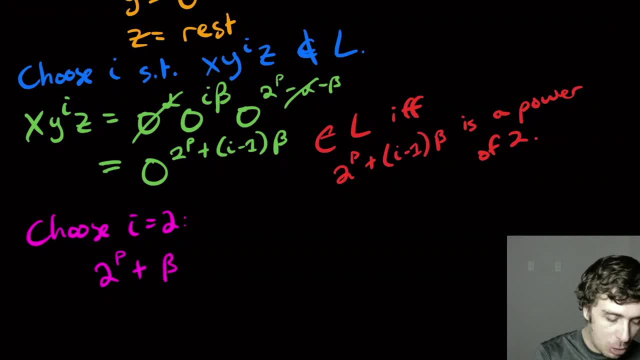 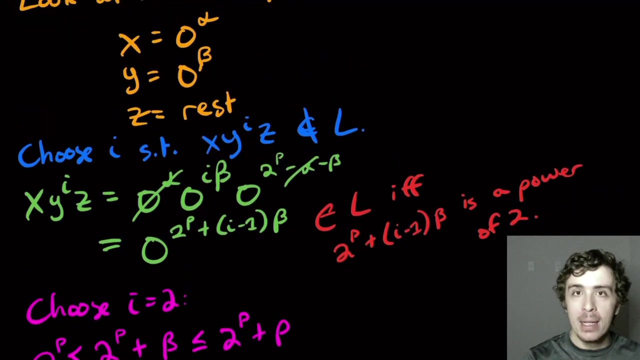 that that is two to the p plus a single beta. well, we know that beta is at least one, so this is strictly larger than two to the p because beta is at least one, and it's at most two to the power p plus a single p because the beta is at most p. and how do we know that? because the x, y pieces. 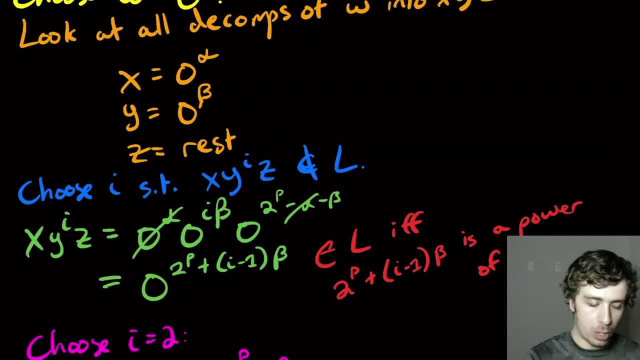 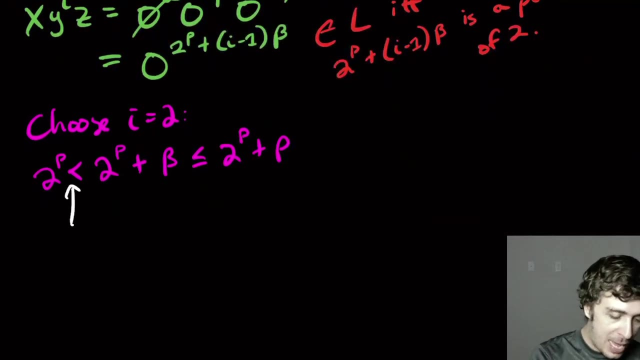 together are of length at most p in total, and what we're asking is: what is the length of y by itself? and that is at most p. so that's what we get here. so let me actually write where all this comes from, so that inequality comes from the fact that beta is at least one that one comes from. 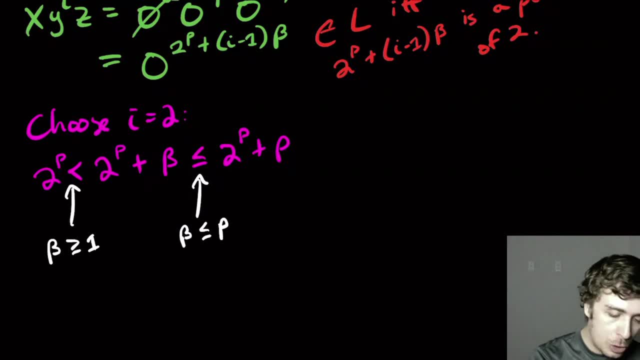 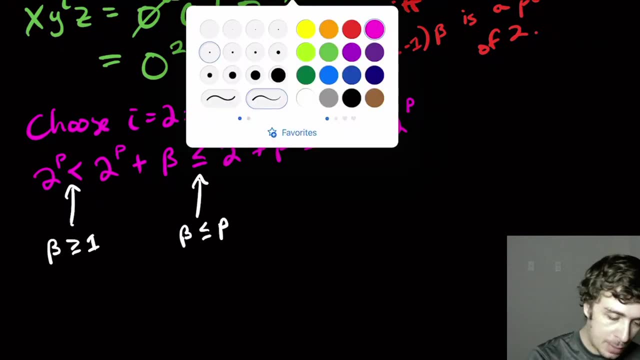 the fact that beta is at most p, and i'm going to do one more inequality, which is that this is at most p, and that one comes from the fact that beta is at most p. and i'm going to do one more inequality, which is at most two to the p plus two to the p, and we know that is true because p is. 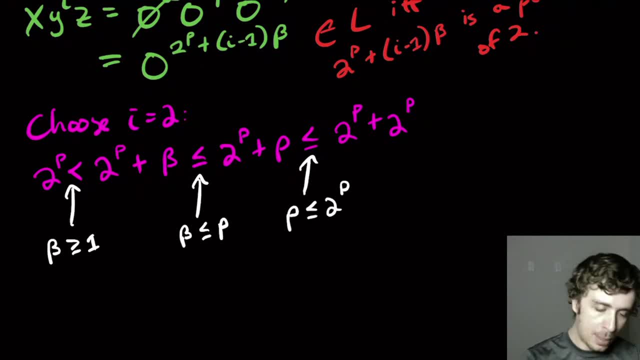 always less than two to the p. okay, and what we know over here is that this is two to the p plus one, because that's just that's just what the definition of perfect squares, the powers of two, are. so here, uh, what we can actually infer is that two to the p plus beta could be equal to this one. 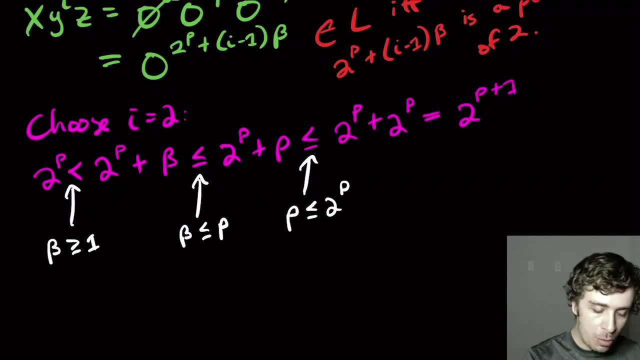 except what we're going to do is we know that it's not just a single uh, less than or equal to it is a strict inequality. it's strictly less than two to the p, and if it wasn't, we can just pick a higher value of p if it wasn't large enough. but it always is so there's no issue here. so it's not. 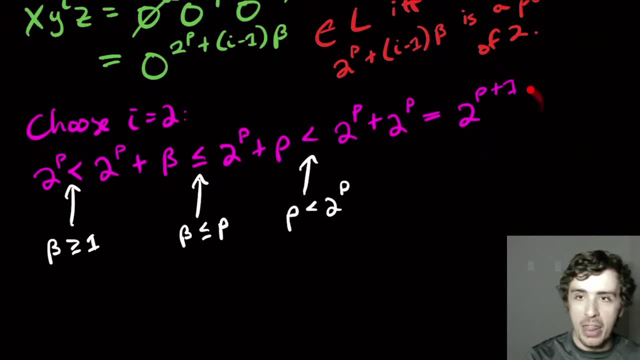 equal to this power of two. it's not equal to that power of two and these two are consecutive powers of two, so it's kind of like a two to the p plus one, but it's not equal to that power of two and it's kind of like the perfect squares proof, except now we have a slightly different uh thing that we 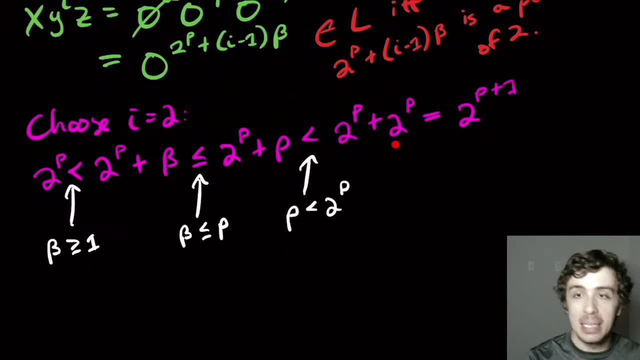 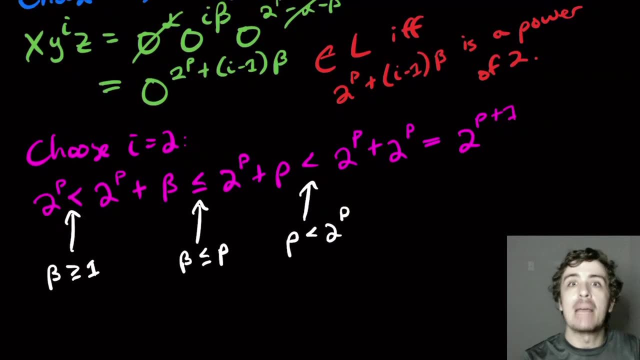 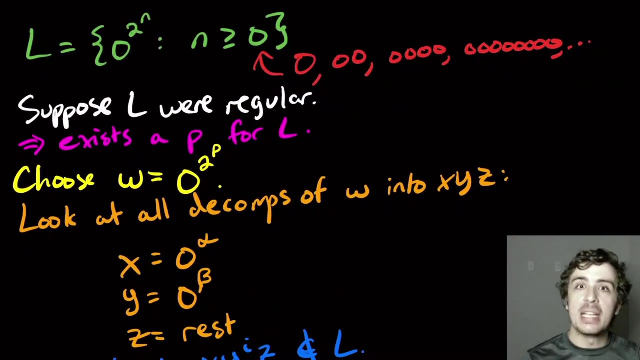 need to check right here, which is that p is strictly less than two to the p, and so, since it's strictly between two consecutive powers of two, it can't be equal to either one of them, and so it itself is not a power of two, implying that this language of perfect powers of two is not a. 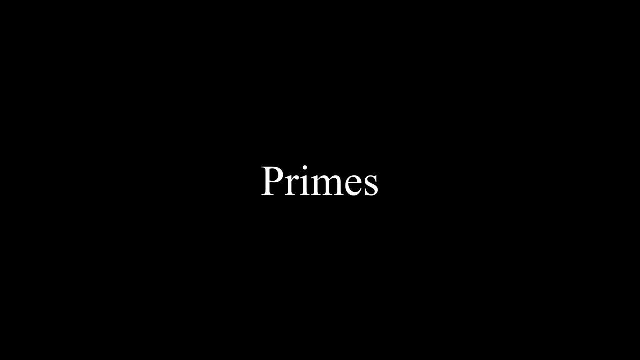 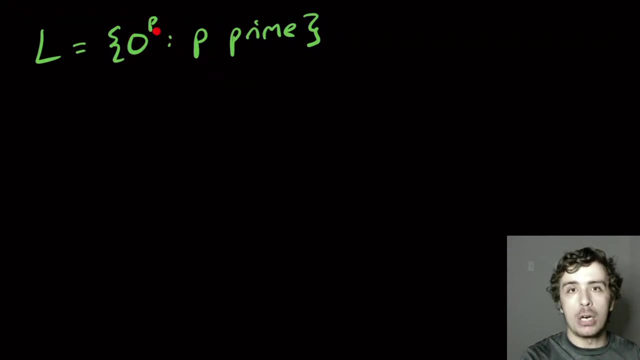 regular language. okay, so i want to prove that the language of all strings of zeros which are of prime length is not a regular language. so this is actually one of the more complicated- uh, pumping lemma in the sense of traditional pumping lemma- proofs. but we're going to get through it, so we 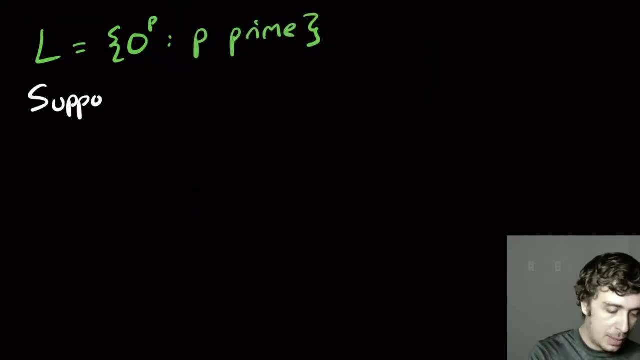 always start off every pumping lemma proof by supposing that l were regular. then we know that there exists a pumping constant p for for l, so that implies there exists a p for l. i'm just shorthanding it here, and what we need to do is we need to pick a string that's in the 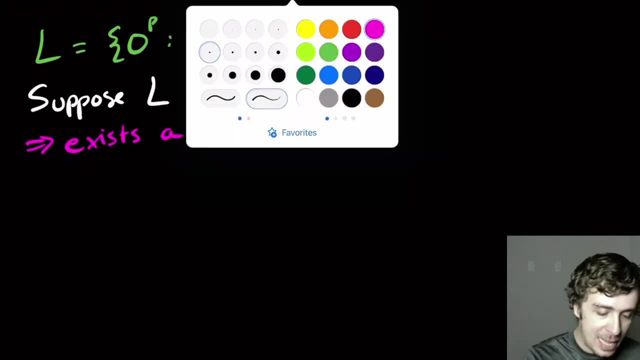 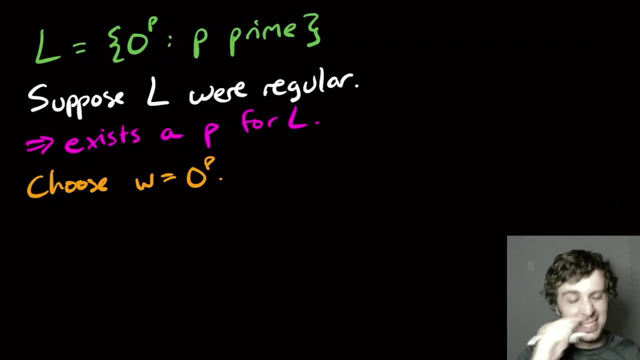 language and long enough, meaning that it has length at least p. so let's choose w equal to zero to the p. it's clearly of length at least p and the the p's match up. so therefore it's in the language, except it might not. so this p. 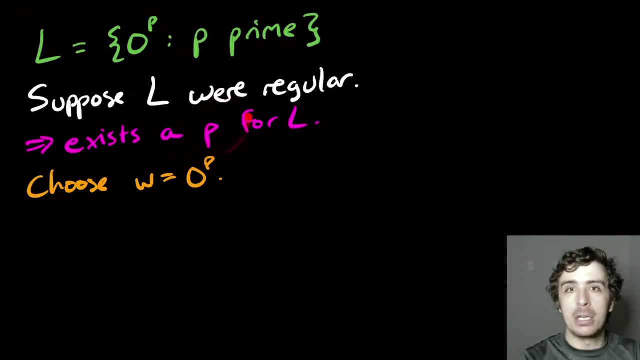 can be any imager. we don't know necessarily whether it's prime or anything, so we don't know whether this thing is a prime length, which is kind of crummy. so the way to get around this is use the fact that there are infinitely many primes. so whatever this oops, whatever this number. 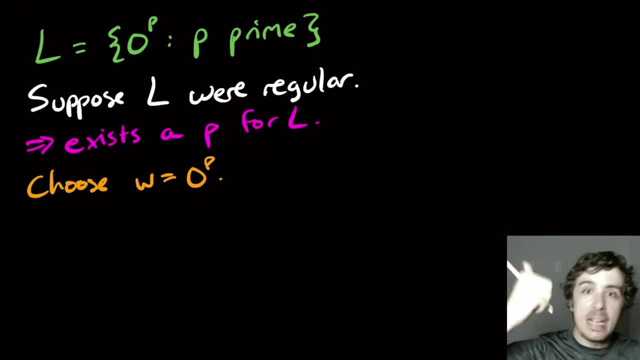 is: there's always a prime length and there's always a prime length, and there's always a prime length larger than it. in fact, there are infinitely many primes larger than it, although that's not as important. so what i'm going to do here is: i'm not going to do this. i'm going to do this in the way. 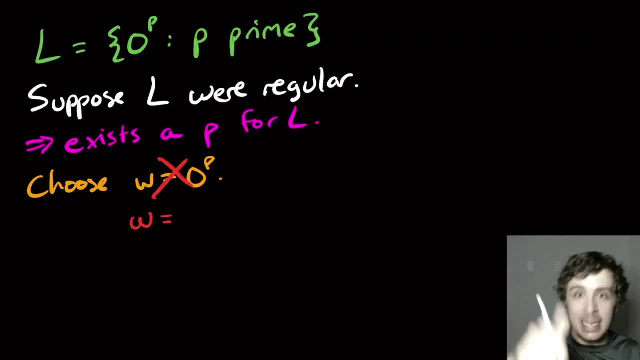 here's how i'm going to write it. so i'm going to pick the next next prime above p. so i'm going to pick zero to the r, where r is the next prime after p. okay, i'm actually not going to do that either, uh, and we'll see why. so i'm going to actually do. 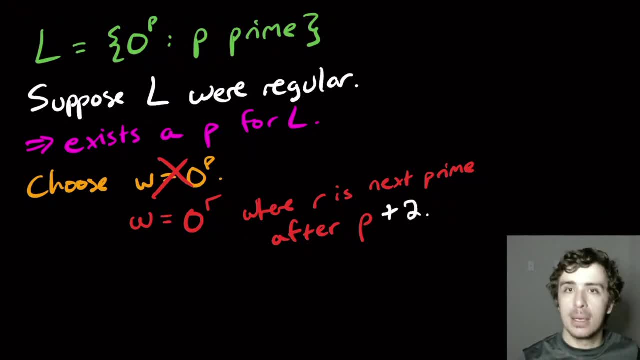 after p plus two. okay, well, there's always a prime, at least p plus two. so that doesn't. that doesn't change anything, and since it's more than p, therefore this is of length at least p, and it's in the language because we forced it to be a prime, and so therefore that's not an issue. so you may. 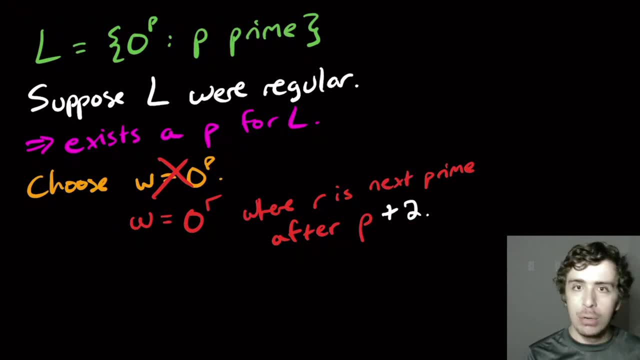 think: okay, i'm going to do this and i'm going to do this, and i'm going to do this, and i'm going to why there's, why is there a plus two here? so it goes back to the definition of what a prime is. so a prime, remember, is a number where the only way to divide it into it is either itself or one. 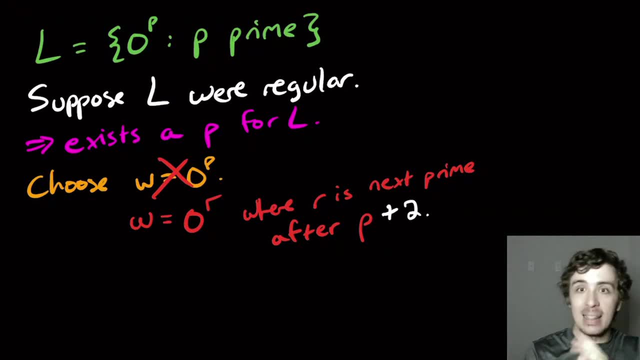 there's no things that are um at least two that multiply into p. okay, so where does this plus two come from? it comes from we need to be able to exhibit two things that multiply to the length of the string's length, and the way to do that is to try to break up the string in a nice 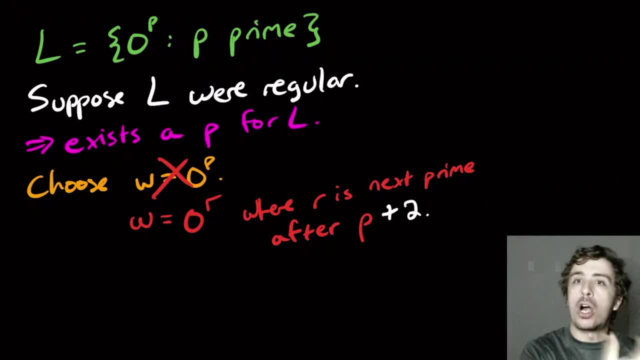 way, so that we have two things that are of both length, at least two- and multiply. so, therefore, the length of the string is not prime. why do we want a string that's not a prime? because we want to get a string that's not in this language, because we start off with a string that's in the language. 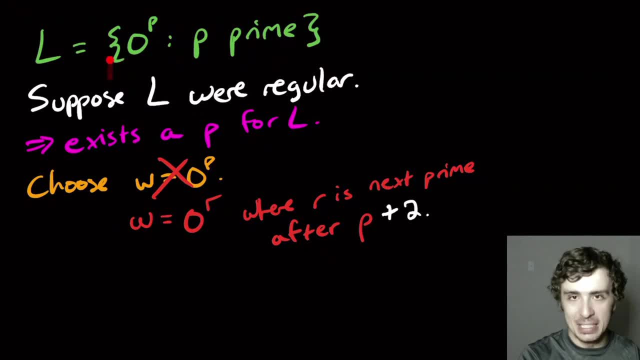 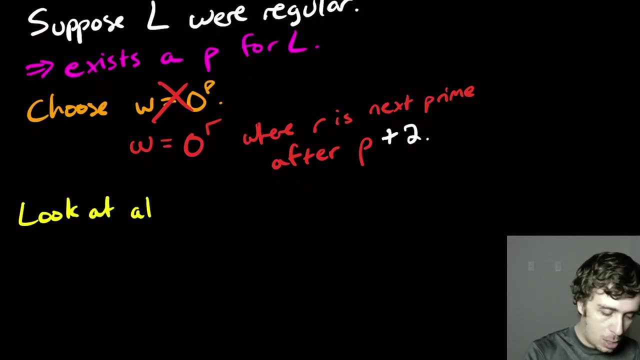 and we want to end up with a string that is not in this language. okay, so we need to look at all decompositions, look at all decoms of this string: w into x, y and z. according to the rules. well, the, the whole string is zero, so it. 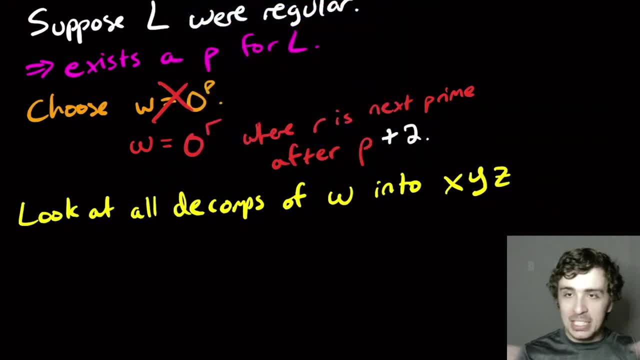 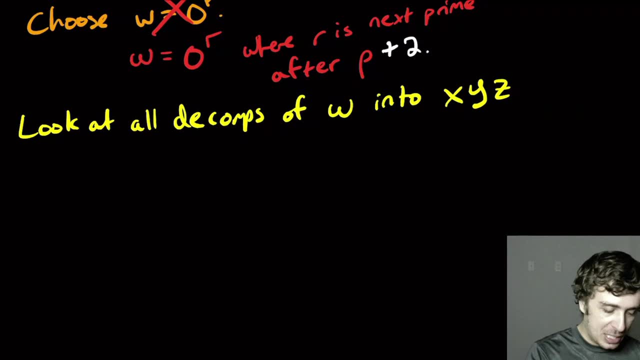 doesn't matter, and i'm not going to actually exhibit the, the three pieces, because it's just not going to matter. um, so, um, let's see. so what, eventually, what we need to do is we need to choose an, a value. i such that x, y to the. 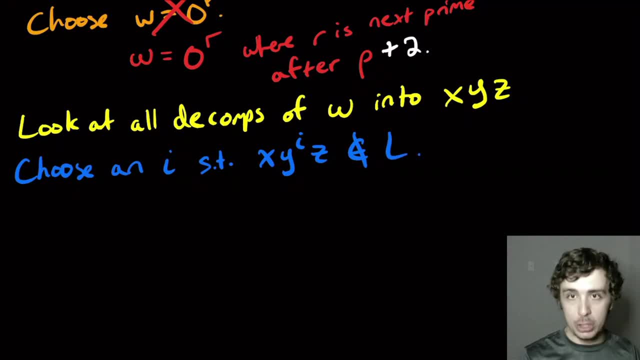 i z is not in the language. okay. well, we don't know what this is, so we don't know what this length is, but we eventually need to exhibit an i, for which it leaves the language. so, since the string is only zeros. so the only thing that really matters here is the length of the string, not the length of the string. 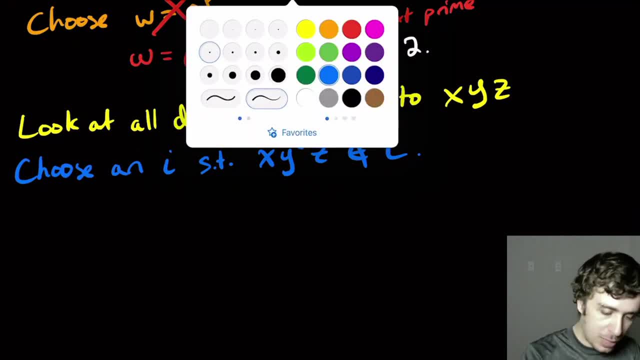 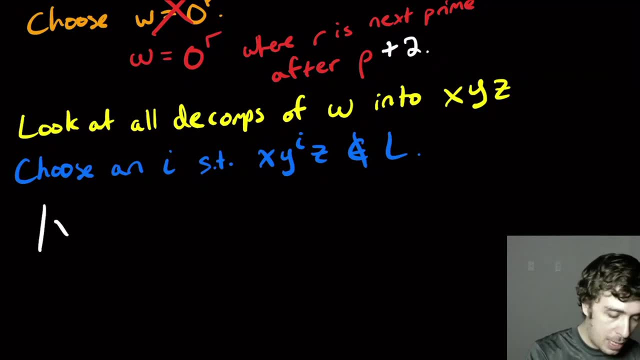 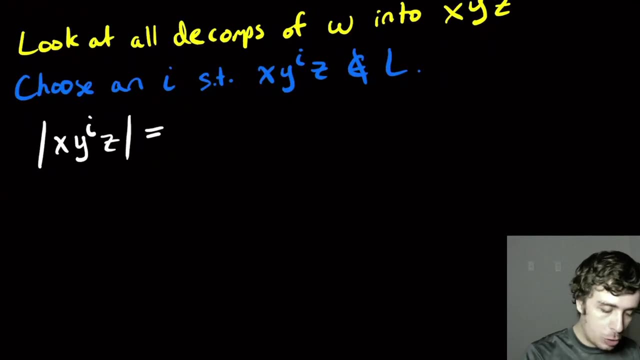 the string itself, because it's just all zeros. so let's try to look at that length. oops. so i want to look at the length of, not w. i want to look at the length of x, y to the i, z, whatever it is. well, this is equal to the length of x, z, oops, x z plus i times the length of y. 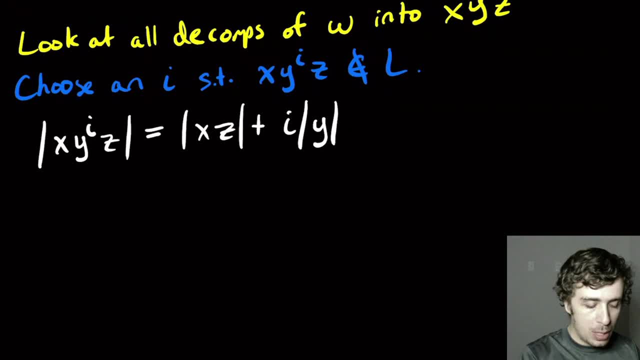 so why is this true? because i have a single copy of x on the right side, a single copy of z over here and y to the i. that's just i copies of y. so that's just i times the length of a single instance of y. so it is literally the same string because it's all zeros, but i'm only considering the length. 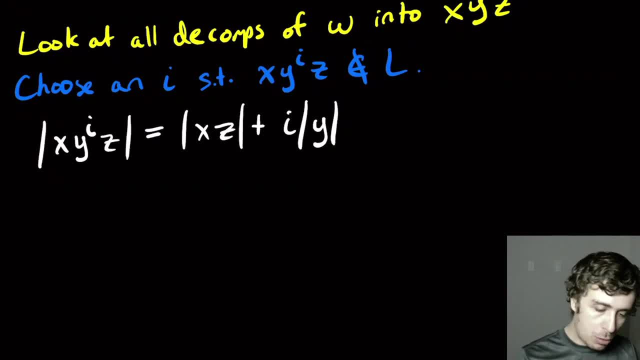 of the string. okay. so what can we infer from this? well, we know, based on the length of the string, the pumping lemma conditions that this thing is at least one. we know that the length of y is at least one, okay, uh, how do we get from at least one to at least two? because we need two things that are: 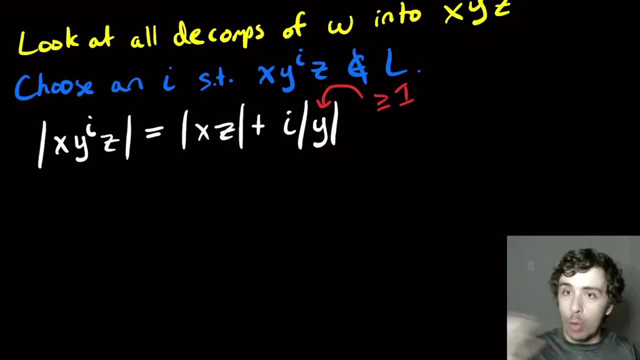 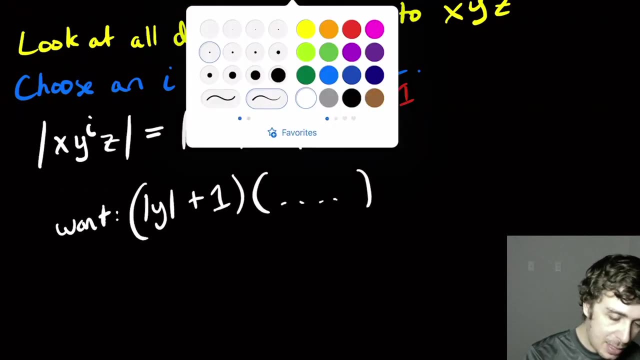 both, at least two, to multiply into the number, well, we add one to it. so what we want, so, uh, so what we want is the length of y plus one times something, and we want that thing to be also at least two. we know that thing to be at least two. 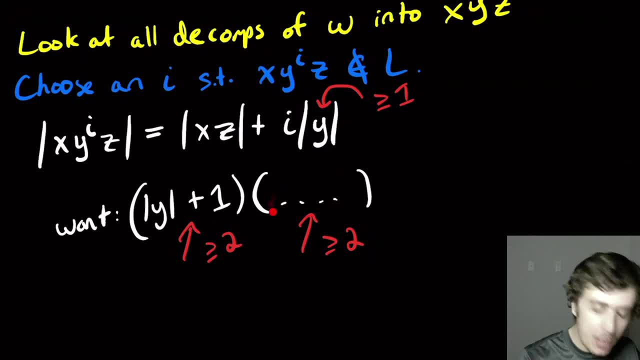 because we forced it to be. but we need something in here that is also length, at least two, and that's where the plus two from before comes into play, because it turns out that we can sub into here the length of x, z, which comes from from this. and why can we do that? 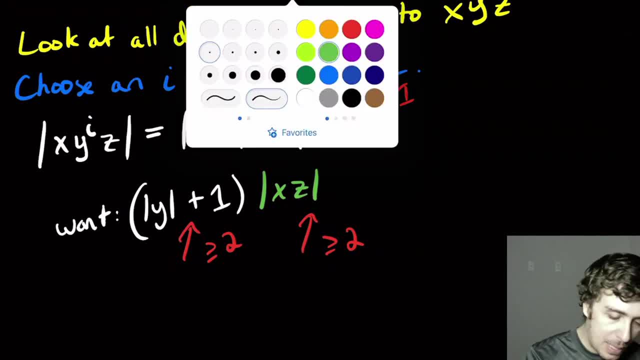 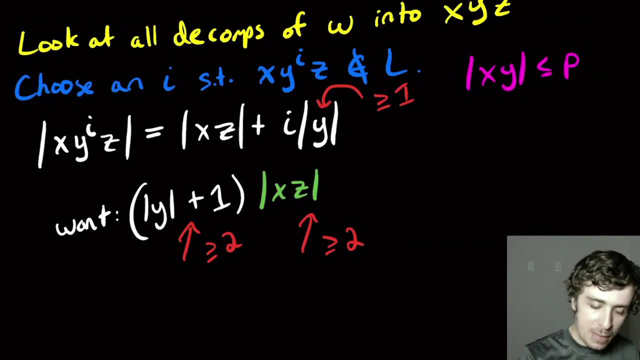 well, let's see, we know that the pumping lemma condition says that the length of x, y is at most p. so the length of w then, which we constructed earlier, is at least p plus two, because we did that little plus two thing, and p might itself be a prime in the absolute worst case, but even in that, 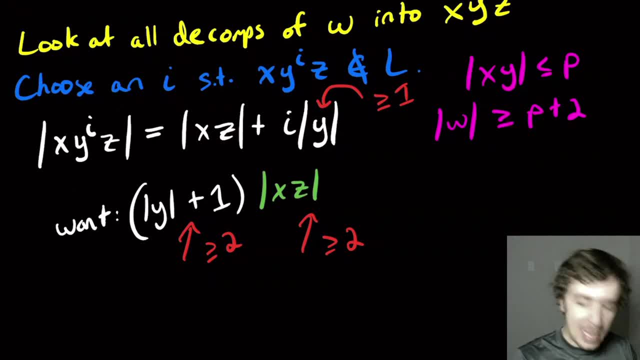 worst case is at least two more, so that implies that the length of z itself is at least two. we know that to be true because even if x, y took all p characters at the beginning, there's still two more left, and z is the only thing left in the string to. 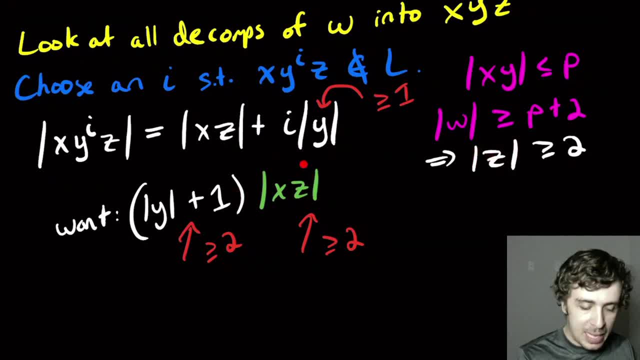 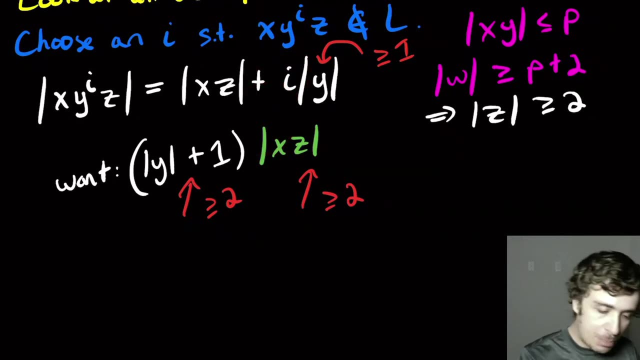 take any characters, and so the length of z itself is at least two, and x may be empty, maybe not, but it doesn't matter, it's at least two. so, uh, but how can we get from the length of z to the length of this line? to this line, it's by subbing that value of i, so the value of i that we're going to pick. 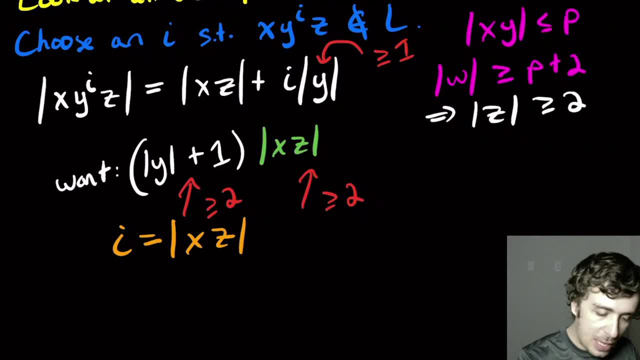 is the length of x z and if you actually check, that actually works out. because if we actually compute this, so this is x z it's length plus the length of x z times the length of y. and since we got an x z in both cases, i'm just going to factor it out and we're going to get 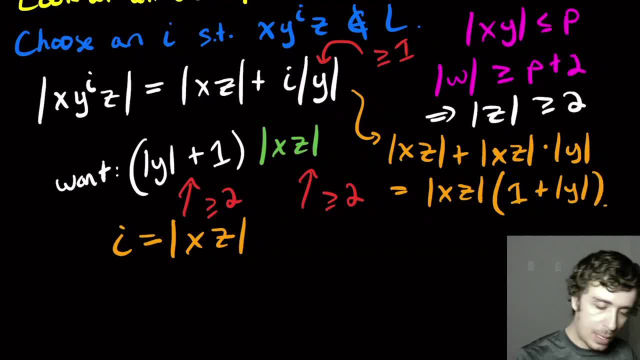 exactly the same expression that we had before. okay, so this is a interesting example of the pumping lemma, in that the value of i that you pick depends on the decomposition. but that's okay, as long as you find some value of i for which you get out of the language, and we did. 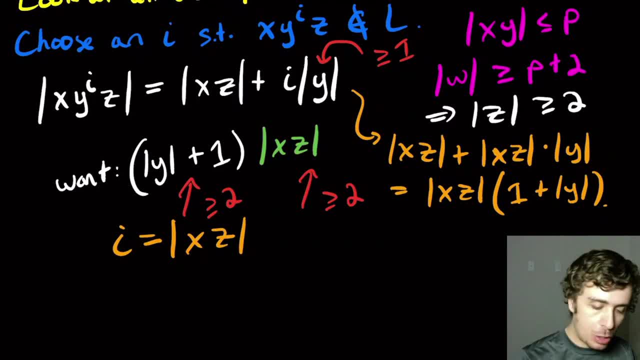 that's all that's needed. so we found the value of i. we constructed something that is some number that's at least two times another number, also at least two. so whatever that number is, which is the length of that string, has to be composite. it's not prime, and so therefore this string is not in. 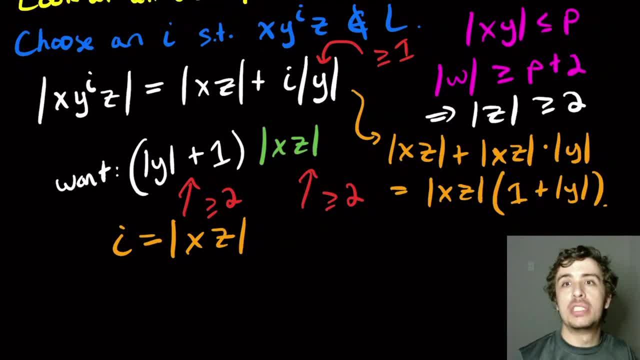 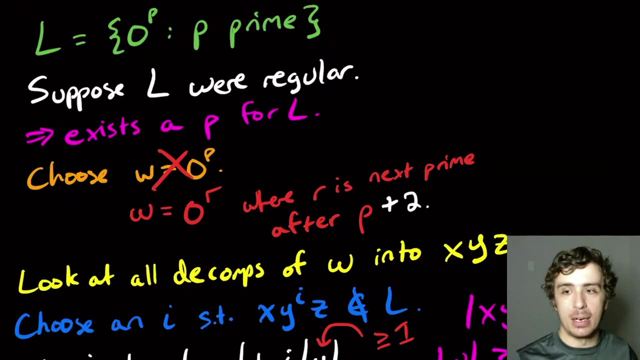 the language and because of that, that shows that the language is not regular, because if it were, it would always be a prime, but we found an example of where it is not a prime. so that's how you show that the language of primes is not regular. all right, we should be able to convert this into a primes. 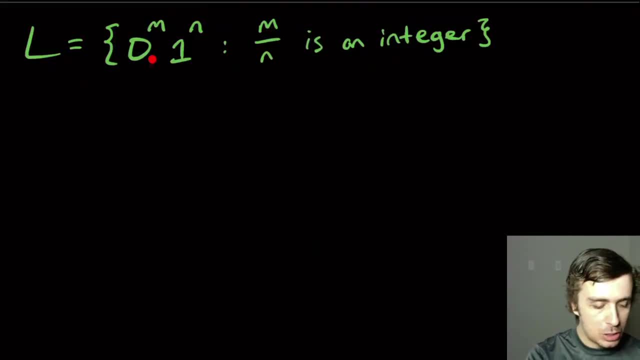 all right. so we have to prove that this language, which is all the strings of the form, zero to the m, one to the n, where m over n is an integer. so here this is just saying that the number of zeros is a multiple of the number of ones. so, as an example, if we have, let's say, six zeros, 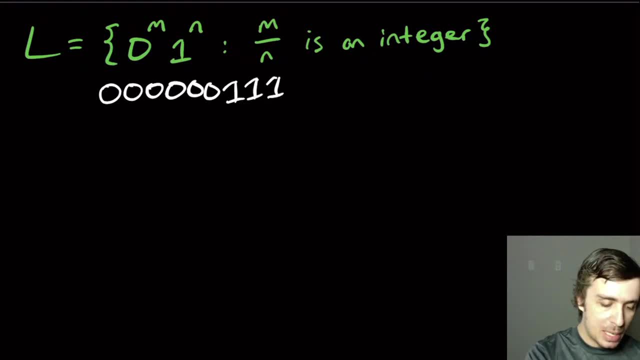 then i can say that the number of zeros is a multiple of the number of ones. so, as an example, have three ones, because six over three is two, so that's an integer. but if I struck one of those zeros out, then this thing would not, that string would not be. 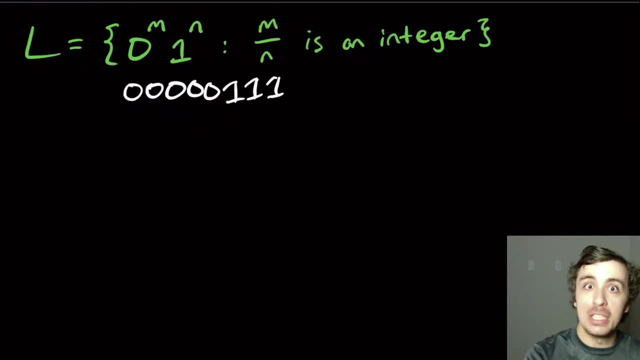 in out, because five over three is not an integer, and I want to show that this thing is not regular, so let's suppose that it is. so suppose that L were regular, then that means that there's a pumping constant P for L. so let's go ahead with that. so there exists a P for L, and again I'm shorthanding this, okay. 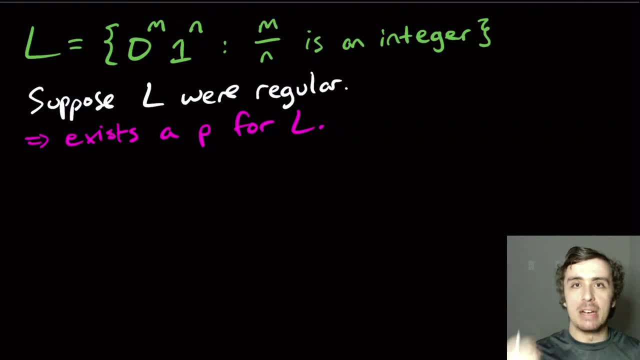 so then, now we got to pick a string that's in the language and of length at least P. so- and we also have to, of course, we need to have the number of zeros divided by the number of ones, being an integer, in other words, the number of zeros is a multiple of the number of ones. so let's. 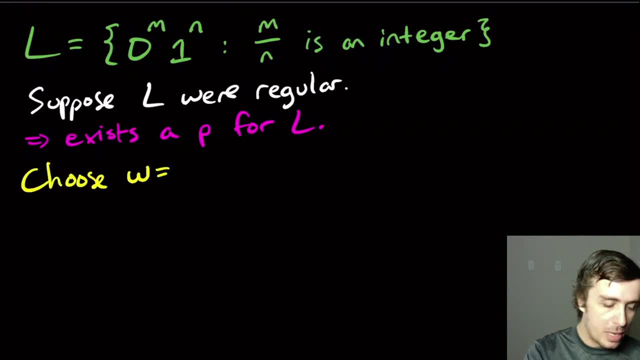 go ahead and choose a string, and this string will not be useful for us, but I just want to show it anyway to give you the idea. so here let's pick it. look at this string: so we definitely have at least P characters, because there are three P characters here and this thing is in L, because 2 P divided by P is 2. 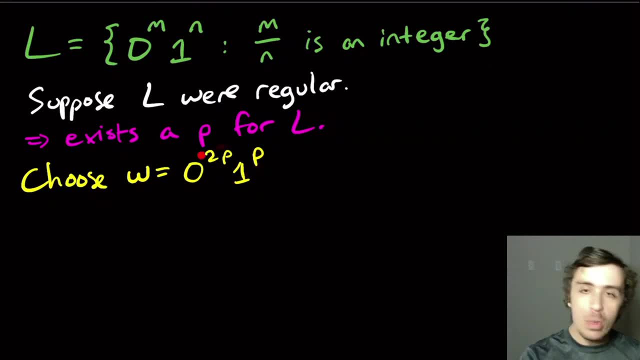 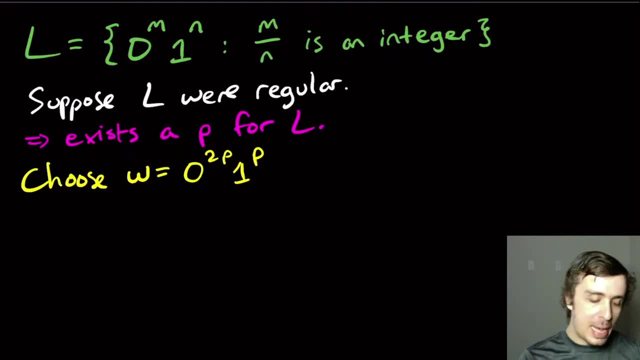 string that is not in L. so in other words, the number of zeros is not a multiple of the number of ones. but in order to do that we have to pump into the zero part, because that's one of the conditions of the pumping lemma. so if I 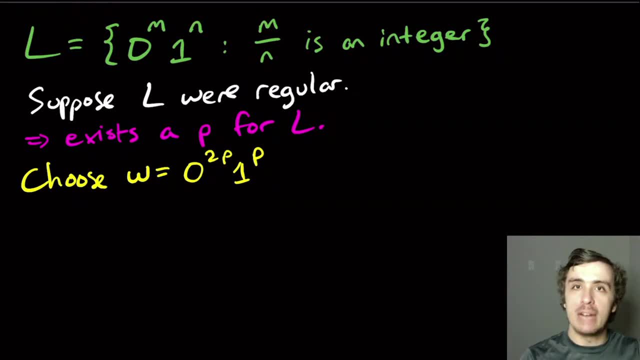 might be that we increase it by p zeros every single time and that is a valid decomposition of the of the string according to the rules. so it could be that we we could have any number times p over here and p over here, and we'll never escape the language there, because um m over n is. 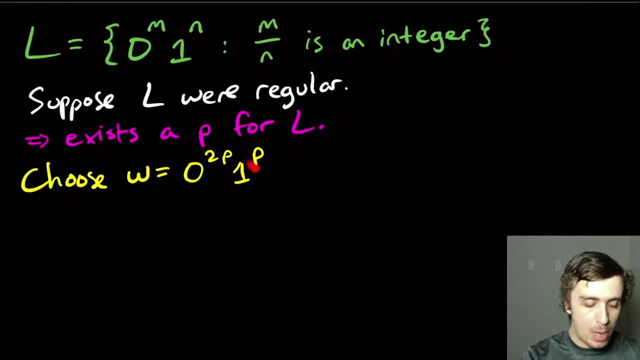 not an integer. it is always an integer there because we have one p over here and some integer times p over here. if you pump downward, you may think, okay, that's fine, because we're going down here and it's not twice as much. it could be that we take away p characters here and so we'll have 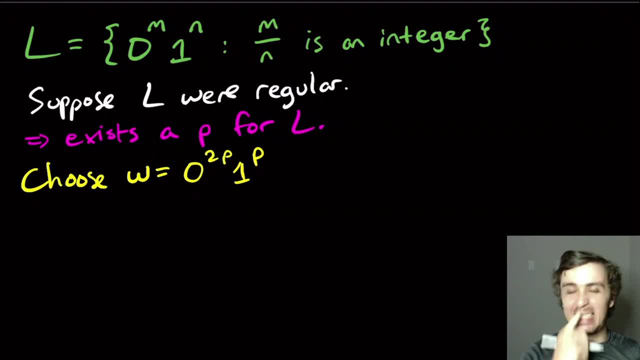 zero to the p, one to the p, and uh, that will not help us very much. so, uh, there are actually two routes we can go. so one route is we can just pick zero to the p, one to the p and then pump down, uh. but the problem is that, um, uh, if we tried to, let's, let's just say we tried to do that, um. 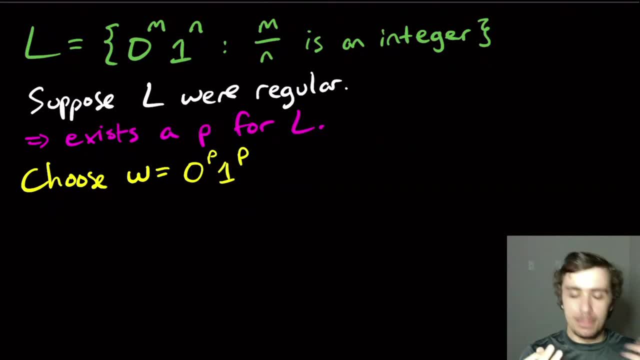 then what would happen is what if we had the decomposition where we took away p characters, so the the x and y bit the first two parts, it occupied all of these zeros right here. then what would happen is that if we took away all p of those characters which we're 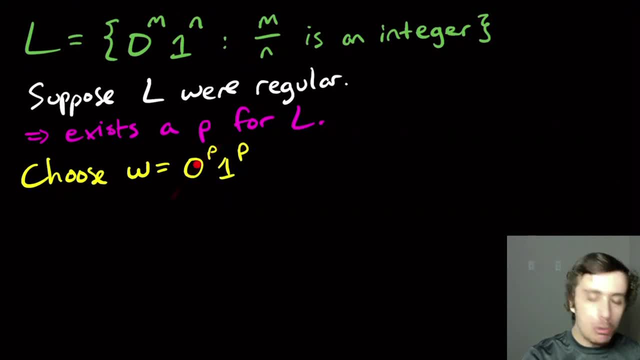 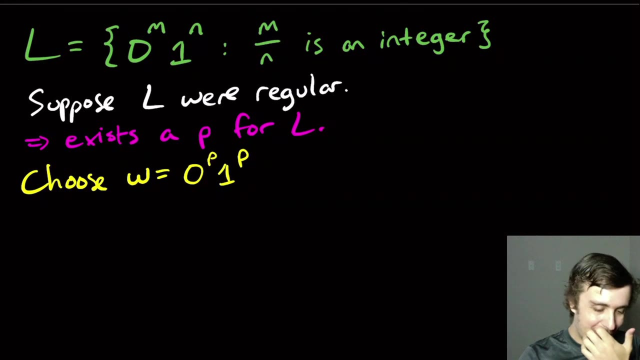 allowed to do when pumping down. it might be that we have zero zeros there, and so this fraction will be- is will be- zero, and that's not really allowed. uh oh, sorry, that is allowed according to the language, but it's not the conclusion we wanted. we wanted to have something that is not an integer, so this idea will not help us. however, 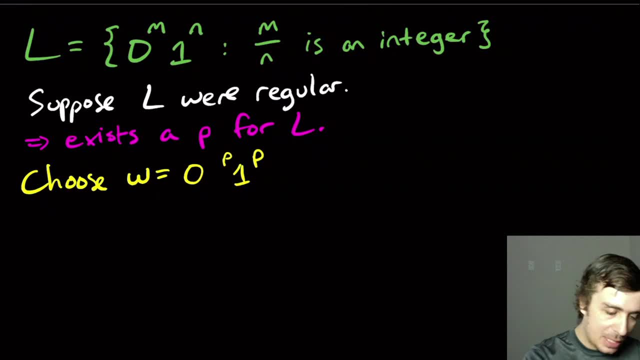 what if we did this? what if we said: okay, let's pick some other fraction, let's, we got to pick a fraction for which, um, it is an integer, when, uh, dividing here at the start, but we will end up in something that is not an integer. so let's pick. let's say, 3p here and 2p here. oh sorry, 4p, 4p, that's what i wanted. 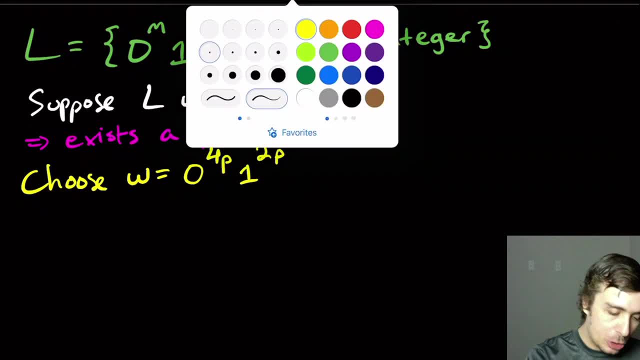 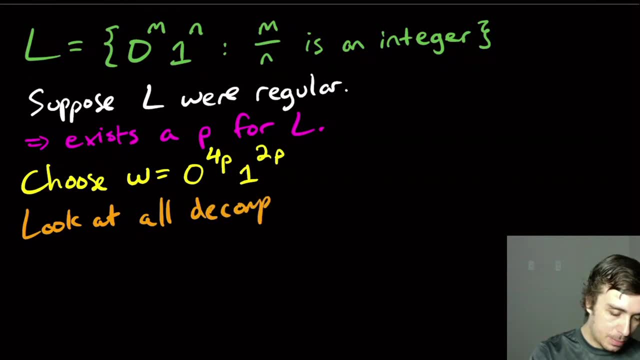 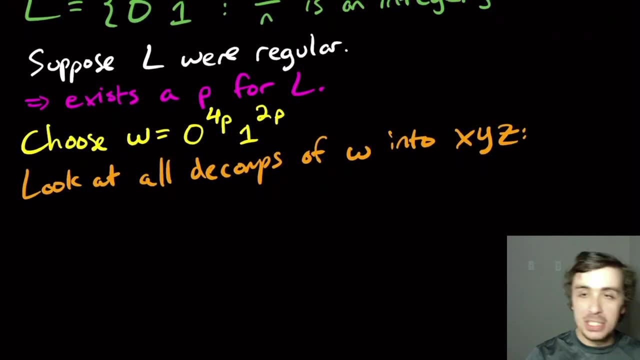 so then let's see, let's look at all decompositions now. so look at all decompositions of w into x, y and z. well, since x and y are at most p characters and the first p characters are all zeros, we know that the x and the y bit are some number of zeros. only let's call. 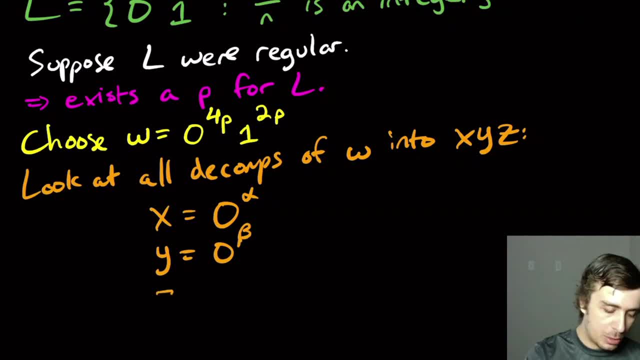 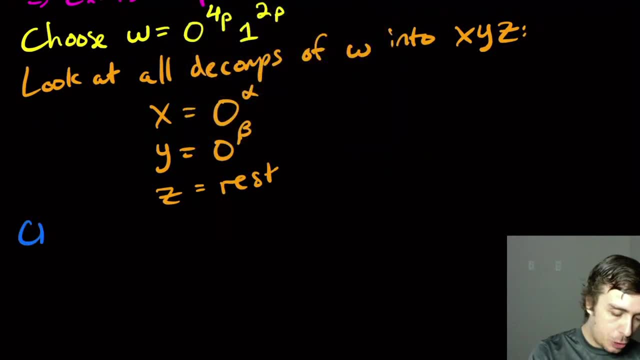 them alpha and beta, as the number of zeros and z is the rest, which i'm not going to bother writing down. so then we need to choose a number of zeros, and then we need to choose a number of zeros and i such that x, y to the i, z is not in l. okay, well, it's pretty clear. uh, well, actually. 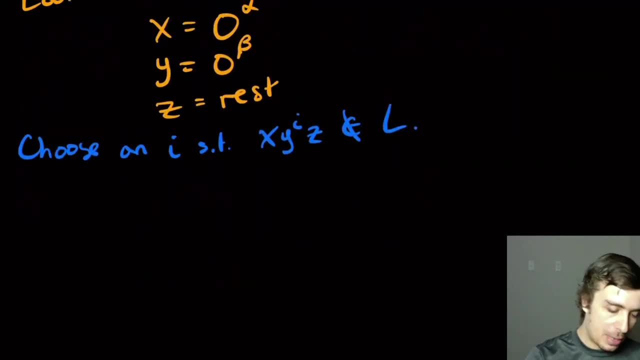 no, it's not so clear. so we gotta pick an i for which is not in the language. so let's actually look at this string: x, y to the i, z. so that's zero to the alpha, zero to the i beta, and i'm going to put down what z actually would have been. 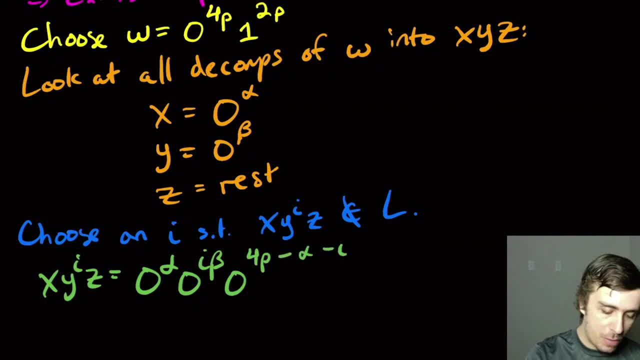 four p, because that's what we started with: minus alpha, minus i beta. uh, yeah, yeah, yeah, yeah, that's right, it's, it's, it's not i beta. sorry, it's four p minus alpha, minus beta, because that's what the y part had. i really should have done that. and then we have a one to the two p. 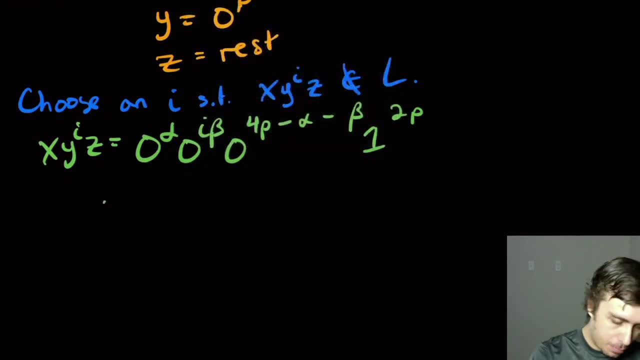 there. so then let's let's shrink down all of the zeros here so the alphas get killed off. so i'm going to have four p plus i, minus one times beta, because that's how many betas i have, and then one to the two p. so it's very obvious that this thing is in the language if, and only if. 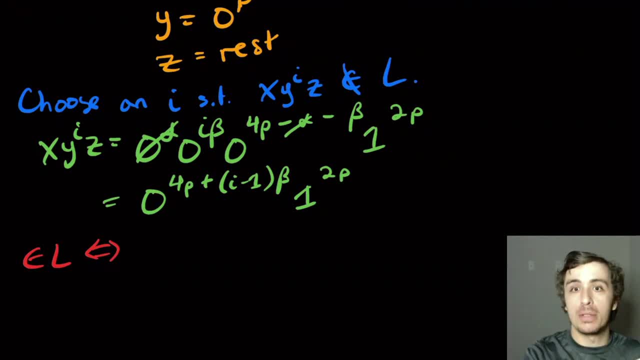 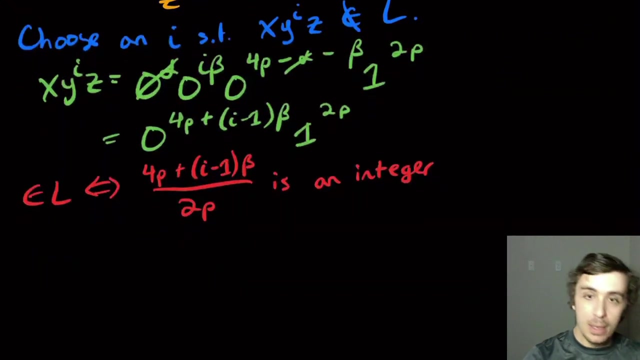 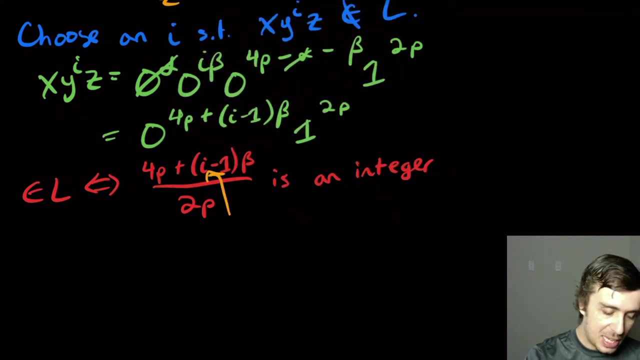 the. the number of zeros is a multiple of the number of ones. so four p plus i minus one times beta over two p is an integer. okay, that's the only way it could possibly be in there. so let's actually substitute a value in. so let's put in. let's say i equal to two. we can't put. 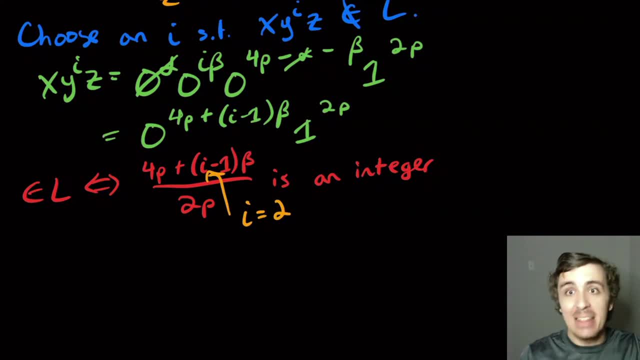 one, because that's what the original string was and that's in the language. so we can't prove it's not in the language. if we choose, i equal one, so let's look at i equal to two, so that's four p plus beta over two p. but if we look at this, we know from the pumping lemma: 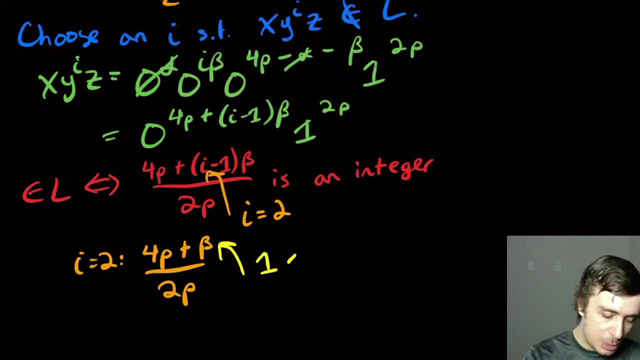 statement that beta itself is between one and p. so where this comes from the actual statement, the one of the things that we need that the part that we pump is not empty, and this part says that the first two pieces have length at most p in total, and so that's where this 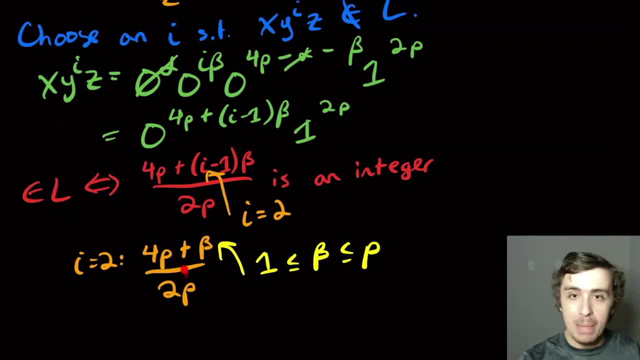 comes from. so here the only way that this could really be an integer is if p, if beta is equal to two p, because it can't be zero according to this, and so the next higher point would be two p for beta, because then this would reduce to three. if beta was zero, this is two and there's no. 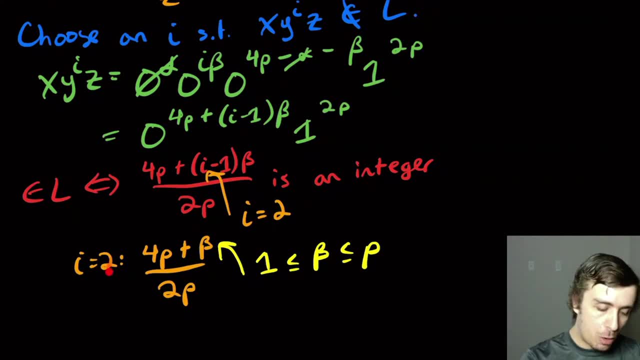 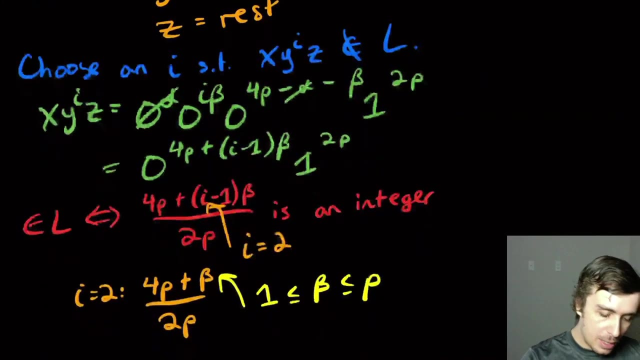 integer in between two and three. so therefore, if we pick i equal to two, no matter what beta is, this thing is not an integer and so therefore we are not in the language as a result of that. if you pump down, so if we like, chose i equal to zero, that also would work. we would have four p. 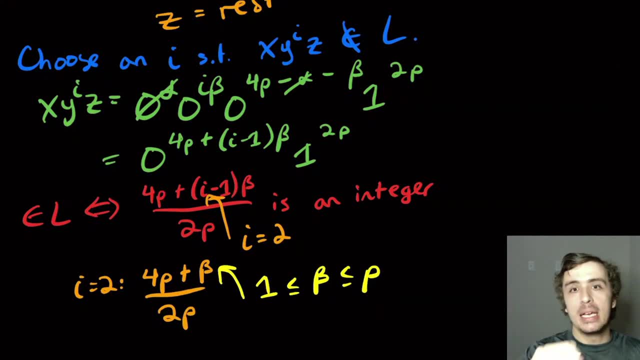 minus beta, and the only way that that could be an integer is if we had two p upstairs, which means that beta would also have to be two p, and if we did that, we would have to be two p, and that would, and that's just impossible according to this. 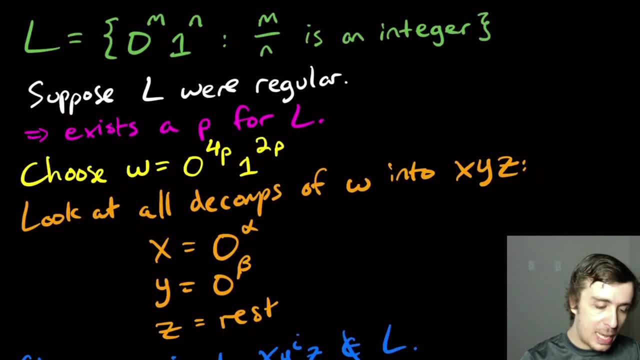 So that is a quick proof to show that this language is not regular. The key to understanding this is that you have to be able to think about whether or not the string makes sense. So the 2p 1 to the p example seemed reasonable. 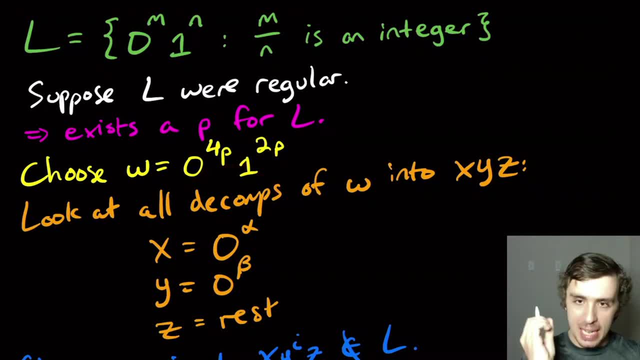 until you thought about: okay, all the decompositions, you gotta handle all of them, including the ones where the length of y is equal to p, and that's where the problem arose in that case. Here, the gaps between where the left side- 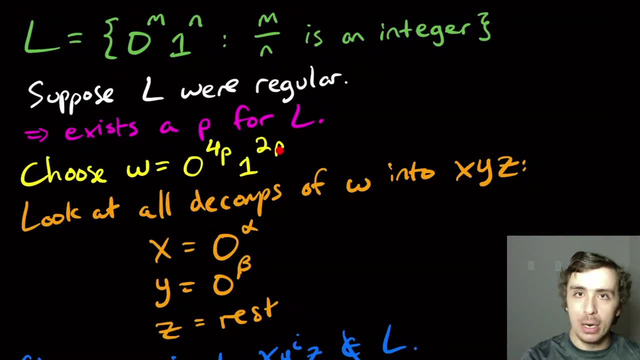 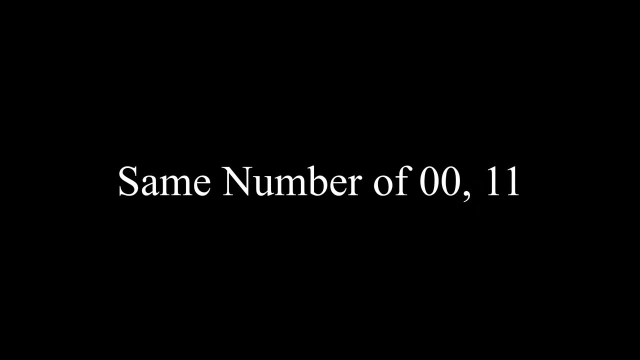 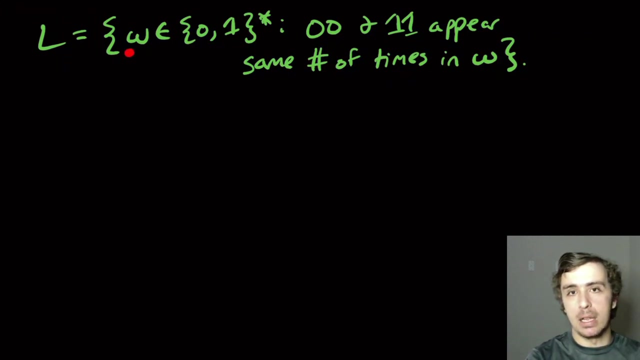 divided by the right one is an integer- are much wider, And so that's why this allows us to escape the language, whereas before they were short enough to allow us to stay within the language. So this language is not regular. All right, so let's prove that this language is not regular. 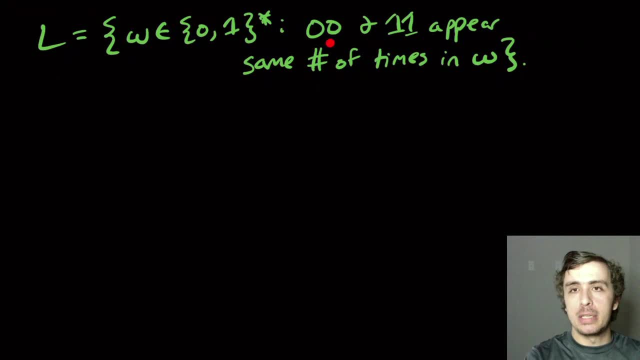 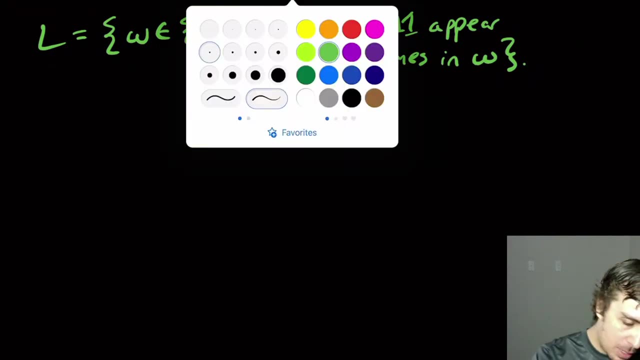 which is the set of all strings over zero one star, such that the number of zero zeros and one ones in w is the same. So, as an example, if we look at the string zero, zero, zero, one, one one. 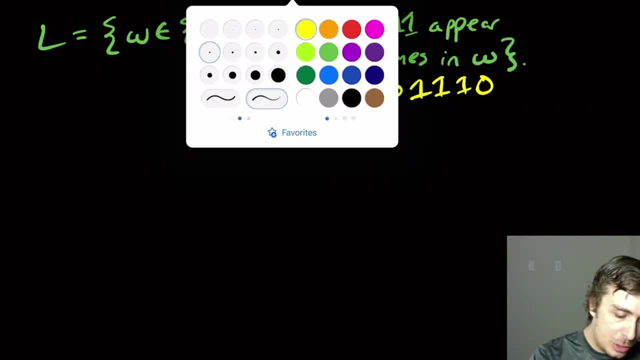 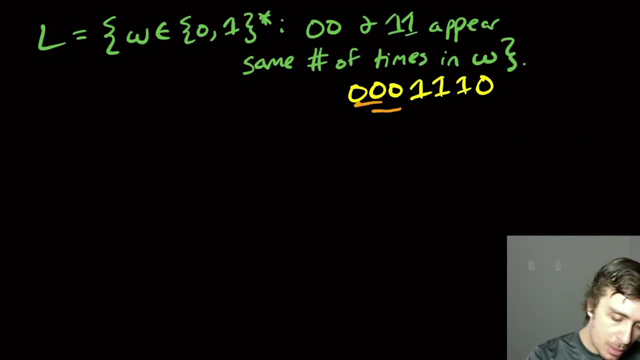 and maybe a zero at the end. So let's count the zero, zero occurrences. So there's one right there, there's one right there. They can be overlapping possibly. There's a one one there and a one one there. 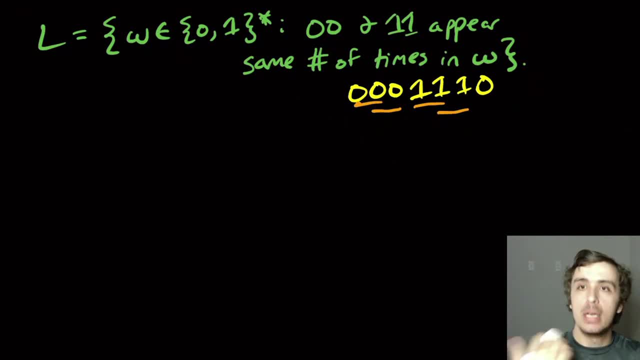 And so, since there are two occurrences of each, therefore, this string is in the language, And if we took off that zero on the end, that doesn't change anything. However, if we took off this one right here, then it's not in the language anymore. 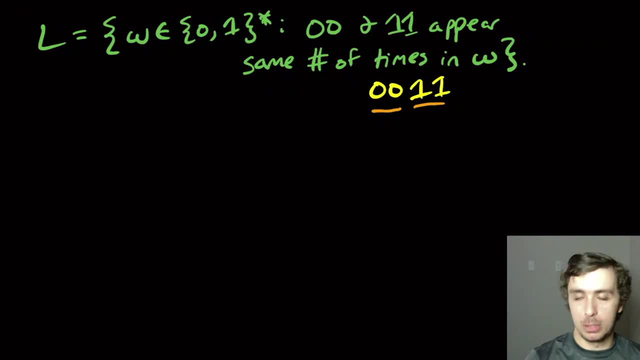 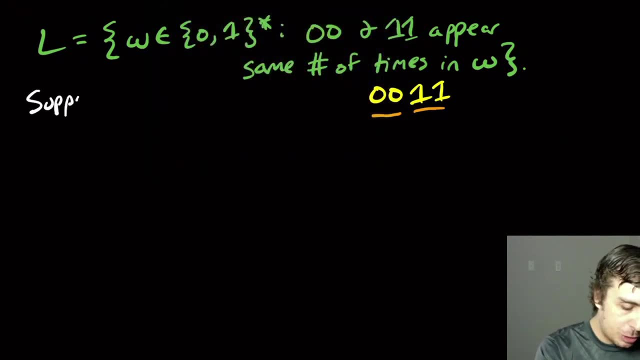 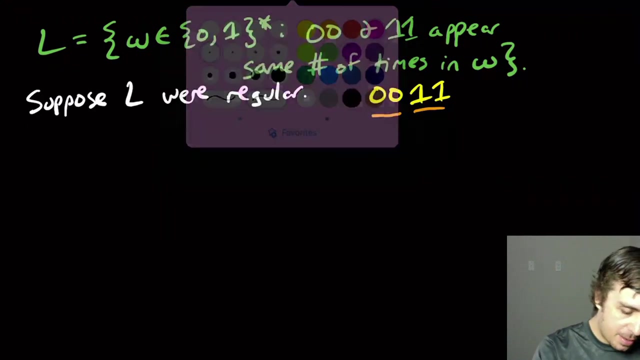 If we deleted the first zero, then it's back in the language. okay, So let's prove that this thing is not regular. So again, as always, we need to suppose that L were regular. Then that means that there exists a pumping constant P for L. 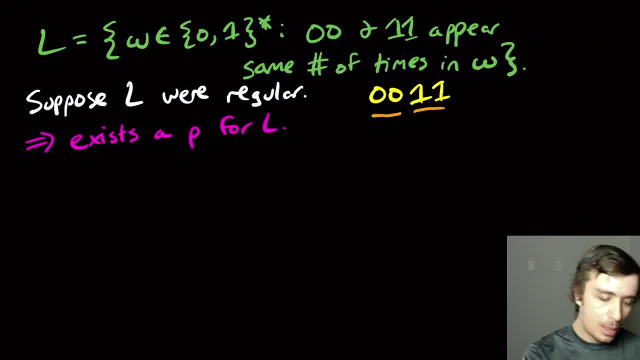 I'm just gonna abbreviate it, as exists a P, So we need to find a string that is in the language and has length at least P, So it has to have the same number of zero, zero occurrences as one one occurrences, And there's a lot of different strings. 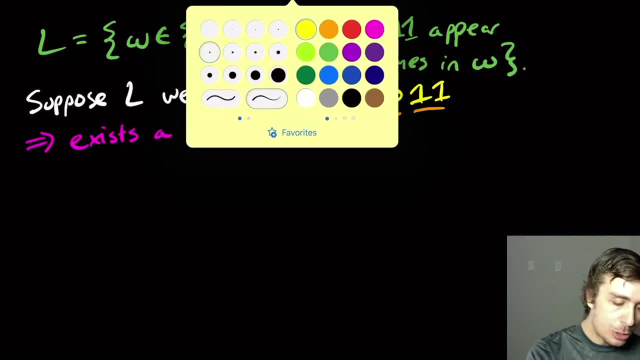 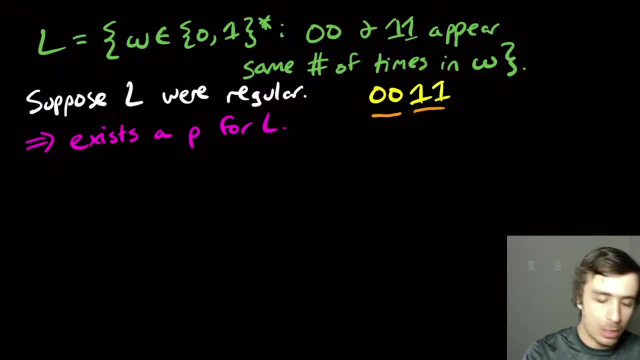 that you can actually pick. in this particular case, I'm just going to do a common use, a common one that is kind of similar to the example that we did a little earlier. So I'm gonna choose W to be equal to zero, to the P. 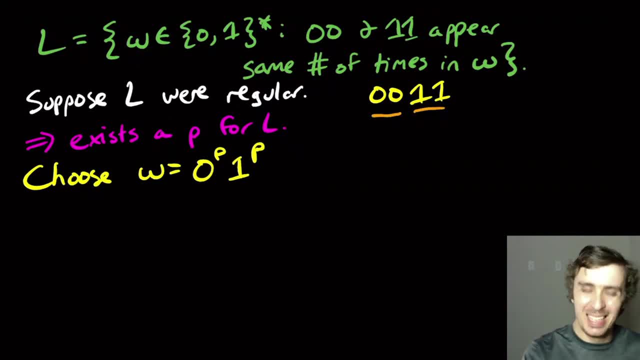 one to the P And you think, huh, there's no zero. zeros in there, Ryan, There's no one ones in there, All contrary. So let's think about what this string actually is. It's a whole bunch of zeros and then a whole bunch of ones. 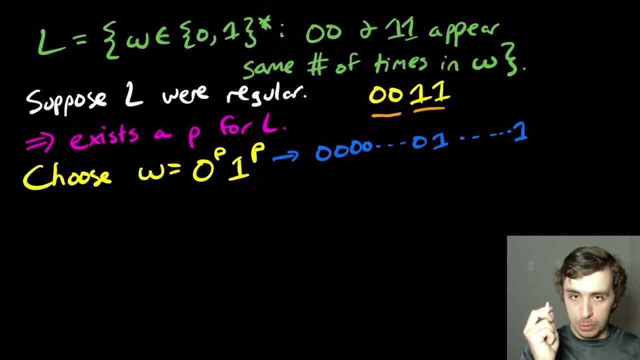 So let's think about where the zero, zero occurrences are. It's right there, right there, right there, And it's kind of like this staircase pattern that goes down and then the one ones occur in the same way. In fact, there are P minus one occurrences of zero, zero. 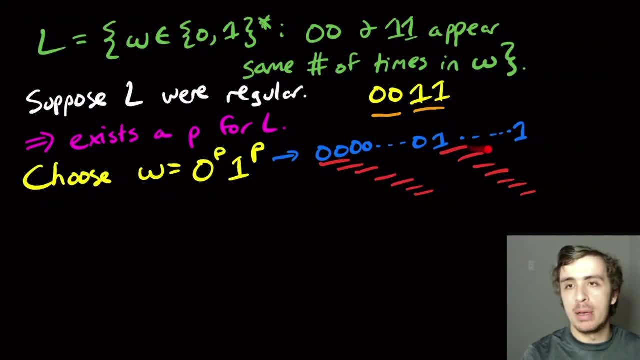 in there. try to think about why that is P minus one. occurrences of one, one in there for the same reason. All right, so then now we need to look at all decompositions. Look at all decompositions of W into X, Y and Z. 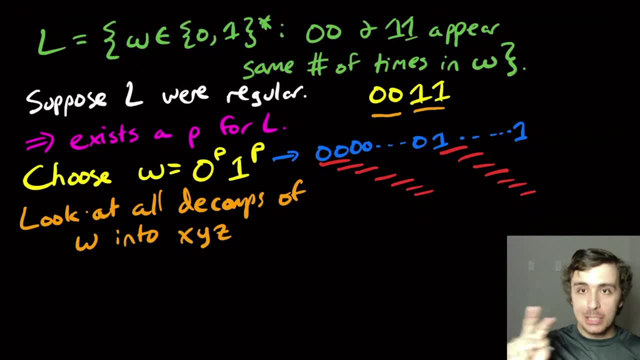 according to the three rules, Such that X, Y has length at most P and Y has at least one character in it. So since X and Y are the beginning of the string at most P characters, they must live entirely within the zeros. So I'm going to have X be some number of zeros. 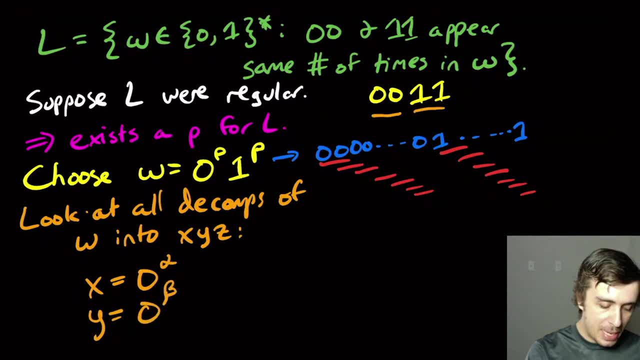 let's say alpha of them, Y is zero to the beta, some number of zeros, And let's say Z is zero to the P minus alpha, minus beta, because that's the number of zeros left, And then one to the P at the end. 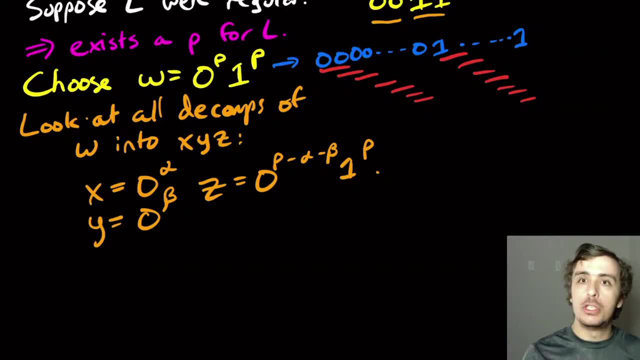 So now we need to choose an I for which the number of zeros- zeros and ones- are One one's is different, And so, more precisely, we need to choose an I such that X, Y to the I, Z is not in L. 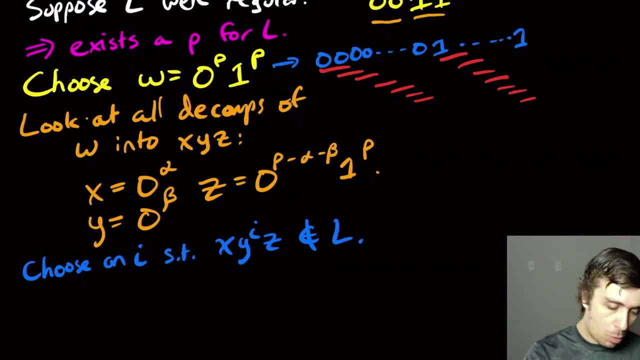 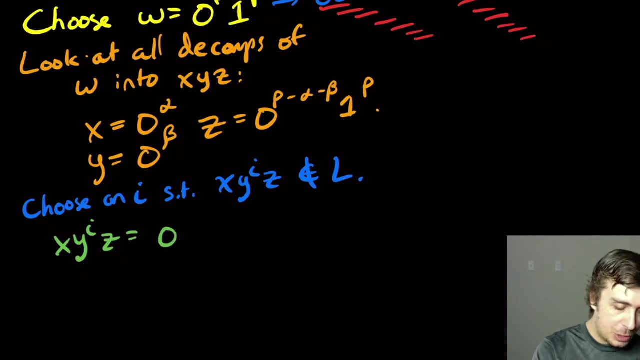 So it's not in L. Okay, well, what is this? If you actually compute it, it's going to be this string: It's going to be zero to the P plus I minus one times beta And then one to the P. 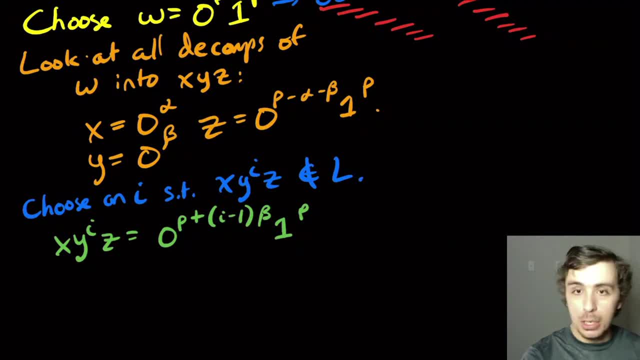 So here, because we have the alphas get killed off, we have I beta right here because that's how many choices of Y we have, And then we have a minus one beta from this. So that's where the I minus one comes from. 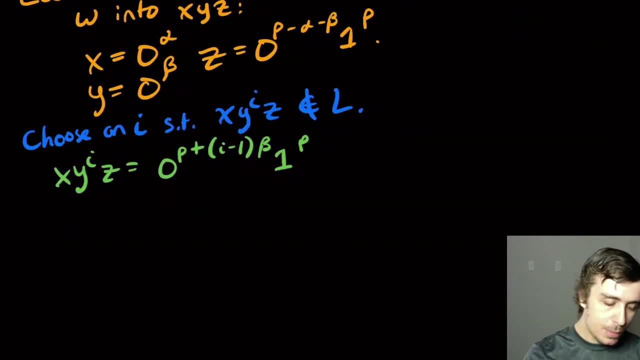 So this thing is in L if, and only if, the number of zero zeros is equal to the number of one ones. So that's where the I minus one comes from. So this thing is in L if, and only if, the number of zero. 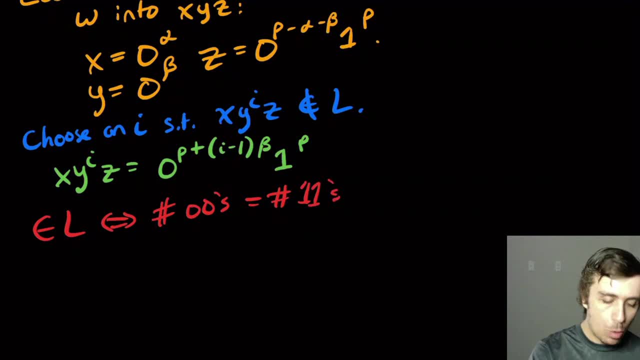 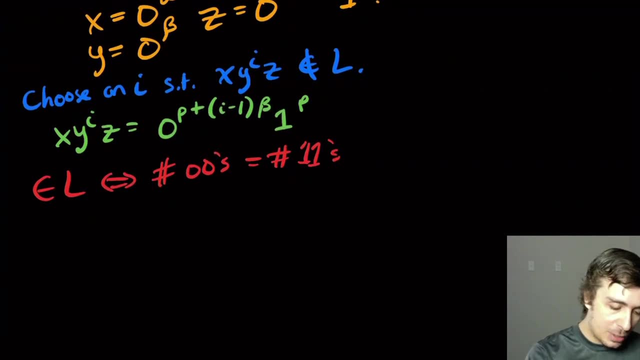 zeros is equal to the number of one ones, And we want to show that the numbers are actually different, or choose an I for which they are different. So what does that mean? So that means, well, what is the number of zero? zero occurrences here. 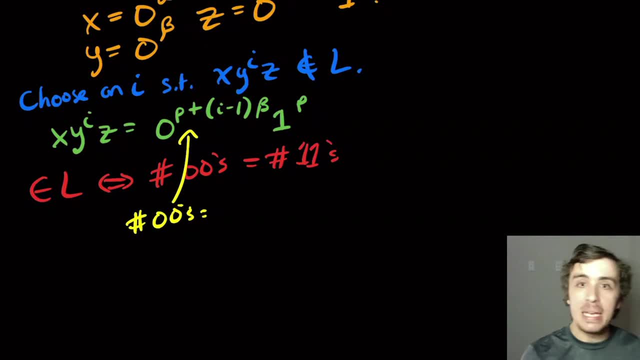 So the number of zero zeros is going to be: since this is a contiguous range, it's going to be one less than that number. So it's going to be P plus I minus one times beta minus one, That's the number of zero, zero occurrences. 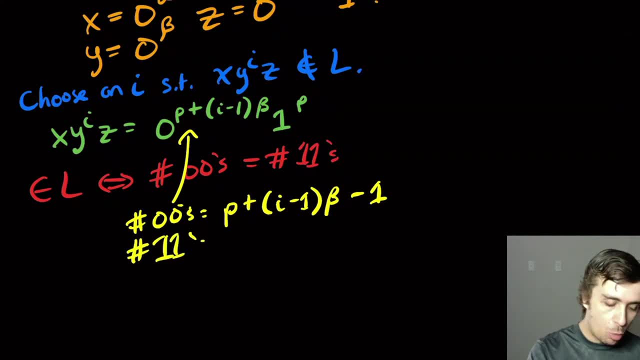 And then the number of one one occurrences is going to be one less than the other range of length, which is going to be P minus one. So this thing is in L if, and only if, these two numbers are the same. So I'll go back to red. 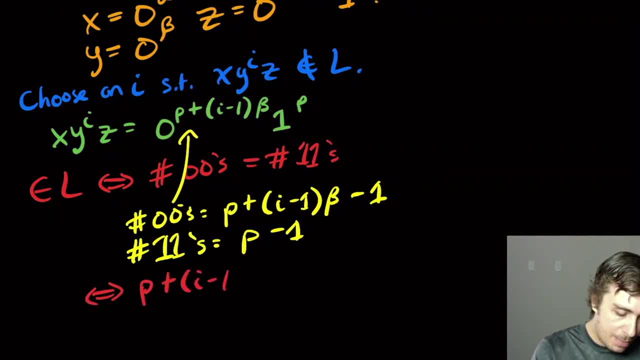 So this is if, and only if, P plus I minus one times beta. minus one is equal to P minus one. Well, we see a P minus one on both sides. Let's kill those off. So this is if, and only if, I minus one times beta. 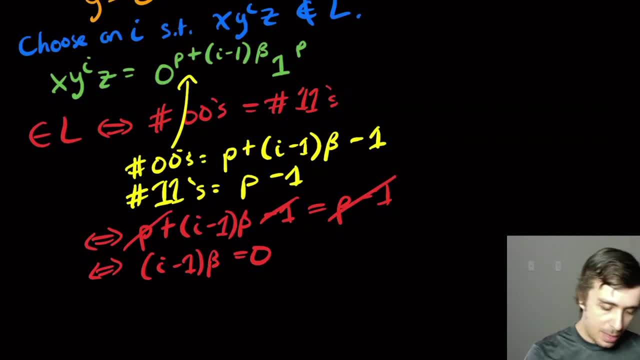 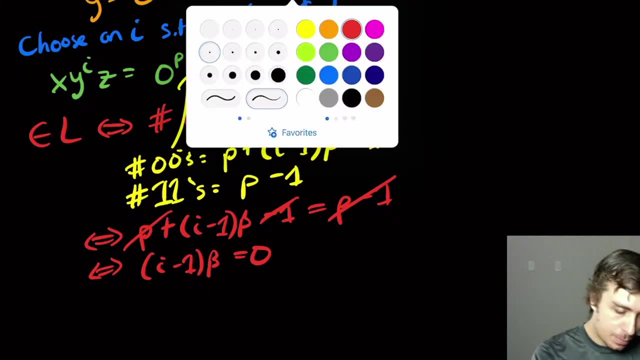 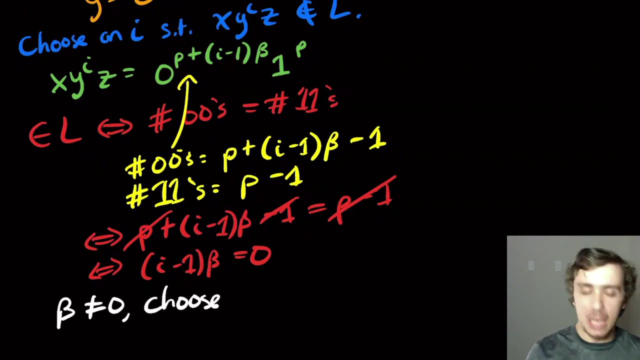 is equal to zero, And that would imply that either I is equal to one or beta is equal to zero. Beta is not zero by definition, So that's not zero. So let's choose some value of I that's not one, Let's pick two. 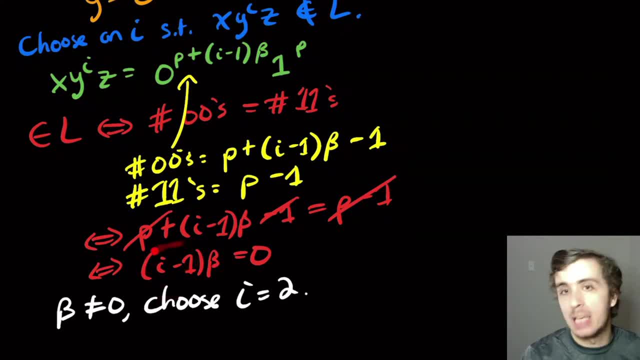 You can pick by this. you can pick any value of I that you want, as long as it's not one. Okay, so that shows us that we have arrived at a string that is not in the language and that would contradict the for all statement. 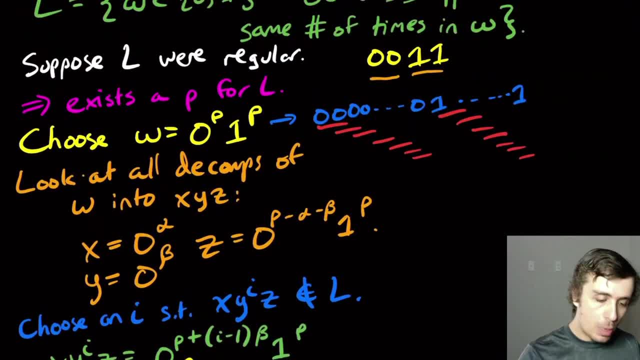 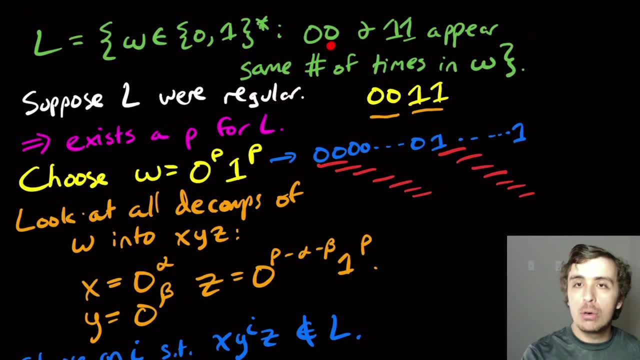 in the pumping lemma there. So therefore, we have shown that this language is not regular. Try to actually try to generalize this. So if you substituted this with zero one and one zero, it turns out that that is regular, Okay. 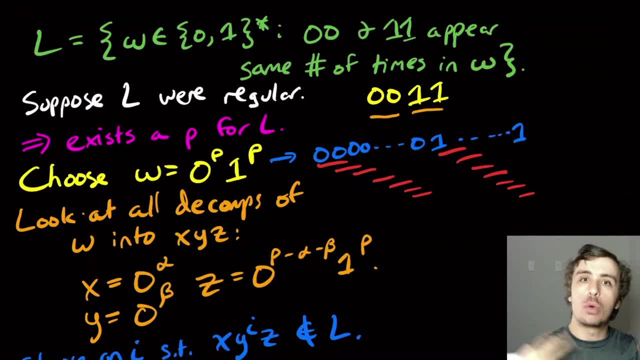 there's a whole bunch of strings, pairs of strings- where it is regular and a whole bunch of pairs of strings where it's not regular And it turns out work that I've done and some other people have done have actually shown when is this regular and when is it not. 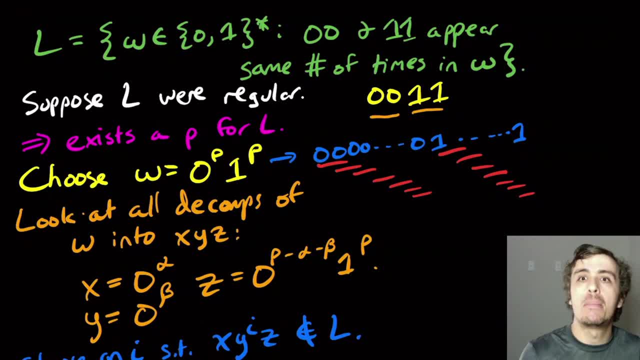 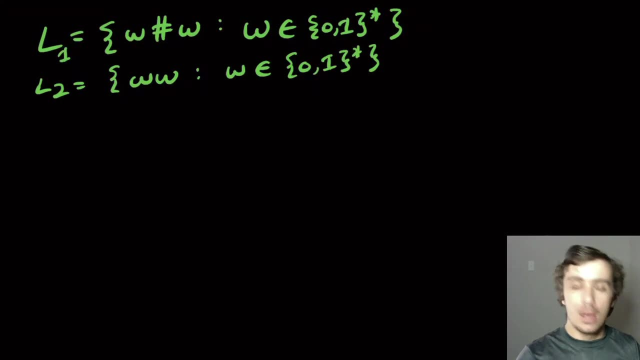 And try to actually think about. is there some kind of general pattern that you can see? And there is, and it's really cool. So we have shown that this language is not regular. Okay, so let's prove that these two languages are both not regular. 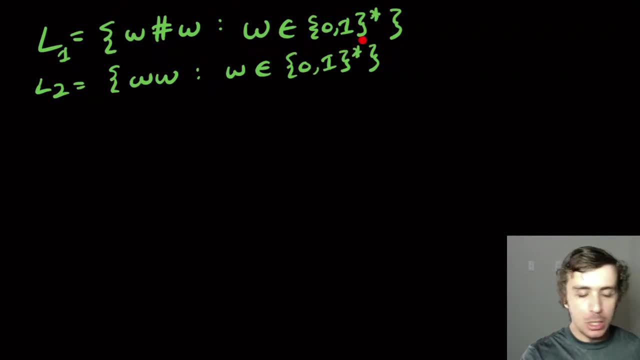 So they're very, very similar. So we have W ranging over all possible binary strings, Here are zeros and ones, And the first language has that. we have exactly the same W on both sides of some pound sign And in the second case we have the exact same string twice. 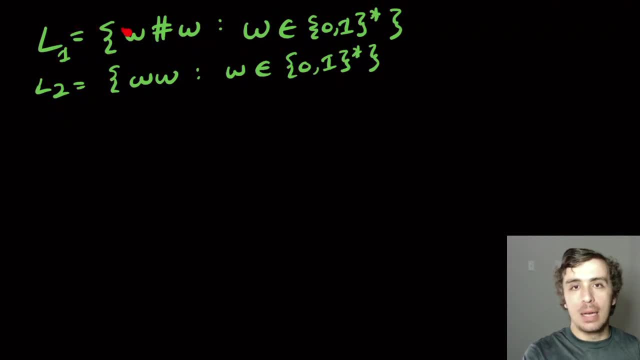 So effectively L1 can? it's exactly the same as L2, except you stick a pound sign in the middle, And I wanna show that both of these are not regular. So let's go about doing this, And what I'm gonna do is I'm gonna prove. 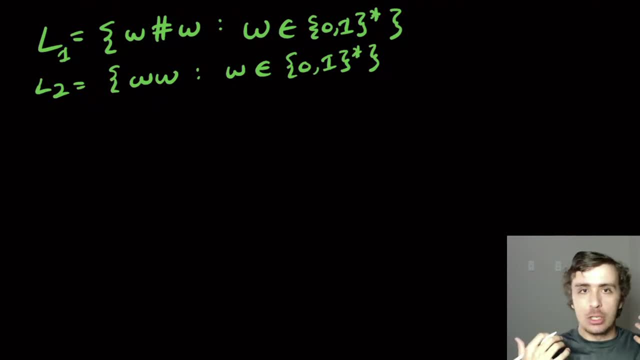 that L1 is not regular. And actually, no, I'm gonna prove that L2 is not regular And then immediately, or we'll see how to get that L1 is not regular. So let's suppose then that L2 is not regular. 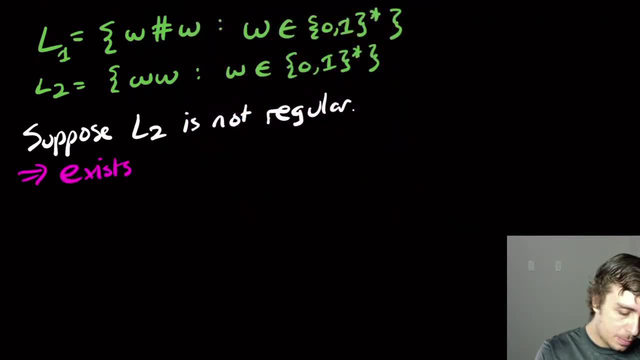 Then that means that there exists a pumping constant P for L2.. And we need to pick a string that's in the language and at least P in length. So let's go ahead and do that. Let's choose some string, and this string will not work. 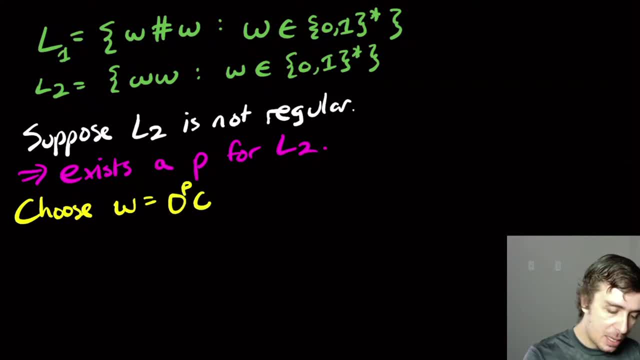 And I'll explain why. So let's pick zero to the P, zero to the P. Okay, It's in the language, because it's the exact same string twice. It's length at least P, because it's length two P. so that's good enough. 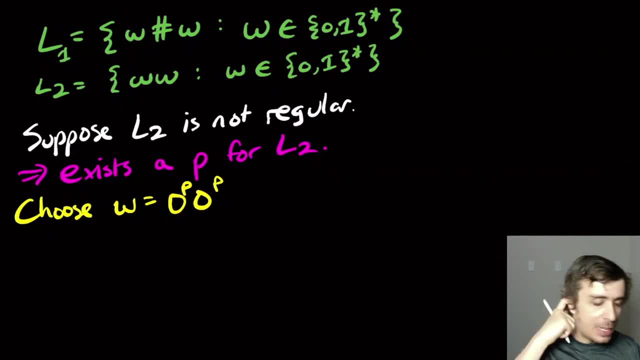 But this string won't help us. Why, Well, we need to eventually try to pump our way out of L2.. So we wanna have two pieces that are completely different from each other. The problem with that is, since this string is all zeros. 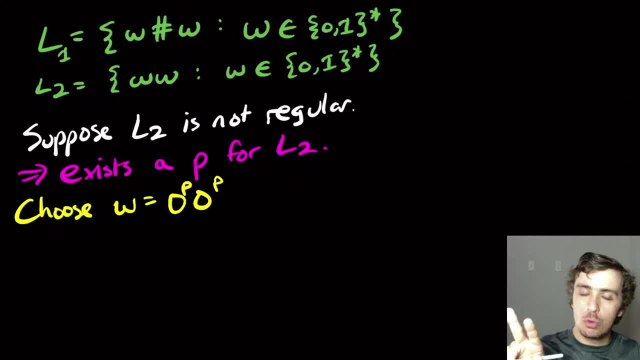 if the decomposition has the pumped piece have two or even an even number of characters, then if I pump up or down, then I'm gonna have an always have an even number of zeros. And since if I have an even number of zeros and the whole string is zeros, 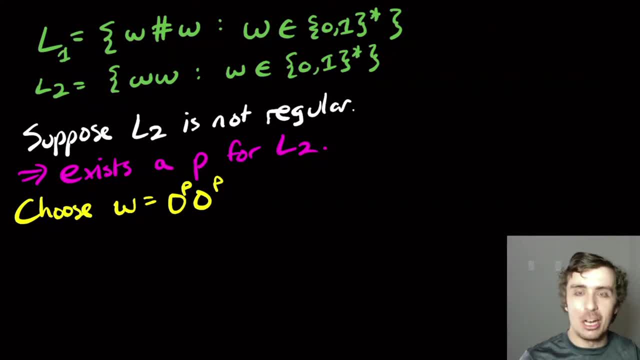 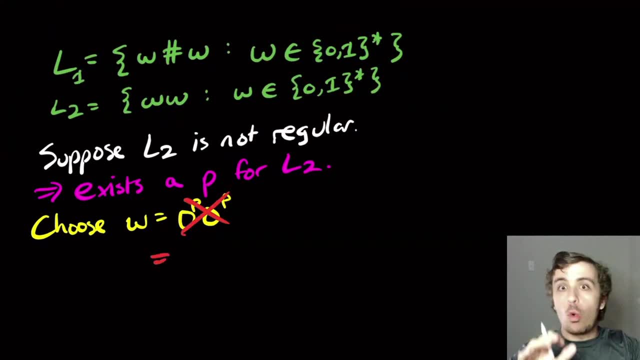 then the two halves are exactly the same, And that doesn't help us. So, yeah, so let's not do this. Instead, let's pick, have some ones mixed in. So if I have zero to the P one, zero to the P one. 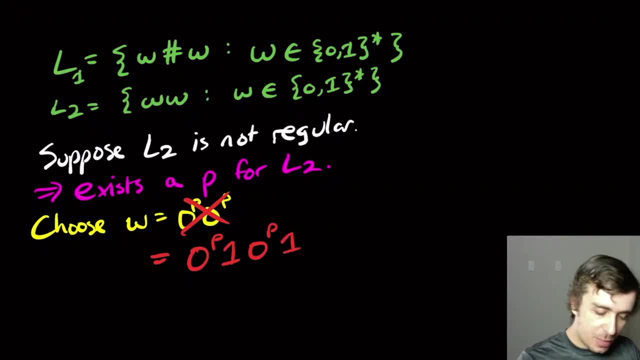 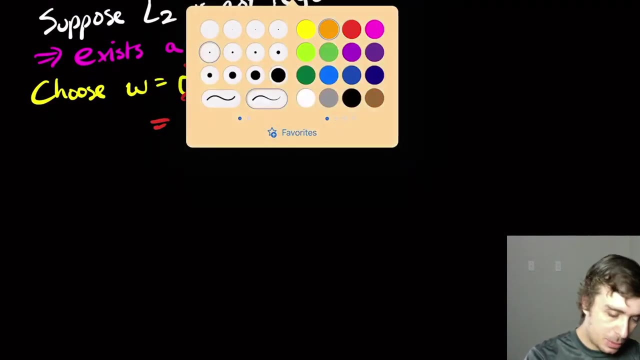 then effectively these two sets of zeros are separated from each other, And then that causes some problems with trying to keep the same number on both halves. So let's try to work with this. So we need to look at all decompositions of W. 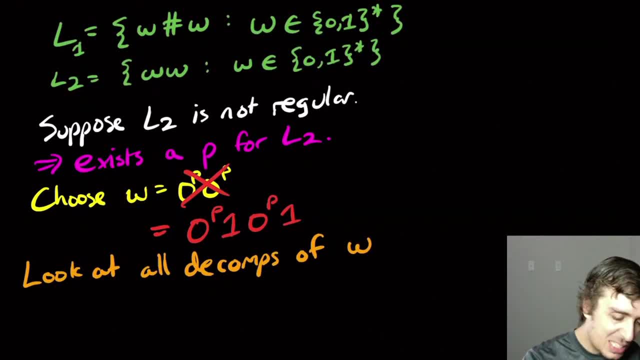 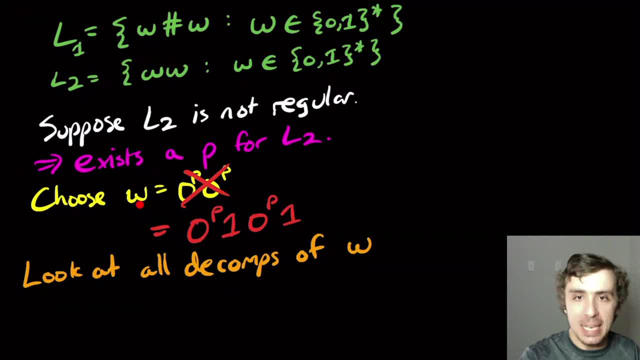 This is just a variable over a set. This is a particular string that I'm choosing. It's not being pasted up here, It's just they just happen to have the same name. This W is completely different. You should use a different variable name here. 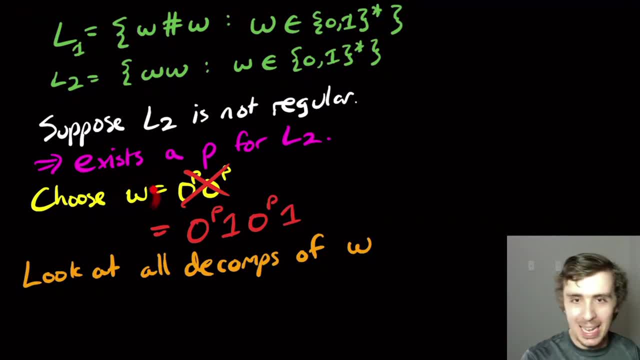 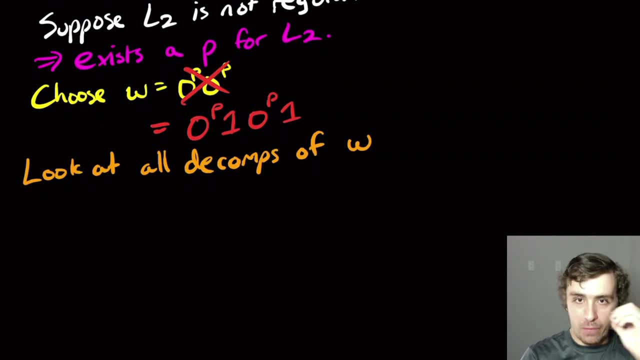 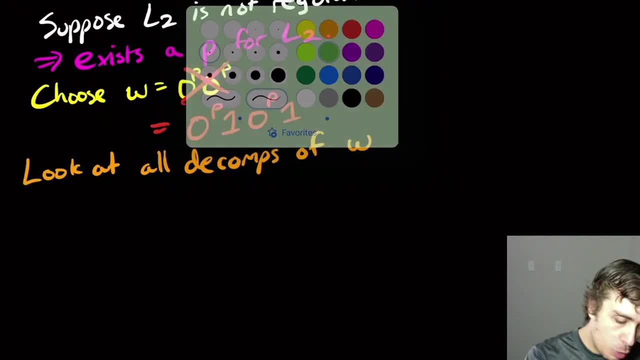 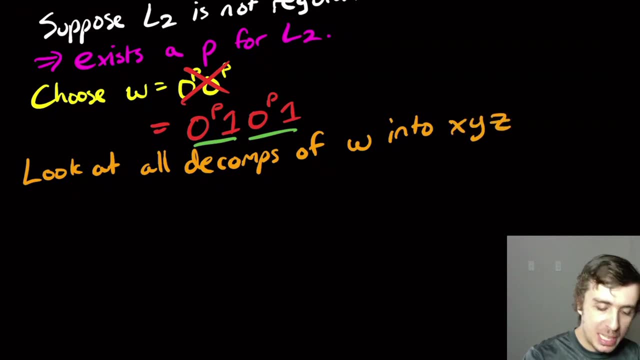 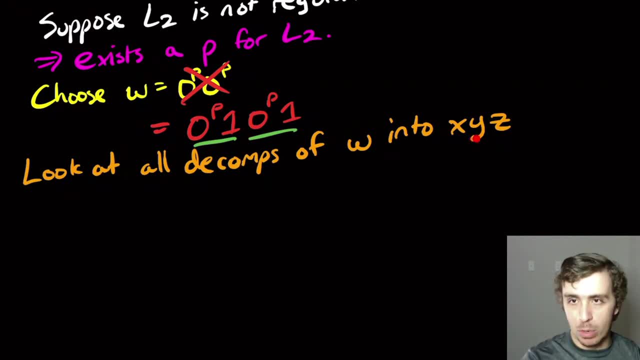 Well, here X, Y has length at most P. that's one of the rules, And since that's the start of the string, they must only contain zeros, because the start of the string has P zeros in it. So we know that X has some number of zeros. 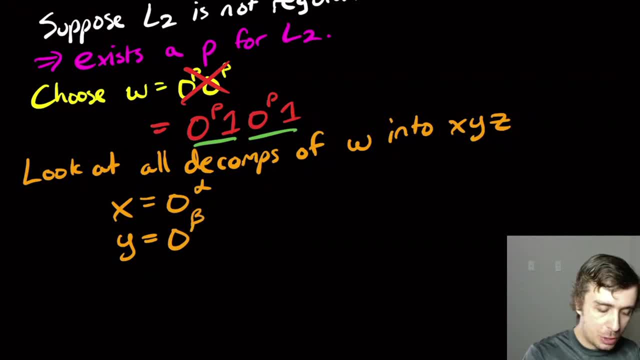 let's call it alpha. Y has some number of zeros. call it beta. Y has some number of zeros. call it beta. Y has some number of zeros. call it beta. So we know that X has some number of zeros. call it alpha. 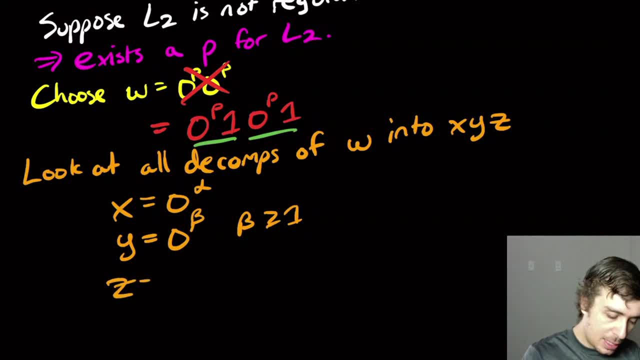 So we know that X has some number of zeros, call it beta. So we know that X has some number of zeros, call it beta. And beta is at least one And Z is the rest of that run of zeros. So P minus alpha minus beta, the single one there. 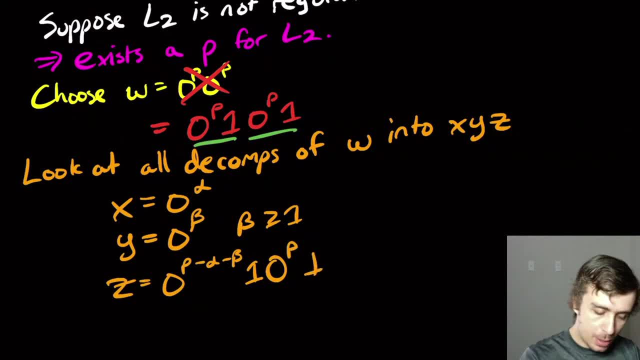 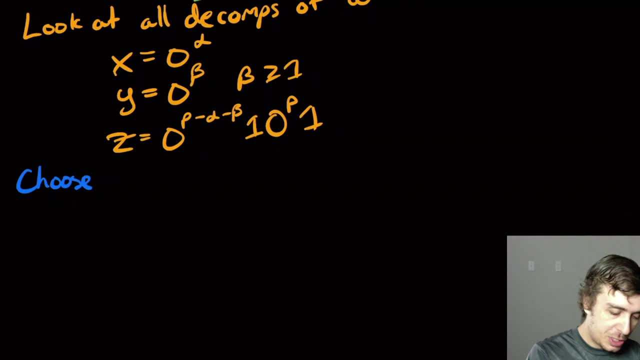 Then zero to the P- we never touch that region- And then the final one at the end. So what we want to do is we want to choose some value I such that X, Y to the I, Z is not in L2.. 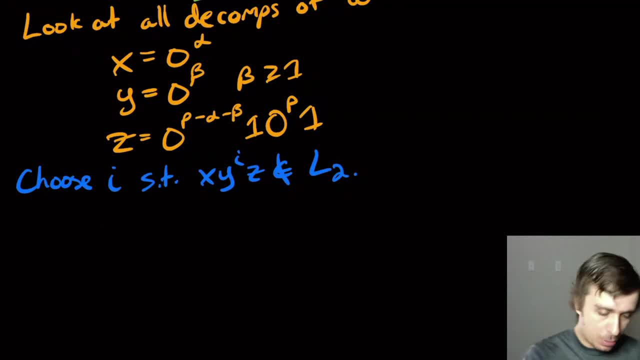 It's not in L2, okay, So let's look at it. What is the string X, Y to the I Z? We'll just paste all the things down, So zero to the alpha, zero to the I, beta. 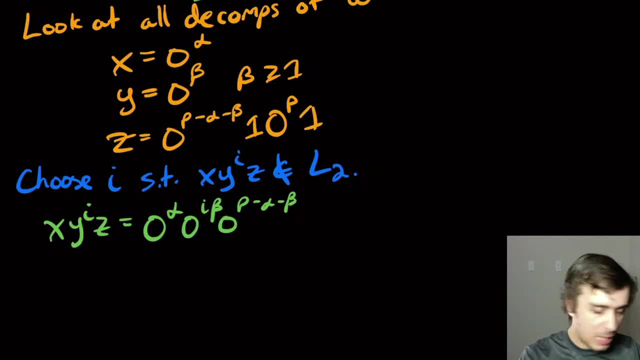 zero to the P minus alpha minus beta. It's just copying everything down, except for the Y to the I piece, because we have I copies of it. We have a run of zeros, so let's compress them So we'll have P plus alpha minus beta. 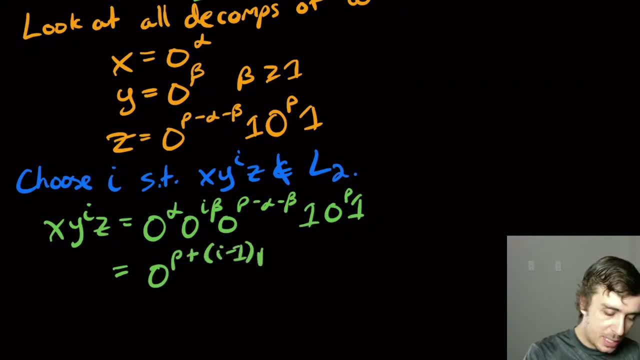 So we'll have P plus alpha minus beta. So we'll have P plus alpha minus beta. So we'll have P plus I minus one times beta, a single one, and then zero to the P one. So this thing is. I'll go up here. 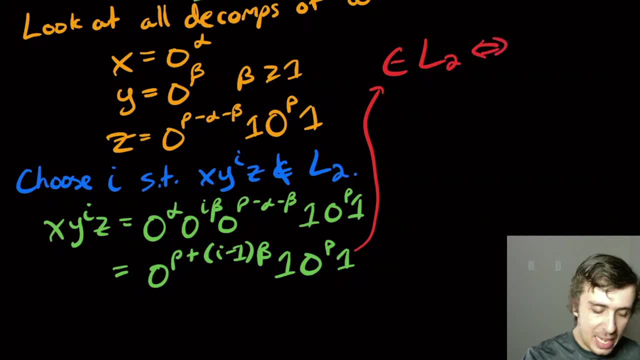 So this thing is in L2, if, and only if, the two halves are the same. So it's a fallacy to think that the middle is right here anymore. It's not So the middle has actually moved, Depending on the choice of I Z Y Z Z. 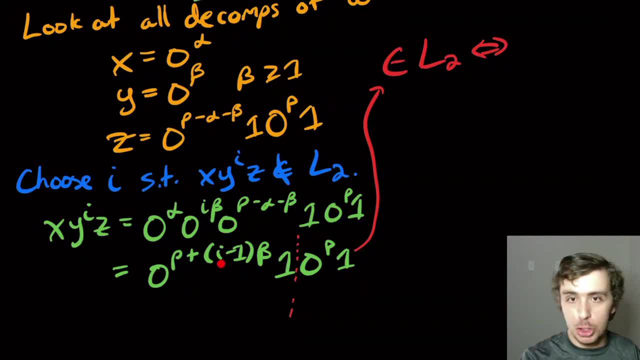 or the other half of I here. So if I is two or more, then this line has moved left because we put more stuff over here. So the middle point is over in here, somewhere in the zero, somewhere, Whereas if I is zero, 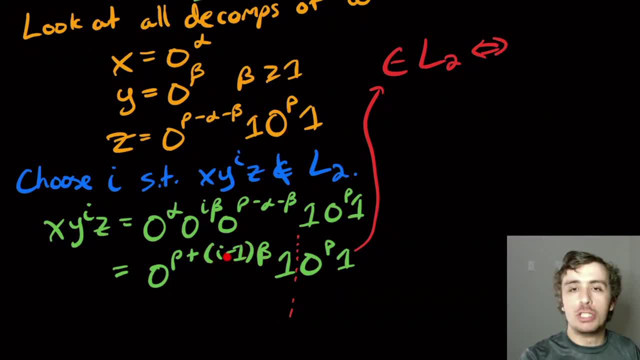 but we can't choose. I equal to one because of the original string. If we chose zero, then it moved over here. So let's choose some. let's choose some. I at least two. If you choose, I equals zero. you'll get a different conclusion. 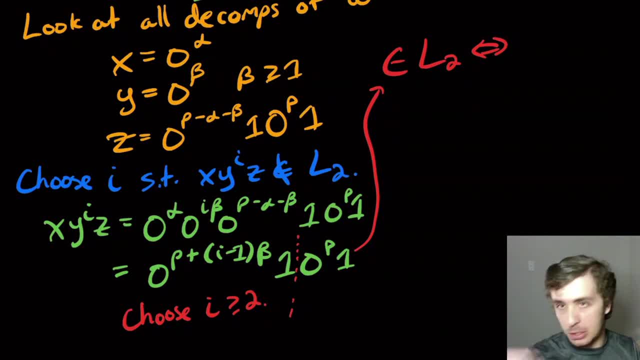 but it's the same. You'll still show that it's not regular. It's just a different conclusion. So that means if, and only if, the two halves are the same, the two halves are equal. Well, let's try to visualize what it looks like. 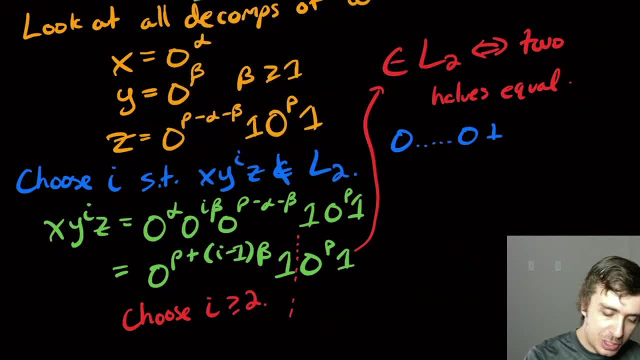 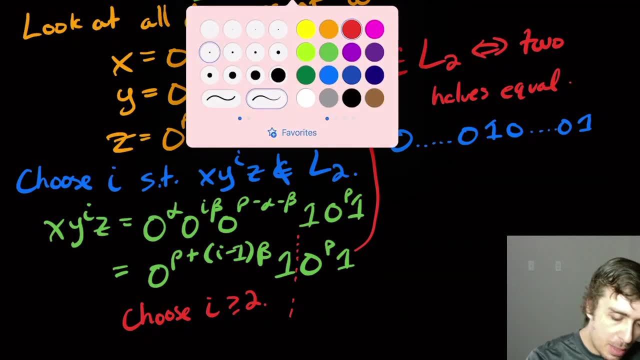 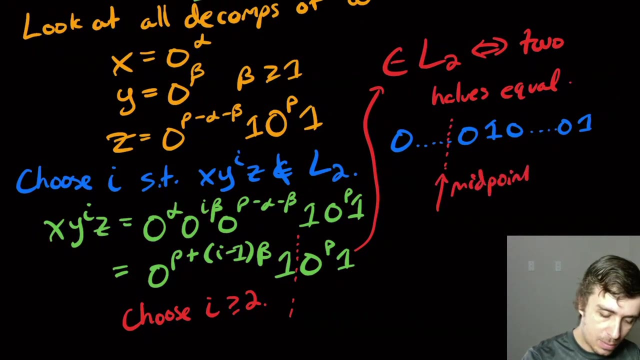 So we have a whole bunch of zeros: at the beginning, The single one, Some smaller number of zeros there, And then the one, But here the midpoint is right in here somewhere. So that is the midpoint. But notice what happened here. 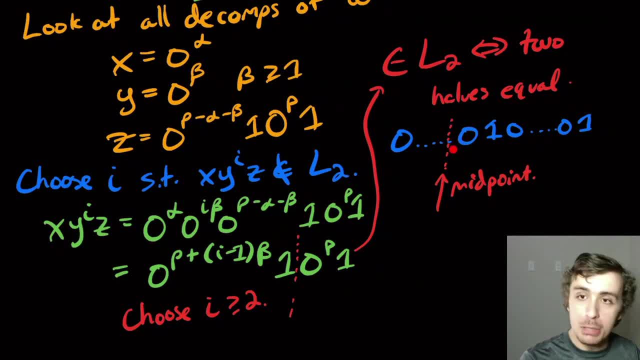 So this right half starts with the zero, or it's actually not necessarily starting with a zero, but it ends in a one for sure. The second half ends in a one, And the first half ends in a zero, And so the two halves cannot possibly be the same. 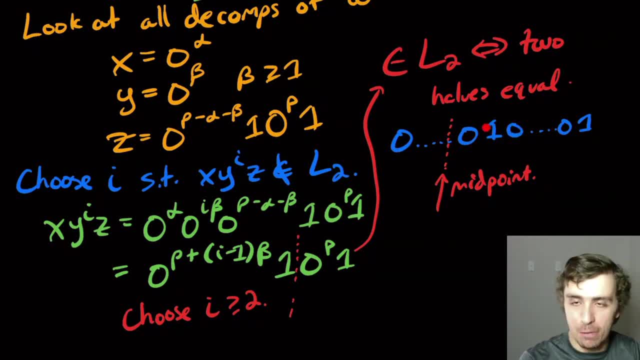 because they, in this case, end differently. If you choose, I equals zero, you'll find out that the two halves don't start the same. Okay So, or you'll actually have a different structural problem, depending on what actually happens. But here we know that the strings end differently. 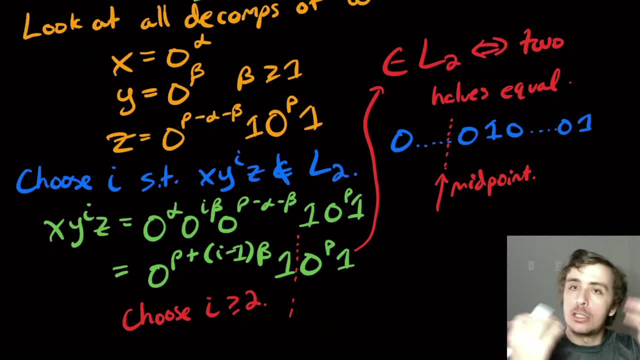 the two halves. This ends in a zero, This ends in a one. So therefore, the original string, this string that we just made, is not in the language L2.. And then, therefore, L2 is not regular because we contradicted the for all statement. 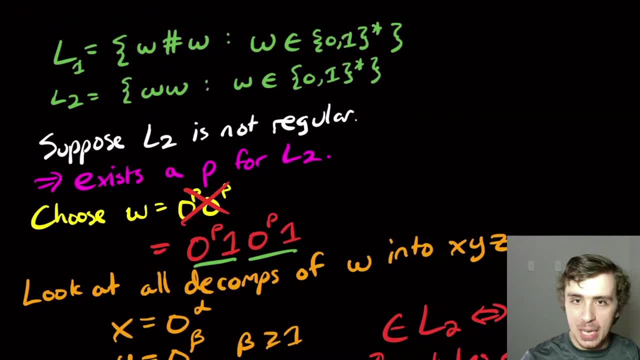 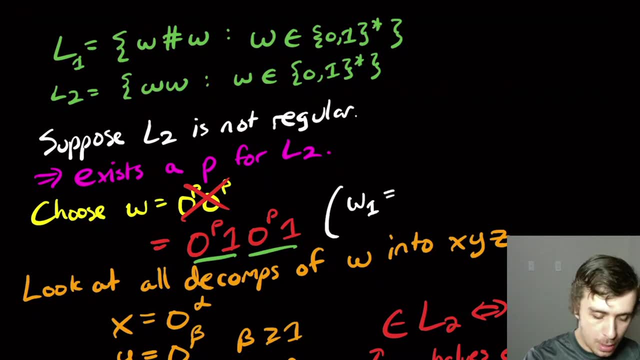 in the pumping lemma. Okay, So let's prove that L1 is not regular. So for L1, what would we need to do? I'll call the string W1.. Well, that's, we're going to do something very similar. 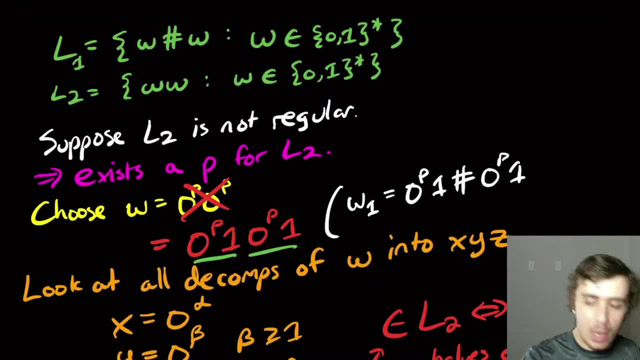 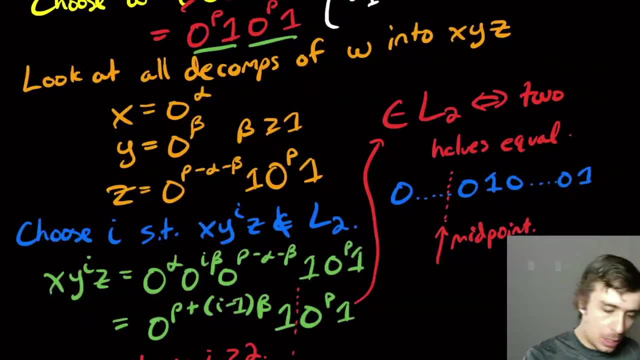 We're going to have zero to the P1, zero to the P1.. There are actually many other strings you could have picked, not just this one. Well, let's think about what happens. So if we substituted the pound sign right there? 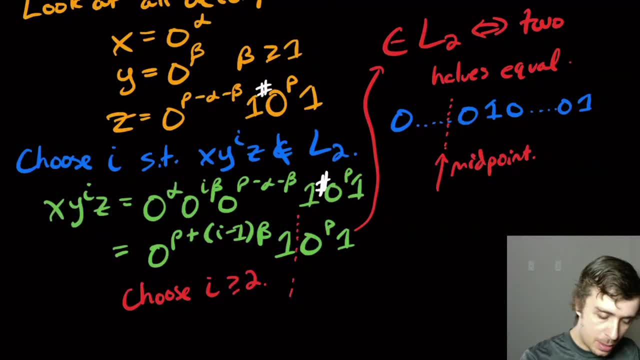 and then let's see what happens. The pound sign is right there. The pound sign is right there, probably. So then here the. what are the things that can happen? Well, we need. so let's see where the midpoint is. 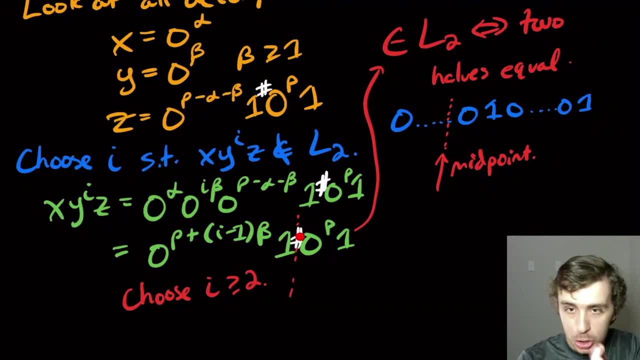 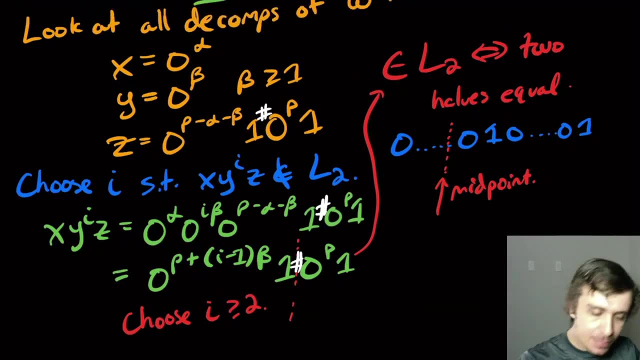 So the midpoint was right on the pound sign initially. So the midpoint was right on the pound sign initially, But then, because we put more stuff over here, it's on one side of the pound sign. So for a string to be in L1,. 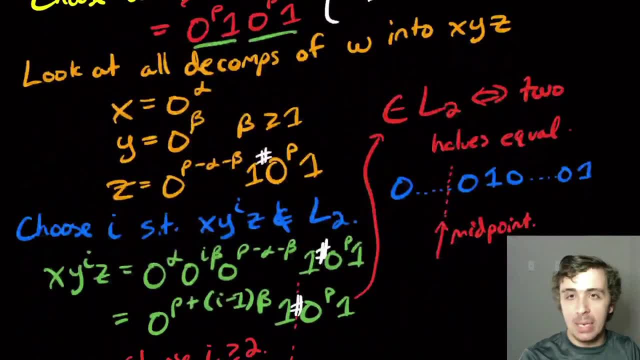 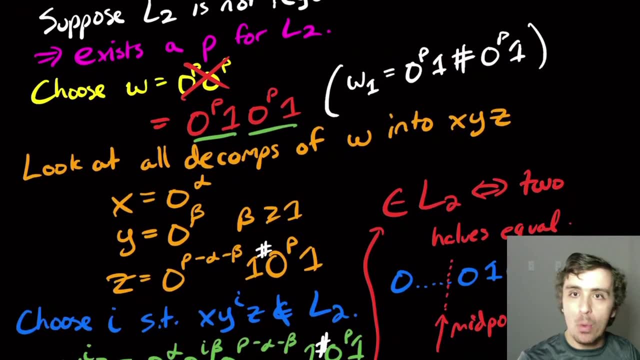 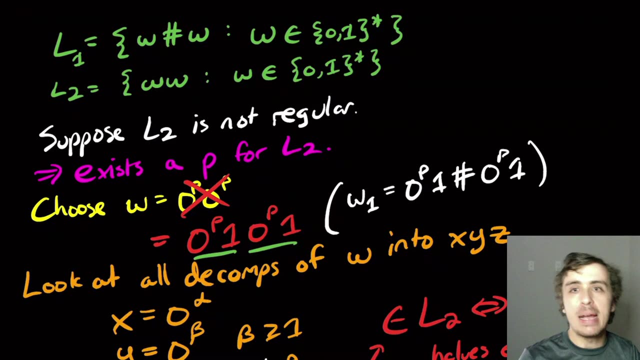 it needs to be right on the pound sign, the midpoint, Whereas here it moved past the midpoint. So it's a little bit more illustrative of where the midpoint actually is. But the languages are very, very similar in that you can prove that both are not regular. 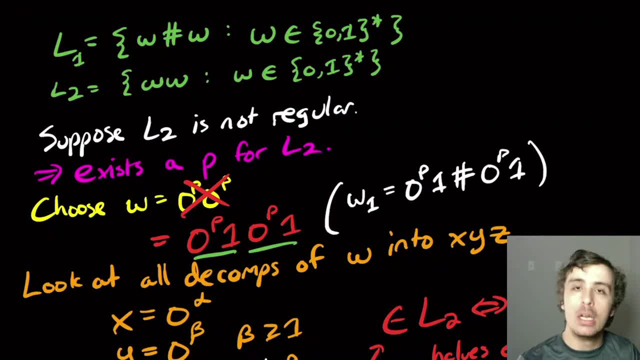 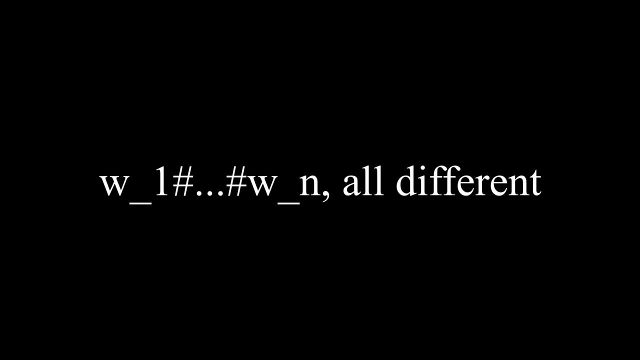 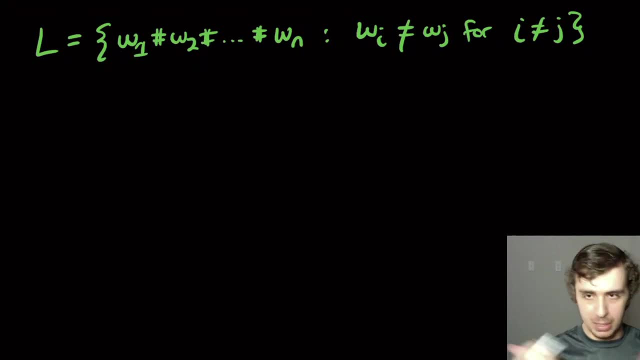 just using one proof and adapting it. just using one proof and adapting it for the other language. So here we have shown that these two languages are not regular. Okay, so let's prove that this language is not regular. So it's a little bit complicated to explain. 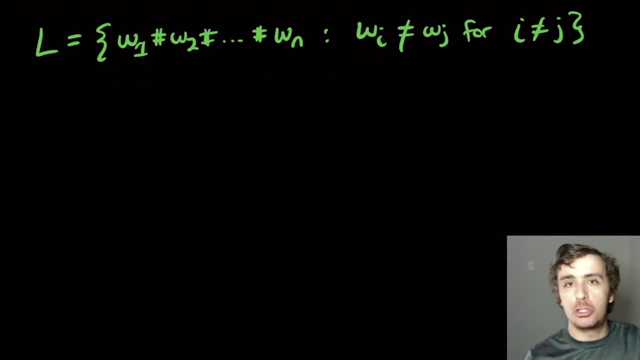 but the basic idea is that we have a whole bunch of different strings delimitered, separated. So here we have a bunch of Ws right here. So these Ws, let's just say for convenience that they are strings in zero, one star. 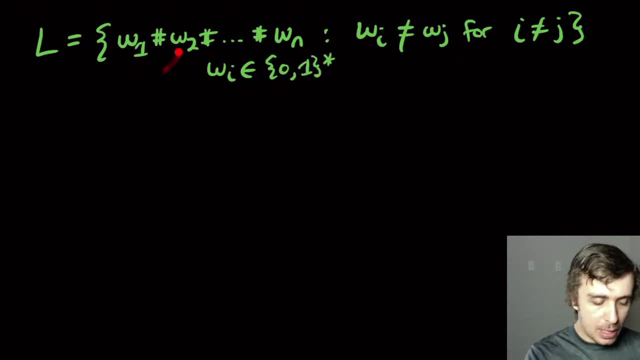 just purely for convenience. But here every single one of these strings is different, So there's no duplicates among these end strings. Okay, that's all it is. Okay, there's no bound necessarily on how many strings we got, but we can have as many as we want. 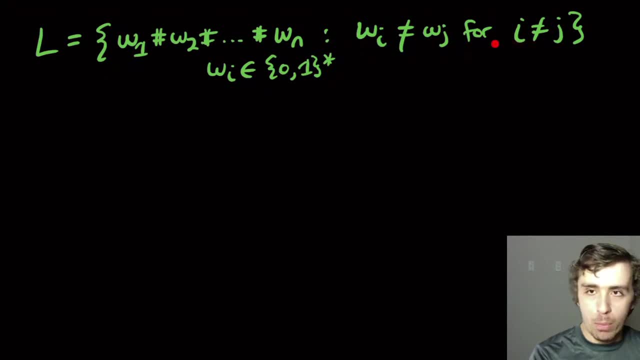 as long as they're all different. Okay, this is just a formal way of saying that if you have different indices, then the strings corresponding them are different. If I look at W1 and W1, then clearly it's equal to itself. 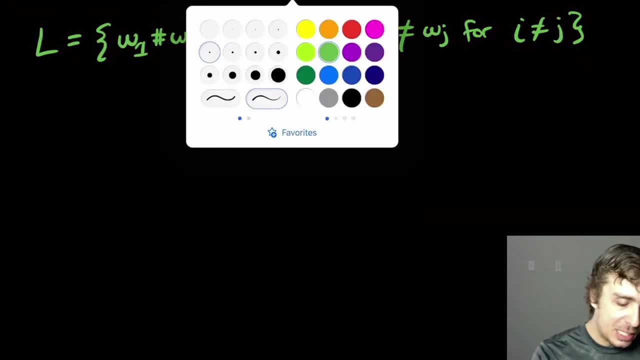 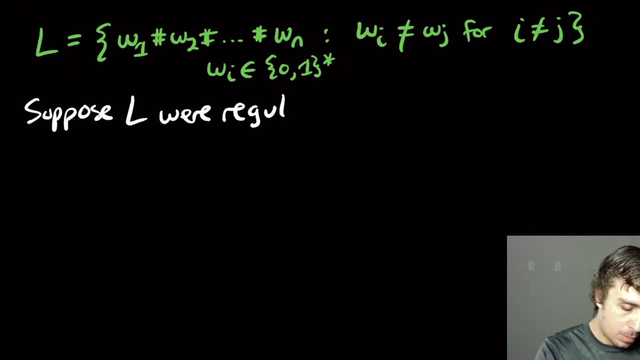 So that's not really useful. So let's prove that this thing is not regular. So let's suppose L were regular. Then that means that there exists a pumping constant P for L. I'm just short-handing it here. So now we got to. the hard part is to pick up the string. 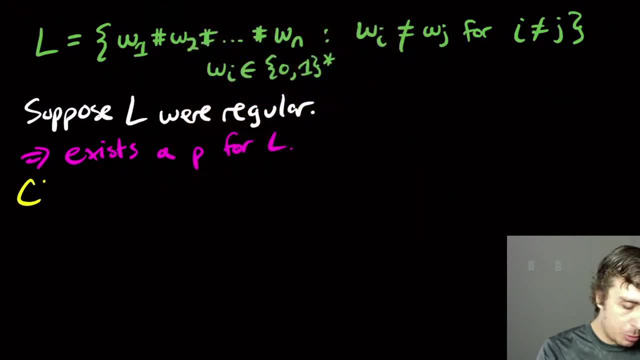 So now we got to, the hard part is to pick up the string. So now we got to, the hard part is to pick up the string. So let's think about what we would do. So we would choose W equal to something. 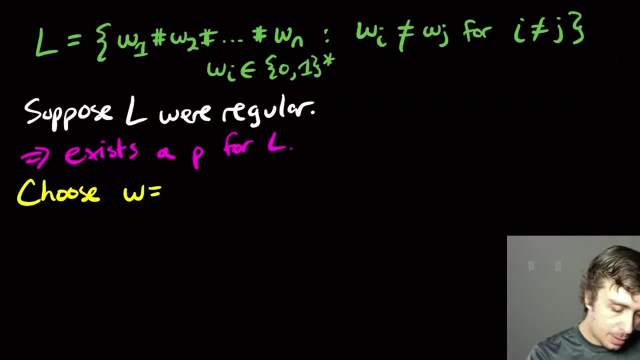 And what you would think to do is to, let's say, I'm gonna pick zero to the P and then pound sign some other stuff. Well, think about what happens. So if I have this at the beginning, then I'm gonna be only pumping in this region right here. 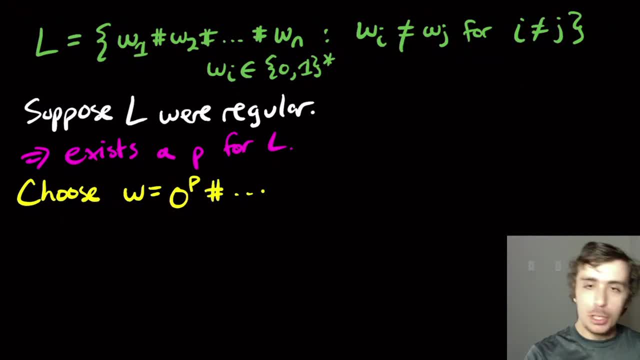 Okay, because that's one of the conditions of the pumping limit. So let's just say: we pump up one time. Okay, if we pump up one time, then the number of zeros in this region is between P plus one and two P. 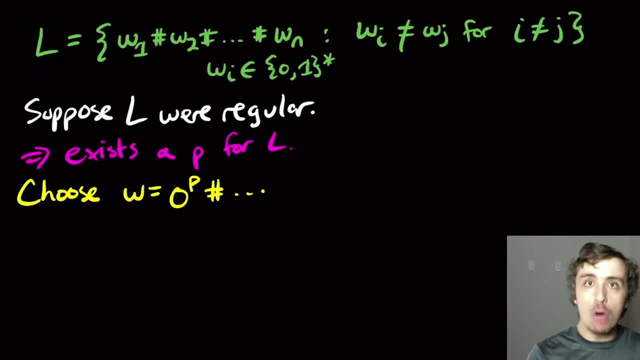 You must have at least one more one, and at most P more zeros, sorry, And at least one more zero and at most P more zeros. So what we can do, then, to try to get a contradiction, to get a string that's not in L. 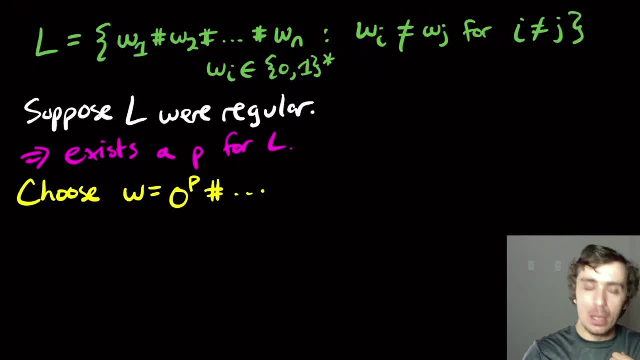 to get a string that's not in L from a string that was in L is to say, okay, well, this thing can land somewhere between P plus one and two P, Let's embed it in the string. So by embed, here's what I mean. 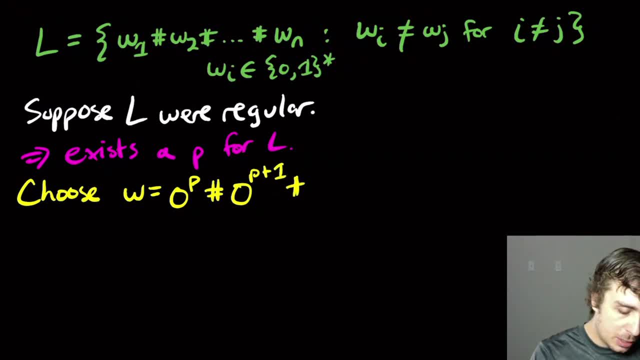 So I'm gonna have P plus one zeros here, delimiter, P plus two zeros, delimiter, And keep going up by one until I reach two P. So note that this is way more than P characters. It's like P squared, probably, or something like that. 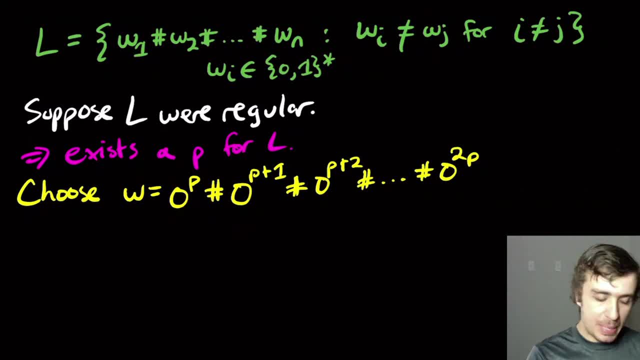 But notably that this is in the language, because each one of these runs is different than every other run. In fact, we didn't even need to have the one character here, but if we pump this region up one time, then we are gonna have this region's length. 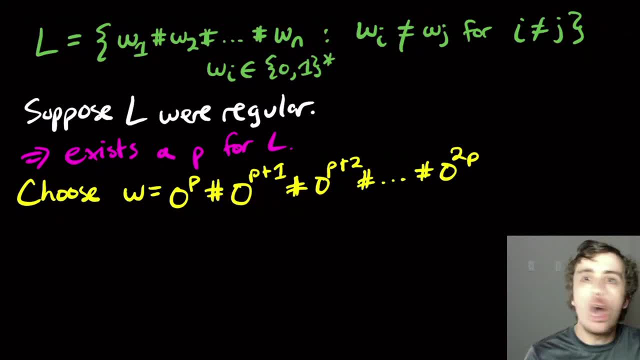 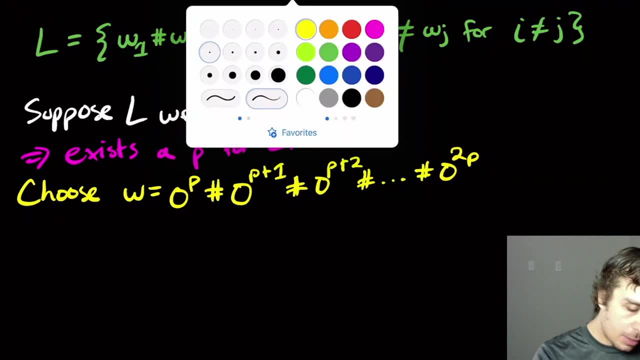 to be the same as one of these other ones. I have no idea which one, but we know it must be in one of those somewhere. Okay, so then let's try to make this a little more formal. So we need to look at all decompositions. 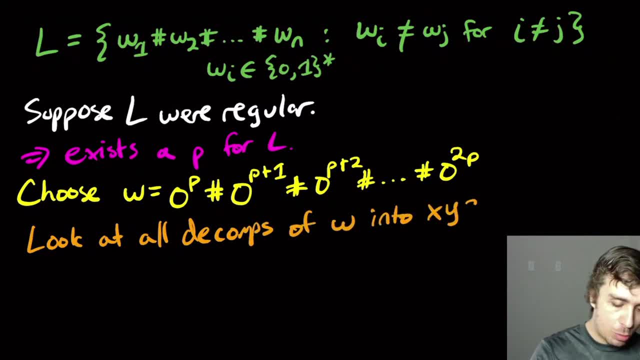 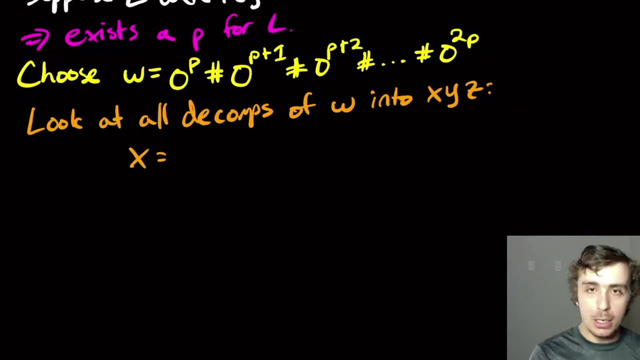 of W into X, Y, Z, according to the rules. So the rules say that X and Y have at most P characters. So in this case, since the string starts with P, then we must have all zeros in the X part. 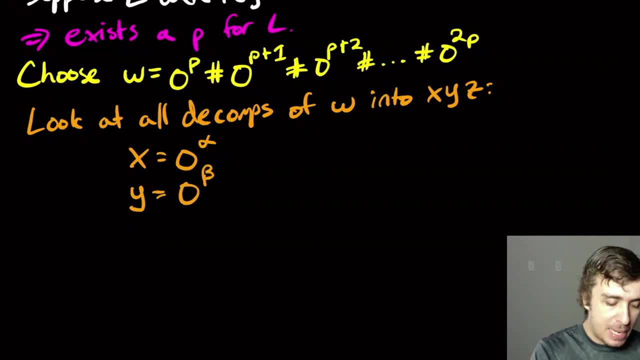 Let's say alpha of them, And Y has beta zeros. Let's just say it can have any number of zeros as long as it obeys the rules and has at least one, And Z is the rest. Well, Z is gonna be P minus alpha minus beta. 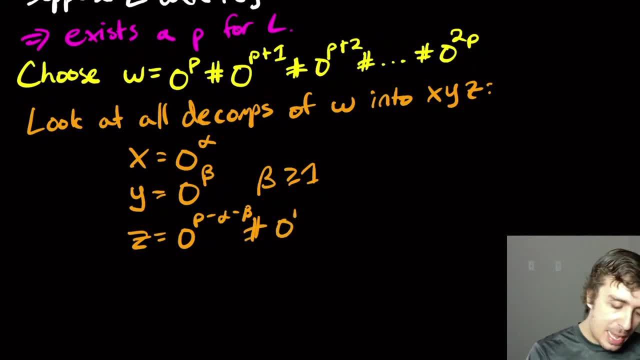 That's the number of zeros at the beginning that are left, And I have all of these other ranges still there. Okay, I still got all those other ranges over there And you could have done something similar if you wanted to pump down or pump up twice. 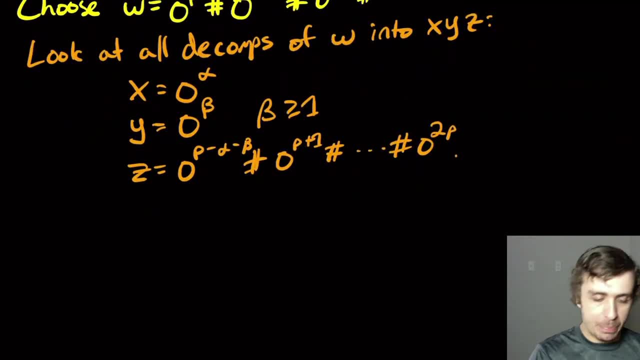 There are many other things you could have done here. This is just the simplest example I can think of. So we need to choose: I equal to two. We're choosing I equal two because that's what we started, what we wanted to do in the first place. 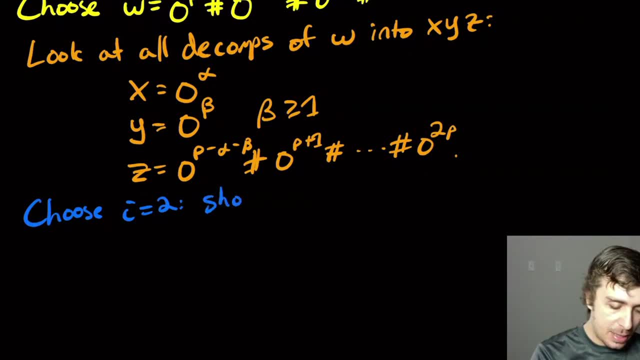 And we wanna show that this thing is not in the language. So we wanna show that X Y to that number two is not in the language. It's not in the language, So let's compute what that is. So X Y squared Z. 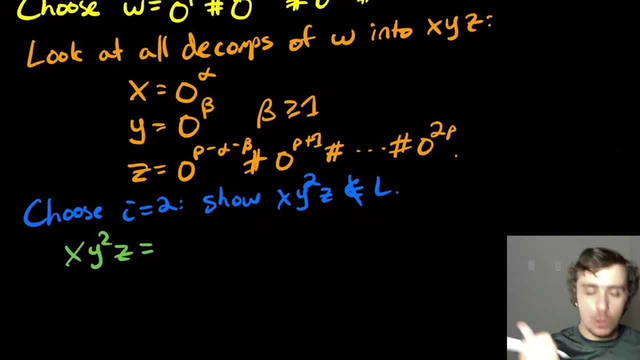 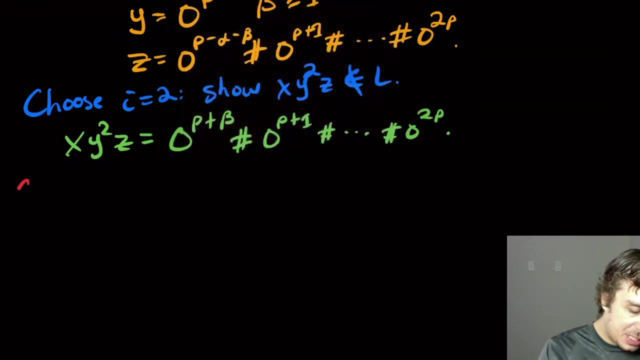 Well, we're gonna basically just get a gain of beta in the first run. So we're gonna get P plus beta, pound signs, P plus one pound sign, et cetera, pound sign, two P. So this is in L. 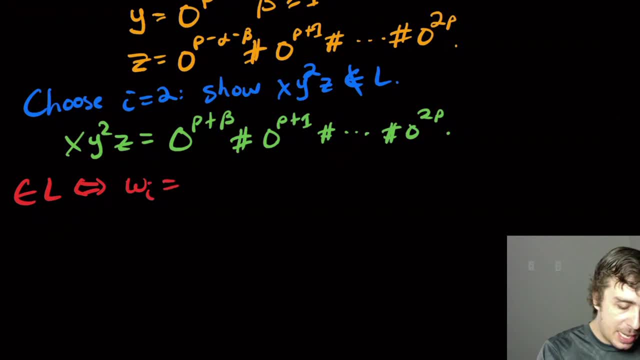 If, and only if, W I is not equal to W, J for all I not equal to J. Well, among the ones over here they're unmodified. So therefore any pair among here is, they're automatically different. So we don't need to worry about those. 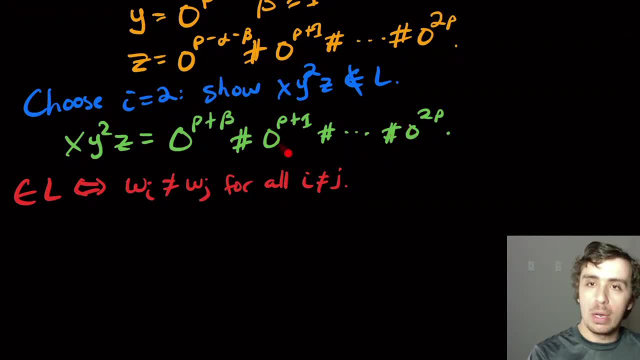 The only thing is this one could be equal to one of these other ones. So this is true. This is in L if, and only if, P plus beta is not equal to P plus I, for any. oh, let's see, between I is between one and P, okay. 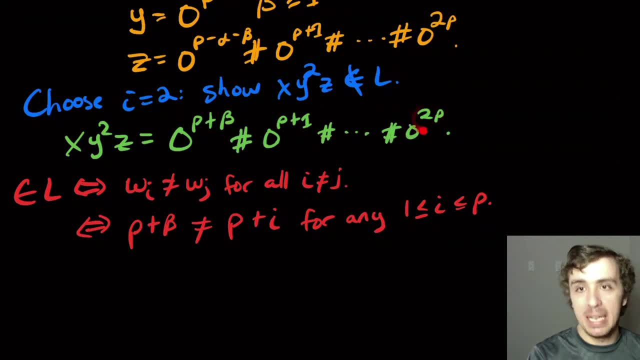 I'm just encoding how many more I add to the initial P that I have. So I started with one, which is right here, and I ended up with P, which is this one here. So this is if, and only if, beta is equal to I. 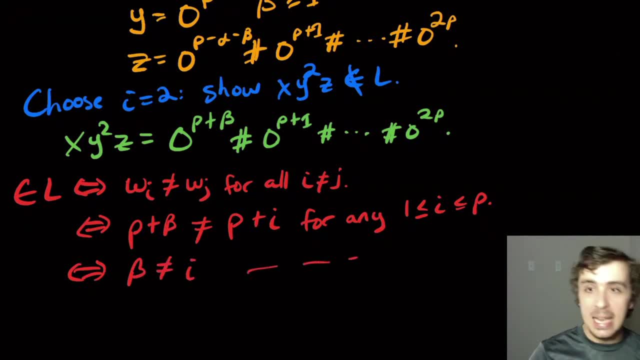 if, and only if, beta is not equal. Okay, for any i between one and p, but beta has to be one of those numbers, because it's at most p and at least one, which is a contradiction. so therefore this, so this is a contradiction. so therefore, this string is not in the language and so therefore, this language of all these. 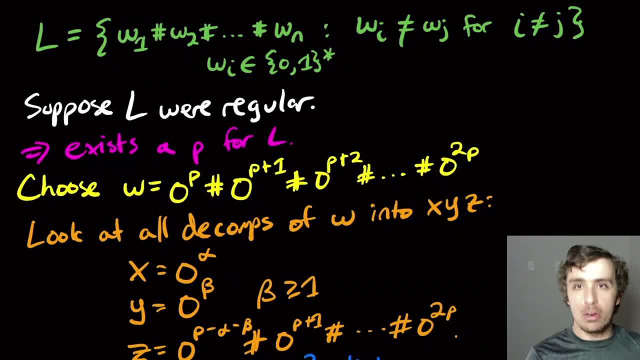 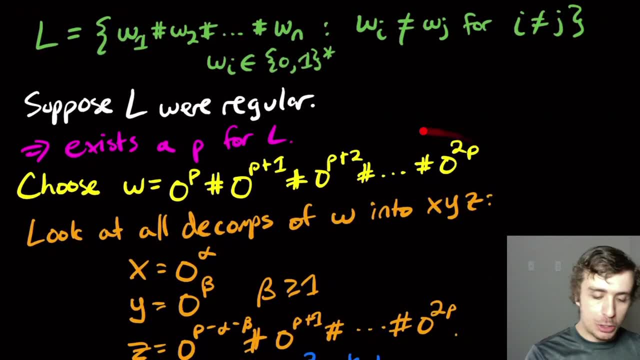 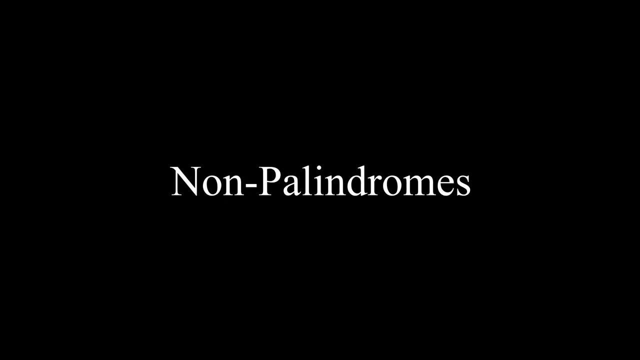 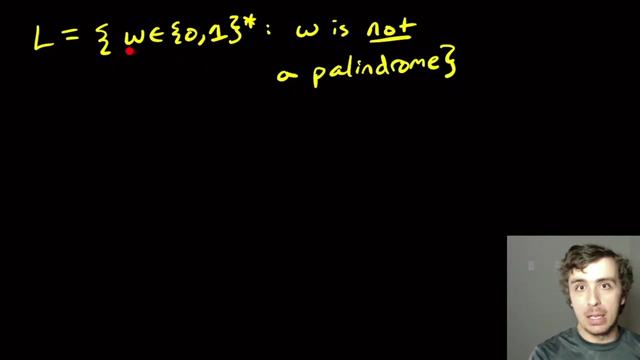 different strings that are different is not regular, because we can show that we can arrive at a string that is not in the language from a string that initially was in the language. okay, so let's prove that this language is not a. it's not regular, so it's the set of all strings. 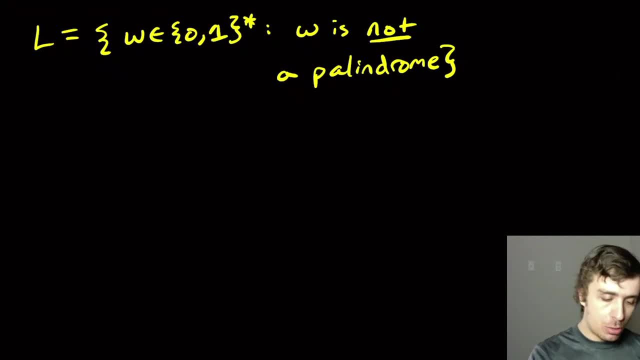 that are not palindromes. okay, so as an example, a BBA that is a palindrome, so it's not in L. but if I take away one of those characters- let's say that one- then it is in the language L here. so whenever you have a question to show, 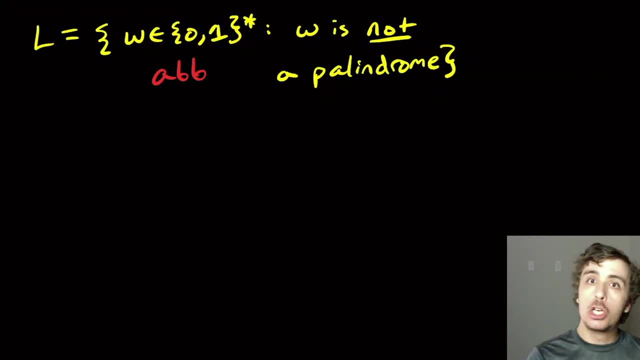 something that's not regular where it says: is not something. a good technique is something called a p factorial trick. you can search it on YouTube if you wanted to. I made a video on it. thank you very much, but I'm gonna reintroduce it here. so let's try to prove that this thing is not regular. so 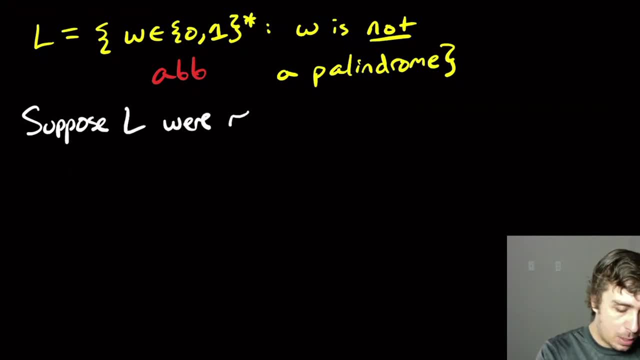 let's suppose L were regular. then there exists a pumping constant p for L. so there exists some string that is in the language for this language, L. so now we've got to pick a string that is in the language and length at least p. so let's choose W, equal to well. we've got to pick something that's not a palindrome and we want 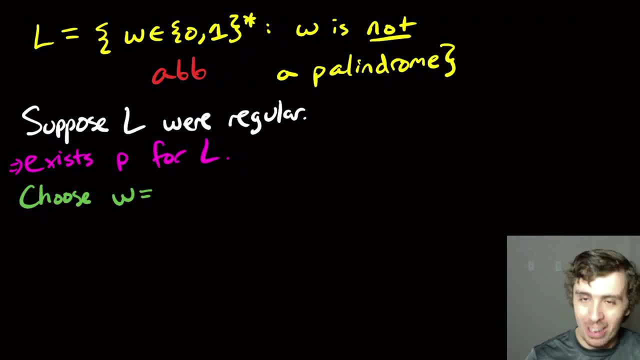 to arrive something. that is something that is a palindrome, which is kind of hard because the things can have a lot of different lengths. you want to make sure that you can always eventually arrive at a palindrome, which is kind of hard if you think about it. So what we're going to do here? 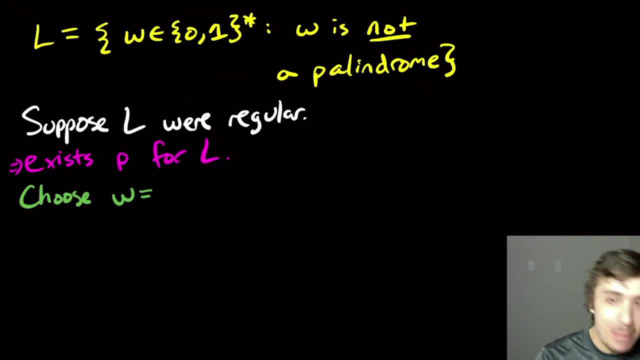 is this. Oh, actually, I should say ABB is not in there. I meant 011.. That's in there, Okay. Okay, So let's pick. let's say 0 to the P1.. I'd like to do 1,, 0, and I got to have some number. 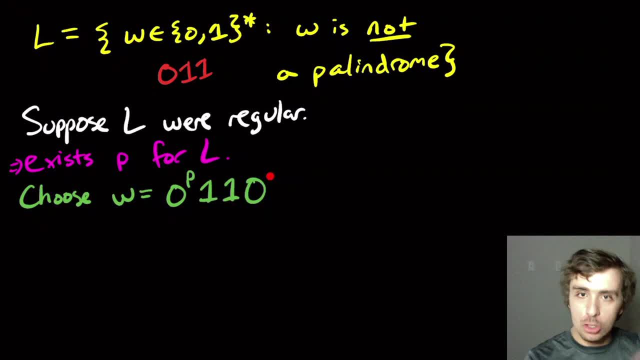 other than P here, because if I put P here then it's going to be a palindrome. I want something in the language to start with. So what I'm going to do is I'm going to pick P plus P factorial, So this is something called the P factorial trick. The reason is that, no matter what you- 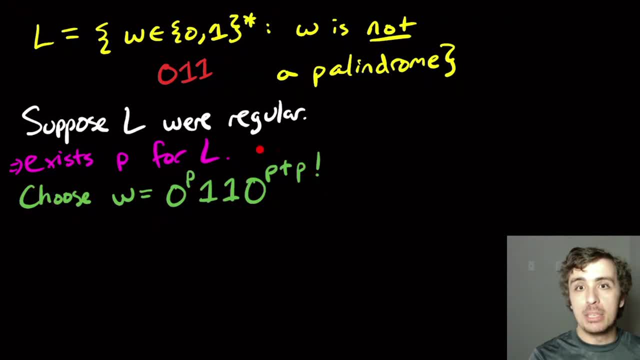 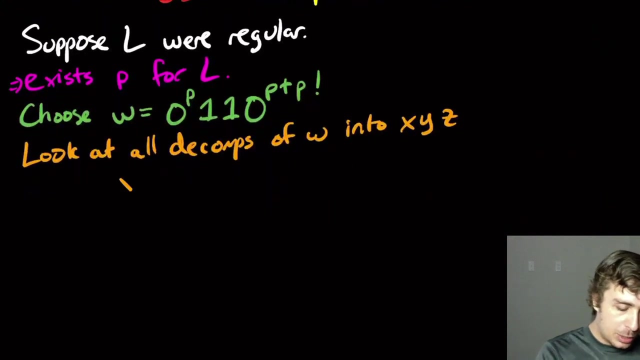 pump over here P factorial. The P factorial is a multiple of the length of whatever you pumped over here and we'll make that more precise later. Okay, So let's look at all decompositions. So look at all decompositions of W into X, Y and Z, according to the rules. So X is going to be. 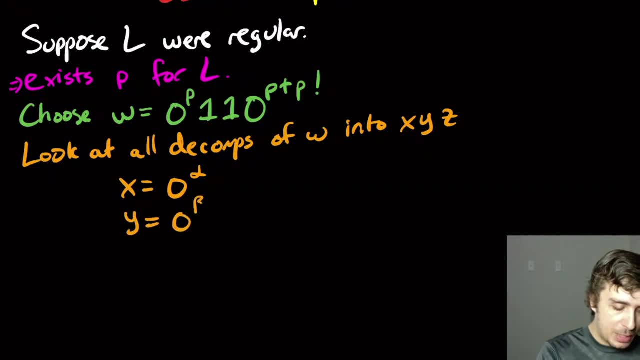 some number of zeros. in this case, Y is going to be some number of zeros in this case, also because the first P characters are zero, and that's one of the rules, and z is going to be the whole rest of the string. so p minus alpha, minus beta, that's the amount left, the two ones in the middle, and then zero to the p. 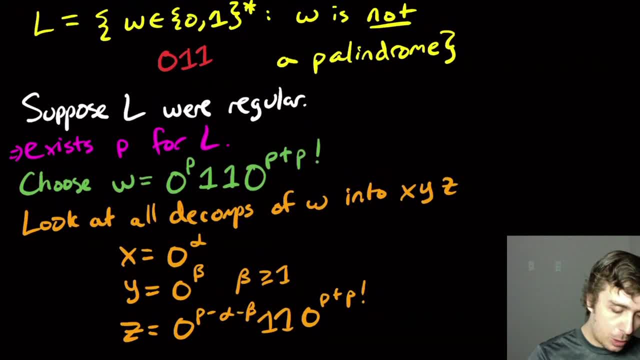 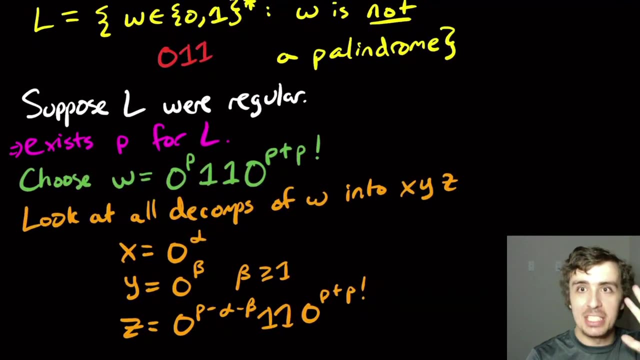 plus p factorial. i should check first. this is clearly a length, at least p, and it's not a palindrome because p fact p plus p factorial is strictly more than than p. so it's not in the language so that. so so it is in the language. i should say it is an l, it's not a palindrome. it. 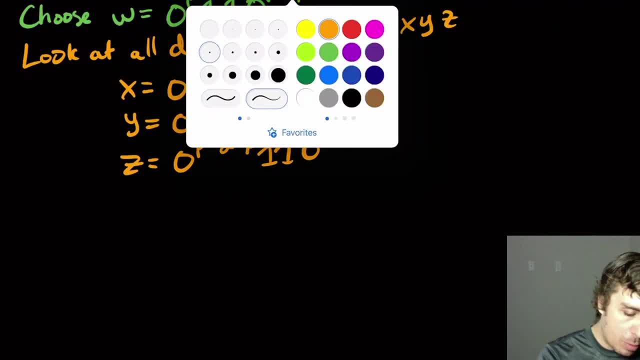 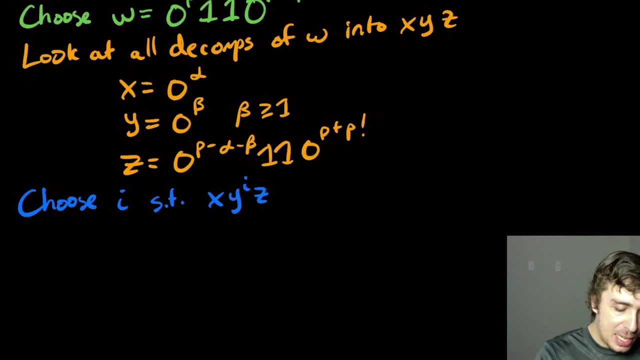 is in the language, okay. so now what we want to do is we want to choose an i an i, such that x y to the i z is not in l. in other words, x? y to the i z is a palindrome. okay, because that's what it means: to not be in the language. 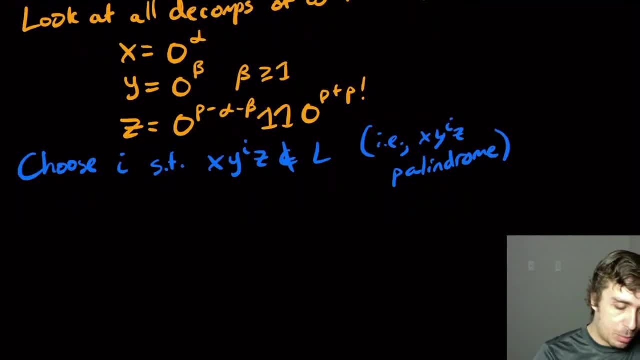 okay, so let's actually compute what this, what this string is. so x, y to the i, z, that's going to be zero to the p plus i, minus one beta- the two ones in the middle, and then zero to the p plus p factorial- the one ones in the middle are preventing the zeros from being squeezed together and that. 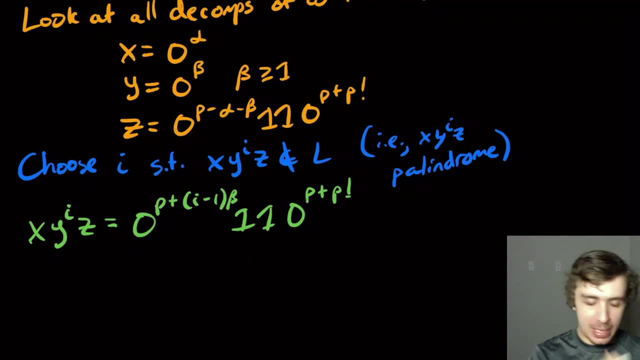 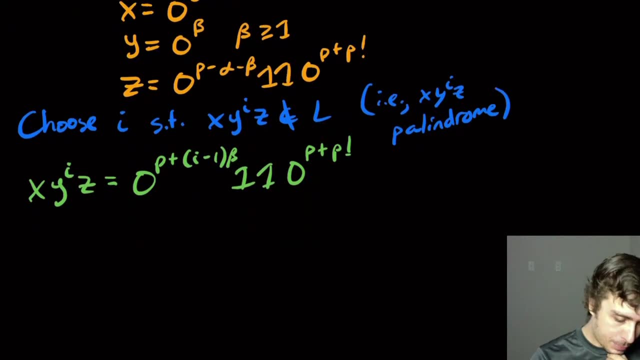 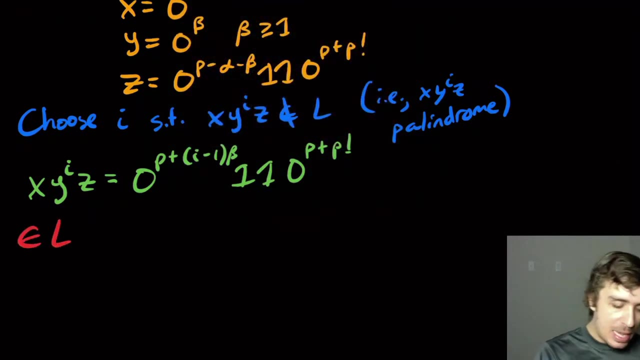 means it already is a palindrome, so the one ones are kind of useful. um, you could have done with a single one instead of two. i just happen to do two here, but, um, okay, so this, what does it mean to be in the language? so it's in the language means it's not a palindrome if, and only if, the two runs of zeros. 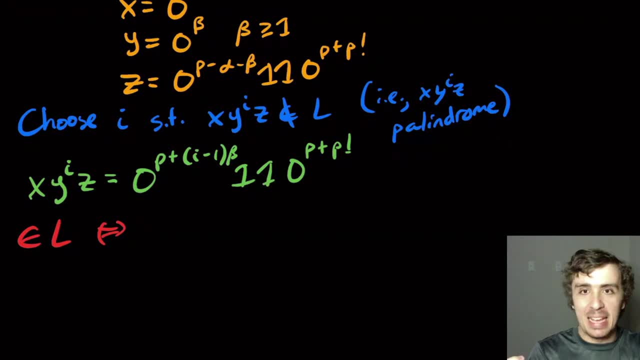 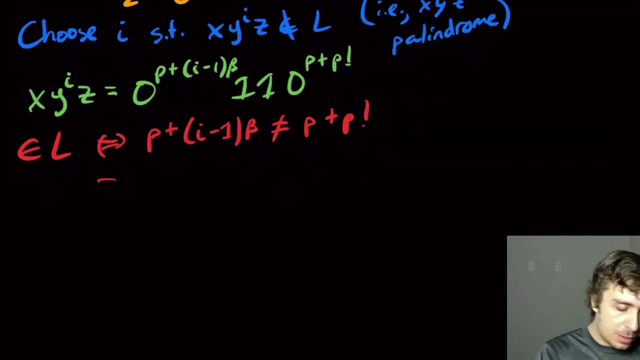 are different because the one ones aren't really contributing anything to whether this thing is a palindrome or not. um, so if, and only if, p plus i minus one times beta is not equal to p plus p factorial. so this is if and only if, if you subtract p from both sides. 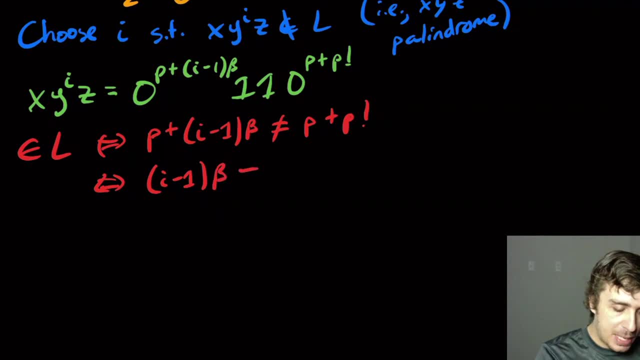 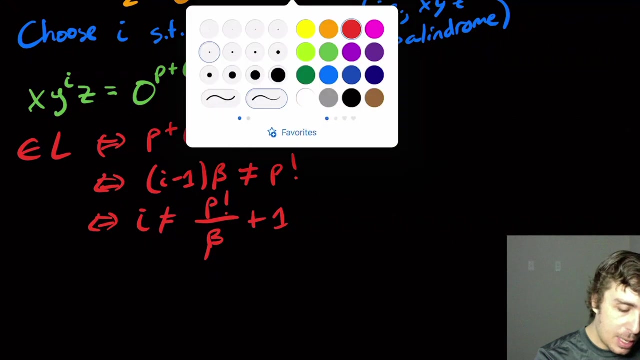 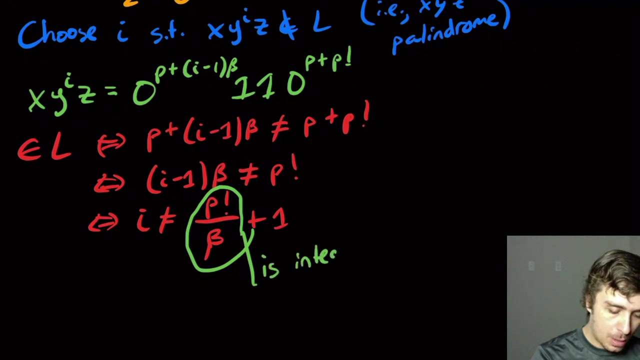 is i minus one times beta is not equal to p factorial. so that means if, and only if, i is is not equal to p factorial over beta plus one. and it's important to note that this quantity right here is an integer. and why is it an integer? 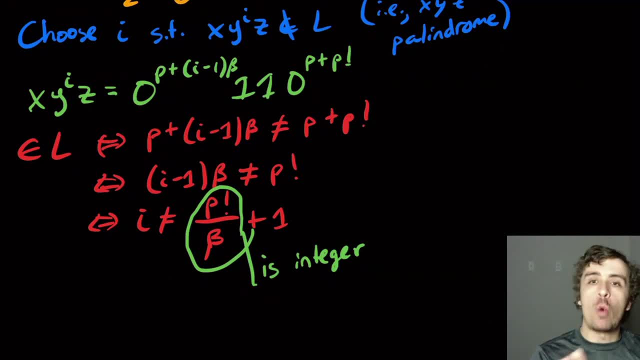 because, uh, beta is between one and p, so p factorial divides, oh sorry, beta divides p factorial, no matter what it is, because it's between one and p and plus one obviously doesn't change whether it's an integer. so let's choose i equal to be that number. so let's choose i equal to p factorial over beta. 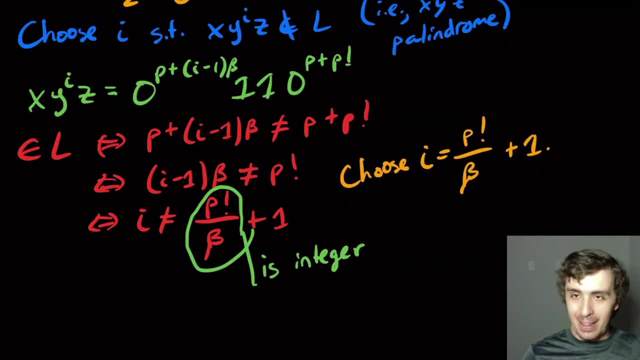 plus one, and that allows us to have an integer that is equal to p factorial over beta plus one. we're just going to have it be a palindrome now. so, because this thing is an energy that allows us to escape the language, the clutches of the language, and arrive at something that is a palindrome. but 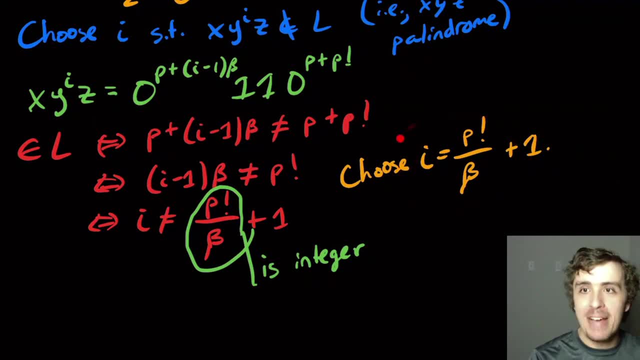 just barely because you have this exactly one value of i that works. it just barely holds on but eventually allows us to to get in there, so that's pretty cool. so this is an application of the p factorial trick to show that this language can be applied to training language to work anything else. 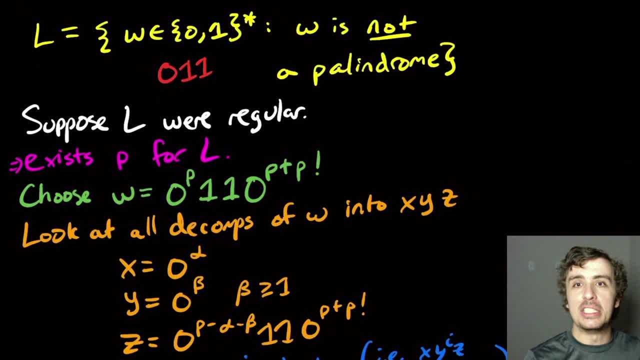 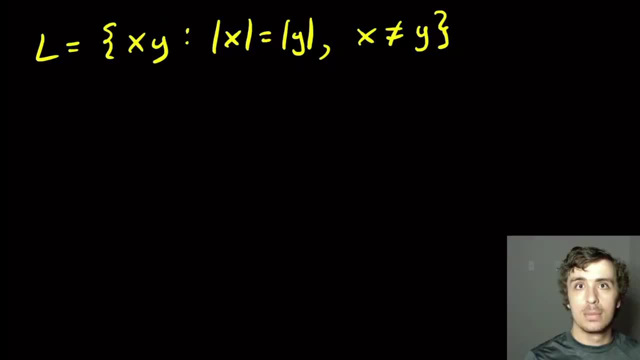 I murderer users. d manager of non-palindromes is not regular. All right, so let's prove that this language is not regular. So it's the set of all strings X and Y. Let's say that X and Y are in. let's say zero, one star. 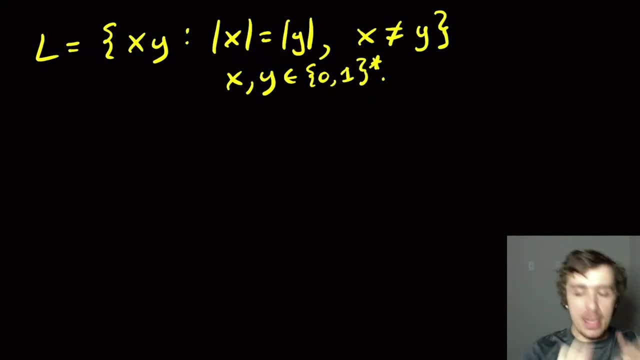 where the two they have the same length and they are not equal to each other. So in other words, this is effectively saying even length strings where the two halves are not the same. Okay, that's all it means. So I've actually done this exact problem before. 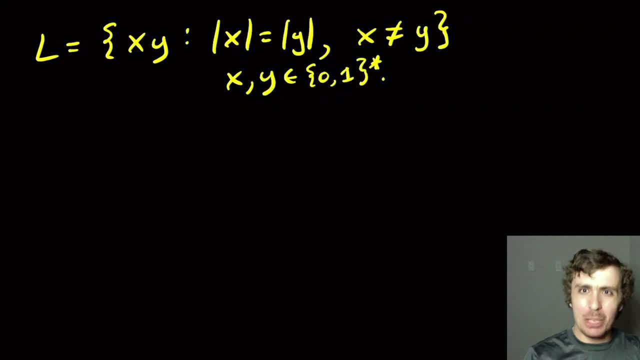 on the channel. you can probably search it, And it's actually pretty complicated proof. I'm just gonna make a single segment on this. So let's suppose that this thing were regular. I wanna show it's not regular. Then that means that there exists a pumping constant. 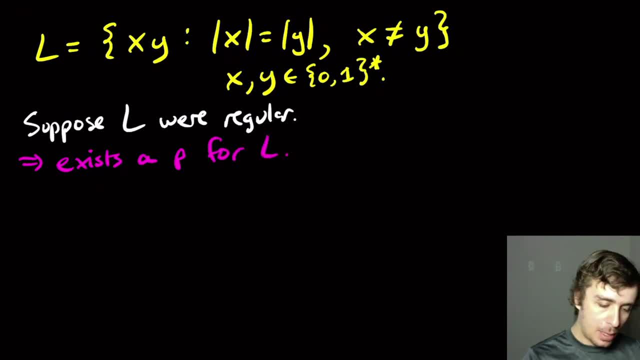 exists a P for this language, L, And what we wanna do, of course, is to choose some string that is in the language. So that means that the two halves are not the same and has length at least P, So we're gonna be using something. 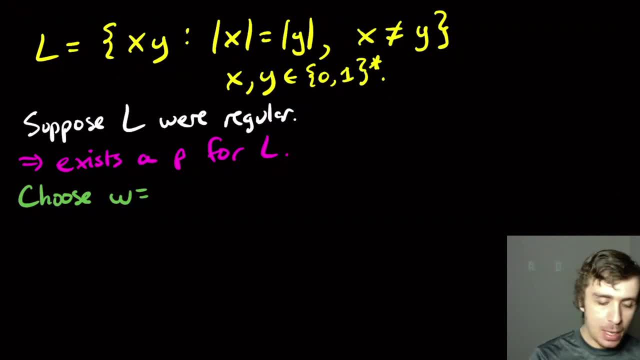 called the P factorial trick. Why am I gonna use such a thing? Because whenever you have something that is not equal and you wanna arrive eventually at something that is equal to- because you need to show that this thing is not regular- you wanna arrive at a string that is not in the language. 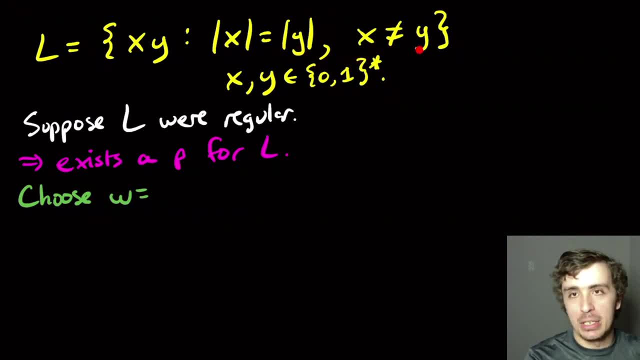 meaning that either the length is odd, but we can't necessarily guarantee that- that the two halves are equal to each other. So I wanna start off with a string where the two halves are not the same and arrive at the strings that are the same. 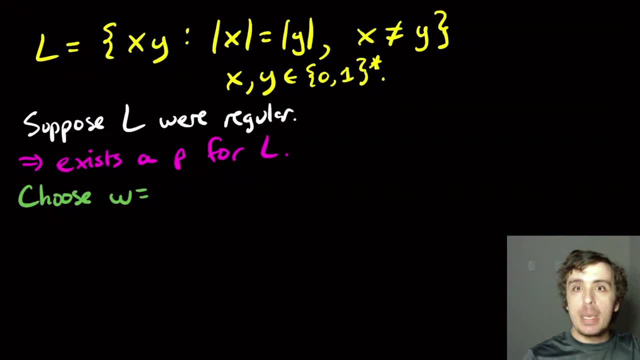 So I'm using the P factorial trick, because P factorial divides any number between one and P. Okay, so that's the reason why, And we'll get more precise on that. So it's going to be zero to the P one. 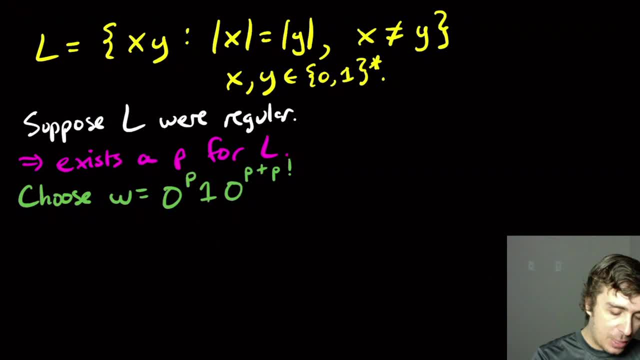 and let's say zero to the P plus P factorial one. Okay, and let's see. So the two halves are equal to one and the two halves are obviously not the same. So let's actually calculate the length of the string. 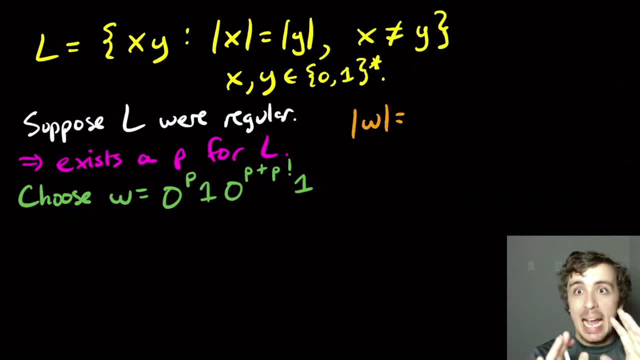 So the length of W, just to make sure that it actually is even. well, we have two ones here, So that's gonna be two plus two, P plus P factorial, because we have two P's and a single P factorial there. So as long as P is at least two, this number is even. 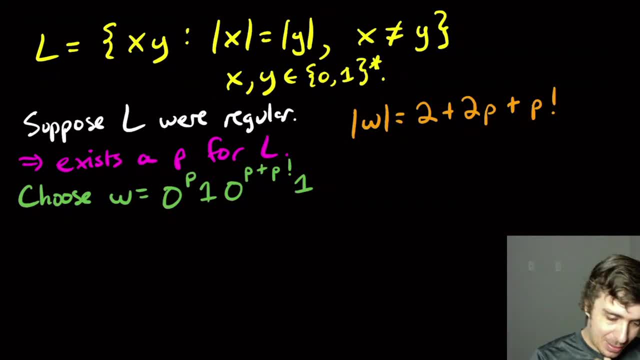 and that's good. So now? so we might as well assume that P is at least two And if it happens to not be at least two, so if P is smaller than two, then we'll set P to be equal to the maximum of two and P 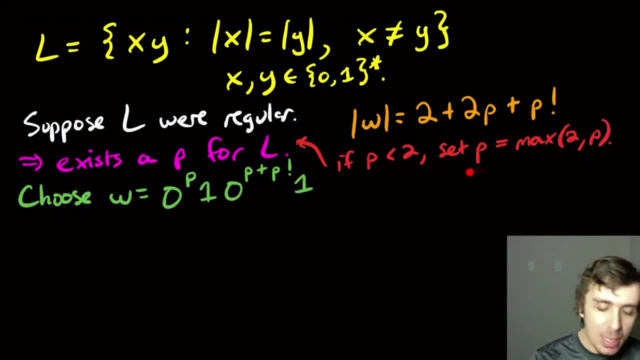 So, as long as it is at least two- And we're allowed to do that because as long as we pick a string, that's long enough anyway and we arrive at a contradiction, we're good. Okay, So we're allowed to do that, because as long as we pick a string, that's long enough anyway and we arrive at a contradiction, we're good. 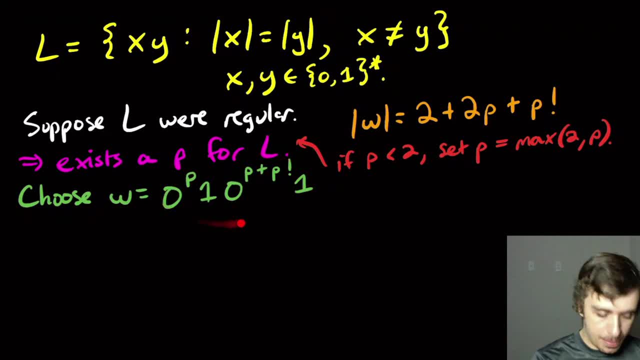 Okay, So we're allowed to do that, because as long as we pick a string, that's long enough anyway and we arrive at a contradiction, we're good. So here, this string is definitely a length at least P. In fact, it's way more than that. 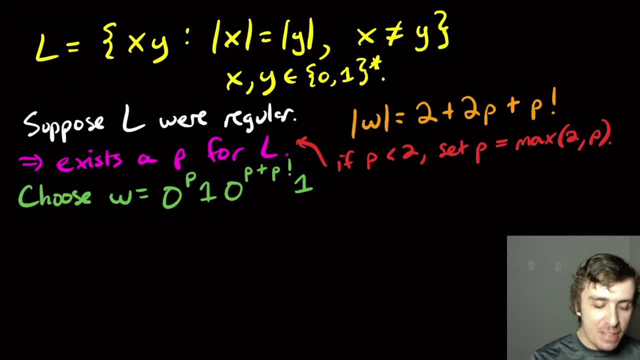 but it's in the language, because it's even and the two halves are definitely not equal to each other because the middle is somewhere in this long run of zeros, And so the first half ends in a zero and the second half ends in a one. 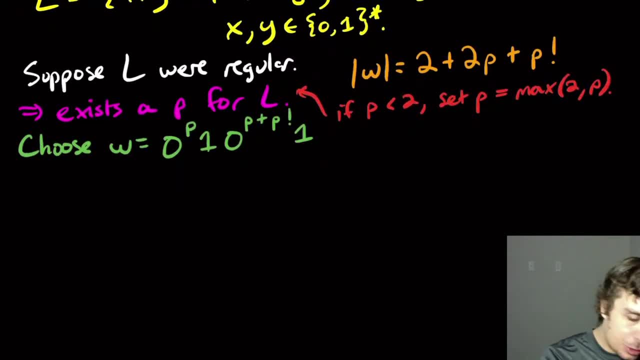 So they can't possibly be the same. All right, So let's try to look at all decompositions. So let's try to look at all decompositions. So let's try to look at all decompositions Then. So look at all decompositions. 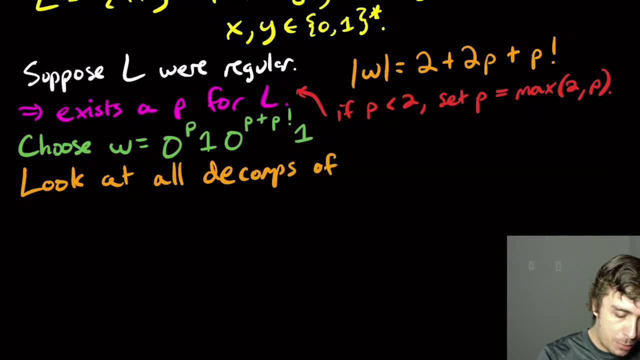 Then. So look at all decompositions Of W into X, Y and Z, and the decompositions look like this. So it's going to be alpha zeros for the X part, beta zeros, let's say, for the Y part. 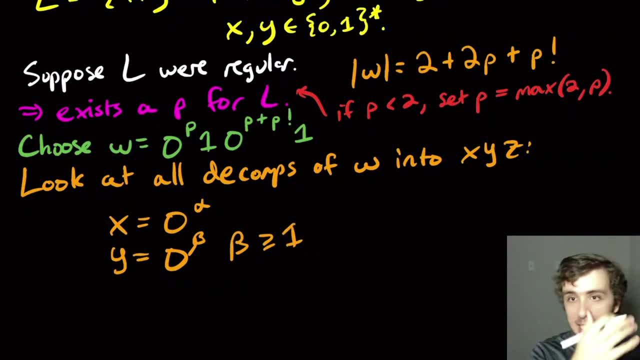 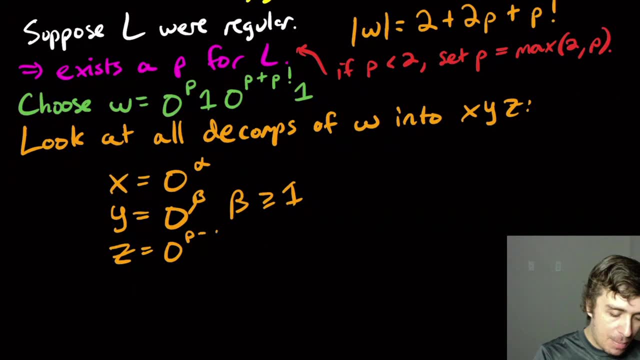 again, these are just any old numbers, because this is any possible decomposition. This is just saying what the length is, And Z is going to be P minus alpha minus P, And this is just saying what the length is minus beta, one. p plus p, factorial zeros and then the one. Okay, so then now we want to pick. 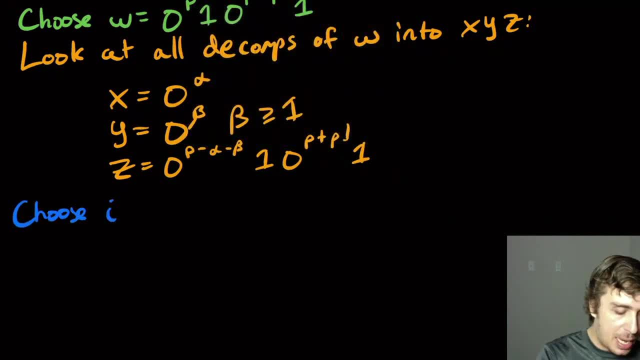 a value of i. so we want to choose an i such that x, y to the i. z is not an l. okay, Because we want to arrive at a string that is not in the language. So let's calculate what the string is. 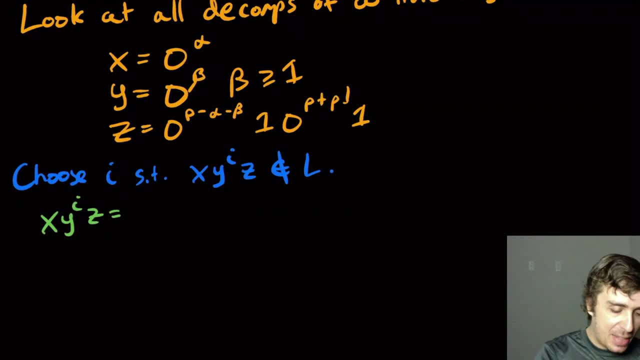 So x, y to the i, z. well, what is that thing? So if we just copy down all the pieces, it's going to be zero to the alpha. that's just the x part. zero to the i beta, zero to the p minus alpha. 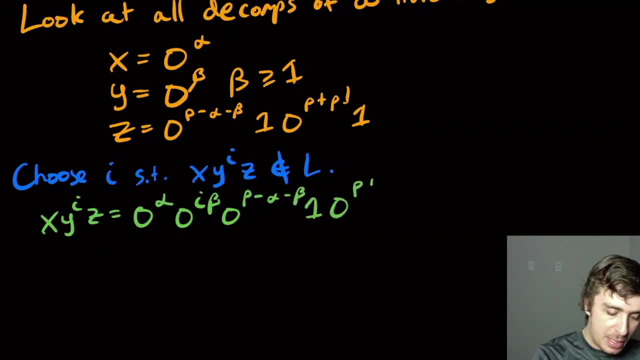 minus beta, and then one, and then this whole mess. Okay, well, here we got a long run of zeros here, so let's collapse. everything Alphas go away. so I'm going to have p plus i minus one times beta one. p plus p- factorial one. So the only way that this could 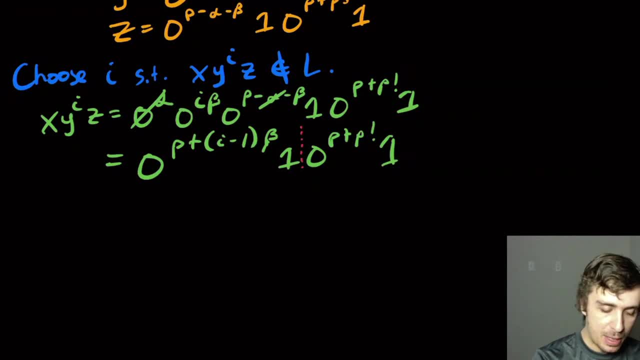 not be in the language is if the straddle point was right there, so the midpoint was exactly there, which means that, because of these singular ones right here, that means that these two runs are the same, So it's nl. if they are different, Okay, so it's nl, if, and only if, p plus i minus one times. 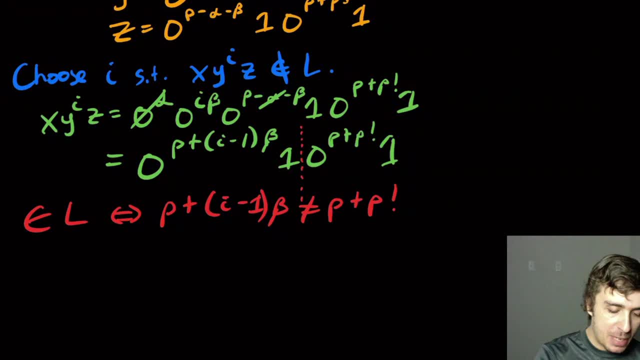 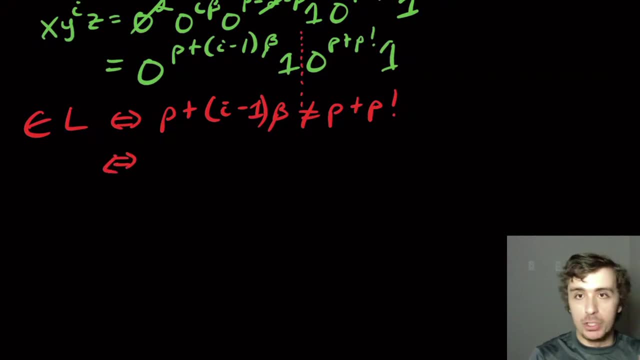 beta is not equal to p plus p factorial. The two runs of zeros are not the same in length. Well, I can subtract p from both sides and that's the same conclusion. So I'm going to get an i minus one times beta. 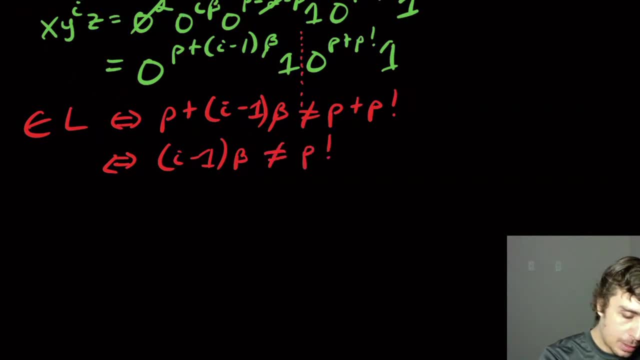 not equal to P factorial. and that turns out to be if, and only if, I is not equal to P factorial over beta plus 1.. It's just rearranging things and it turns out that this thing right here is an integer. And why is it an integer? Because beta is. 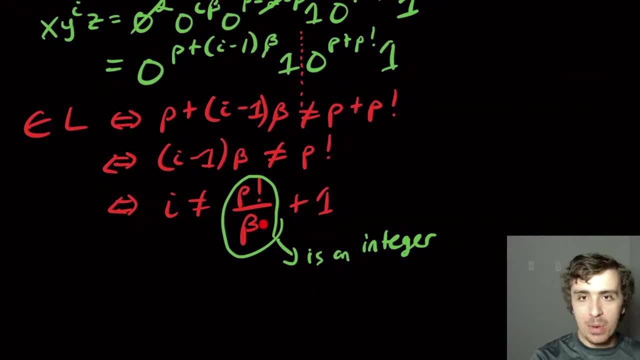 between 1 and P and, whatever that number is, it divides P factorial, because P factorial is 1 times 2, times 3, all the way up to P, and adding 1 doesn't change whether the number is an integer or not. So, crucially, this number is an integer, so it's in L if I is not equal to this, but we 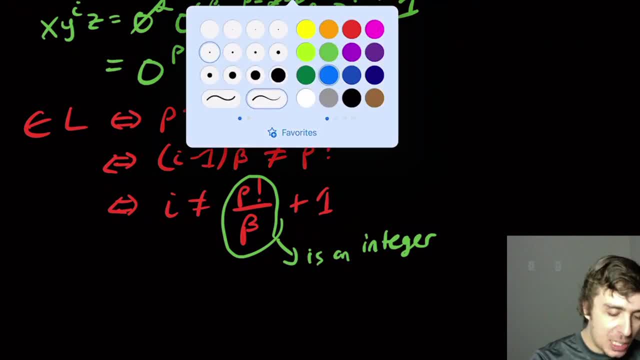 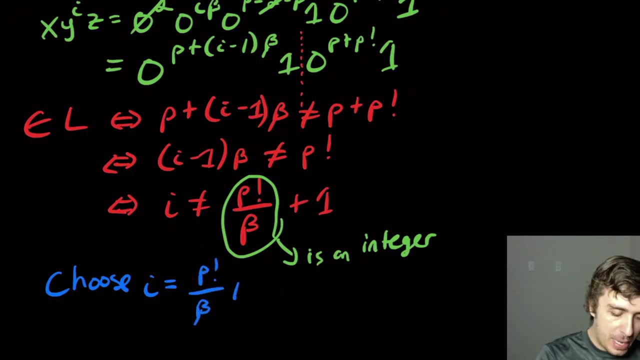 want it to not be in the language. so let's choose I to be that number. So let's choose I to be that number. So let's choose I to be that number. So let's choose I to be equal to P factorial over beta plus 1, and so, therefore, that resulting. 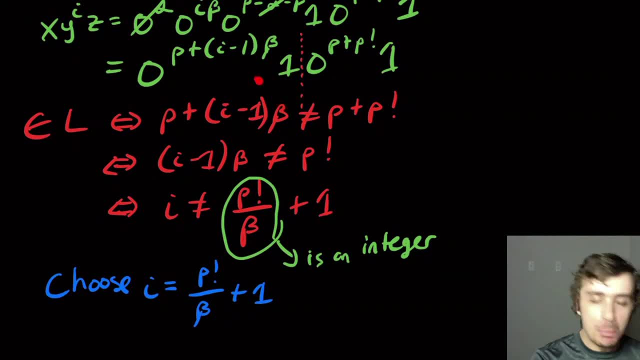 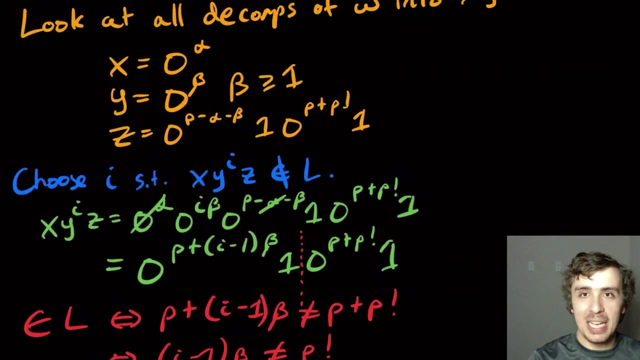 string is: has both sides being equal. Okay, that's the only possibility of these two halves being exactly the same, because they have exactly the same halves, and so, therefore, this string is composed of two things that are exactly the same, which is not what the language says, So note that we didn't. 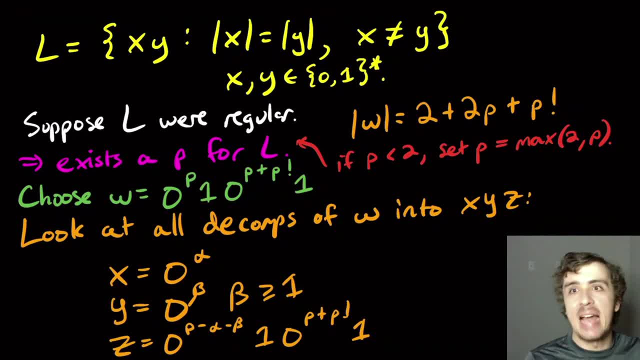 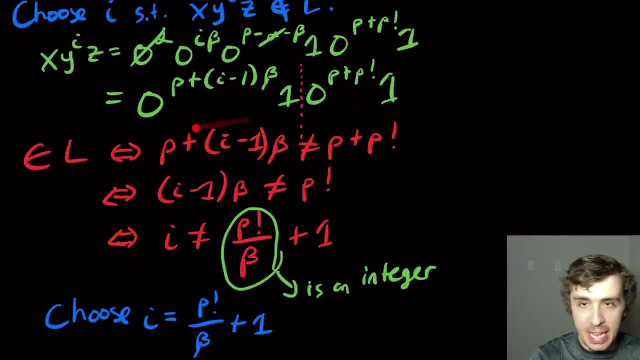 care whether or not we had the same string. We didn't care whether or not we had the same string. We didn't care whether or not this thing was even in length. it didn't actually matter, because if it was odd in length, this thing is not in the language anyway. but we would. we would have arrived there. 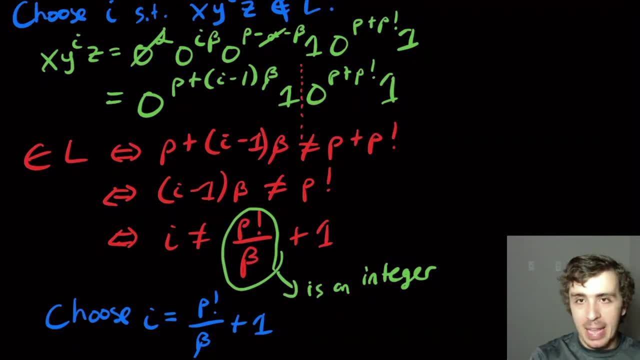 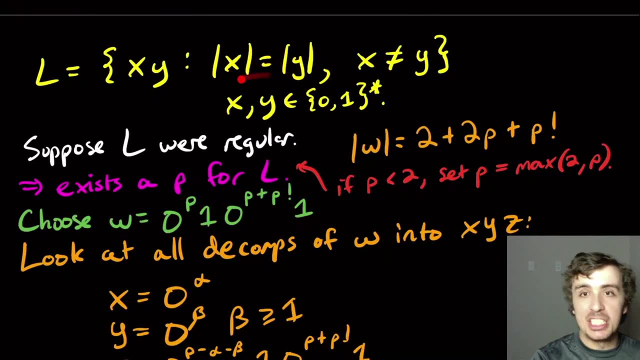 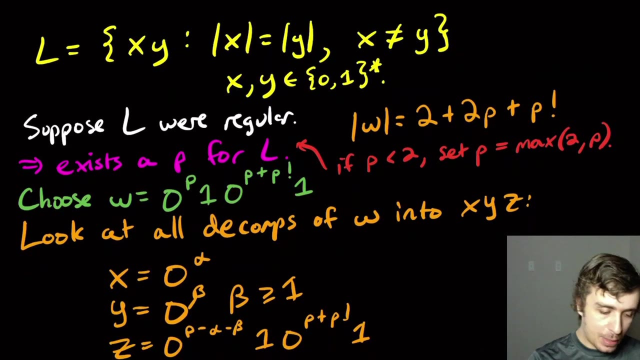 anyway, and this thing is definitely not odd and length anyway, so it doesn't actually matter here, Okay, the thing that mattered is that the two halves had the same length, okay, and here they had to be exactly the same. So hopefully that was interesting to show that this language is. 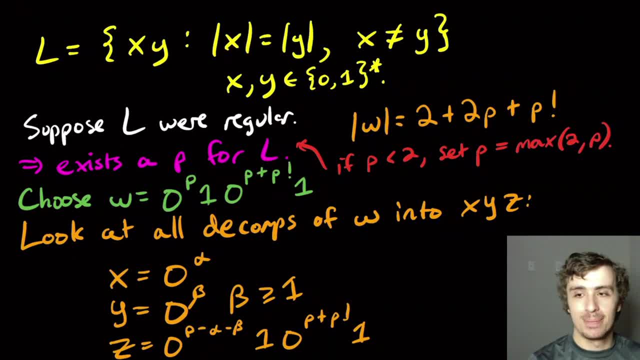 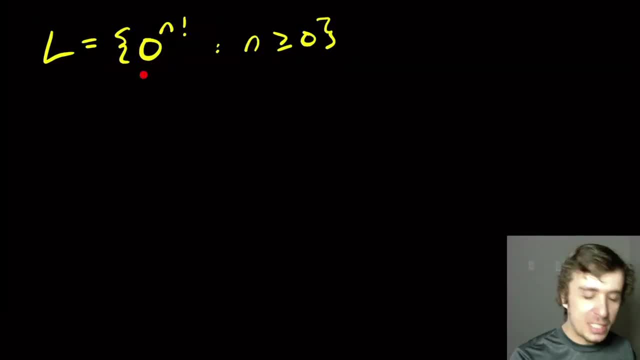 regular using the p factorial trick. Okay, let's prove that this language is not regular. So it's the set of all strings that are composed only of zeros and they have a factorial number of zeros. So zero factorial is one. Well, it's defined to be one, So we would have exactly one zero in here If n is one. 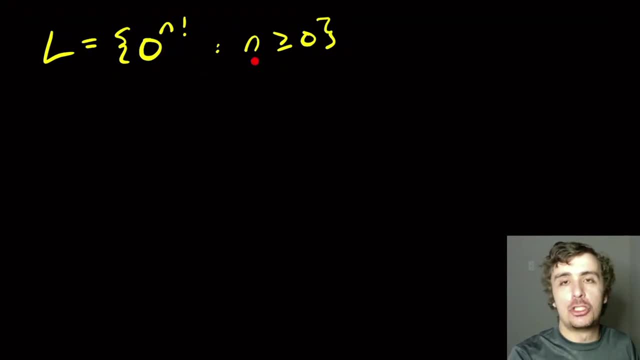 we would have one zero again. If n is two, then this would be two zeros. If n is three, this would be six zeros. If n is four, that'd be 24 zeros, et cetera. So I want to show that. 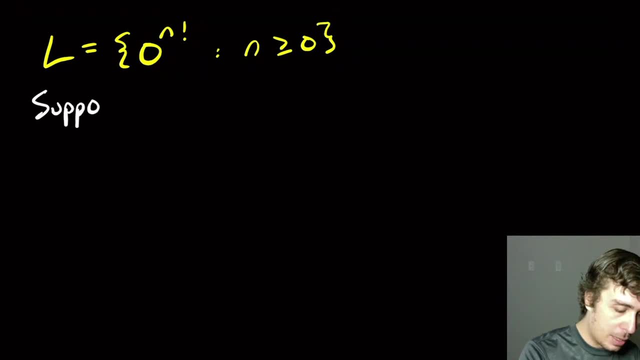 this thing is not regular, So let's suppose that it were regular. Suppose it were regular, then that means that there exists a pumping constant p for L, exists a p for this language, L. Okay. so then now we want to pick a string that's in the language and has length at least p. 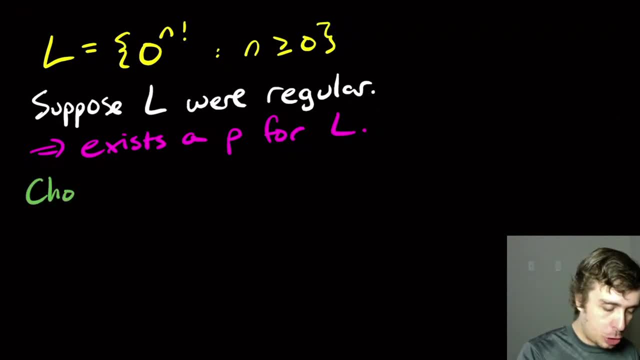 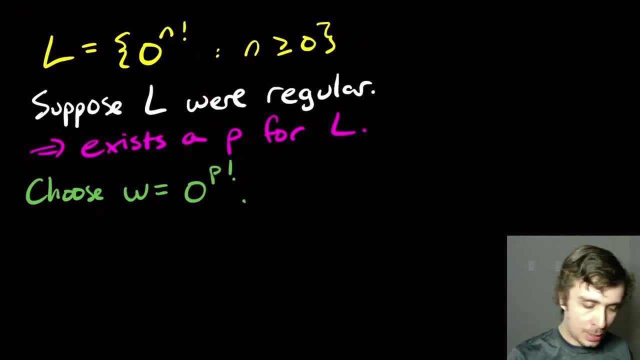 to the p factorial. So let's choose w to be equal to zero to the p factorial. So let's choose w to be equal to zero to the p factorial. So let's choose w to be equal to zero to the p factorial. So therefore, p is in there, Well, p factorial is in here, And p factorial is at least p. So let's. 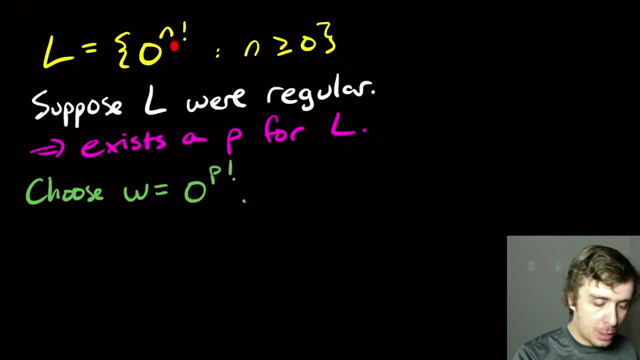 think: Well, those small values. zero, factorial is one, the factorial wins One. factorial equals one, the factorial is equal or larger, and that's fine. Two factorial is equal to two, the factorial is equal Three, factorial is six, so the factorial wins. And then factorial just. 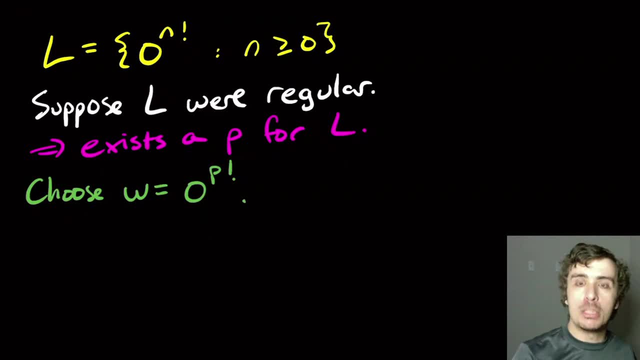 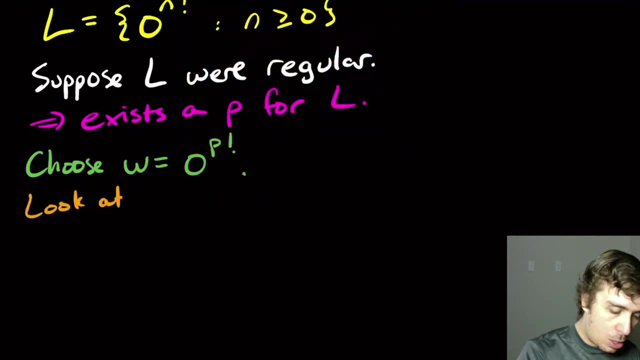 keeps going up and up and up after that, So the factorial is always more than the original number. Okay, so what we need to do is to look at all the compositions of x, y and z, such that the length of x- y is at most p and the length of y is at least one. 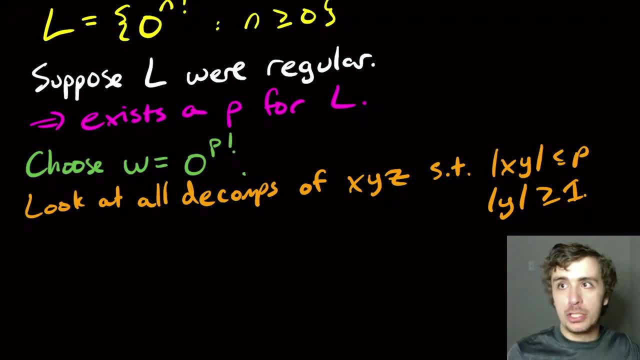 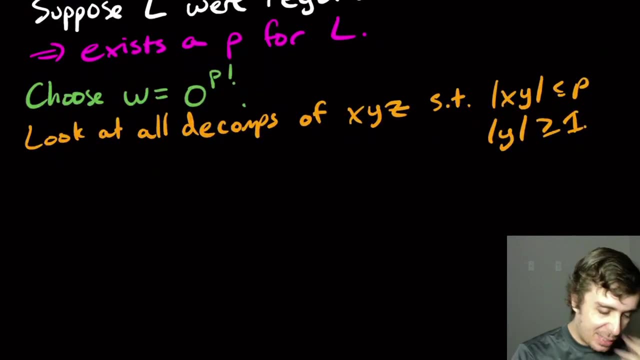 Well, here it's not really as important because the string is all zeros. So therefore we don't really care about what the actual decomposition is. We're just adding some or subtracting some number of zeros into the string. We don't care about the actual string, But let's 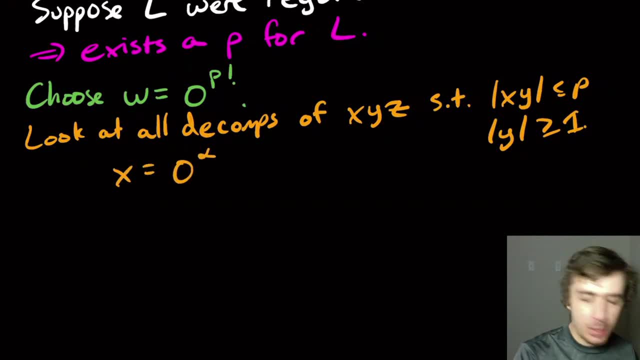 write it down anyway. So x is going to be some number of zeros. since the whole string is zeros, I'm just going to call this alpha. Y is going to be some number of zeros. Let's call it beta. So beta is at least one. let's say: Well, actually that's a rule. 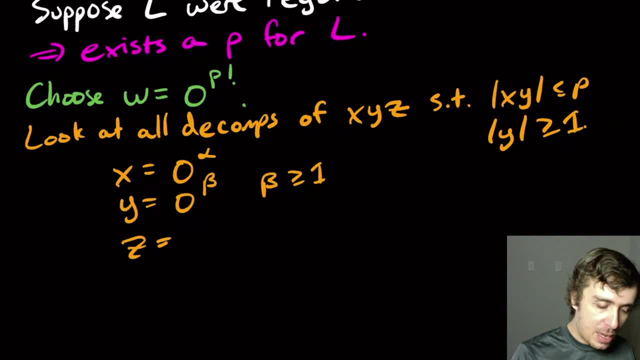 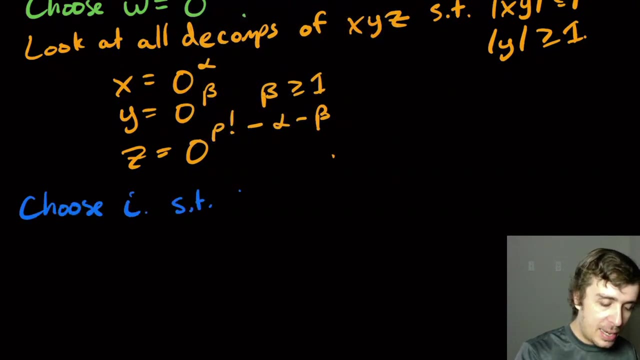 It's a rule over here. And then we have: well, what's the rest of the string? It's p, factorial minus alpha, minus beta, And so what we want to do is we want to choose an i such that x, y to the i. 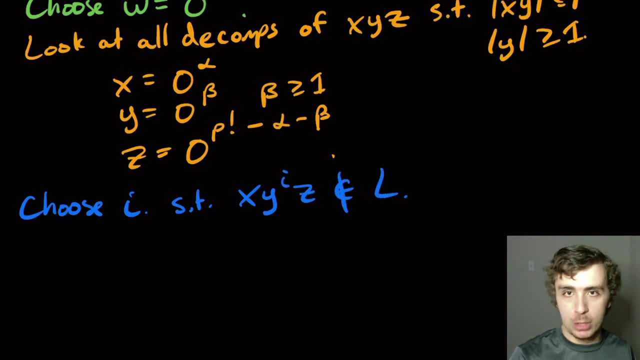 z is not in the language And the reason is that we want to arrive at a string that's not in the language from a string that we had because that would contract. So we want to arrive at a string that's not in the language from a string that we had because that would contract. So we want to. 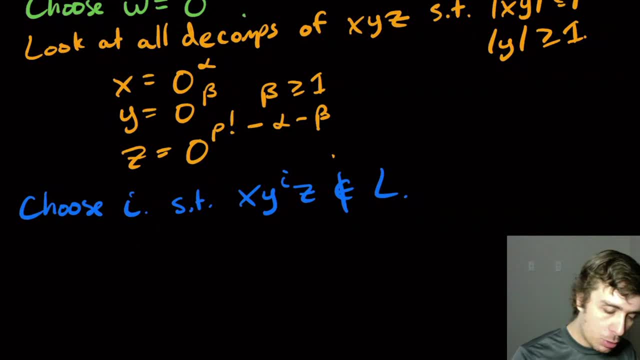 predict the for all statement in the pumping lemma. So let's compute what that is. So that's going to be x, y to the i z, which is going to be zero to the p, factorial plus i, minus one times beta. And the reason for that is the alphas will cancel. I'm going to get an i beta out of this. 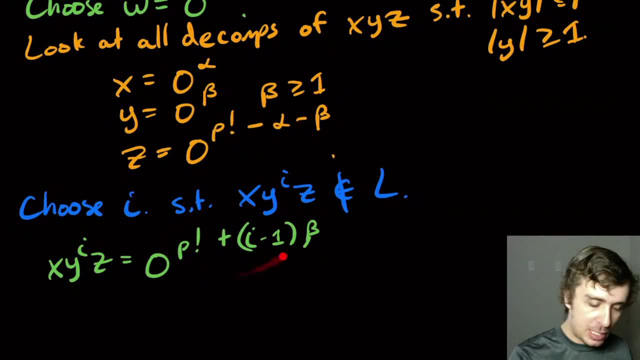 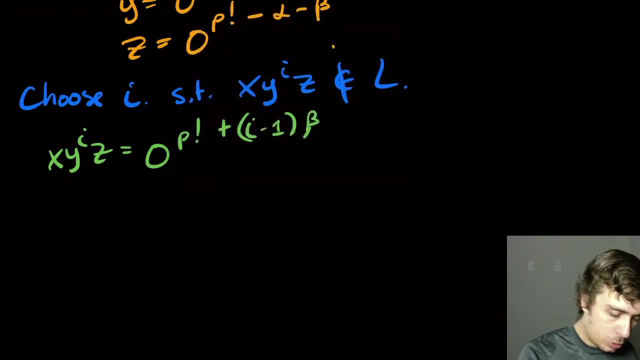 and subtract one beta out of this. So that's what we get here. So therefore, this string is in L. Oops, jump gun. So this thing is in L if and only if. p factorial plus i minus one beta is a factorial of some number. Okay. 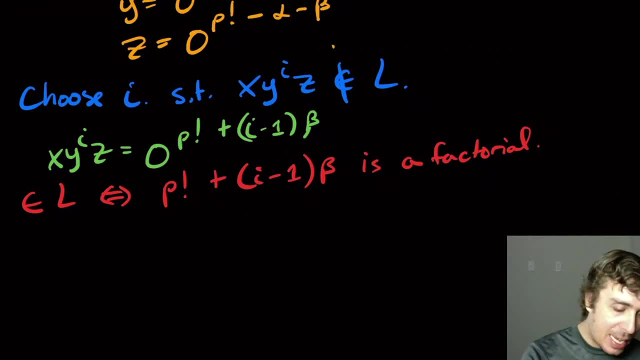 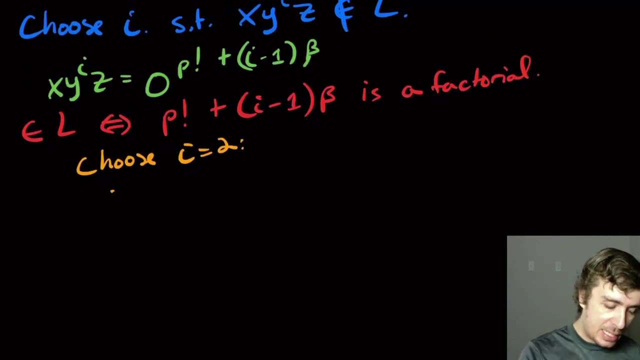 Well, let's see. So if I let's just pick i equal to two, just to see It'll turn out to work, but let's see, Let's choose, i equal to two, Then that's effectively saying p factorial plus a single. 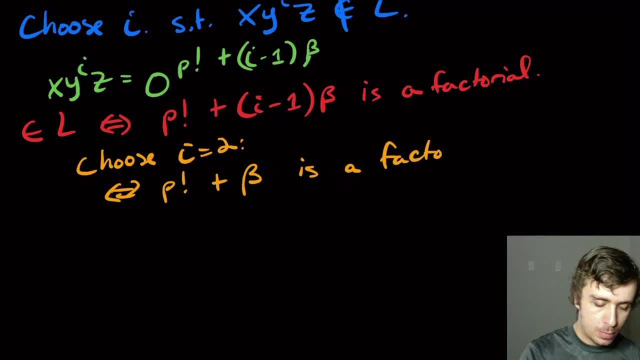 beta is a factorial. Well, we know that beta is at least one, So it's not equal to that factorial, right there. So let's, let's write that down. So p factorial is strictly less than p factorial plus beta, because beta is at least one. So let's write that guy down. So that's because. 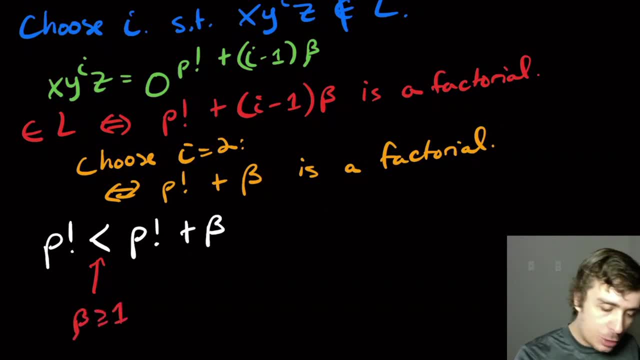 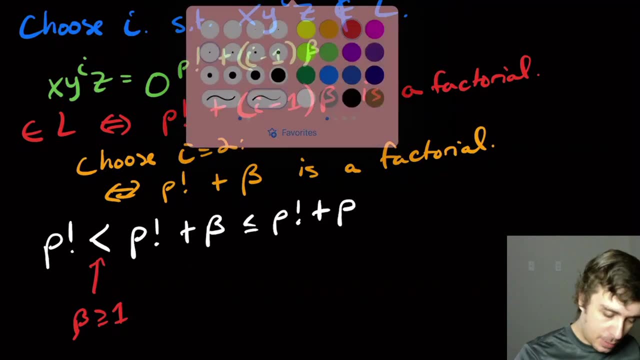 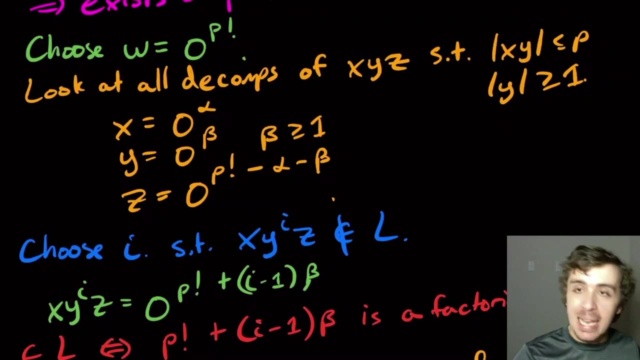 because beta is at least one, It turns out to be at most p, factorial plus p. And- and you may say, okay, where did that come from? Beta is at most p. Well, the condition of x, y's length being at most. 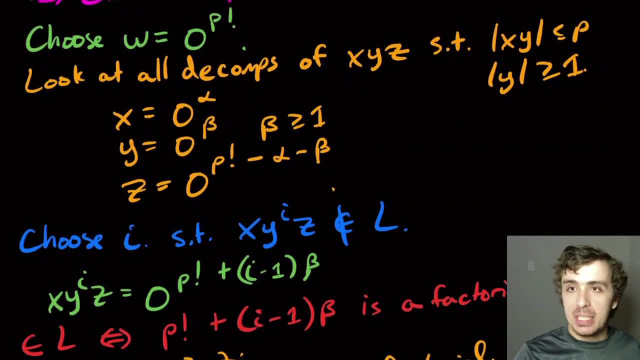 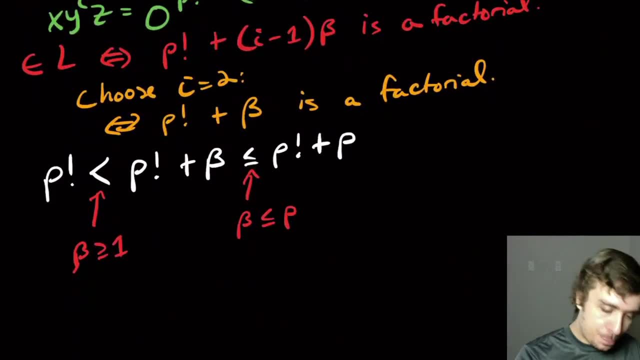 p. way up there on the right. That effectively says that the length of y is at most p, because x can't subtract anything out of it, out of the length. So, um, that's at most that. Well, what is the next factorial? 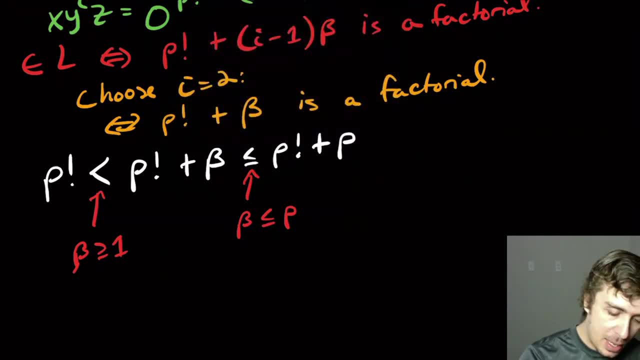 So that's gonna be. that's gonna be P plus one whole thing factorial, which is equal to P times. oops, my mistake. That's P factorial times, P plus one. That's just what it's defined to be. So if it's the case that this thing is strictly less than 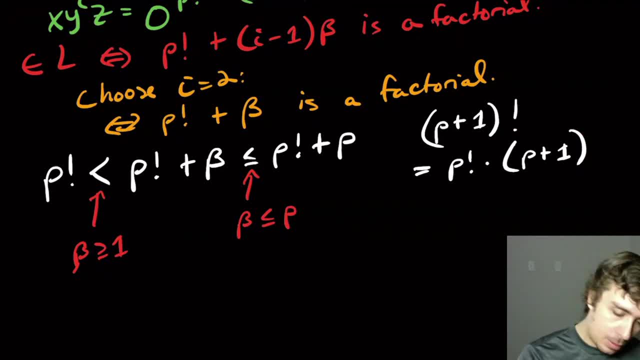 this, then we're done. Well, let's see. Well, we can actually kind of see this, because adding P versus multiplying by P plus one is has this clearly gonna be way bigger than just adding this. So it's adding a small number compared to the factorial.